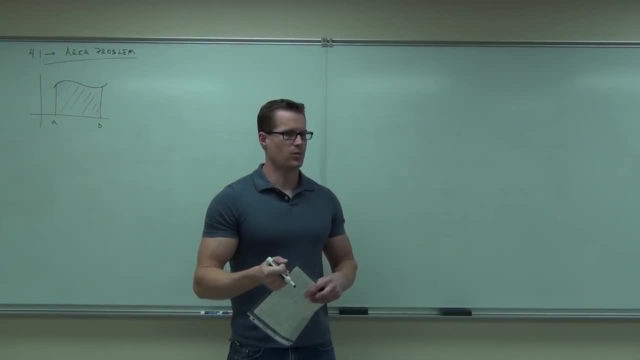 And then we'll talk about what's called the antiderivative method, which is a more concise way to do it. Are you ready for it? So this, I'm going to kind of go in a weird loop. I'm going to introduce this with the rectangular method. We'll talk about antiderivatives, antiderivatives. 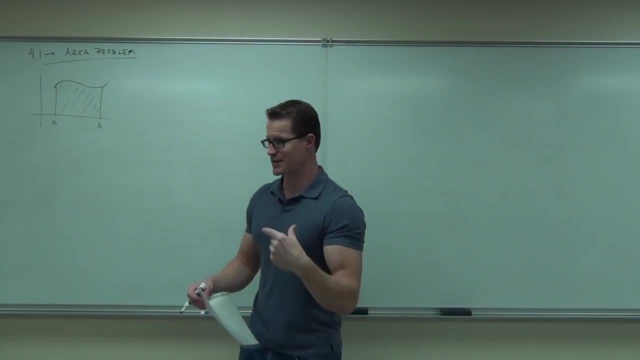 Then I'll use rectangular method to kind of prove what we just learned about antiderivatives. You follow me, So we have to wait until 4.3 to prove some of the stuff I'm talking about here today. I'm going to give you kind of an intuitive approach on it, though Hopefully it makes sense for you. 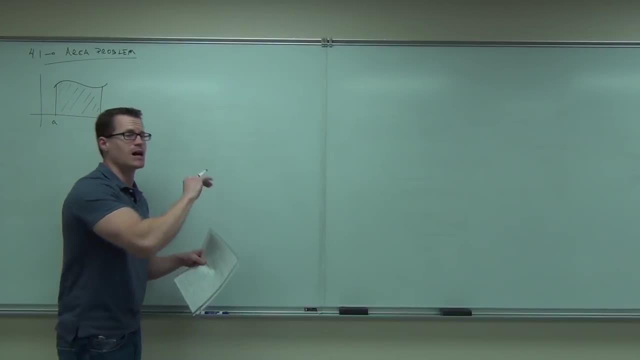 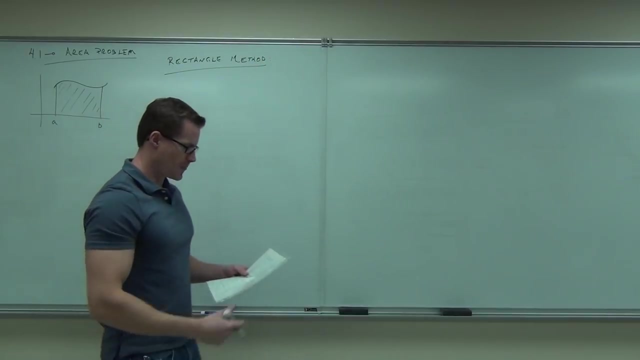 So, first method, let's talk about the rectangular method and at least the idea behind it. So the rectangular method, the rectangle method says: well, why don't you divide your interval into n, some number? n equals subsections, equal, equal as far as their width goes. 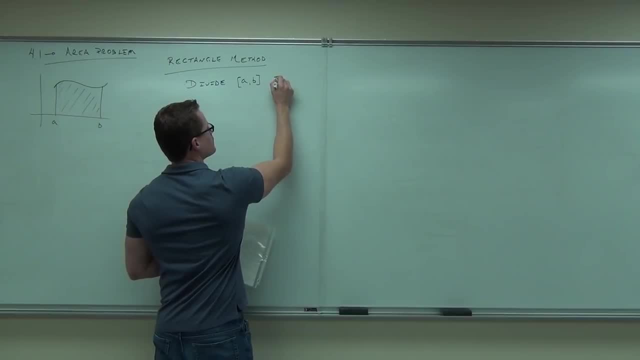 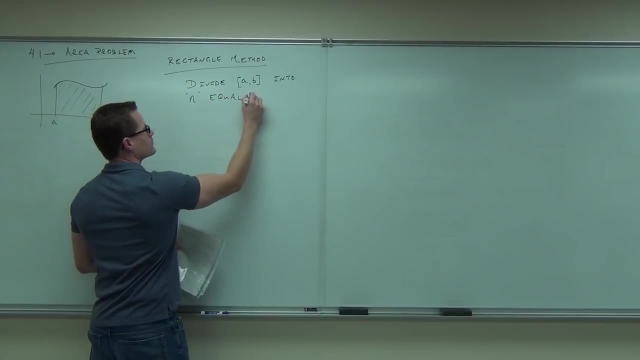 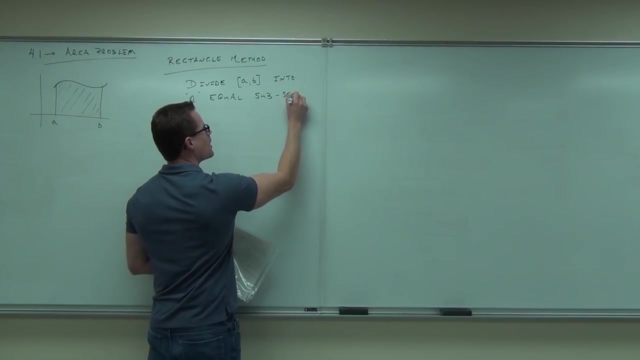 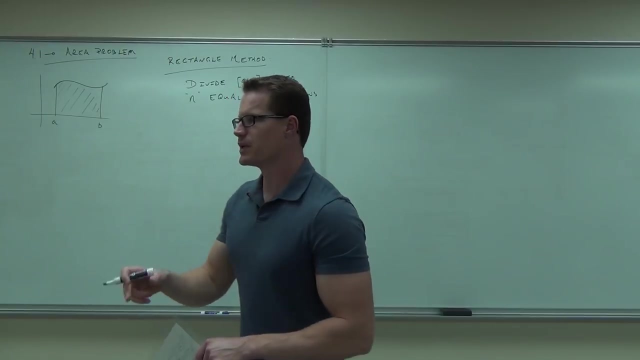 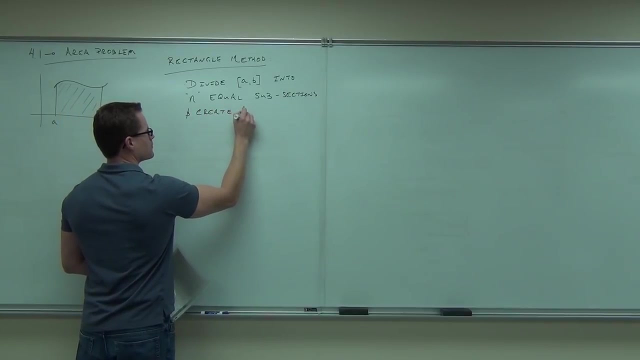 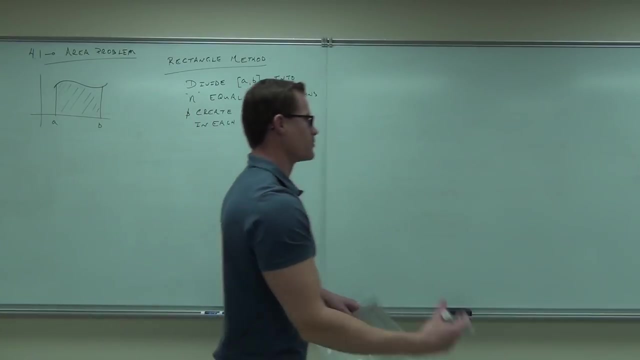 Subsections equal as far as their width goes, Subsections equal as far as their width goes, Subsection, subintervals, whatever you want to call it, and create a rectangle in each subinterval, in each subsection. Hence where we get the term rectangle method or rectangular method. 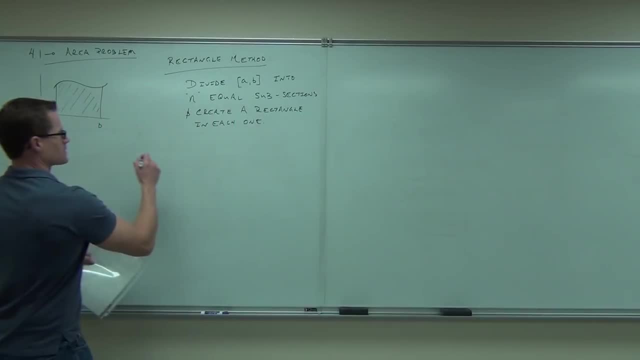 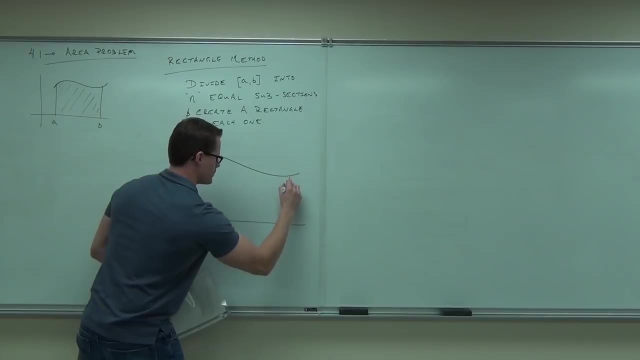 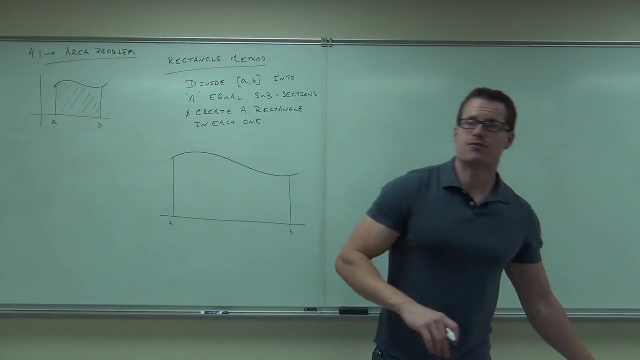 So here's basically the idea. Let me redraw the picture for you. Let's say that I make this a little bit bigger too. Here's my graph, Here's my interval. The idea behind the rectangle method is: can you find the area under this curve the way? 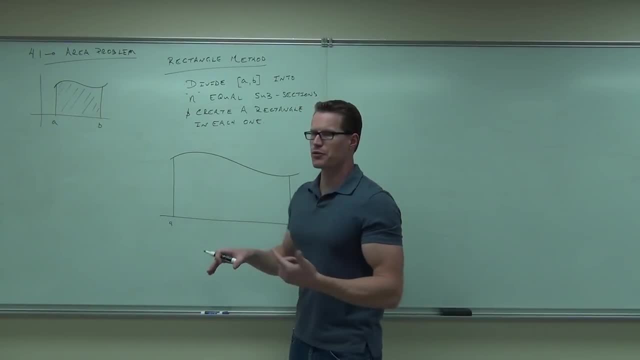 it is. No, not really, because we don't have a formula for this. and even if we did, it doesn't have straight sides, And the only way we know how to take an area, until right now in geometry, is if a figure 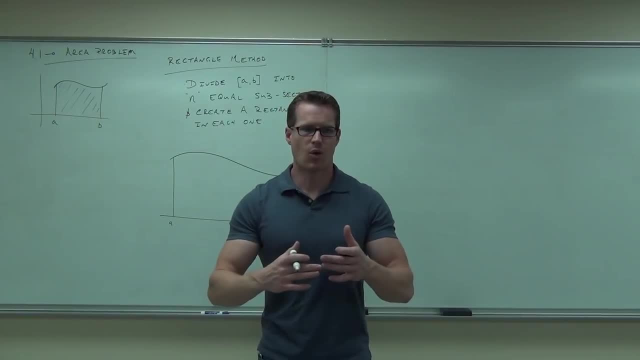 has straight sides, right, whether we break it up into rectangles or triangles, because we know how to take the areas of those figures. or perfect circles, we know how to take the areas of those figures. This, this, is not a regular shape that we know of. it's just some random function. 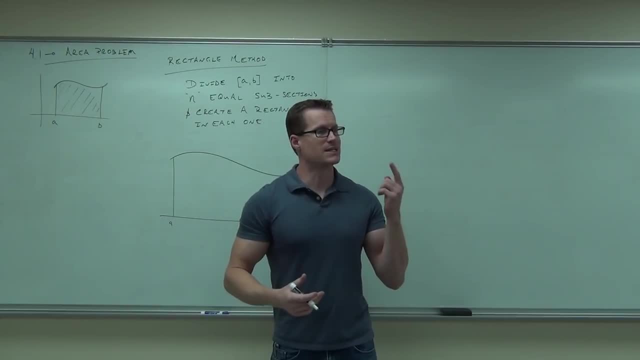 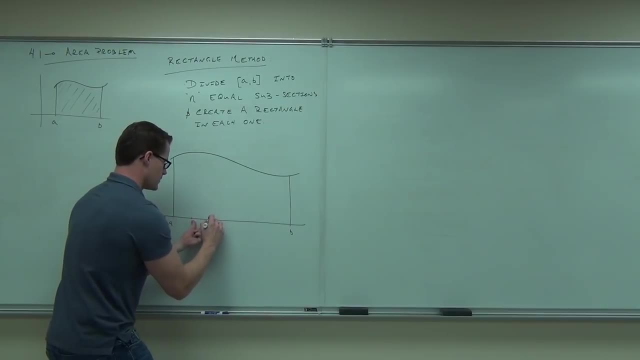 In fact, I haven't even been specific. it could be any function, But the idea is, let's go ahead, let's break this up, We'll say: okay, we're going to split this up into however many parts we choose. 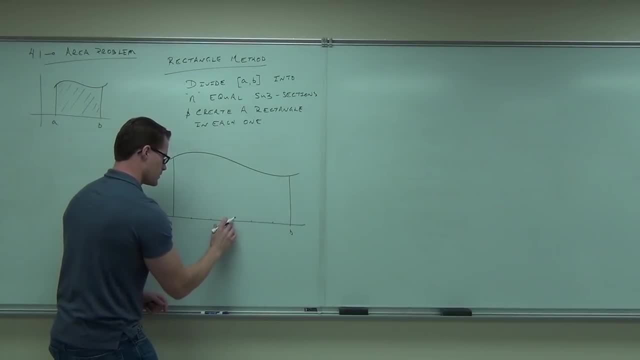 Let's just assume those are equal widths. That's about right. It says: if we have some sections here, what we're going to do is we're going to divide them into parts. What we're going to do in each section, since they have equal widths. I'll tell you why. 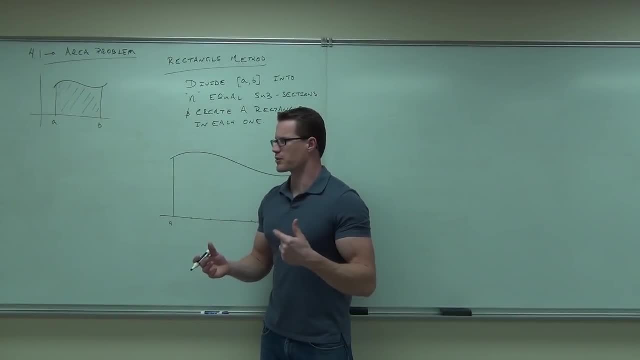 we need equal widths later on in section 4.3, 4.4, but right now let's just assume we have some equal widths, so our bases are all the same, our rectangles. equal bases means they're easy to add together. 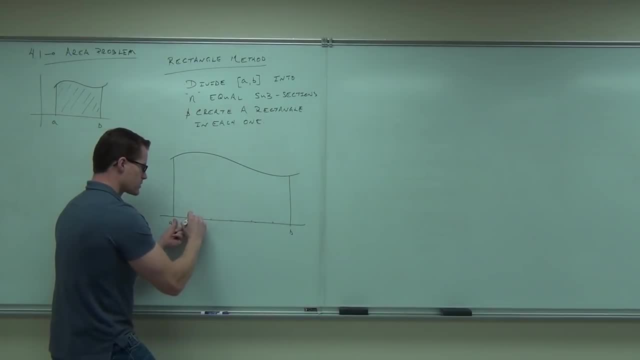 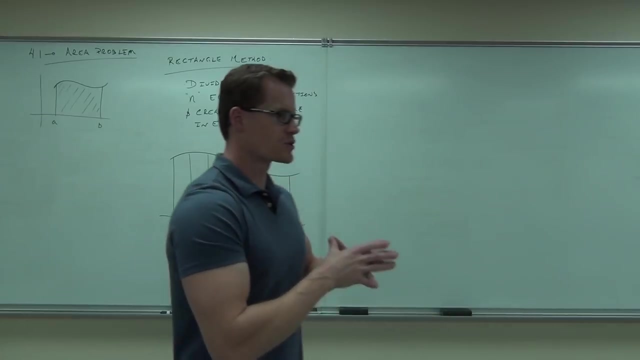 That's basically it. So for each interval, subinterval, let's make a rectangle. Now, there are several ways to do this. I'll show you one way. I'll show you one way. Okay, The problem is now you've got to determine how you're going to have the height of a rectangle. 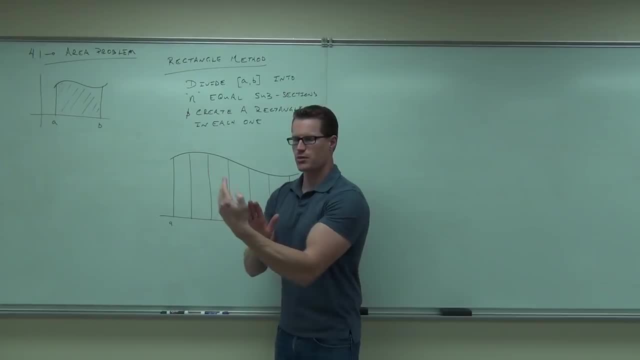 So one way to do this is to use what's called left endpoints. another way is to use right endpoints, and a third way is to use midpoints. And here's what that means: You go to the right endpoint of your interval. here's my interval: I go to the right endpoint. 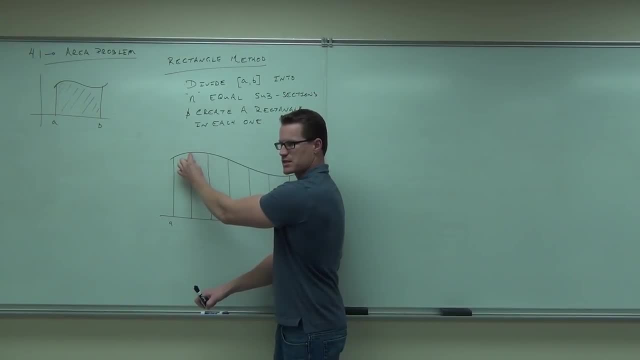 and say: I'm going to go to where that touches my figure. Does that make sense to you? A left endpoint would say: I'm going to go up to where my left point touches my rectangle. A midpoint would say: go to the middle, see where that touches the figure, and then make. 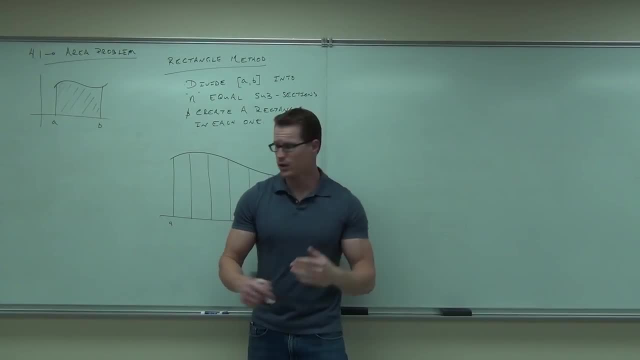 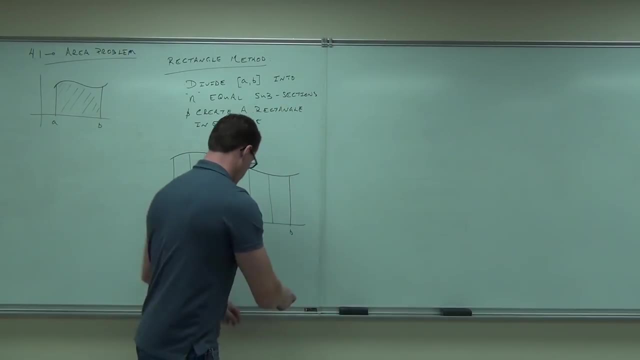 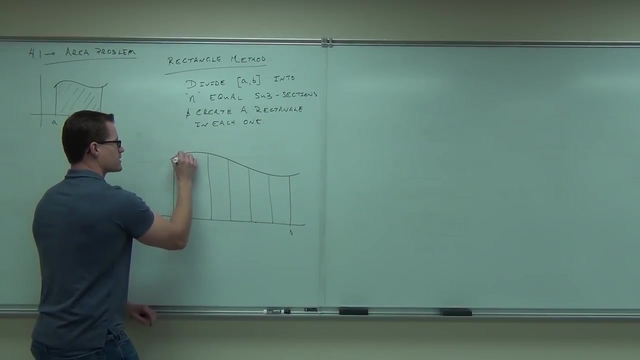 your rectangle. That would determine your height. So we have left endpoints where that touches, right endpoints where that touches, or midpoints. Let me show you the midpoints and here's how you do it. Okay, from my midpoint I go up here where it touches that f of x, wherever my function. 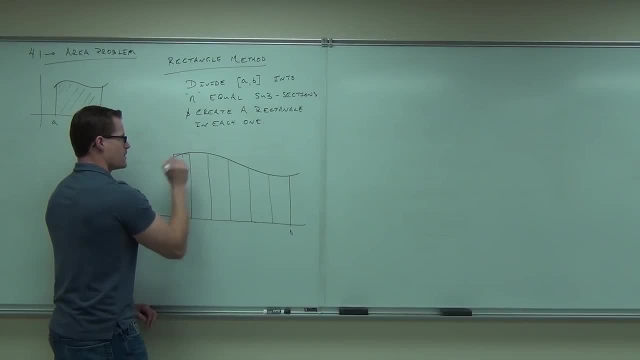 is. That's where I cut it off and that makes my rectangle. Does that make sense to you? Why do that? Well, it's actually not going to matter. when we finish 4.4, we'll talk about what's called. 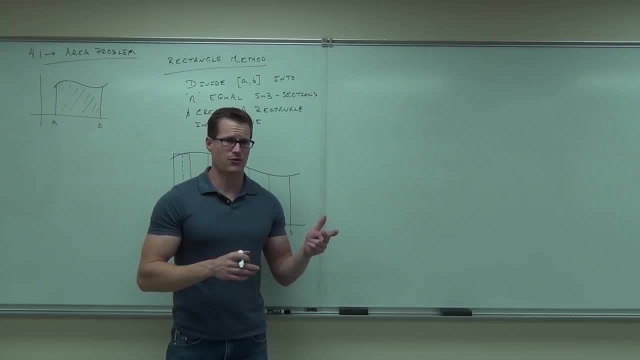 the definite integral. It doesn't matter whether you use left, right or center, But for us, if we are always using one endpoint, sometimes you can systematically over or underestimate the area, and that would be a problem for us- Then this one would go: okay, let's go up. 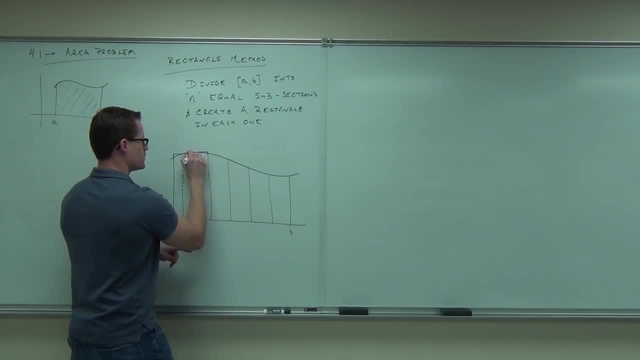 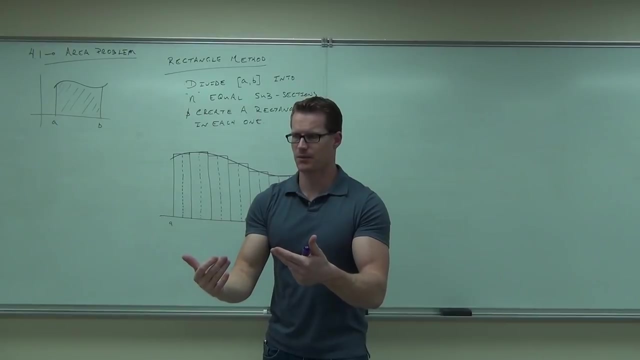 Where that touches, I'll draw the top of my rectangle, finish it off, And you would do this for every interval that you have. How many of you feel okay about the idea here, the idea of drawing rectangles there? Do you see where the midpoint's coming into play here? 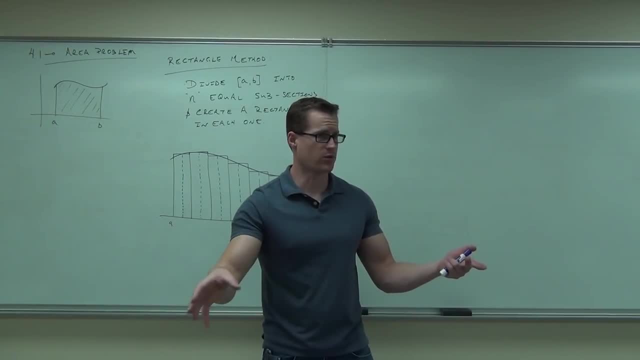 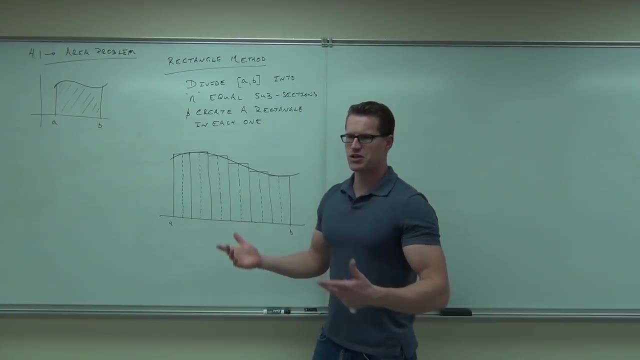 The midpoint gives us the height of our rectangle. That's going to be useful when we get down to 4.3 and 4.4, very useful Now. how would I find the area of this figure, the approximation of this area? 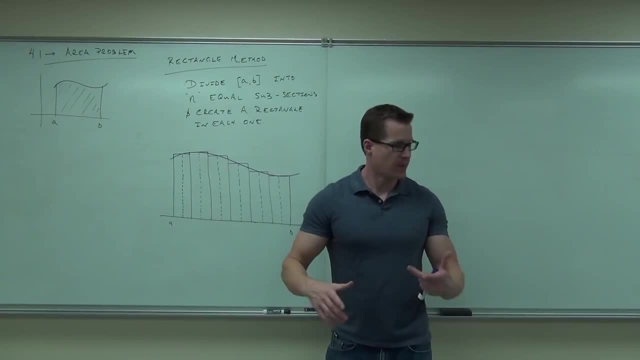 What would I do with this? If we know the area of a rectangle, which we do? right, a rectangle is just a geometrical figure. If I can find this area and this area and this area and this, if I can find all the 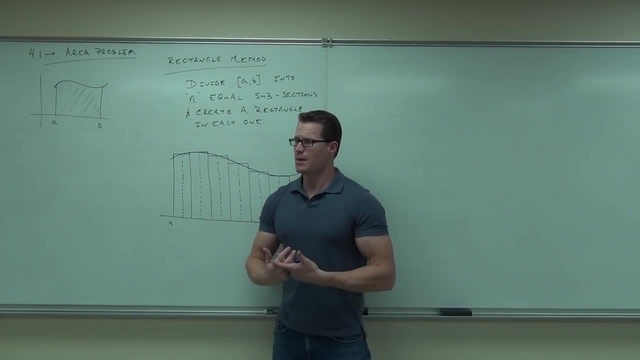 areas of all my rectangles. all I have to do is add them together And I'm going to get at least an approximation of the area of my figure. You follow me Now. is it going to be exact? Well, you can tell it's not. 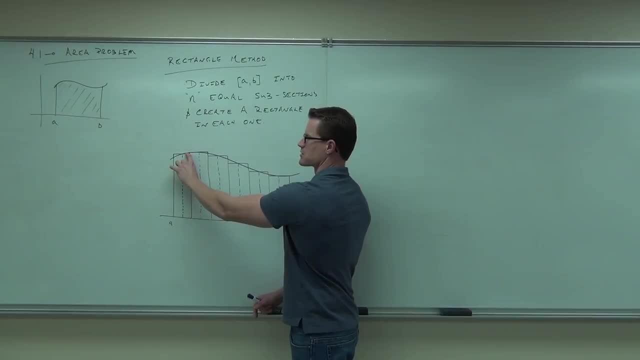 I mean, sometimes I've overestimated, sometimes I've left out some area, Sometimes it's about right, But sometimes- and I don't know whether I'm perfect or not, So I'm not going to be exactly right- It'd be a miracle if it was exactly right. 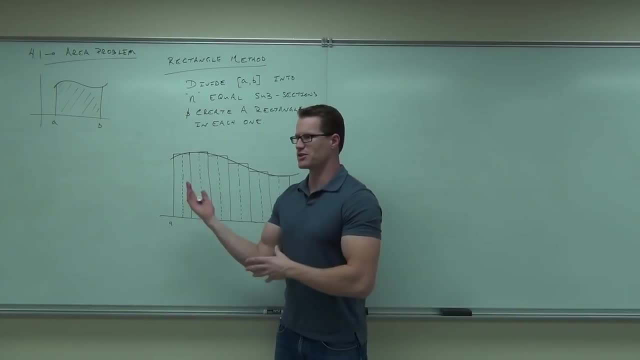 It's not going to be a miracle. This isn't Harry Potter mathematics, so magic doesn't happen in math sometimes. But anyway, That's another topic. I suppose It's not going to be exact, It's going to be an approximation. 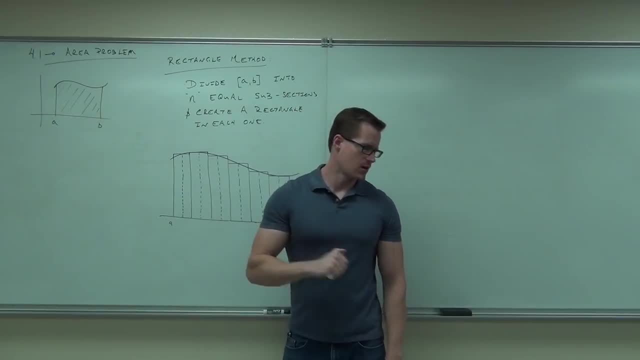 Now the question is: how can I make this better? So would you agree that the more rectangles I have, the better approximations will be? So I mean here I had one, two, three, four, five. I had six rectangles. 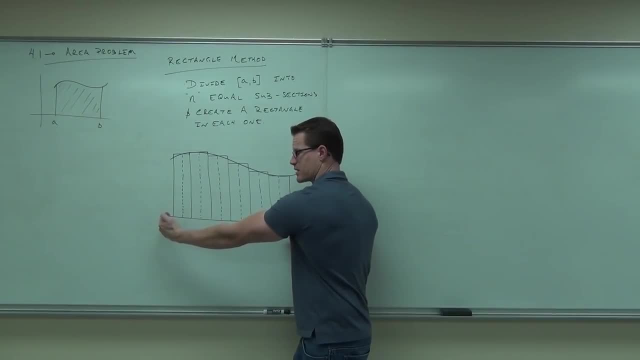 If I had 100 rectangles for the same width, 100 rectangles mashed up in there, I'm going to over, underestimate by a less margin, lesser of a margin right. So the more rectangles I have, the better approximation becomes. So as the number of rectangles n goes to infinity, or as the space between the rectangles. 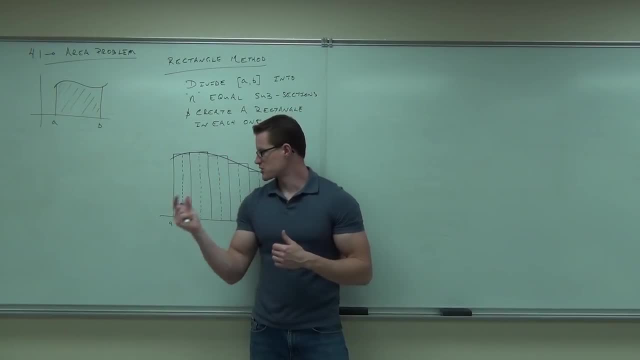 goes to zero, Right? Does that make sense? As the space, as this, goes really really close to zero? that's the idea of a limit. As that goes to zero, then I have a very, very good approximation. In fact, it's so good that it's exact. 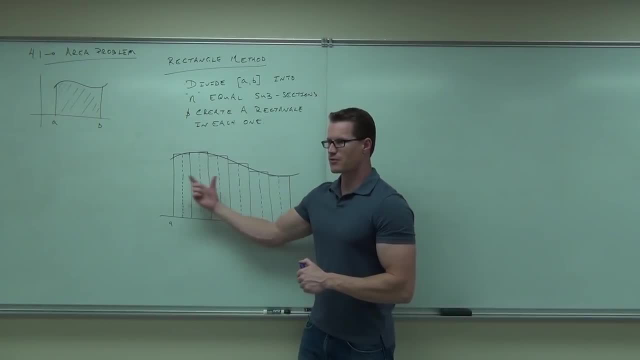 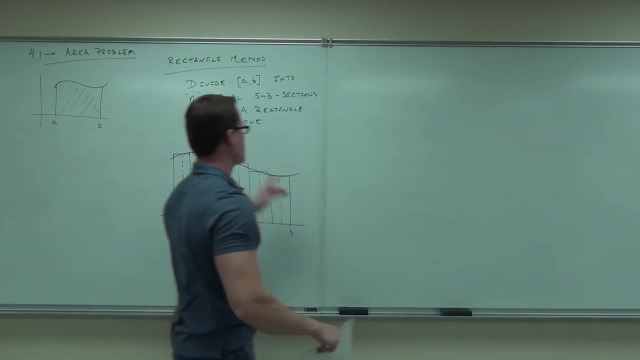 So the idea here is: cut your region into rectangles. Every rectangle you're going to have, Eliminate the area of that. Add all the rectangles together and you're going to get a good approximation of your figure. How do I make it better? You let the number of rectangles go to infinity. The way you do that is let the space between them go to zero For a better approximation. 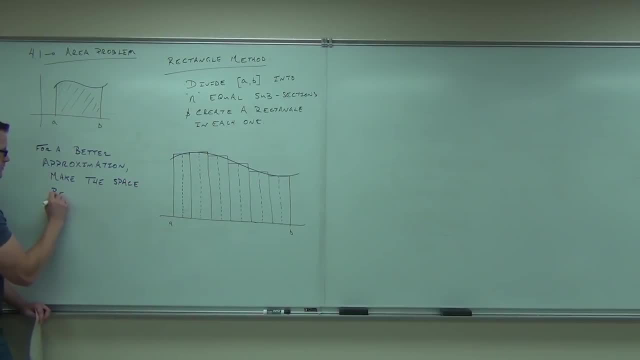 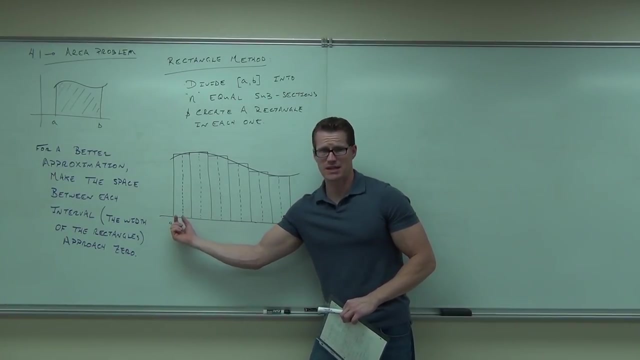 will go to 0,. how many rectangles are you going to have If you have a finite space and you 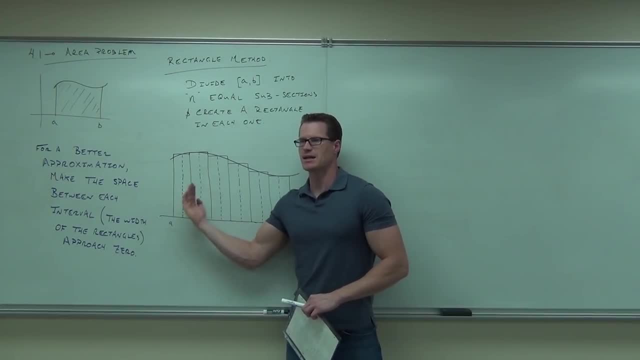 let the distance between here and here go to 0,. you can pack in an infinite number of rectangles, right? If you pack in an infinite number of rectangles, you will have no over or under estimate. It'll basically be like finding the area. 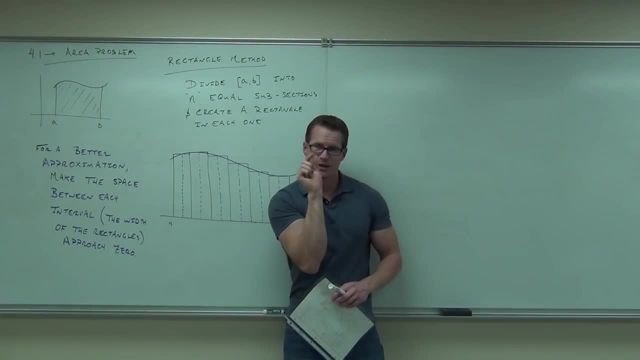 under a distinct point, which is impossible. You can't do that. But if you say it's really really, really small and you can't even put a paper between it, then it'll be exact. That's the idea. 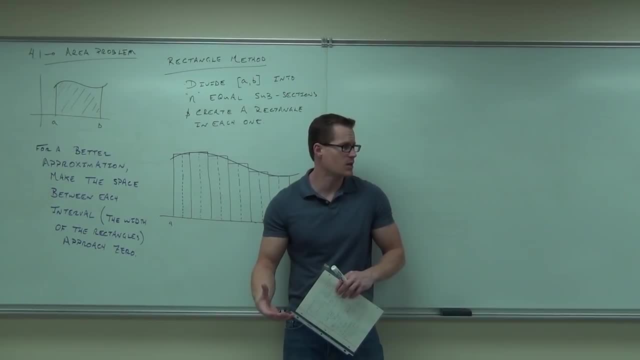 That's the limiting factor. Same kind of basic concept of a derivative right. We'll take the distance and make it 0.. And we're taking the distance and making it 0.. Very similar idea, only now we're talking about an area instead of a slope. 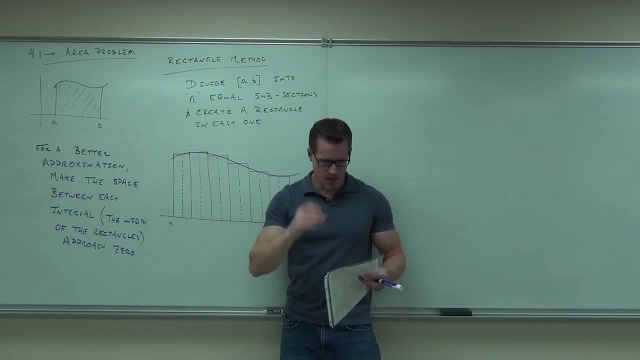 How many people understood the idea of this. Good, That's fantastic. More on this in section 4.3 and 4.4.. This is all you get for right now. just a little taste. This is an appetizer. Are you satisfied? 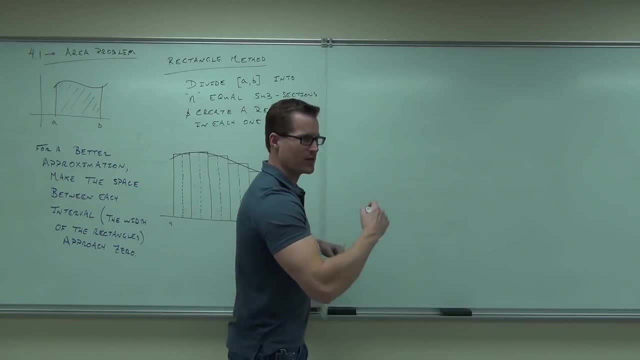 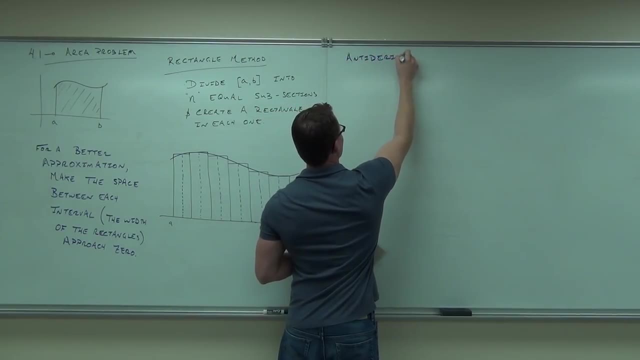 No, of course you're not. That's why you need more of a meal. This is the meal, OK, Different method, Anti-derivative method. You practice that one every day. No, I just made it up on the head. 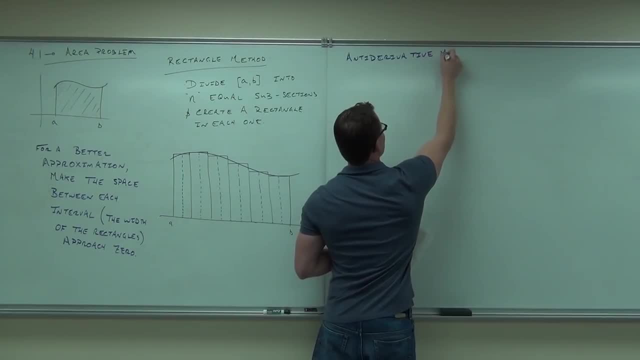 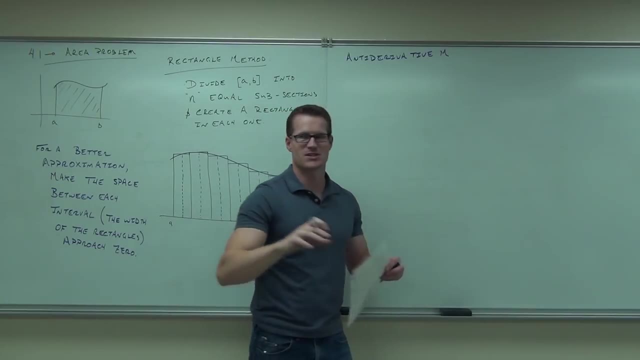 Pretty good. huh, Nice Improv, I suppose. if that's the appetizer, this is like the salad in the main course and we tie it all together as a dessert. And then the chapter 5 is icing on the cake, baby. 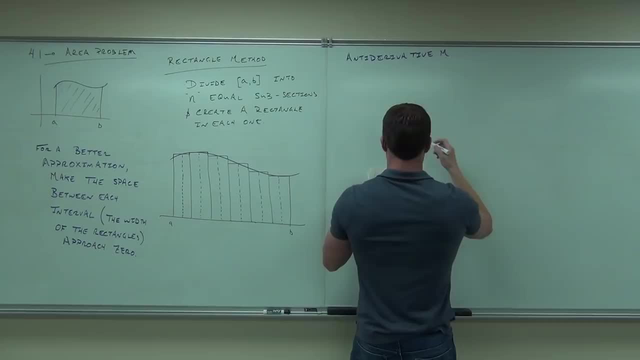 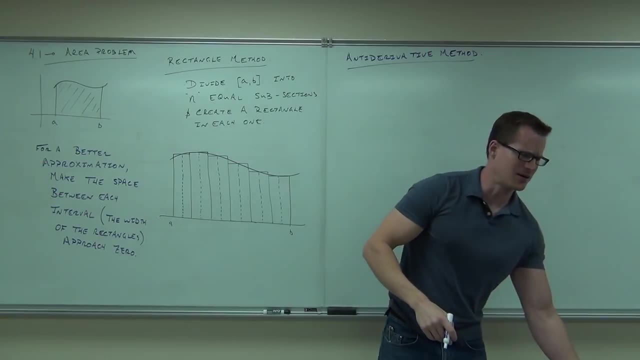 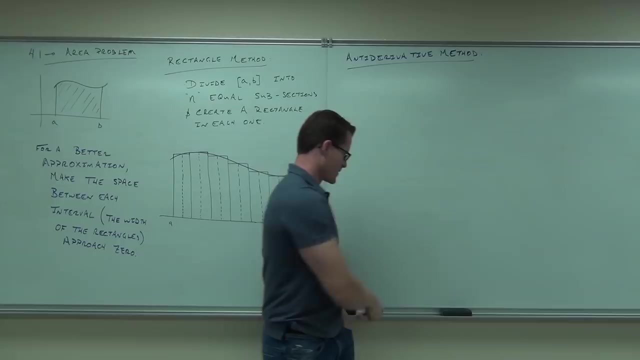 Just how to use it. If you like cake, Insert your favorite dessert here. You don't put icing on a creme brulee. Burn it. You do, You do, You burn it, Anyway. Anti-derivative method. 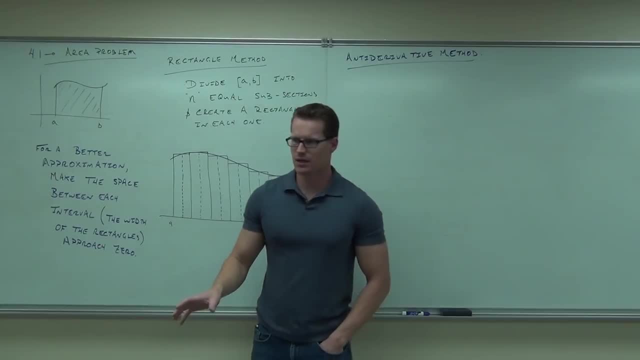 This. I'm going to go a little bit past where the book takes you. The book has you do just what anti-derivatives, how to do anti-derivatives. What I'm going to do is tell you what an anti-derivative stands for and then how to do them. 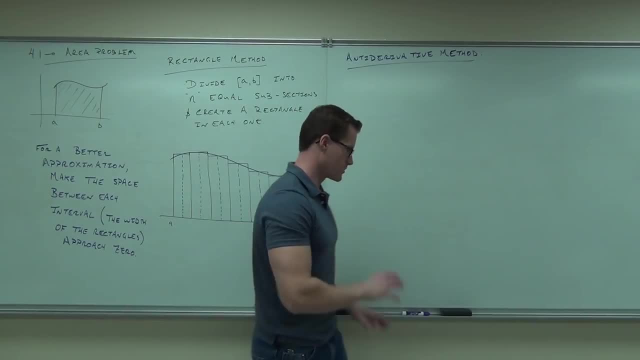 You're going to find out now. I'm going to prove this to you after we do 4.3 and 4.4. So I'm going a little bit beyond That. if A of X, here's kind of the special deal. 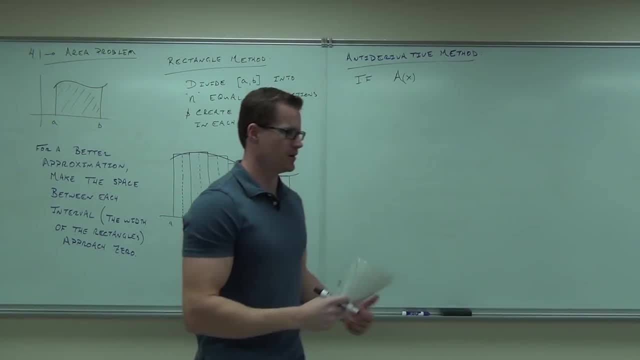 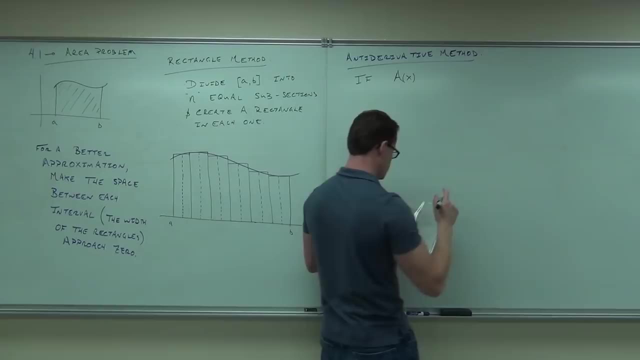 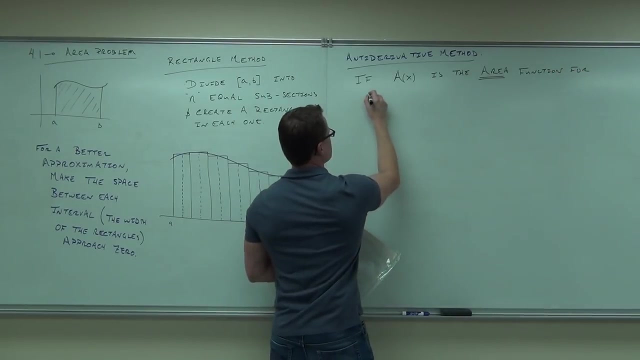 This is what you find out. the end game of section 4.4 is this: basically, If A of X stands for the area under a curve For some function, If A of X is the area function for some F of X, some curve, like this: 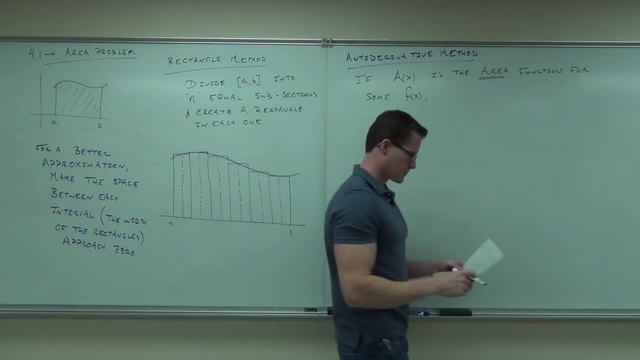 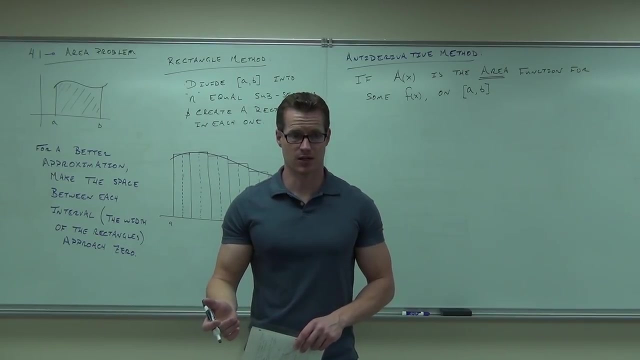 Like this For F of X On some interval. I've got to give you an interval, otherwise you can't find an area. Does that make sense? You have to have an interval. You have to have a definite thing. We'll talk about definite intervals later on. 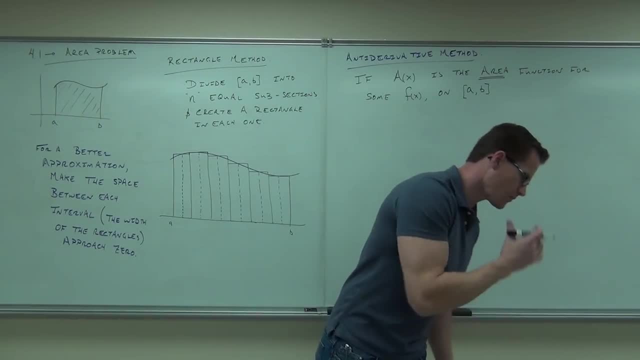 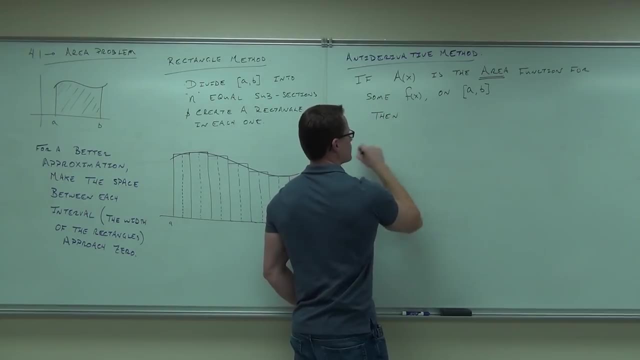 But areas are definite. You have to have points and numbers. Then here's what I'm going to tell you. This is kind of a very cool thing. This is where we're going to end up. Again, I've said it five times now. 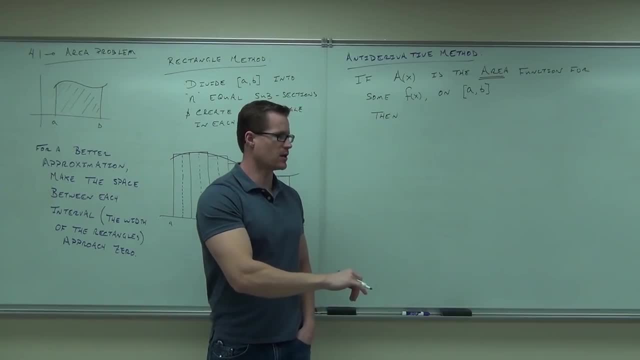 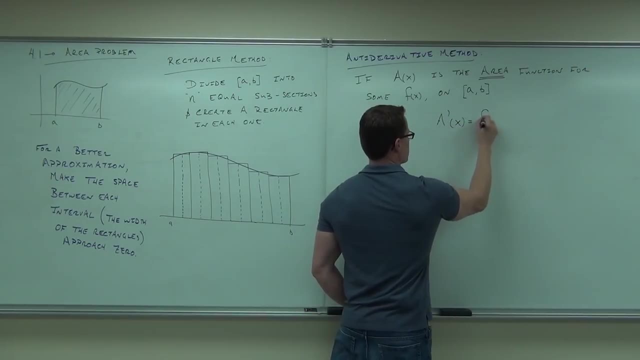 This is where we're going to end up, after section 4.3 and 4.4.. You get it. We're going to end up with this statement, Which is a fantastically marvelous statement. It's magical right now Because you don't know the concept behind it. 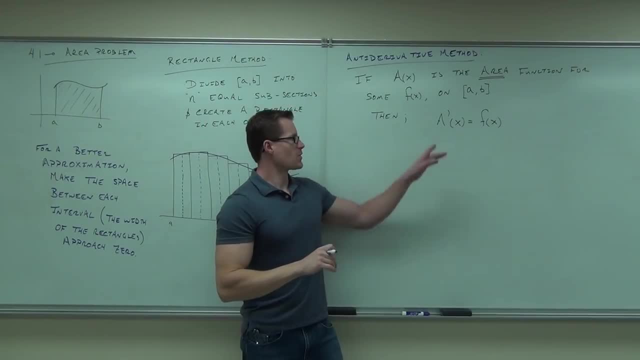 But it's magical. What it says is this thing right, here is an area, This thing is an area, right? It says: if you take This is kind of crazy to think about, But if you take the derivative, That stands for derivative right. 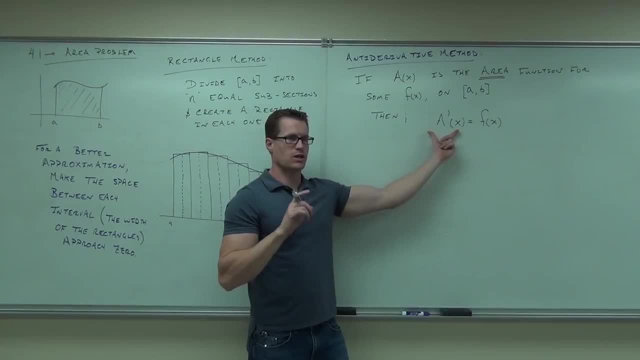 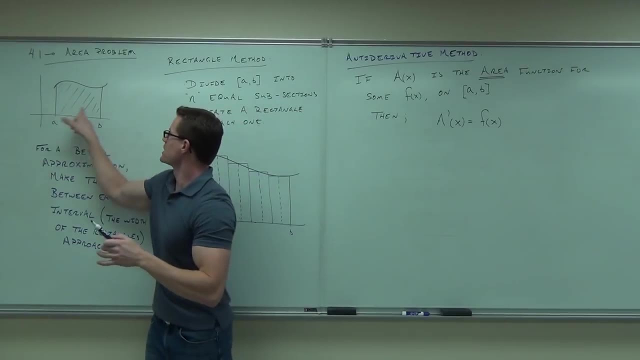 You take the derivative of your area function, It will give you your original function. It will give you the line, The curve. So basically it says this: If your area function represents the area, Take a derivative and you get the function back. 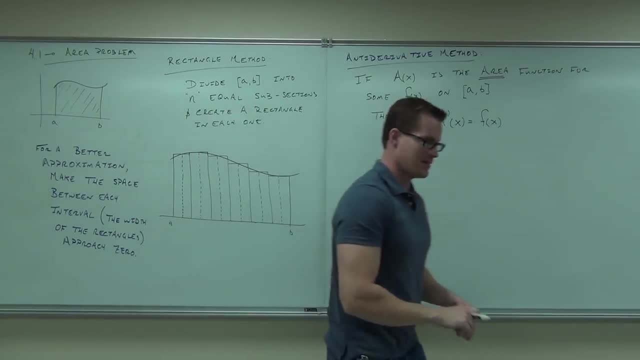 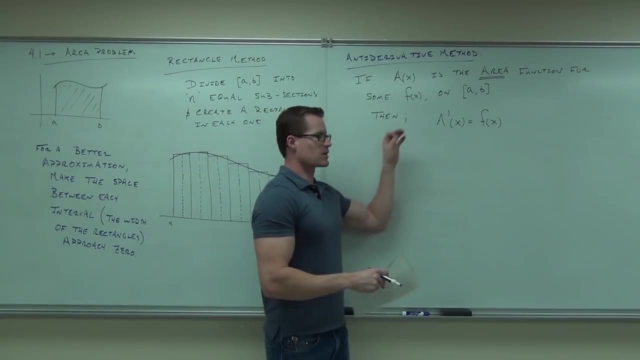 Does that make sense to you? It shouldn't really Not that much. I'm going to prove this to you later. I'm not proving it yet. What you need to know right now is that if you are given an area function, Take a derivative of that thing. 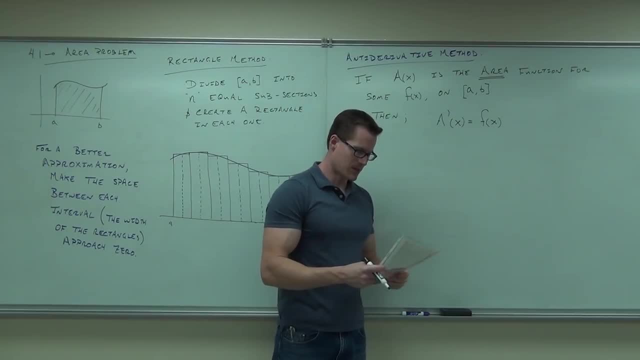 And it will give you your function back. Well now, that's cool, But we're never going to start with this. We're always going to start with our line right? That's where we want to get to. So well, this implies this thing: 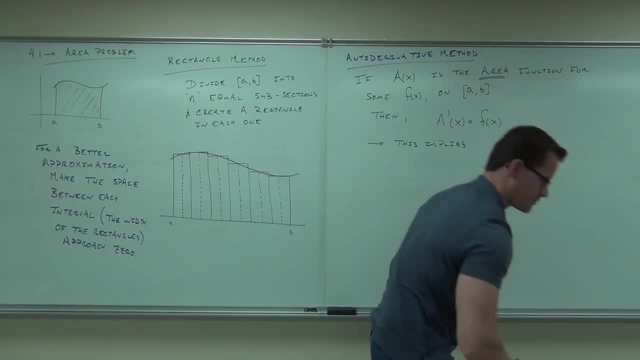 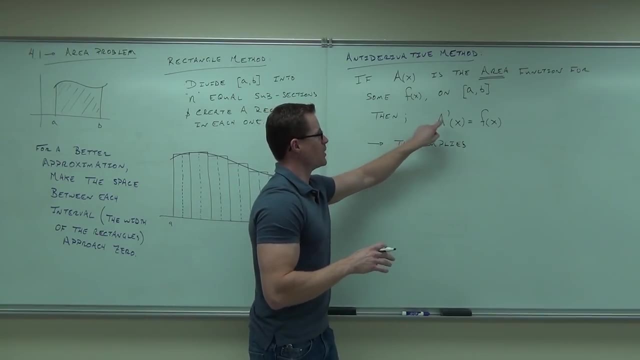 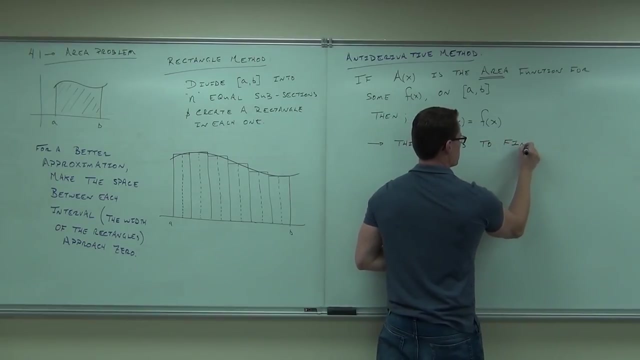 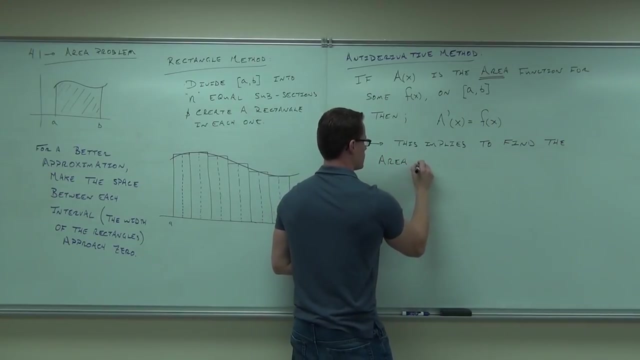 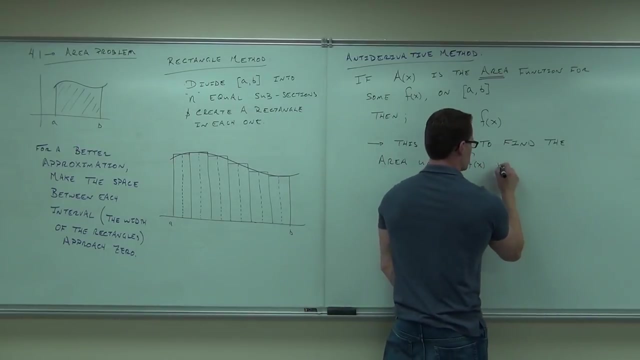 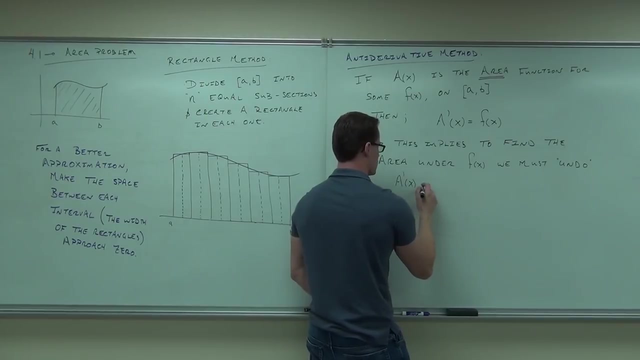 This says: if we want to find the area under a certain function, We basically need to be able to undo this. We need to undo a derivative For some interval. Let me go through this one time for you, So you kind of get the interplay here. 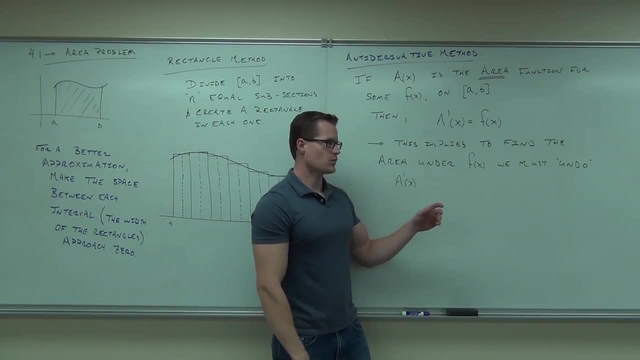 Here's what it says. It says the area of a curve is a of x. What I know for sure is if I take the first derivative of the area, That's equivalent to my curve itself. So if I want to find that area under my curve, 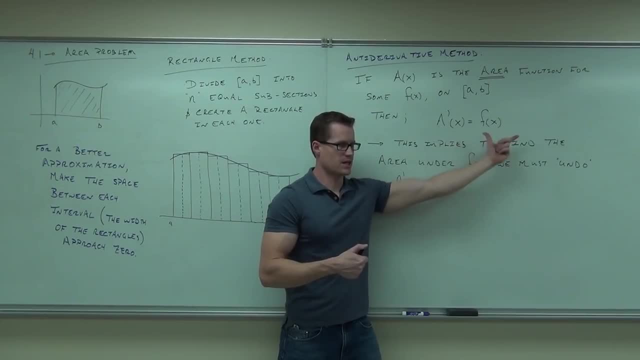 This thing is true, right? The first derivative of the area is the function. So if I want to find the area of the curve Under the curve, What I'm going to do is undo the derivative That gives me the area. So, basically, here's the idea. 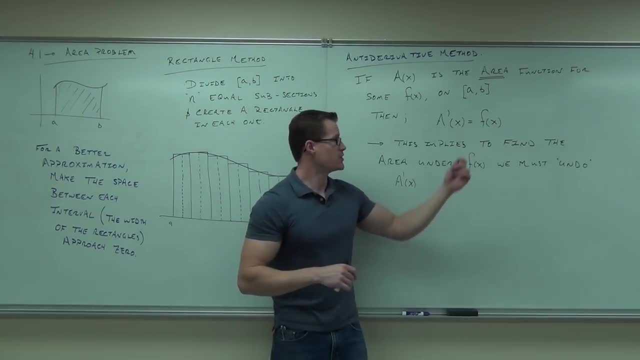 You pretend. You pretend that your function is a derivative. If you undo that thing and treat it like a derivative, You're going to find what's called the antiderivative. That is the area under the curve. That's the idea of the antiderivative method. 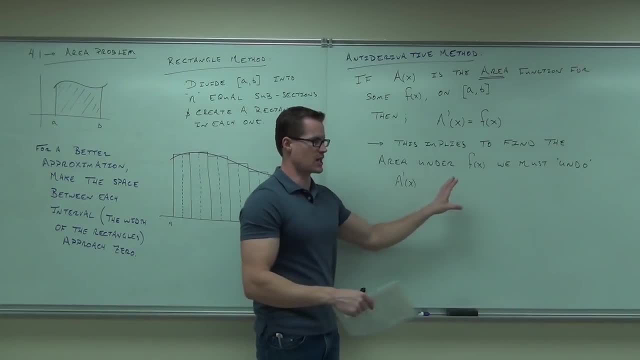 I'm going to get more into it in a second. I'll prove it to you. Well, I'll prove it with an example. I have to prove it to you with 4.3 and 4.4. later on I'll prove it with a couple of examples. 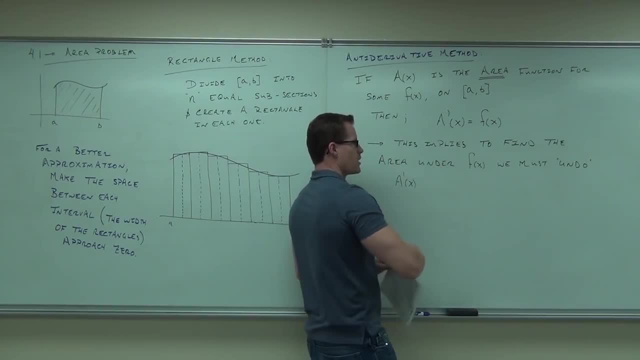 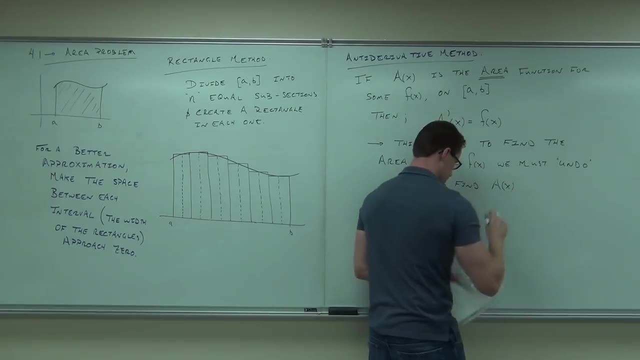 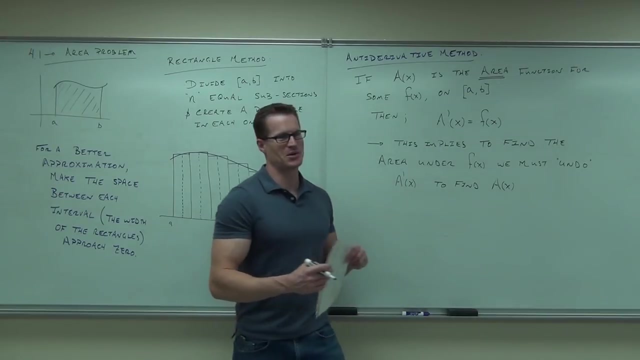 So if we're going to find the area under the curve, Under f of x, We must undo a prime of x to find a of x, The area. Would you like an example that you can actually kind of see? I was hoping you'd say that. 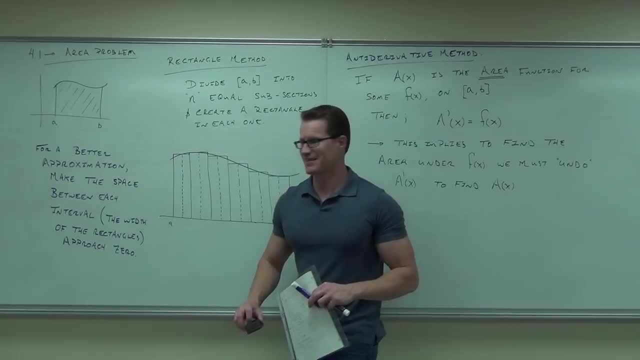 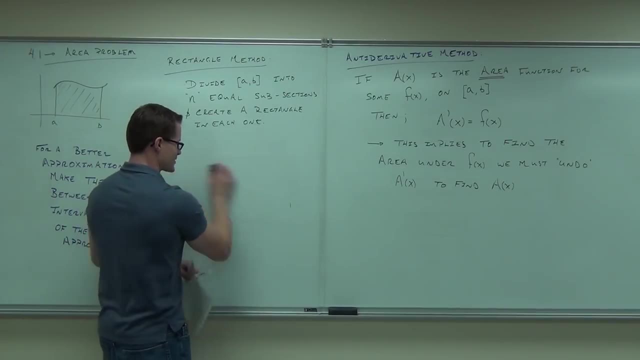 Have I lost you yet? No, Halfway You get this right. Yes, Oh good. Now this is not what we're talking about today, So it's good for 4.3.. Do you get this? No, you don't yet. 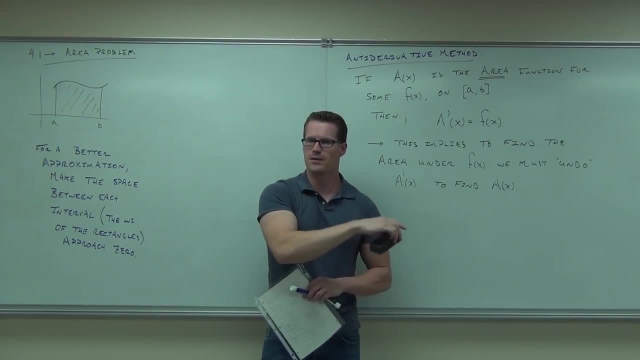 Trust me, You don't. You won't get it fully until 4.3 or 4.4.. The idea is: can you find an antiderivative? I'm going to teach you that in a second. I'm going to explain the concept behind it as well. 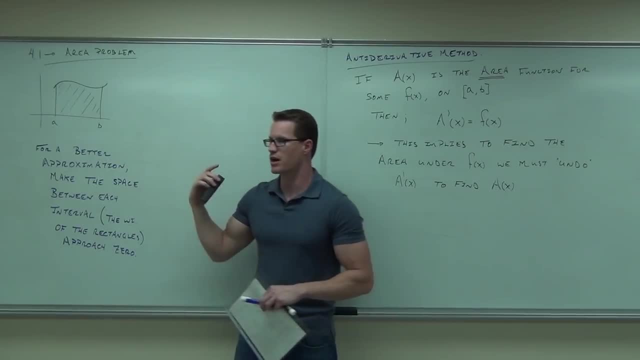 The concept is: we're trying to find the area under a curve. That's why I gave you this introduction. That's the idea. So I'm trying to get that in your head. Remember how I always kept saying what's a derivative? 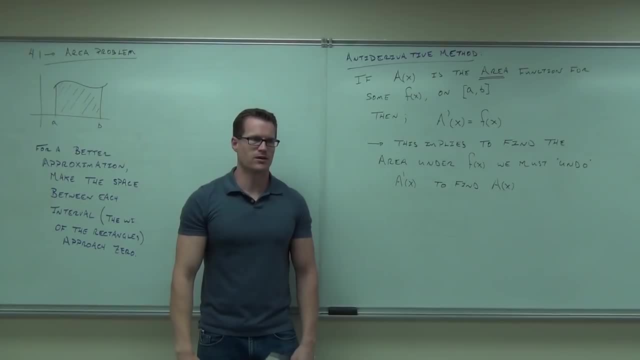 What's a derivative? And you're like, oh my gosh, So here's one. You know that, right, Good, Because I pounded it in your head. And that's when we do the same thing here. What we're doing is we're finding the area under a curve. 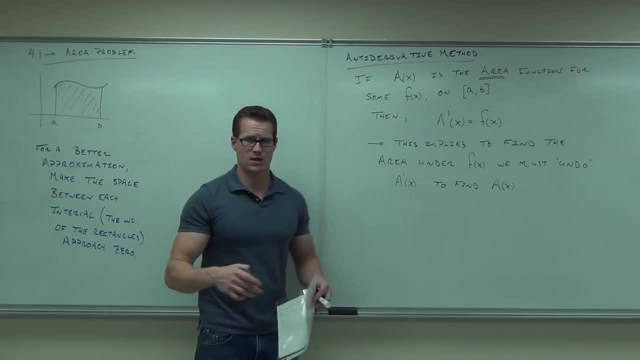 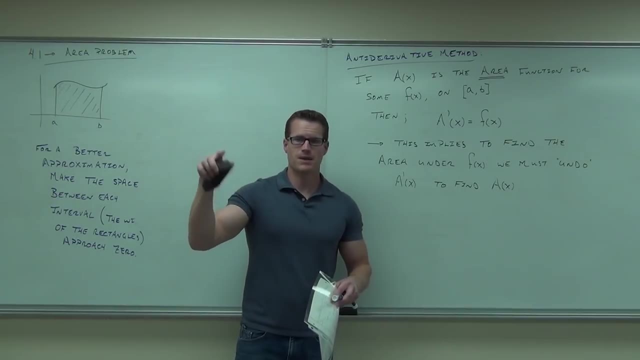 That's what an antiderivative is. What I've told you- and I've done it without proof, I'm not going to prove it until later- I've told you this. I've said: the first derivative of your area is your function. 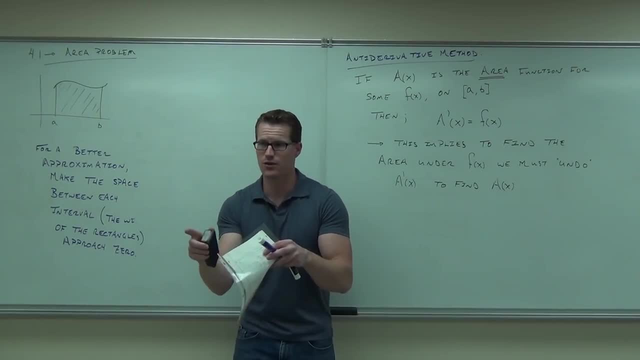 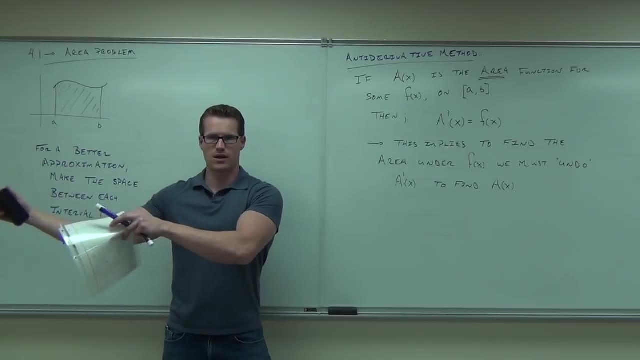 So if I can undo my function by treating it as a derivative, I will find the area function. So basically, we need to go backwards from a derivative. Did you get that? If the function is the first derivative of the area, that's what that says. 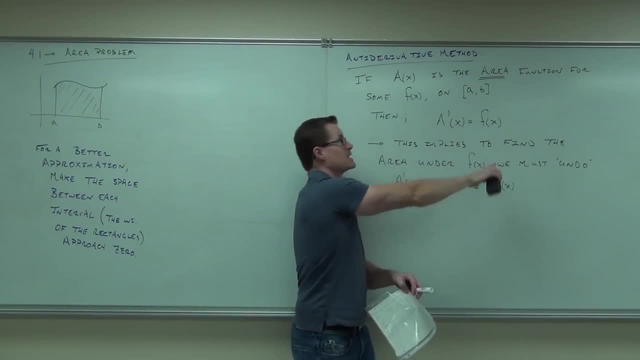 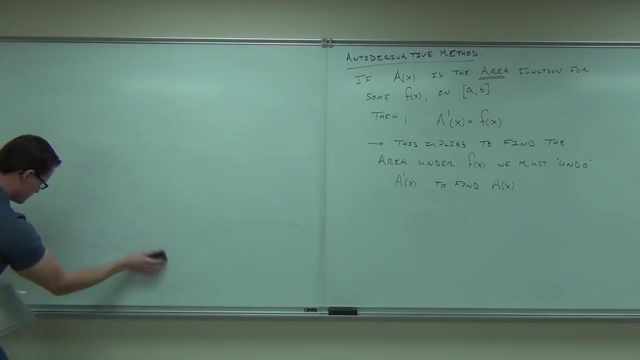 The function is the first derivative of the area. If I can undo the derivative, I get my area. That's the idea. That's the antiderivative method in a nutshell. Very quick statement. Now let me do some of this with geometry. 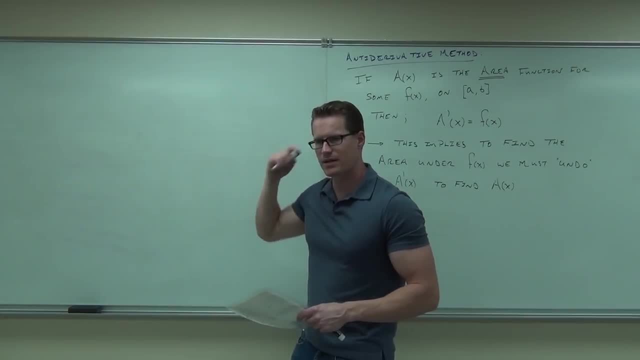 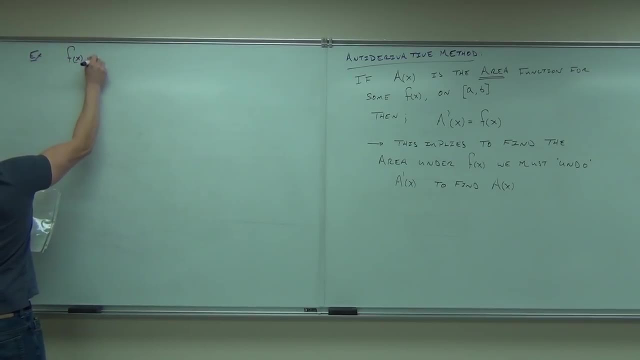 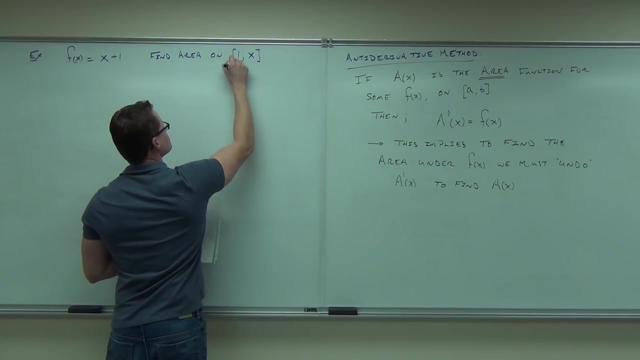 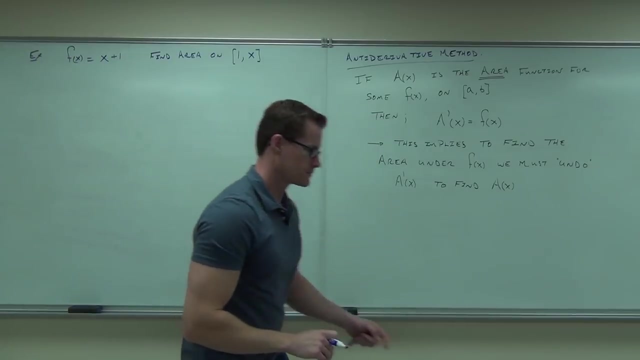 to show you that it does in fact work. Then we'll get on into some antiderivatives and how to do those things. So example: If we have a function f of x equals x plus 1, I want to give you something easy to graph. 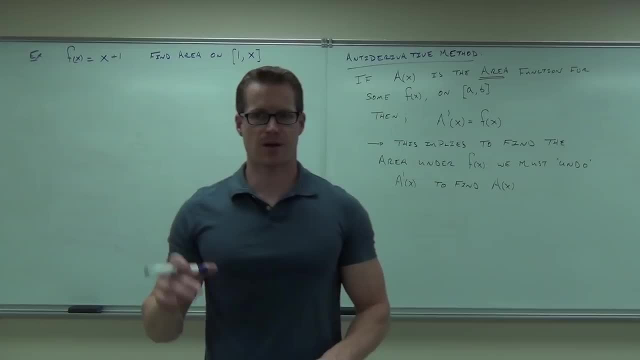 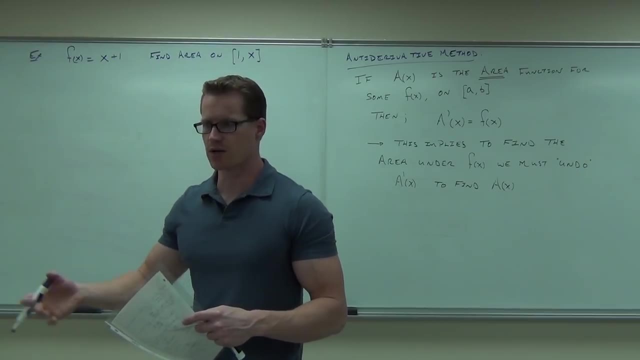 because I'm going to show you the graph in a second. I want us to find the formula for the area on 1 to x. Now, this would kind of be stupid if I gave you just 1 to 3, because we could just use the triangle and find the area. 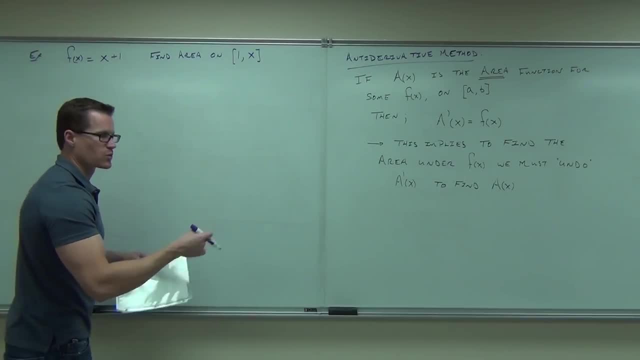 But what I want to find is 1 to x, And I'll show you why this works according to this. I want you to do that First off. can you graph this? Geez, I hope so. What's your y-intercept? 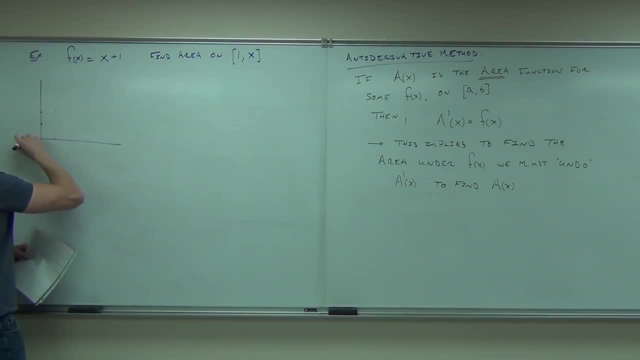 How much is your slope? Would you agree that that is your function? We're trying to find the area of that between. what did I say? negative 1? Oh, you know what I want? negative 1.. Let's make that negative much more interesting. 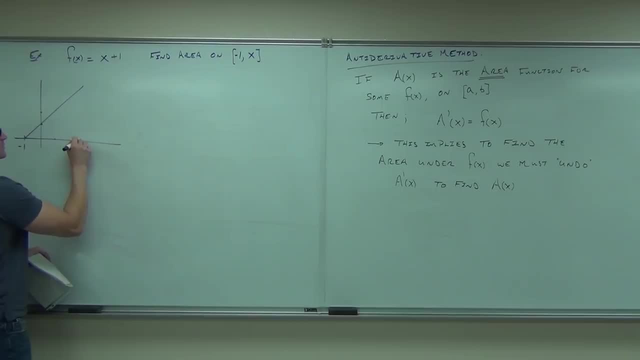 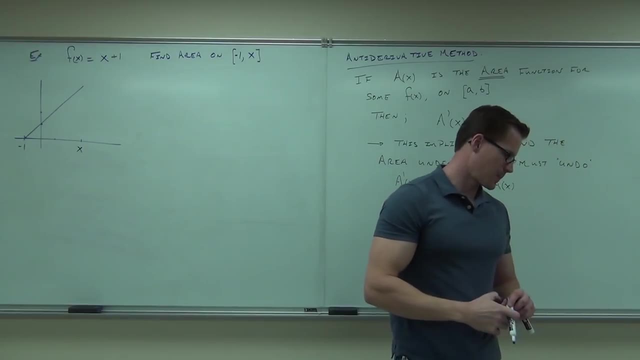 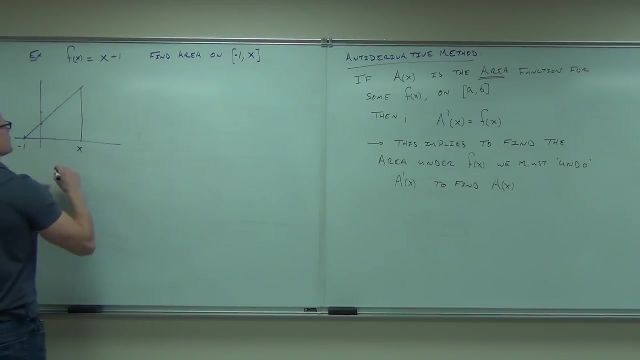 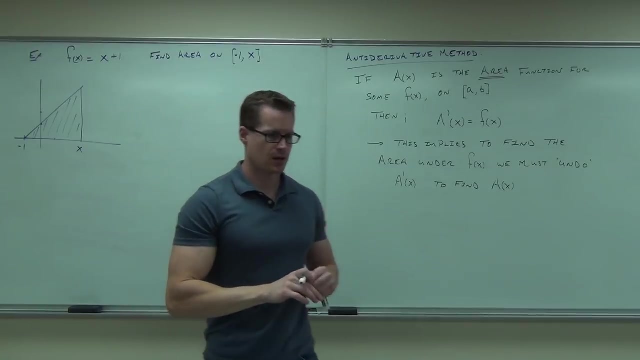 Negative 1.. Negative 1 to x. Now I don't know where x is. I made it positive, but it doesn't have to be positive. What we're talking about, wherever this x is, is the area of that shaded region. 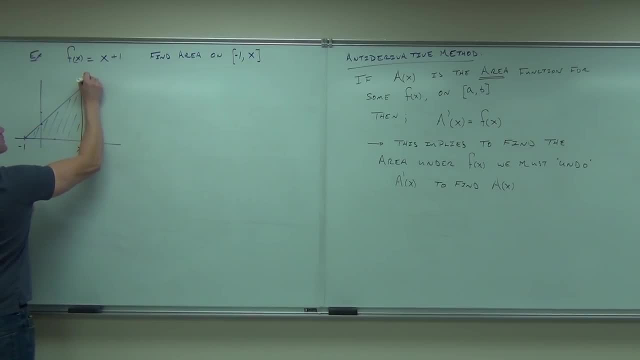 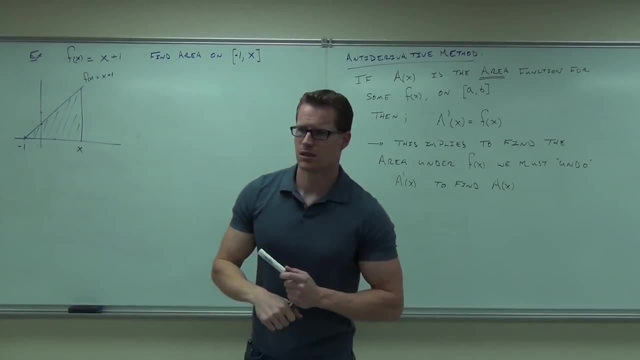 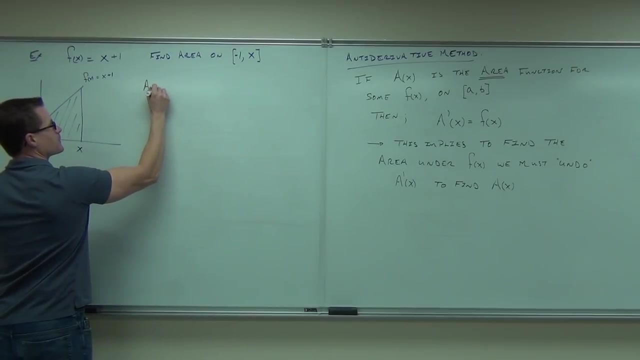 Now keep in mind that this function is x plus 1.. What shape is that Triangle? Can you find the area of a triangle? Yes, Of course you can. yes, Let's find the area of a triangle: The area in terms of x. 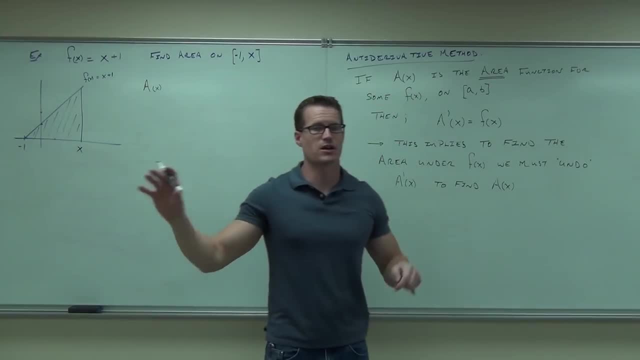 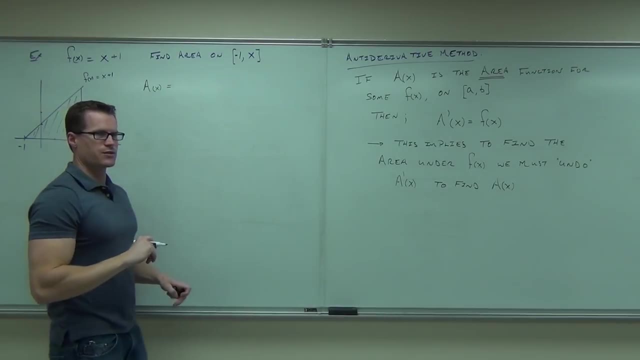 notice I'm using the same terminology I used over here. right, That's an area function. The area in terms of x, wherever x happens to be, is: How do you find the area of a triangle? again, 1 half, Very good. 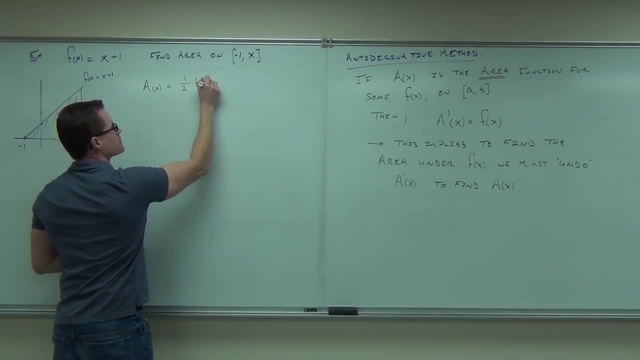 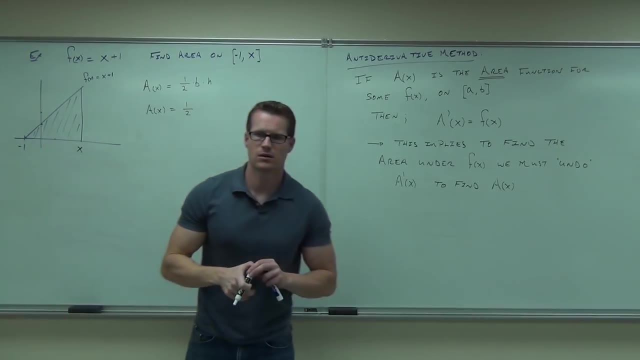 1 half base times height. I'm going to write 1 half base height, so that would be 1 half. Oh my gosh, what's the base? Let's think about that. What's the base? Is the base x? 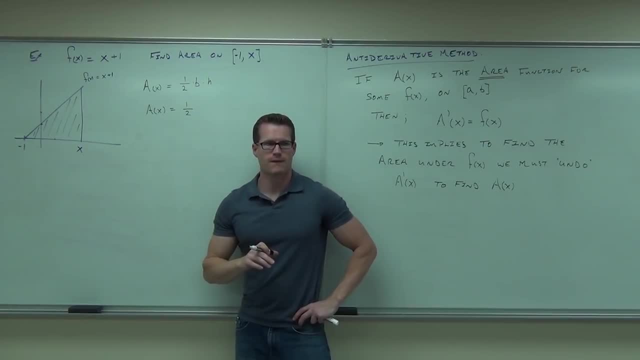 x minus 1.. x minus 1.. Oh, close, Negative: 1 minus 1 plus x. How do you find the distance between two points, between two numbers? You subtract them. You subtract the numbers, right? You subtract them. 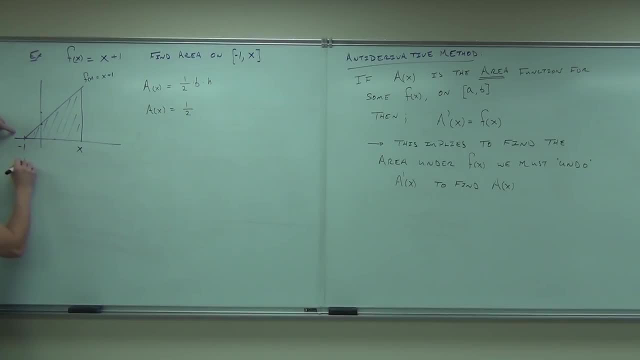 So this would be the distance between here and here is x minus not 1,, not 1.. This would be the distance between here and here would be x minus 1, right, There's going to be a difference here. 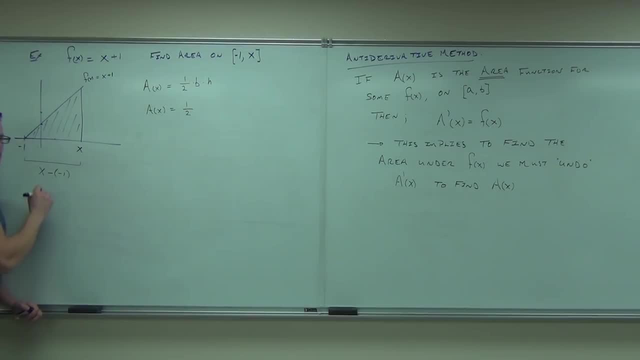 So it'd be x minus negative 1.. Yeah, That's x plus 1.. Do you see where we're getting the x plus 1?? Well, I mean, you can see it. you can just see it on the graph, really, just intuitively. 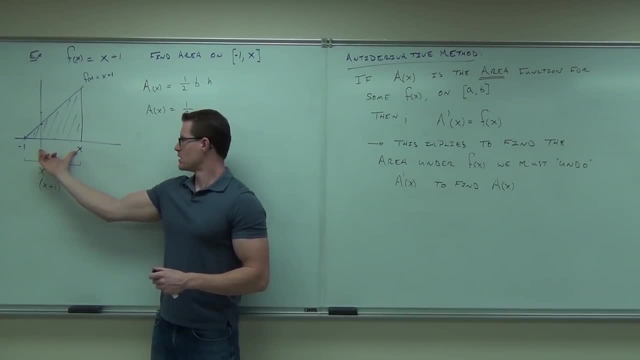 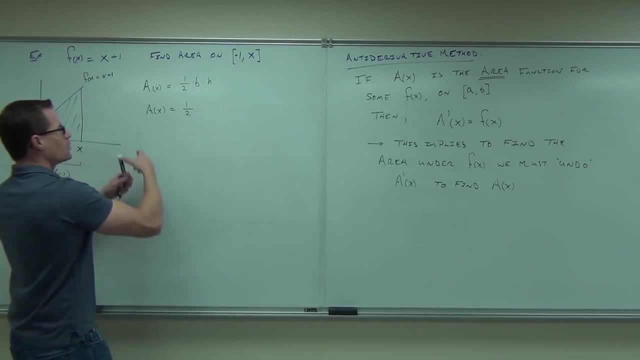 This distance is x, right? Yes, Mm-hmm, That's one more unit. That's x plus 1. Not x minus 1. That would be over here. So we have x plus 1. So one half okay, that's x plus 1.. 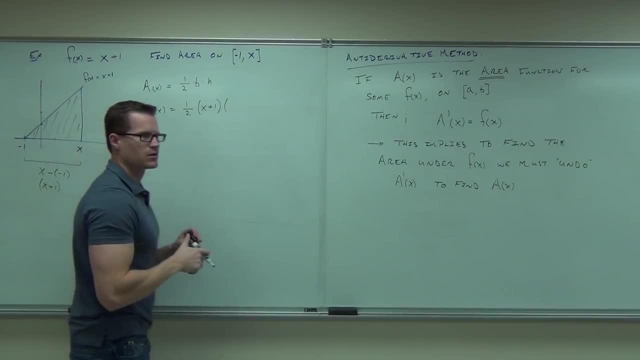 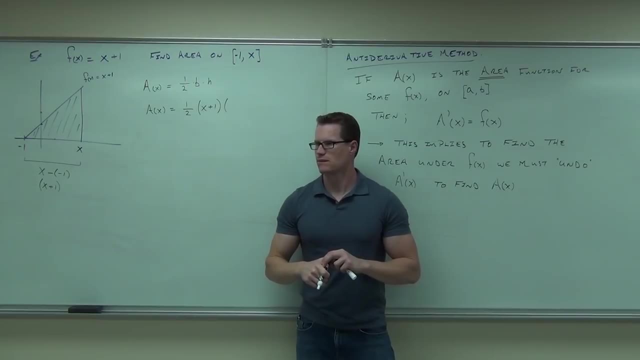 Okay, Oh my gosh, what's the height? What's the height f of x plus 1.. f, okay, f of x plus 1.. Not quite, No h's, We don't want any h's. 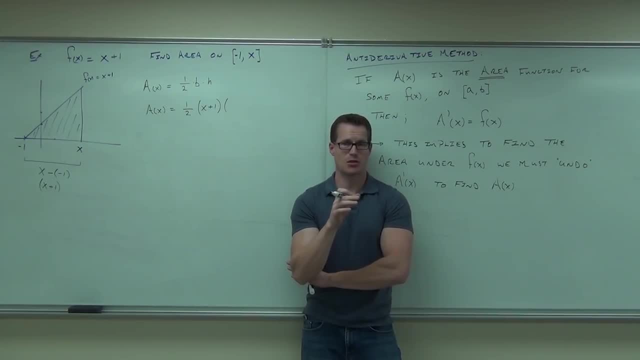 You're thinking. I like the thoughts. Good thinking, You have good thoughts. None of them happen right now, but that's okay. All right, Tell me something, If this was a 3,? if that was a 3,, what would the height be? 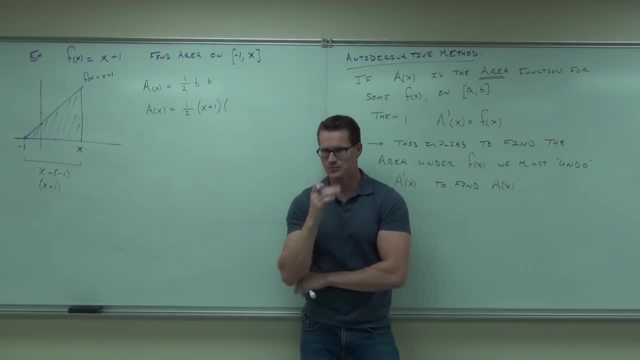 4. Very good, If this was a 7,, what would the height be? 8. 8. You all see the 7,, the 8.. If this is an x, what is the height? 1. 1. 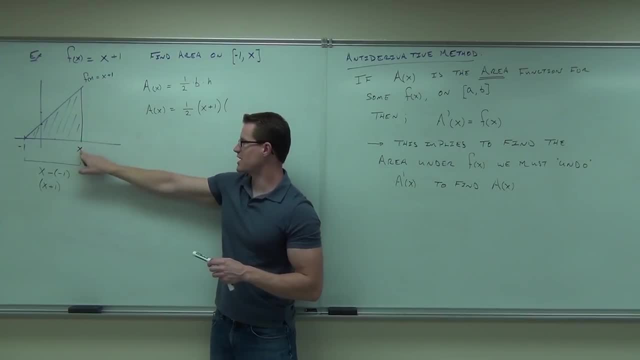 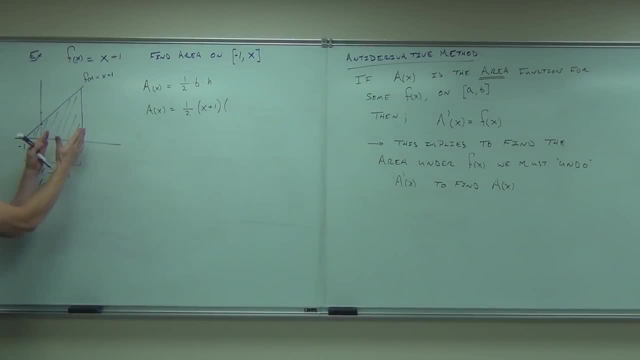 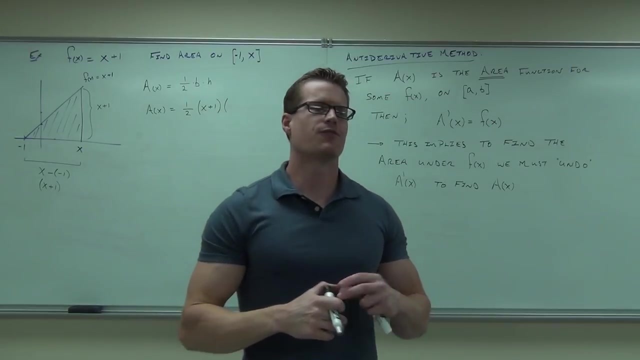 That's what the height is. So this height, whatever this x, is right, it doesn't even matter If it's here. if it's a 1, then it's 1 plus 1 is 2.. So this height, x plus 1, the only thing on the height of x plus 1, the function says: 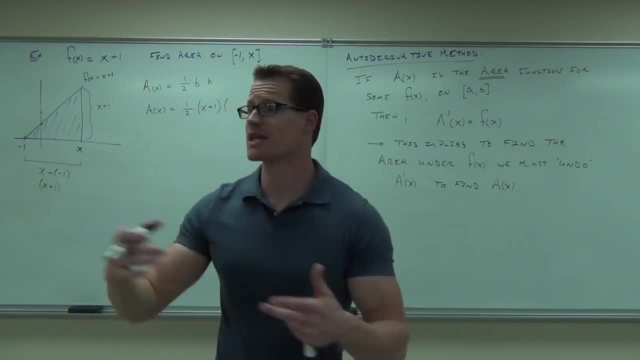 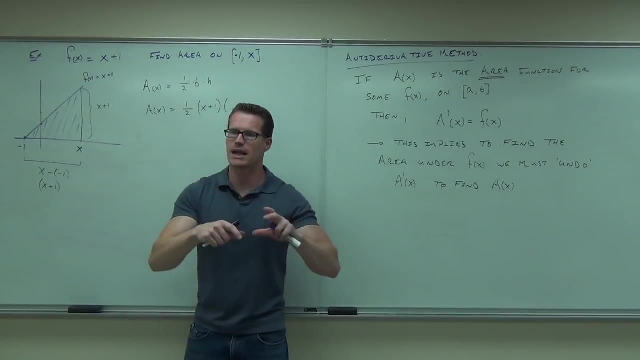 the height. right, That's what the function means. So take the value. The value is x. Plug it into the function. plug in x. I just get x, x plus one. that's what we do. We don't plug it in to get x squared. that's not what we do. 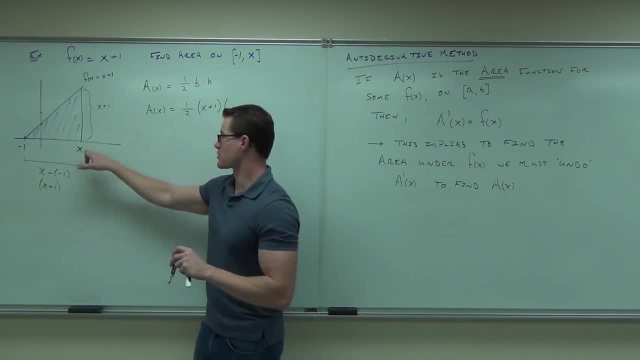 We're not squaring the number and then adding one, we're just plugging the number in. I said: if that's a three, you get three plus one. If that was a seven, you get seven plus one. If that's an x, you get x plus one. 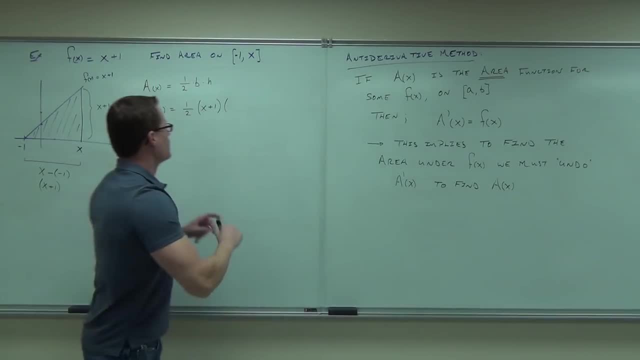 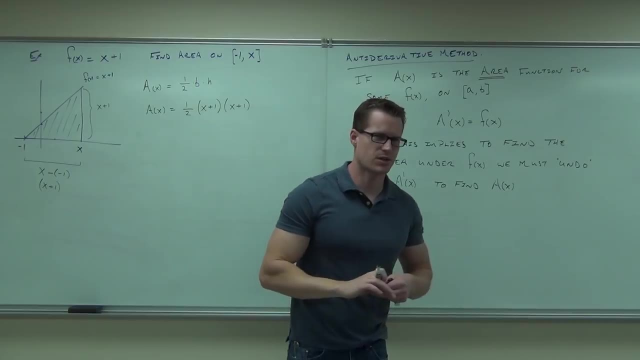 or it is plus one. how many people understand? raise your hand. if you're okay with that, good, Then our height is also x plus one. You okay with this so far? I'm just kind of proving this for you with an example. 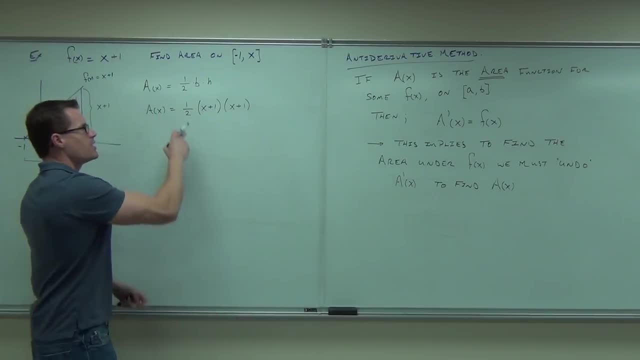 It's not a genuine proof, but I'm showing you that it does work. If I distribute this, I'm gonna get, let's see, one half. that's x squared plus two, x plus one. Do you believe me? You should, because that's right. come on now. 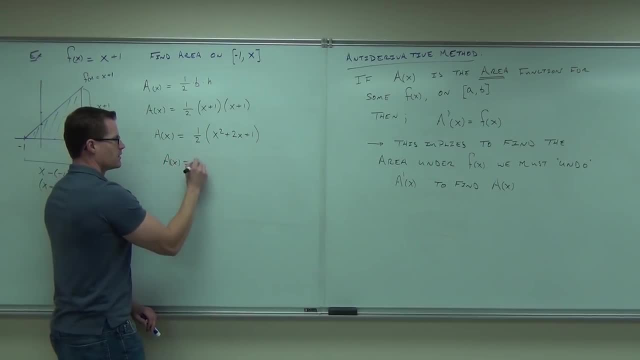 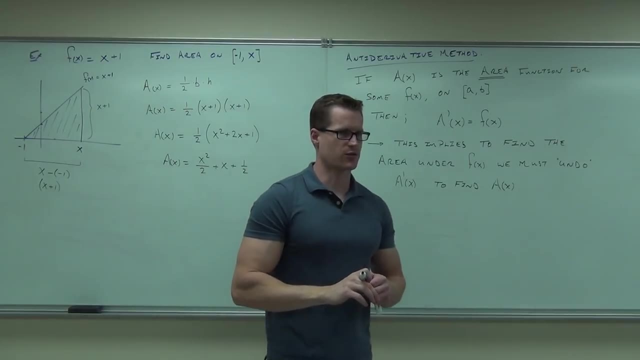 If I distribute the one half even further, I get x squared over two plus x plus one half. You follow me with that so far. Okay, now here's a cool deal. Would you agree that whatever I tell you for x, you could find the area of that triangle? 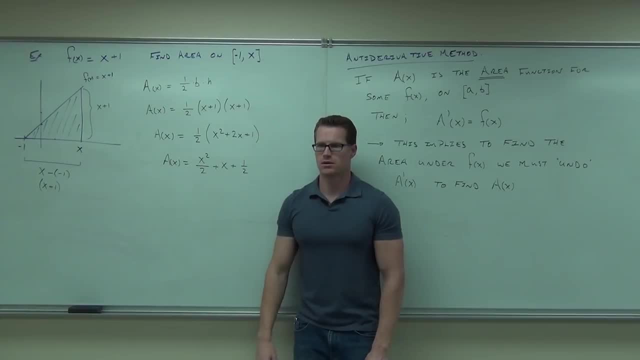 If I said x is nine, could you find the area of the triangle? Yes, you could. You just plug in nine. this is in fact, our area function because we made it up geometrically. It's just the base times the height divided by two. 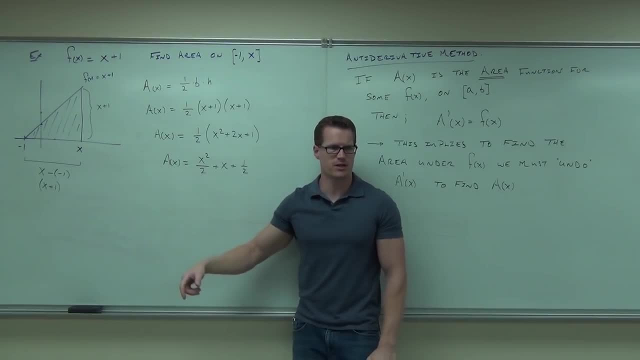 That's all we've done So far, so good. So that's what we're gonna do. We're gonna do the same thing. We're gonna do the same thing. That's what we did. Now, what I want you to do is do some magic. 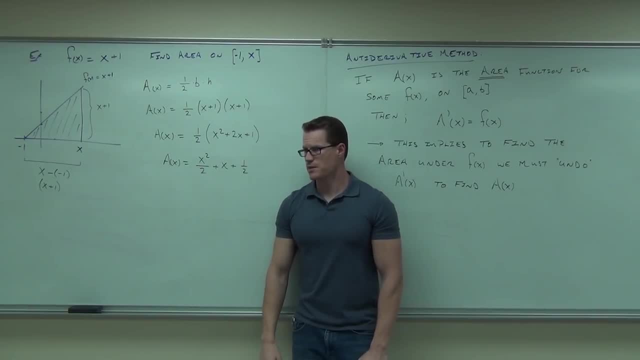 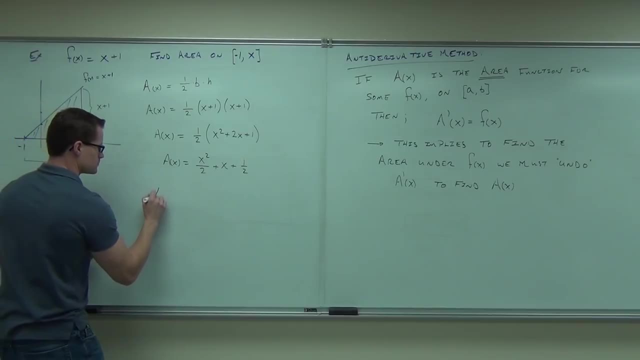 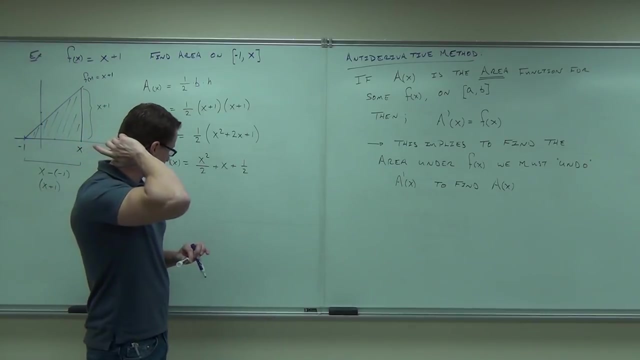 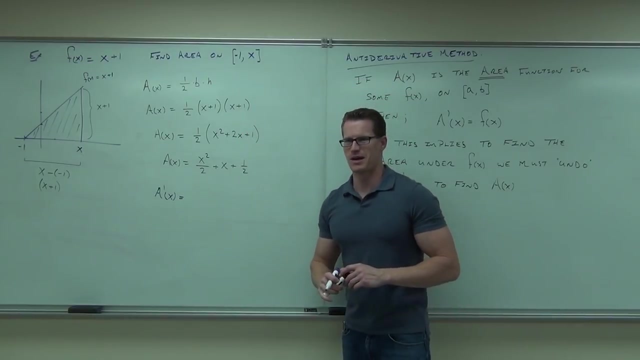 This is the area function. I want you to take a first derivative of that. Would you do that for me? I hope you got magic. I hope so. This is not that great magic. I would've told you it was gonna happen. 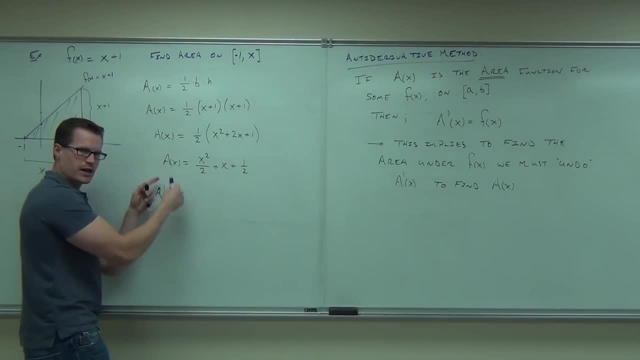 but what's the first derivative of a? And we denote that a prime right. That's the first derivative of a. What's this? x, x. very good, because you bring the two down, the twos, simplify, you get x. 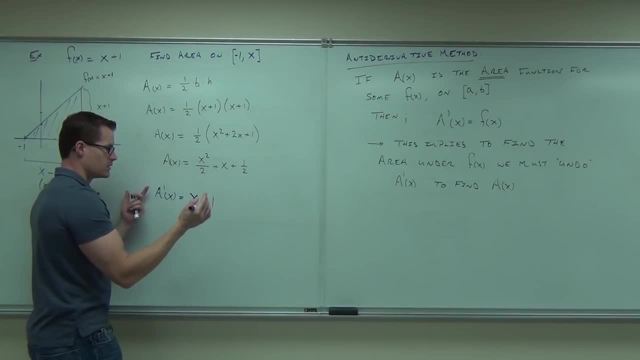 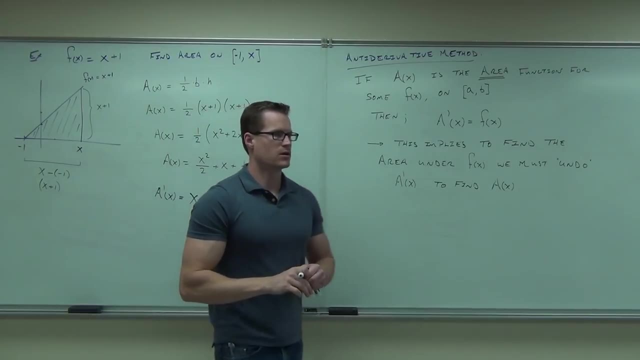 What's this One? What's this Zero? Aha, Does that look familiar? Yeah, in fact, this is your function. That's true every time The derivative of your area is going to give you your function. every time that's going to happen. 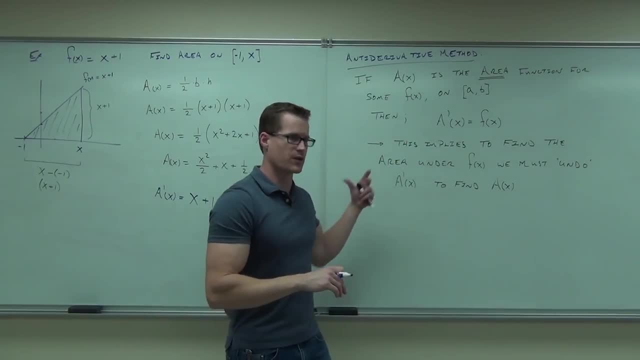 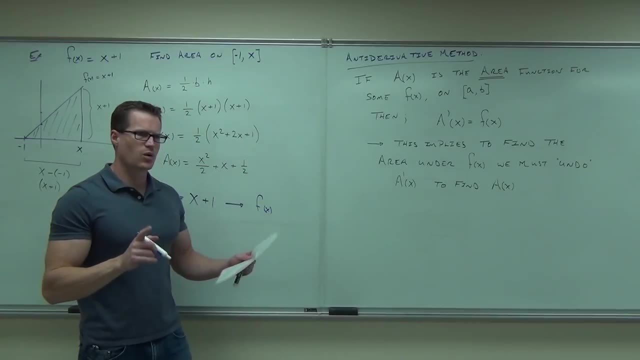 That's just basically one example showing that this is true for this example. Now, it doesn't prove it at length, I will do that later- But it shows you that you can do it. Shall, we do one more. Would you like to see one more? 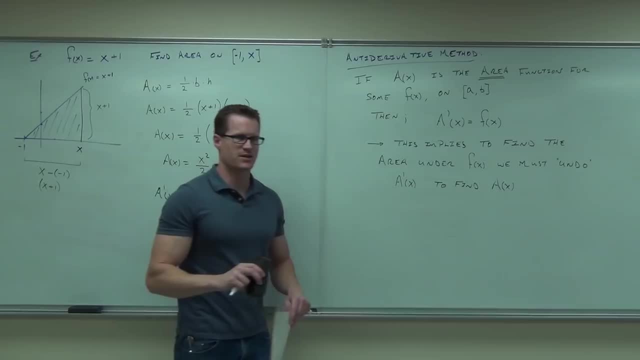 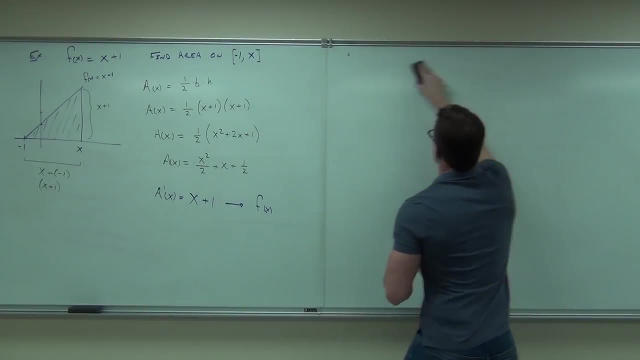 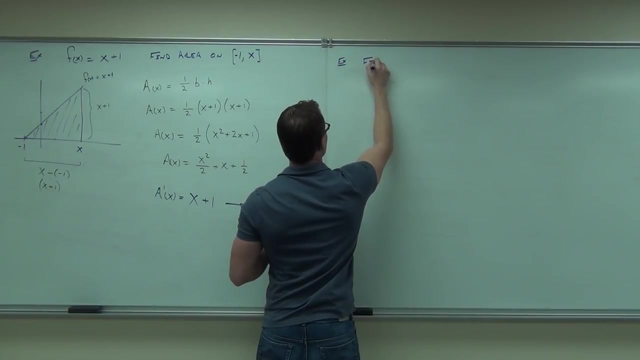 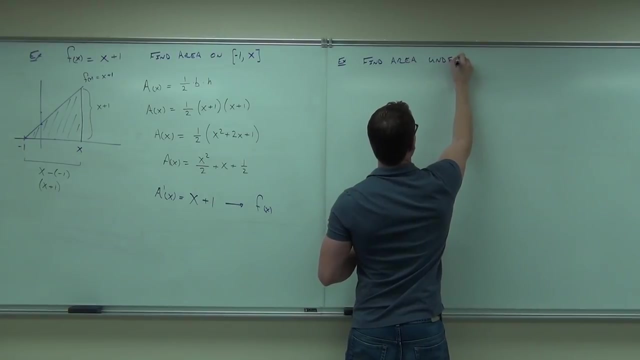 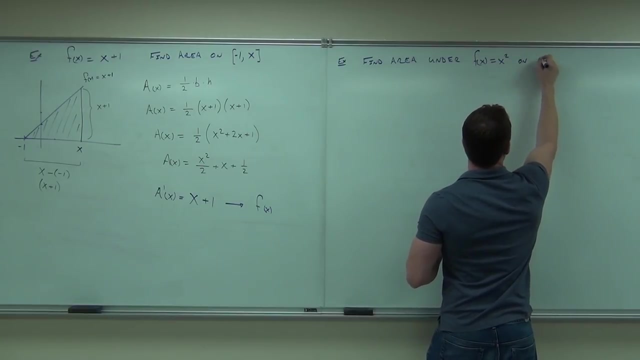 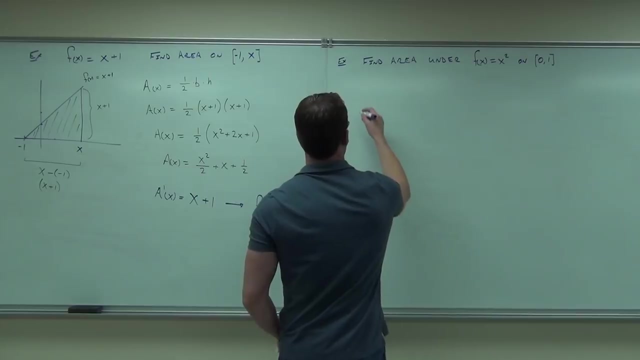 Yeah, I'm gonna kind of start simplifying this a little bit. Okay, You know what x squared looks like, right? Okay now this is only between zero and one, so I'm not gonna draw the left side of this, I'm just gonna draw the right side. 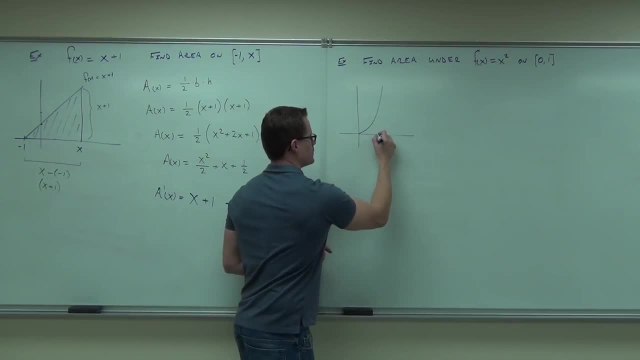 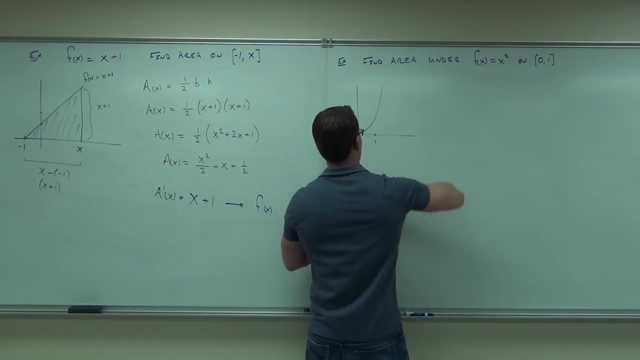 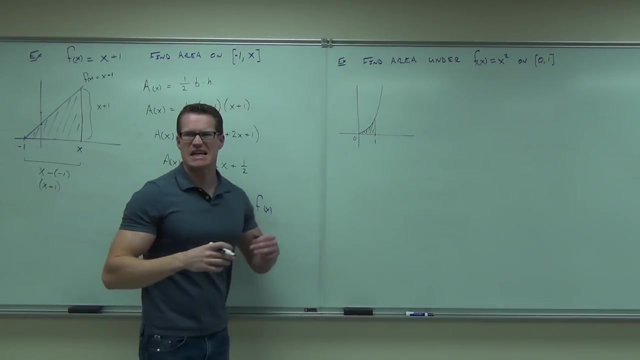 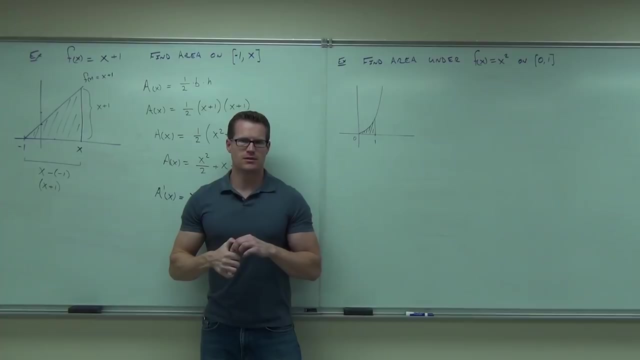 I'm just gonna draw that. Do you all see that? that's the area we're talking about right there? Yeah, I know, Is that a triangle? Is it an exact triangle? No, So we can't do the same thing, but we're gonna use the idea. 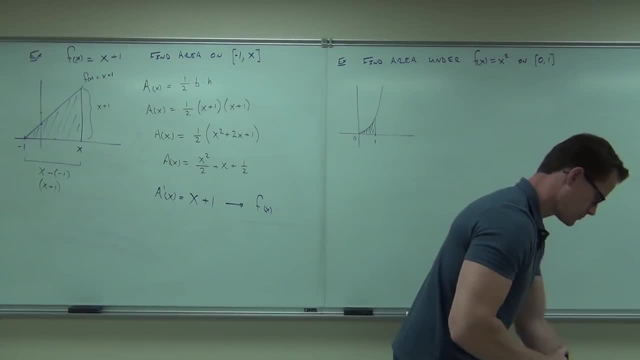 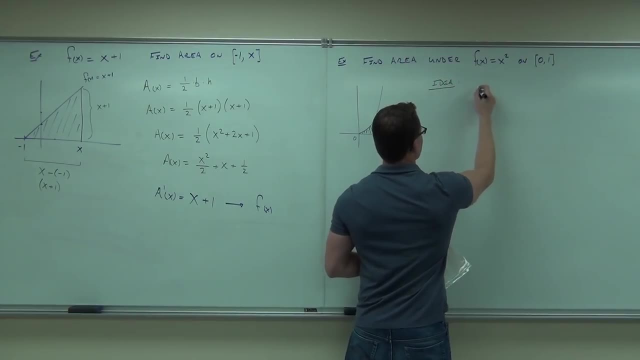 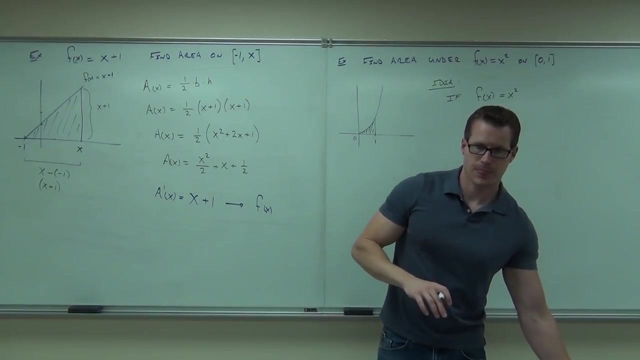 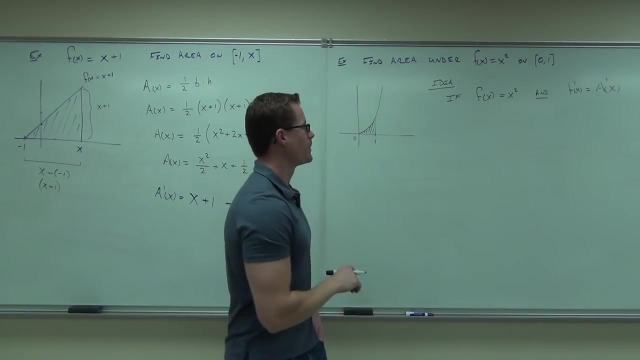 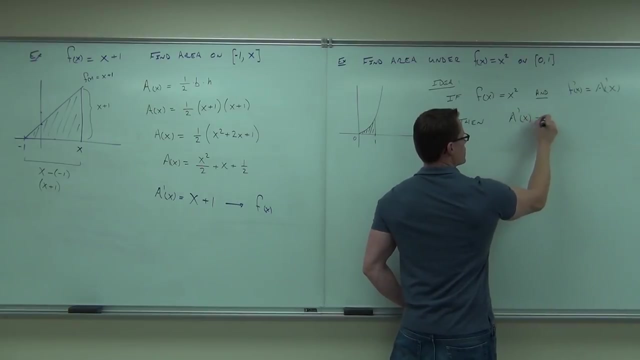 The idea is. Here's the idea: If f of x equals x squared and f of x also equals the first derivative of our area function- you believe that, right, Uh-huh- Then the first derivative of our area function equals x squared. 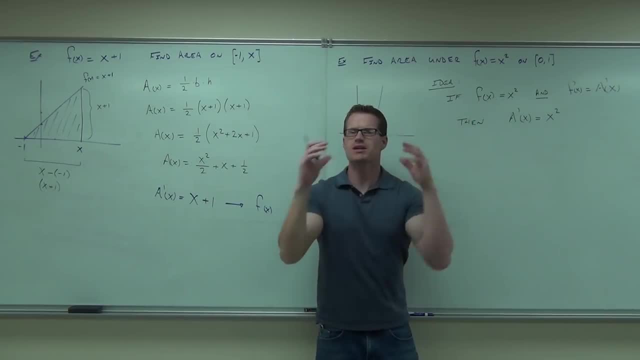 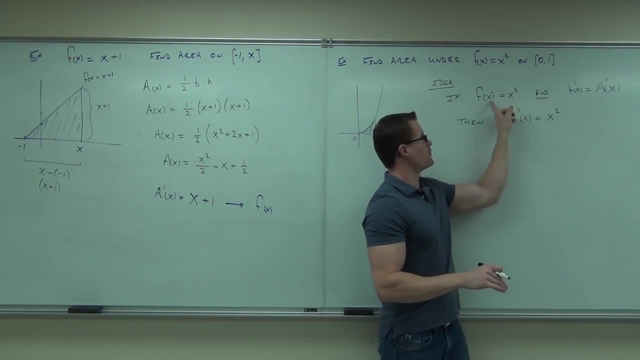 That's a basic substitution. It says: if our function's x squared and we know that a function is equal to the first derivative of its area function, Can you follow me on that? Then we say, alright, well, if f of x is x squared, 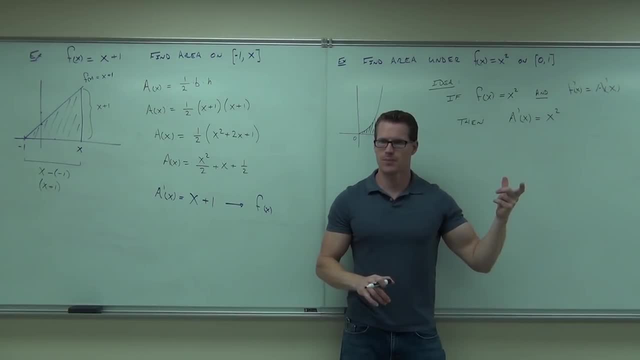 then x squared equals that. That's our jump there. Can you make the jump, Okay? So basically, we're asking this question: Can you find a function whose derivative is x squared? That's the question you ask. Can you find a function? 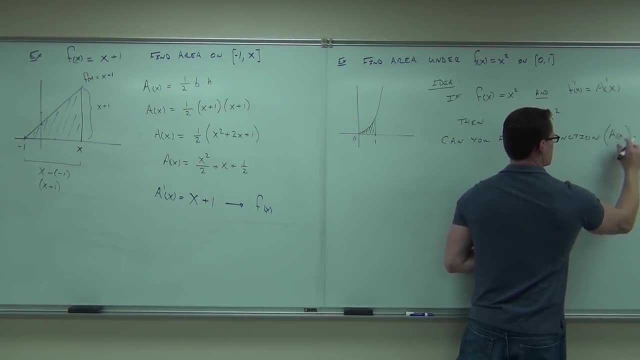 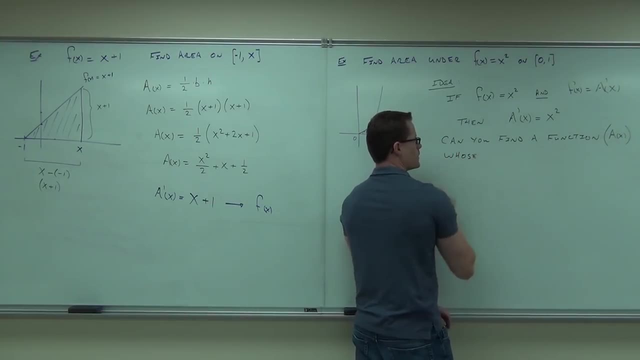 we're gonna call it a of x, because that's gonna be our area. Can you find a function, a of x whose derivative is x squared? Let's try a couple. Let's just have some fun and try a couple. alright, We can take derivatives pretty easily. 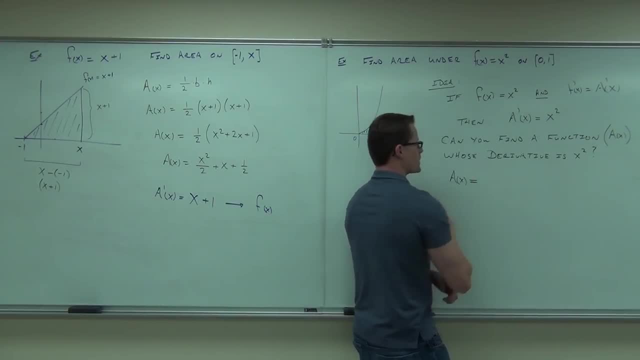 Let's try one. Let's try. well, we'll use some common sense or some critical thinking. I should say. Would you agree that you need a power bigger than two? Probably, because when you take a derivative, that power decreases by one right. 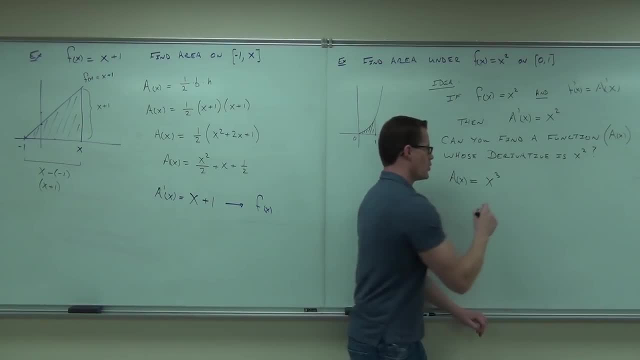 So let's try x cubed. Does it work? No, No, because this is gonna give you a prime of x equals 3x squared Right. That's not gonna work. Divide it by three, Okay. So if I can somehow, 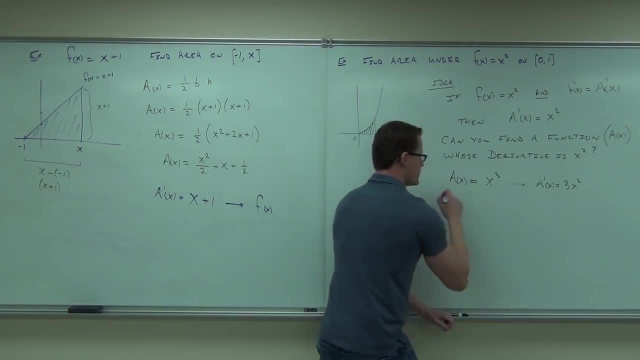 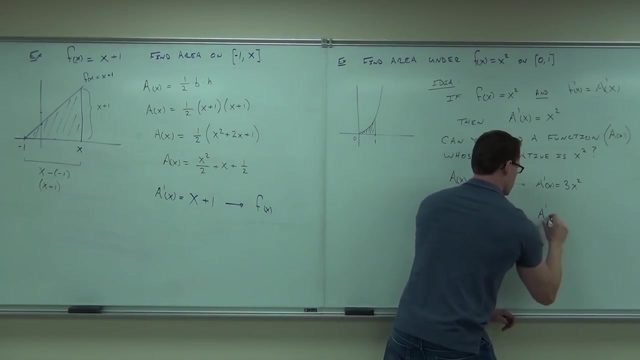 so if I can somehow undo that divide by three, then maybe x cubed over three. Oh, let's try that. Let's try x cubed over three. Would that work? Mm-hmm, Let's try. If I take the derivative of that thing. 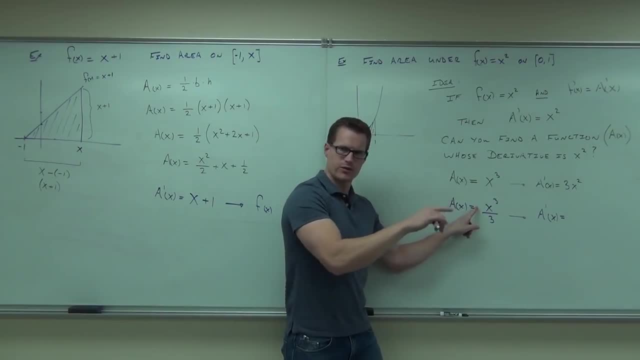 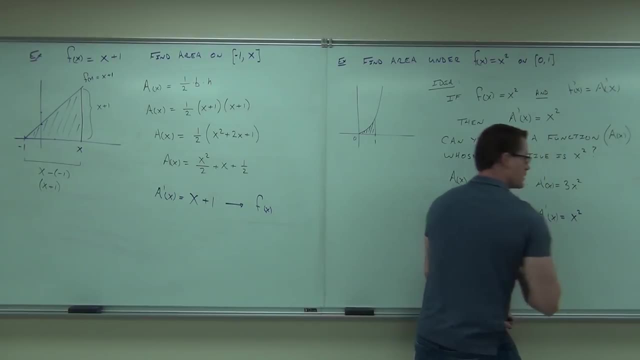 what I would do is I'd bring down the three. right, The three and the over three are gonna be gone. I'm gonna get x squared. Okay, Does that work? Yeah, This one not so much. No, This one, yes, worked. 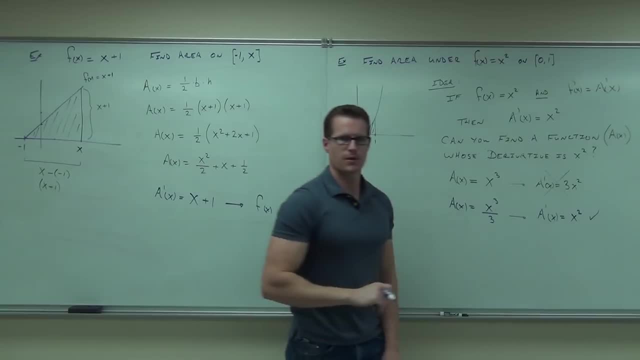 How many of you feel okay with that so far? So you're undoing the derivative, You're going backwards. So is it related to the derivative? Absolutely. But you're going the other way And we had something unique right? We had to have this over three somehow. 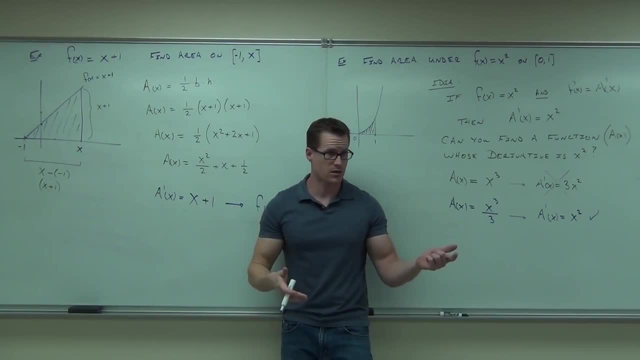 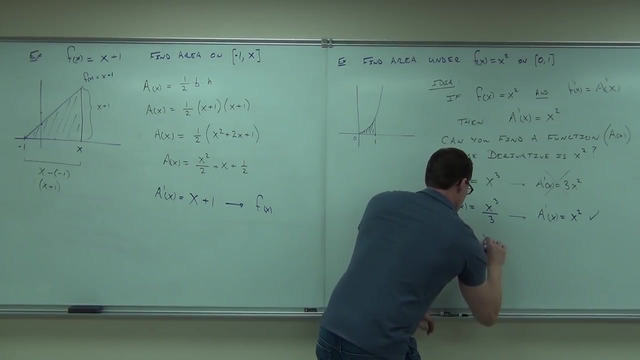 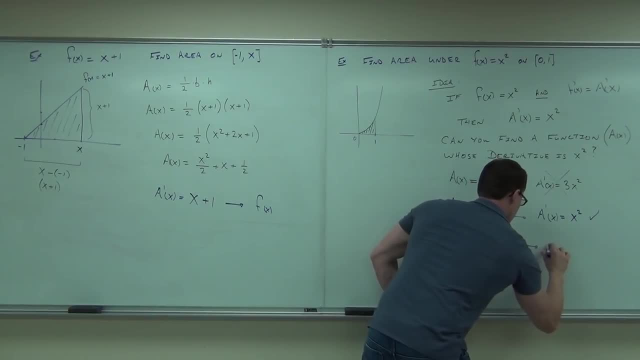 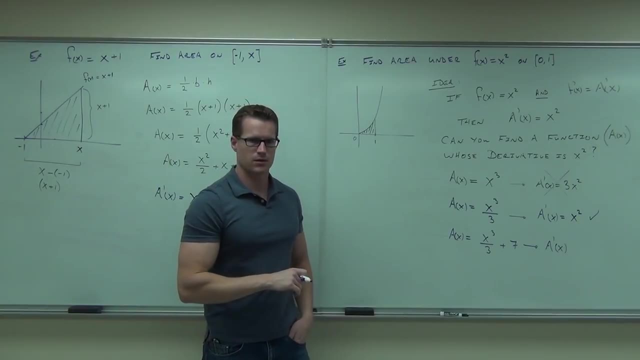 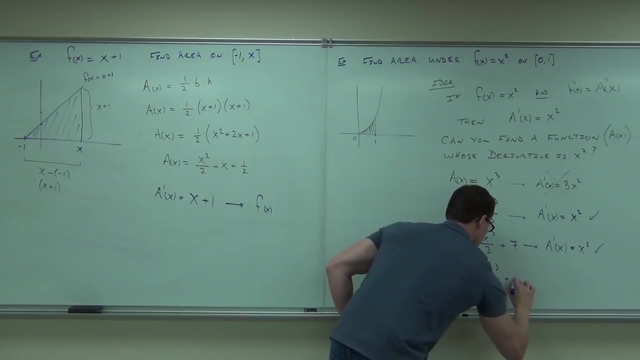 Okay, Okay, Okay. What's the derivative of that? What about the seven? Oh, That's another one that works. What about this? That's not cool, Very cool actually. Okay, does that work? Let's see What about that. 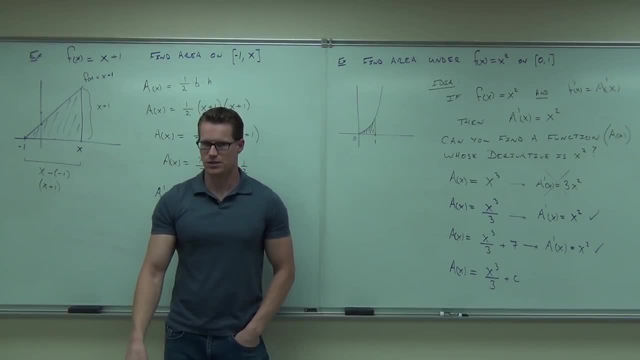 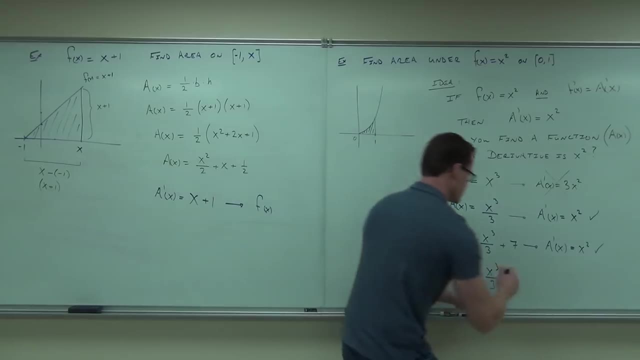 Any constant, No matter what it is. any constant is going to go away when you take a drift right. So what you actually get here is a family of curves, Each of which would work as an area function. So here's what we've done. 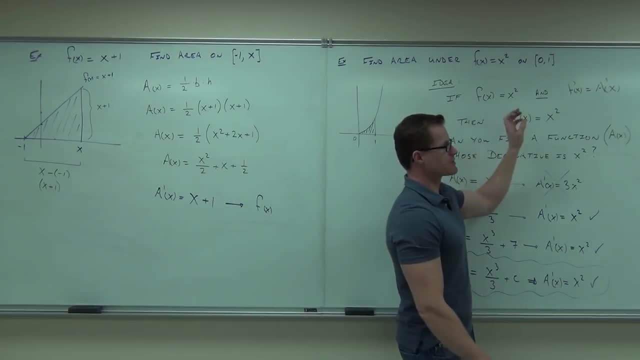 We've started with this function and we've said, okay, I know, the function is actually a first derivative of an area function, whatever that happens to be. So I'm going to set my first derivative of an area function equal to it. I'm going to undo that, treating it like a derivative and undoing a derivative. 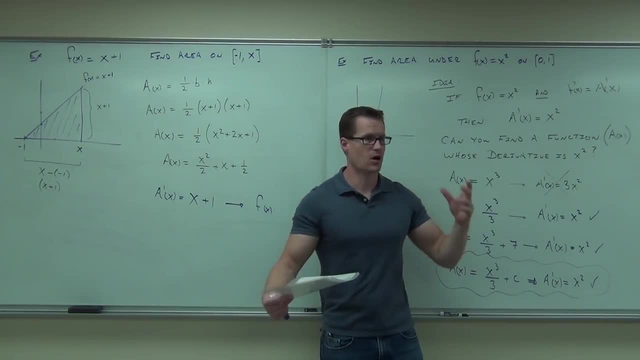 That's why we call it the anti-derivative method. You're undoing anti. It's odd. Okay, Opposite of derivative means derivative. so undoing opposite of you're undoing a derivative. That's what we're doing here. 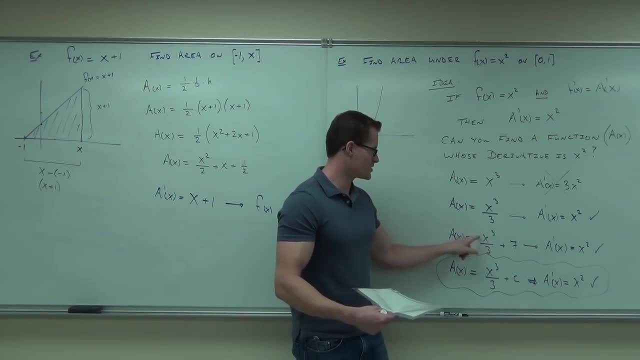 Now, unfortunately for us, this is a. this is a situation. right, We have one, two, we have an infinite number of possibilities for the area function that it could actually be And, in general, that's what you have to put. 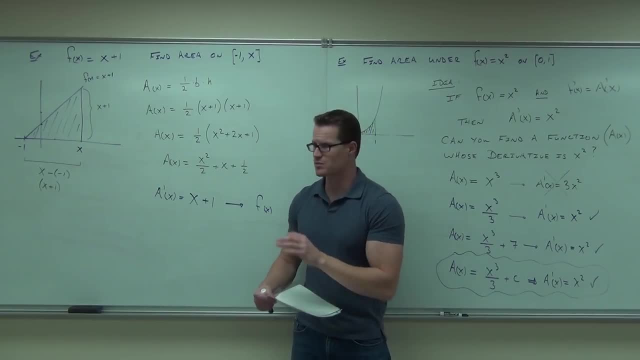 You have to put that centimeter zone out. You have to put that plus C. The plus C is important. It represents a family of curves, each of which could be the area function. Now I've also said some specific things about this. 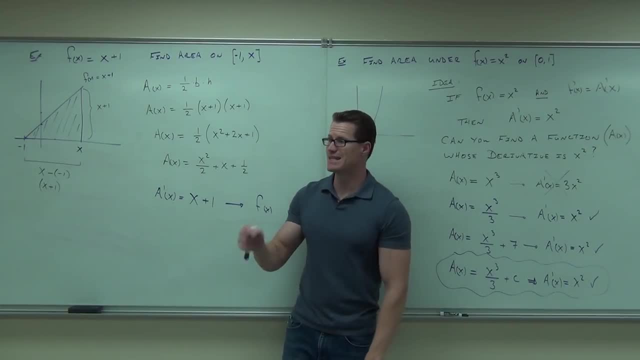 I said between zero and one, which is good. It's going to help us out a little bit. But if I didn't say that this would be the general area functions of X squared, That's what it would be. You'd have to have more specific information in order to give me an actual verified area. 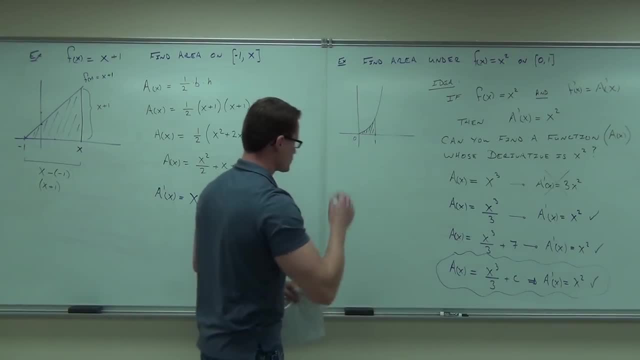 Do you follow me on that? You have to have that, So do you mind if I go over here? Do you have any questions about this one? Are you with me so far that there's more than just one of them right now? 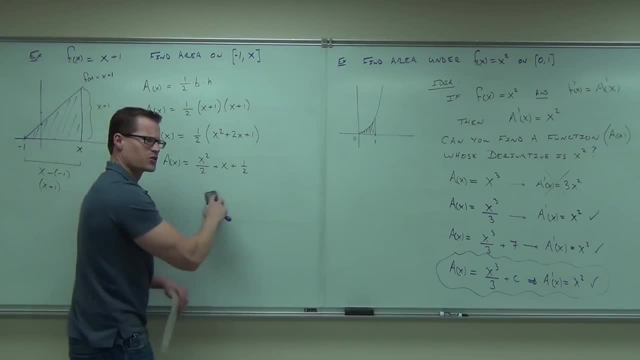 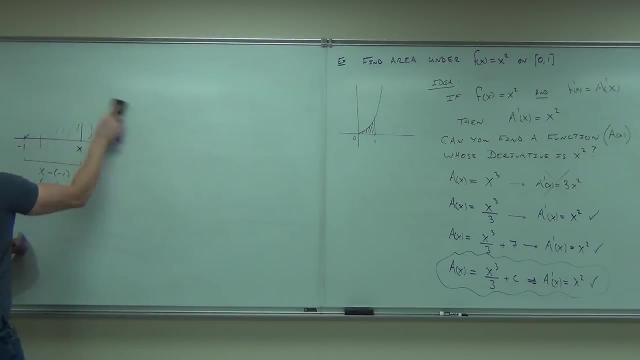 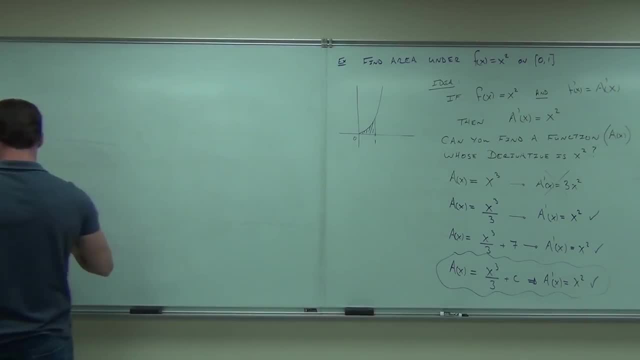 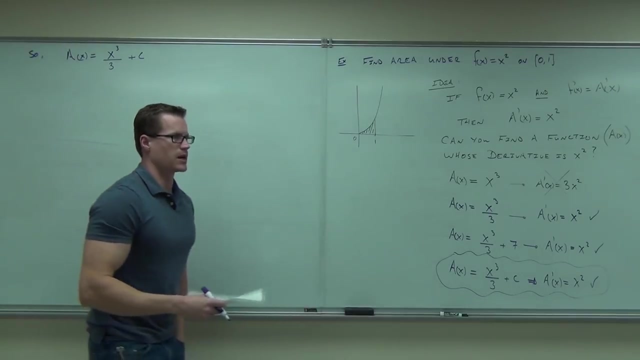 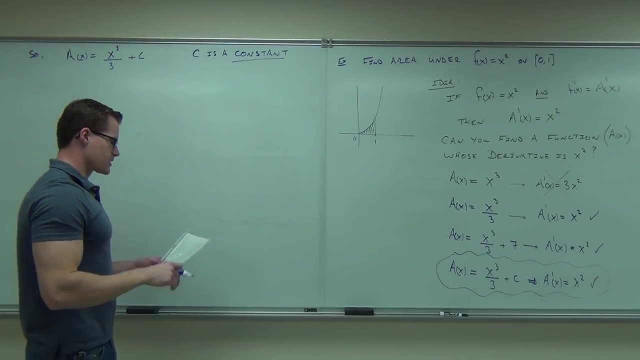 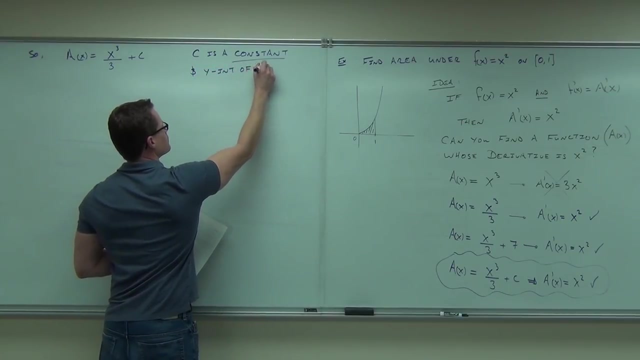 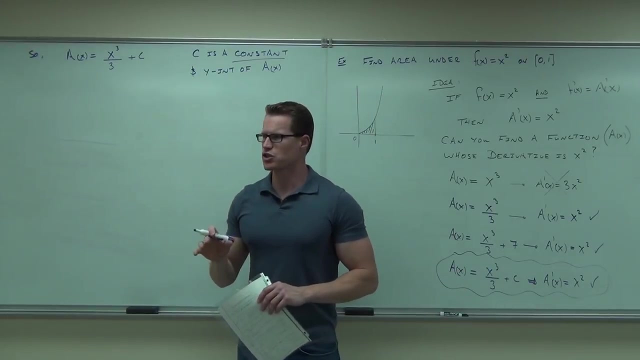 I know right, I was polite today. So heap X equals one third, or X cubed over 3 plus C, C is a constant. C is also the y intercept of a, of x, If something's the y intercept of a function. 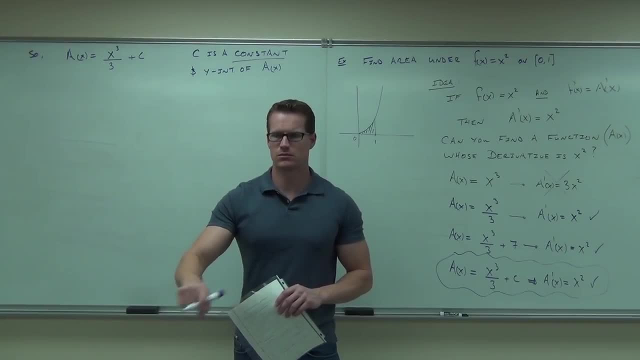 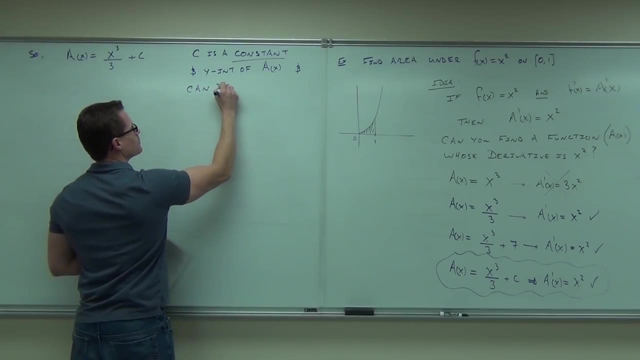 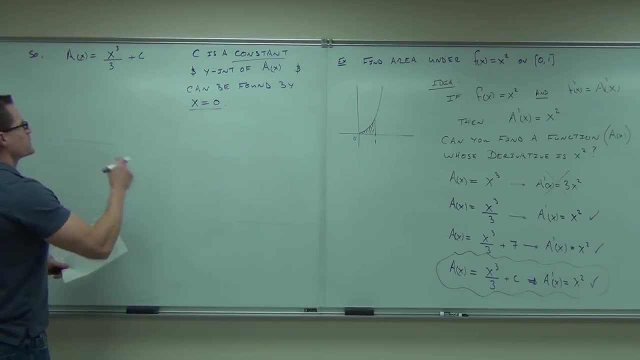 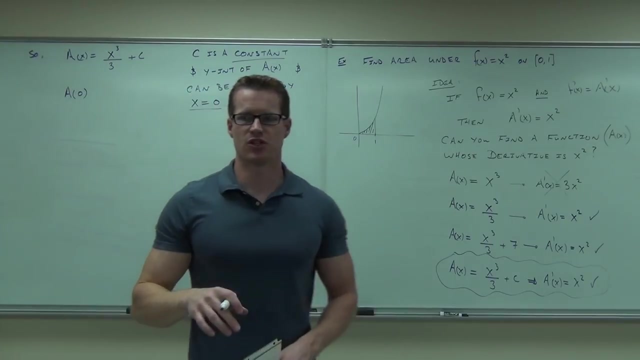 you should be able to find it by plugging in zero, True. So what this means is that a of zero, if I plug in x, equals zero. can you verify that? that's going to give me just the c. Zero cubed over three is zero plus c. 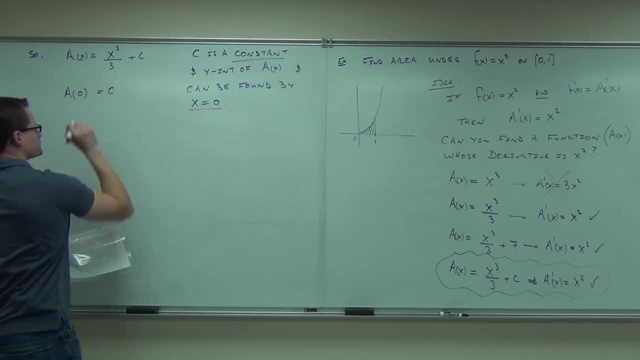 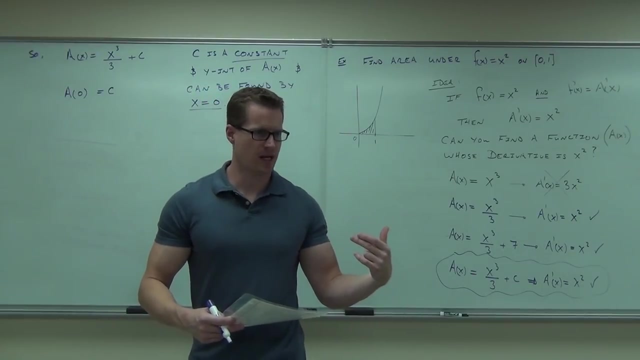 so it's going to give me c. Now, I don't want to blow your mind up too much, but for this context, do you understand that this area curve is from zero to x, wherever x is in this case? That's what that stands for. 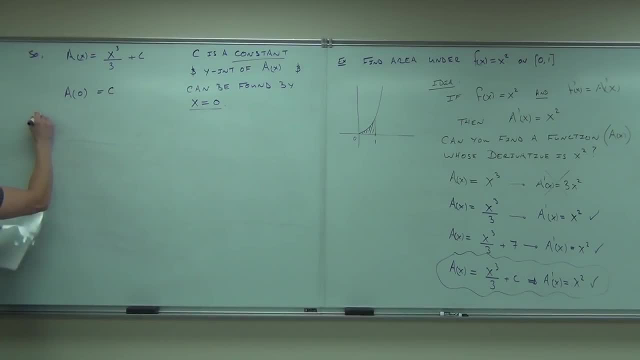 So this interval, The interval is zero to x. This one might throw you for a loop, but I need you to stick with me, okay, If this is the area, If this is the area from zero to x, from zero to x. 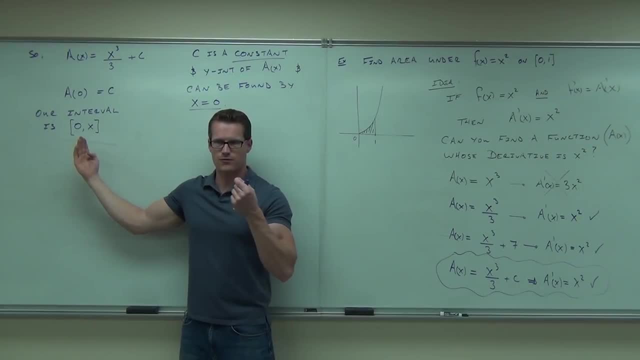 do you follow me on that? It's from zero to x and we are finding the area from zero to What did we plug in for x? One One? No, we didn't plug in one To find this. what did you plug in? 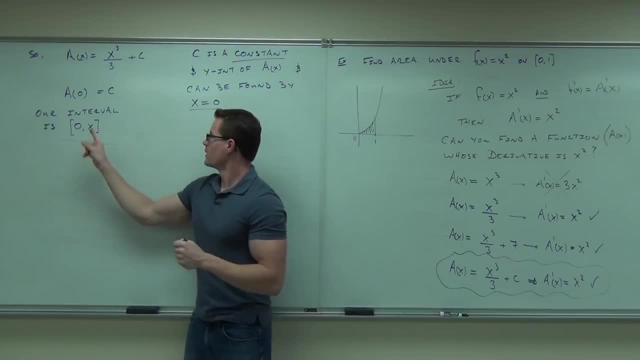 You plugged in zero. When you plugged in zero, what's the area from zero to zero? It's basically saying: what's the area of a single point? Can you find the area of a single point? A point is that which has no breadth. 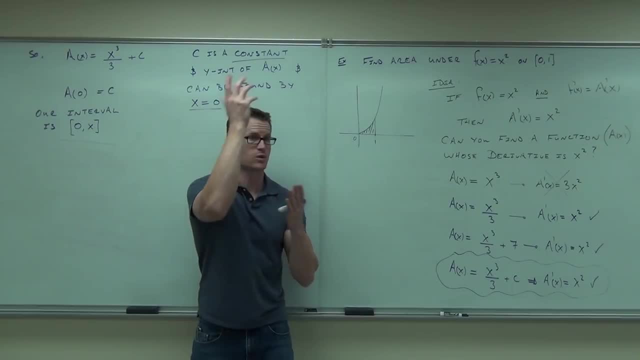 So that means you have no width there, so you can't find an area Zero times, whatever the height is, but you still get zero. So I know this is kind of awkward to think about the area of a single point, but that's what you're doing here. 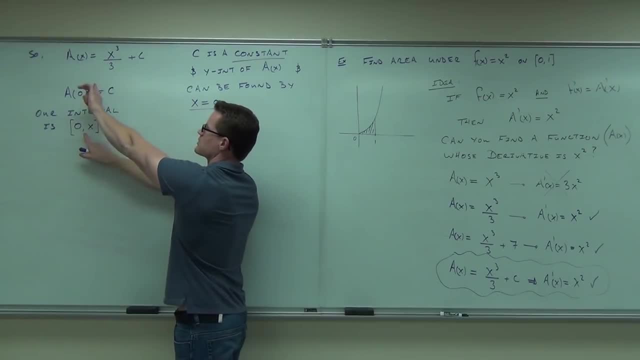 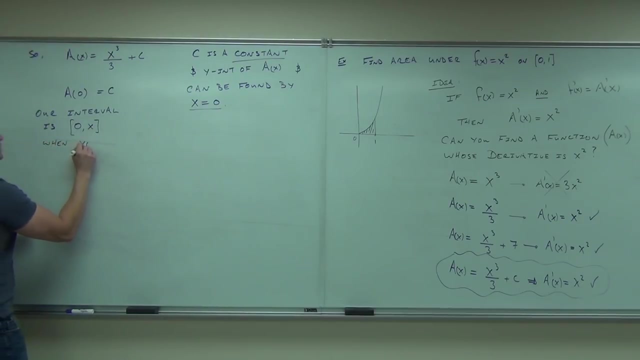 You're saying: all right, I'm going from zero to. I plugged in x equals zero. That's how I got this. That's zero. So what this says is: this is basically the area of a single point. When you set x equals zero, 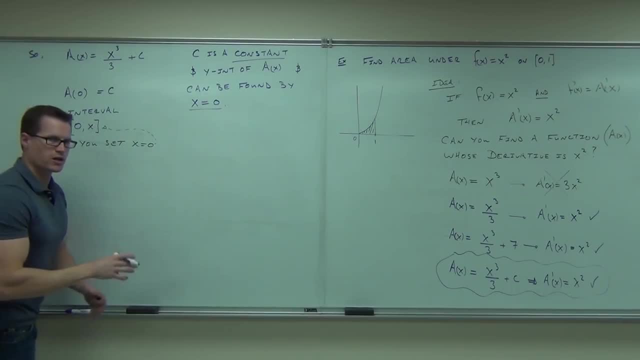 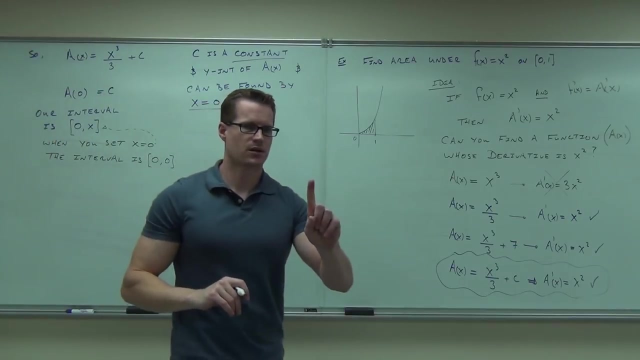 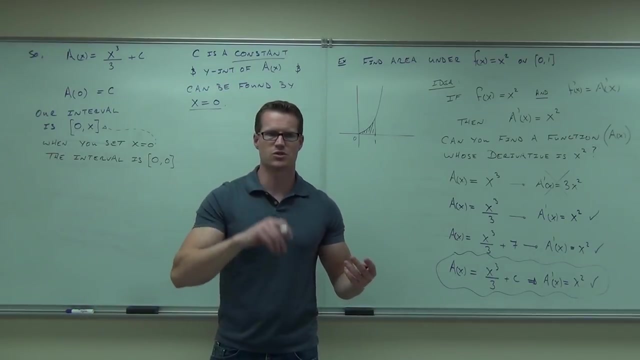 your interval is from zero to zero. That's the area under a single point. The area under a single point is always zero. If you took any statistics at all, you know this, With continuous distributions. if you ask what's the probability of an exact number, it's always zero. 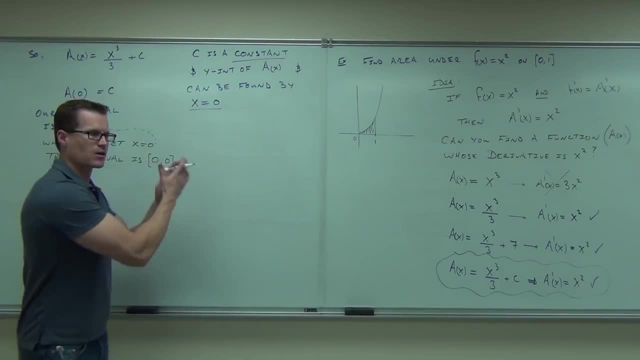 You can't get it because there's infinite number of possibilities. That's the same idea. The area is zero. So when you set x equals zero, the interval is zero to zero. That is the area under a single point. That's the area under a single point. 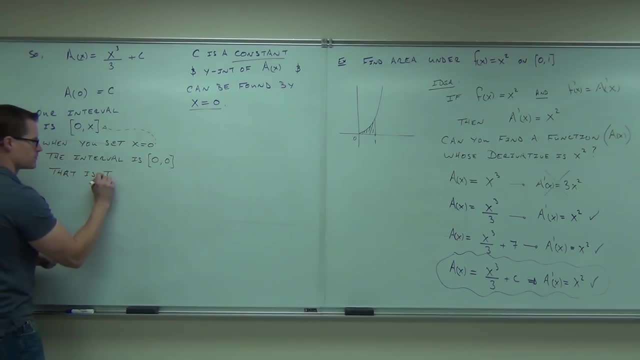 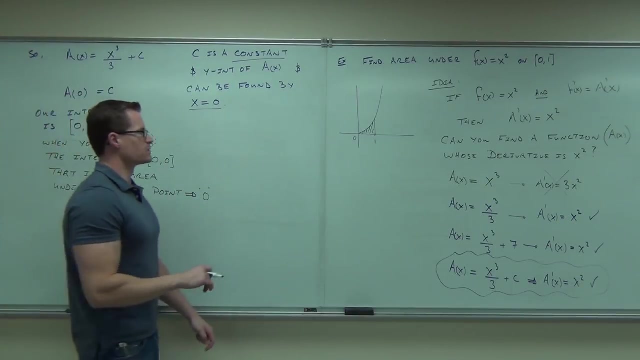 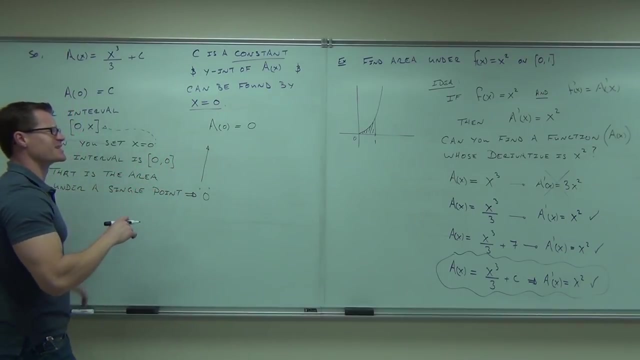 That's the area under a single point And that's zero. So what this says is from here: if you set x equals zero, your interval is zero to zero. Here's what this says. It's two parts. Oh, I got to sneeze. 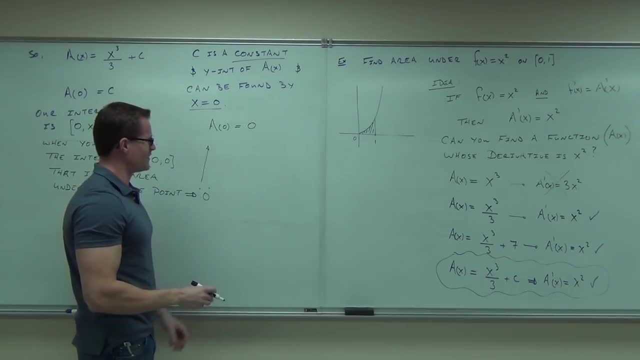 Oh, it did come out. Oh, don't you hate that When you're all ready for it, and then nothing. Oh, I hate that. And then your nose tickles- Yeah, I hate it. Nose tickles, Oh bummer. 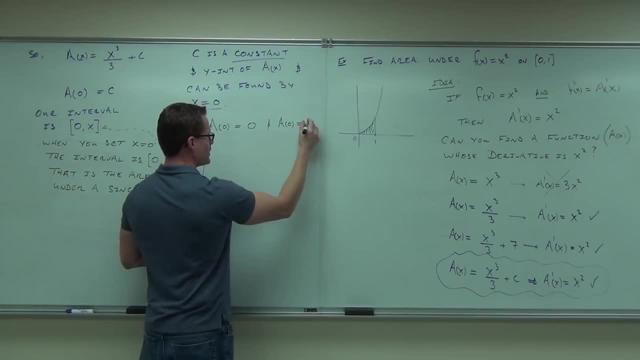 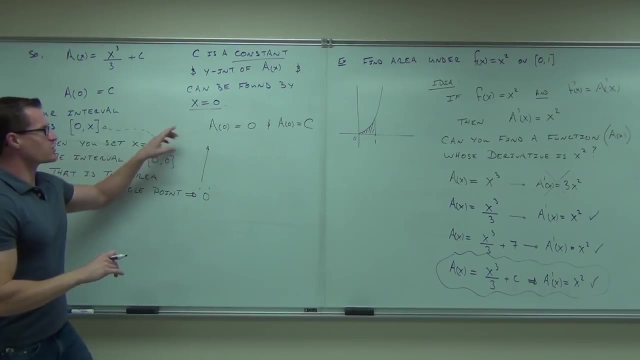 It actually looked like you sneezed for a second. I tried, I kind of pretended, just so it would look good on camera. Yeah, Valiant effort, Thanks. So here's what this part says. This says: if you're going to plug in zero, your area goes from zero to zero. 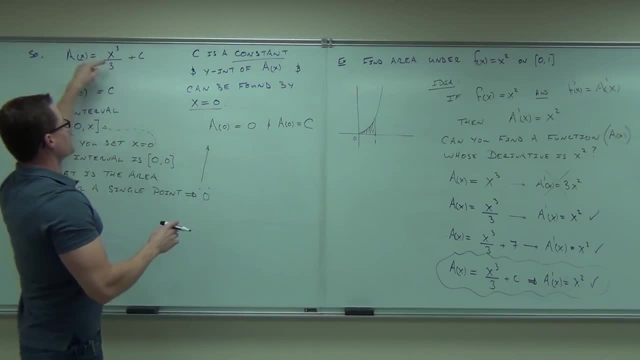 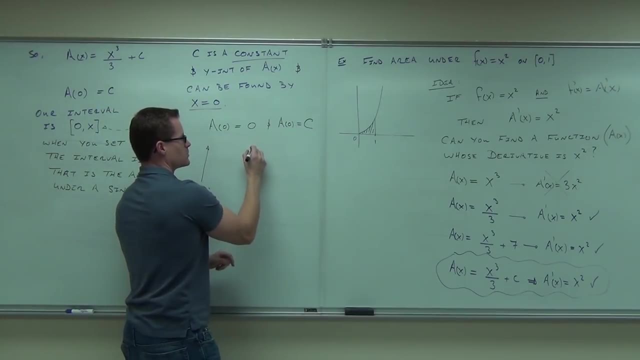 That's area under a single point, That is zero. This part says: well, I know, when I plug in zero to my function, I get c. Therefore, if a of zero equals zero and a of zero equals c, how much does c equal? 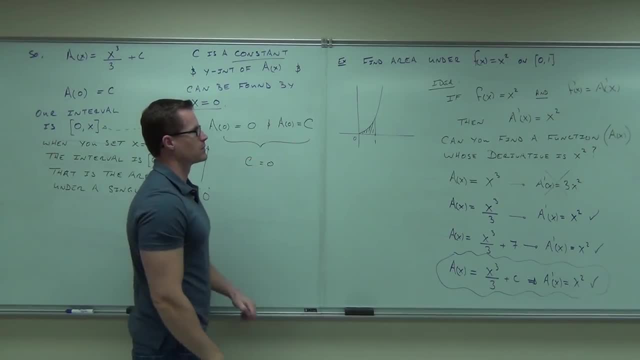 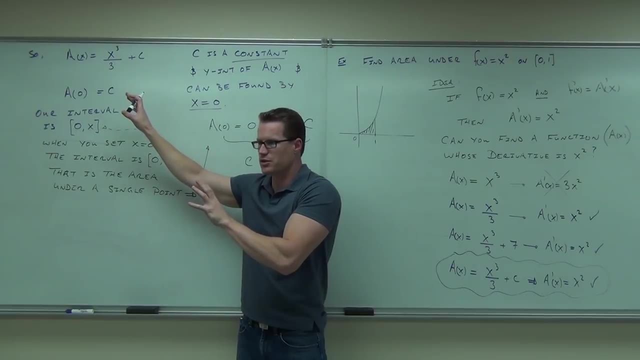 A of zero. Yeah, that's right. What that says is, though, even though we had the c, we had to take care of the c. The c doesn't always have to be zero, It can be numbers too. We're going to talk about initial value problems later on, later on in this section. 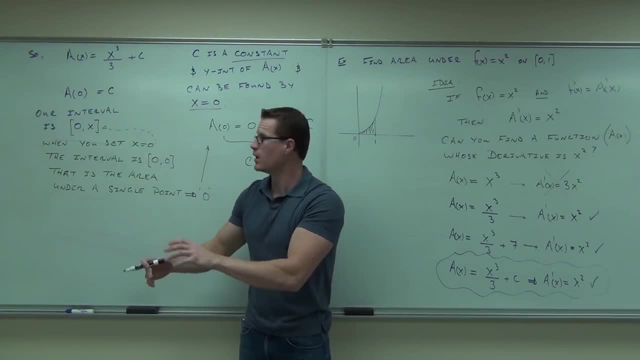 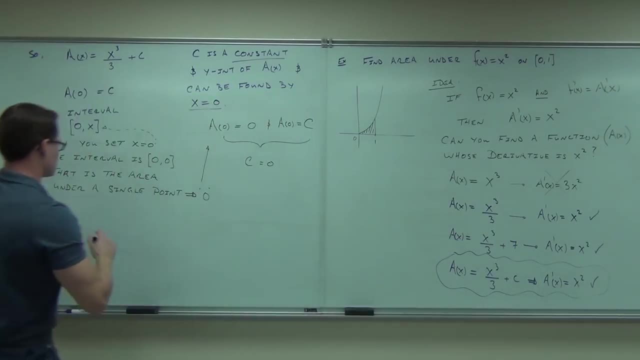 You might have some c's that are numbers. This one: you get a zero. So this is what you'd be able to do from this part. After you find your c, you go. okay, Then the area of that curve is x cubed over 3.. 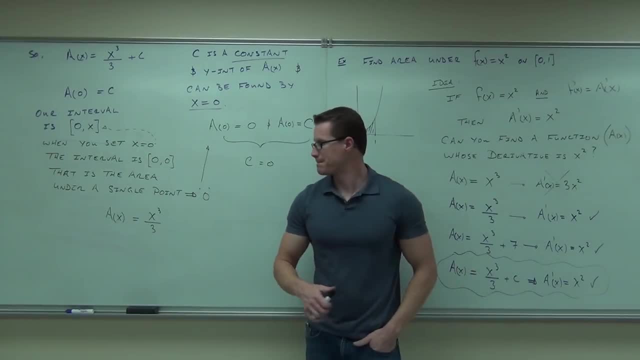 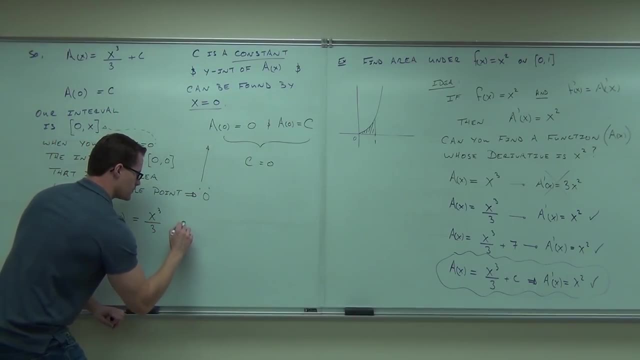 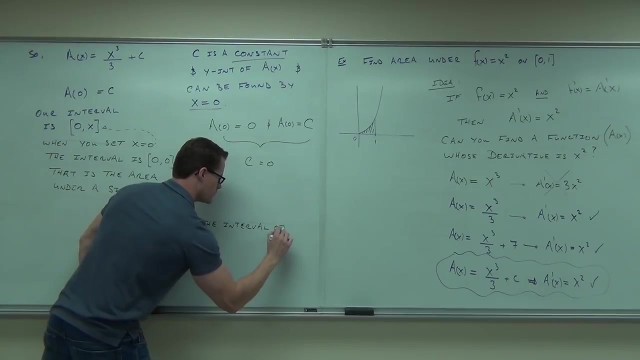 We'll hold it down. Now you can start plugging注意- the numbers in. now that you've d-одled a, c. Now you can start plugging highlights in. Remember on the c function on any unit in the proper order. 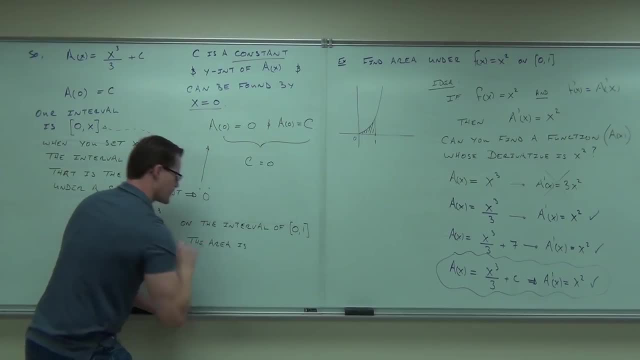 keeping an automatic do lot thing in the proper order And let that be d over c, And I do that very quickly. Now you can start plugging numbers in. Then the area is. well, let's fill that in. Our area went from zero to x. 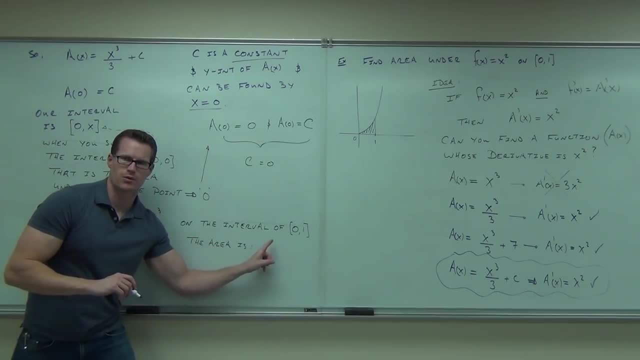 Can you tell me what is the x value of our interval there where we're stopping? You can now plug that in. Now that you don't have that c, you wouldn't know that c is zero, right, You'd be able to plug in the x of one. 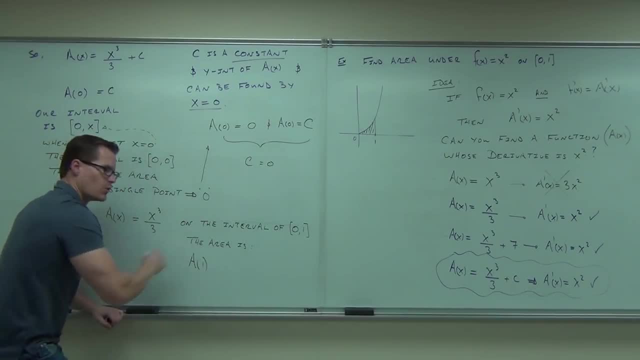 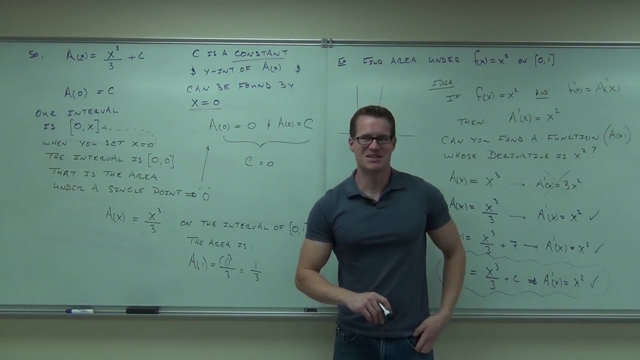 You go: okay, well then, the area that stops at one is one cubed over three, One cubed over three or one-third square units. Now, that's our idea. Did you follow the idea? I've given it to you in terms of geometry right now? 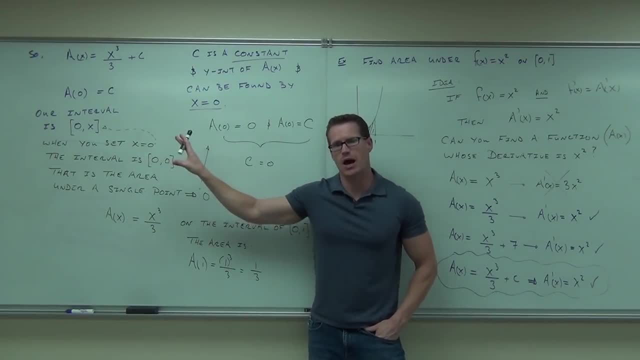 I've showed you some interesting ideas with area to kind of flesh this thing out a little bit. Right now we're gonna take a jump away from the actual area. I just wanted to introduce it to you, So it was a very long introduction. 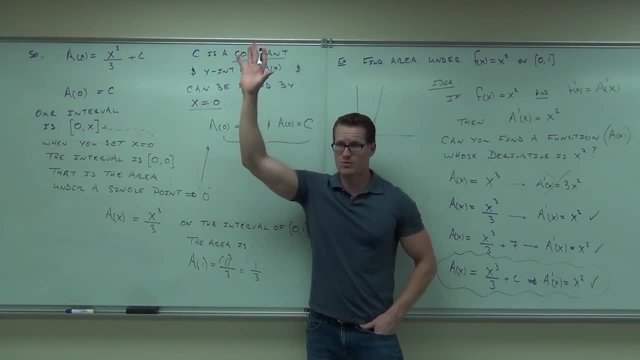 Do you understand the introduction? How many of you feel okay with it? So rectangular method is you cut it into rectangles. So rectangular method is you cut it into rectangles. So rectangular method is you cut it into rectangles. We'll talk about that later. 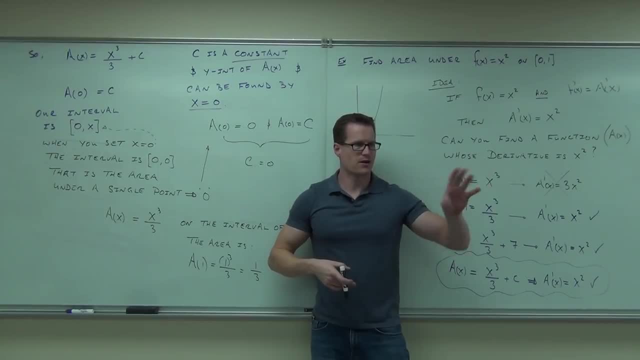 Anti-derivative method is you go? okay, the first root of the area is my function. Let's undo a derivative That gives us an anti-derivative. We somehow have to mess around with the c. We have to figure out what c's are. 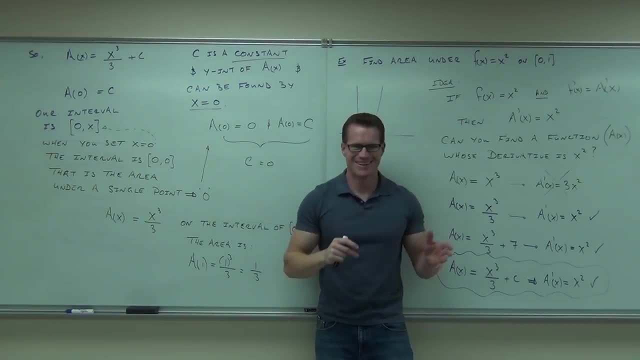 I'll show you better ways to do this as we go on by the way. better ways? Yeah, I don't. I need you to understand the idea, You need to get the idea. I'll show you some shortcuts and ways to work around that. 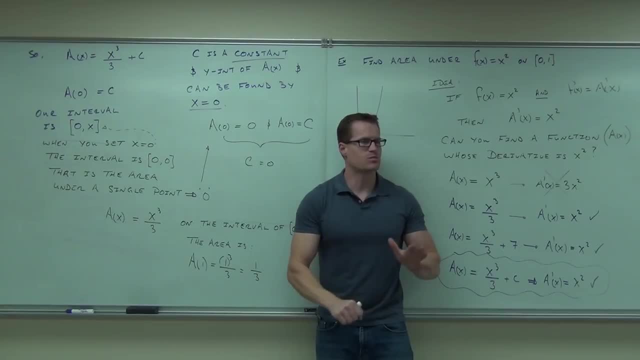 You follow, But you have to understand the idea. Now we're gonna practice most of the rest of our time in this section on how to actually do the anti-derivatives. This was fun, but I haven't showed you any techniques on how to do that yet. 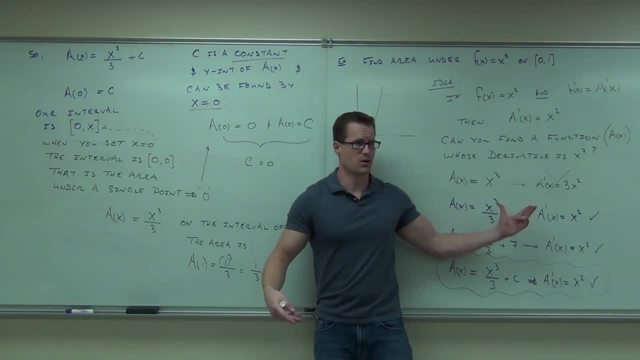 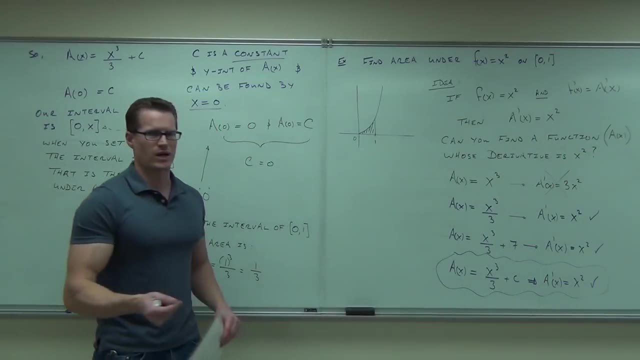 I've said, basically you need to be able to undo it, and we kind of guessed and checked over here. Would you like some better ways to do this? Yes, Absolutely. So we're gonna start talking about that. This is called the indefinite integral. 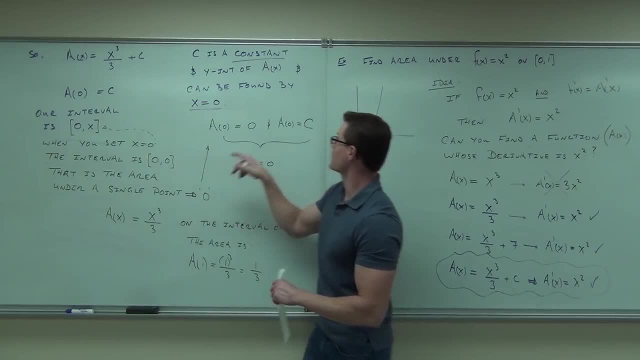 Indefinite means that I'm not gonna give you boundaries yet, I'm not gonna give you zero to one yet. That would be a definite integral. That would be the area between the points. That's what we were able to find right. 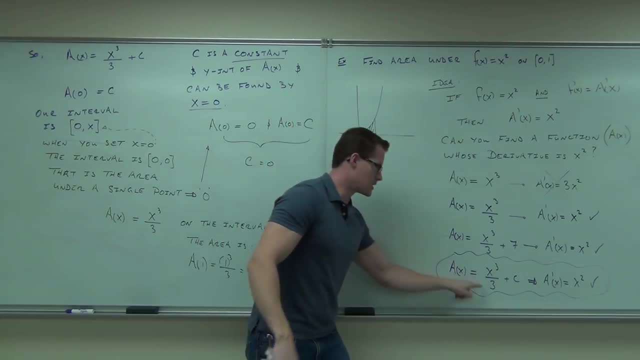 An actual number. What I'm gonna leave you with is how to get down to here That part. This would be indefinite. Let's say you have a plus C, You don't know where you're stopping, You don't know where you're starting. 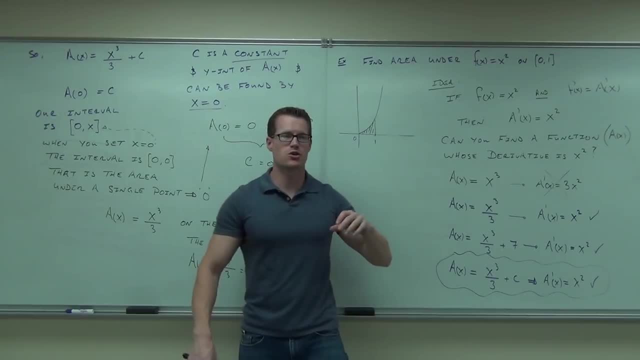 It's just an indefinite integral, because I haven't given you a range of numbers. Therefore you can't find the definite area. We're just having the function of the area. Do you see the difference there? If you didn't catch what I said, 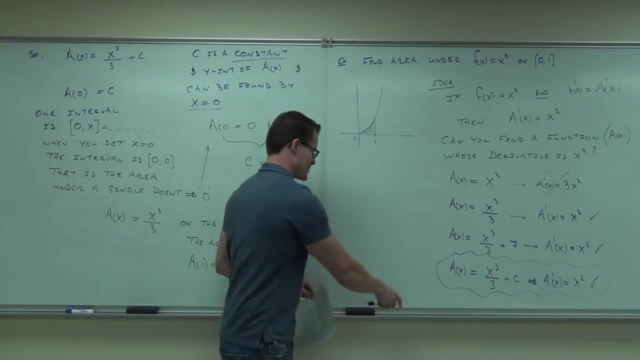 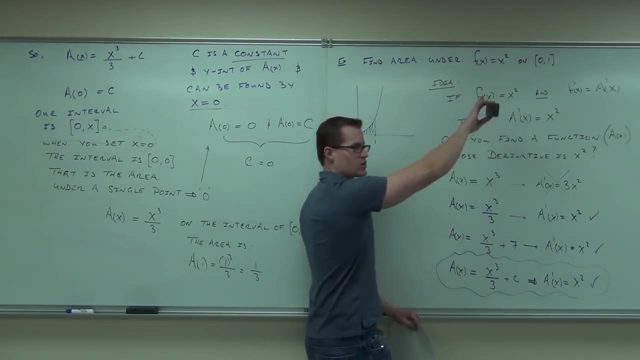 rewind that and repeat that. Some of you are getting kind of like weird looks. You don't quite get that. I'm gonna leave it here. I'm not gonna give you numbers to start and stop at. I'm gonna leave it here. 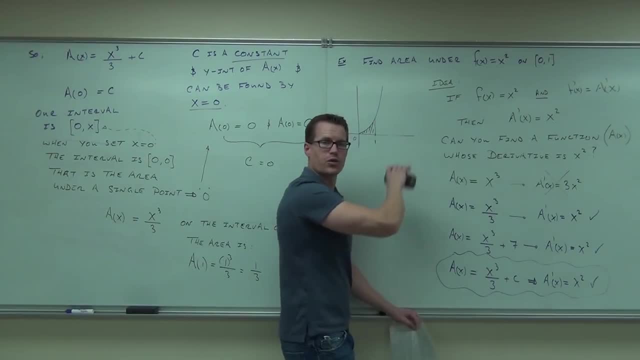 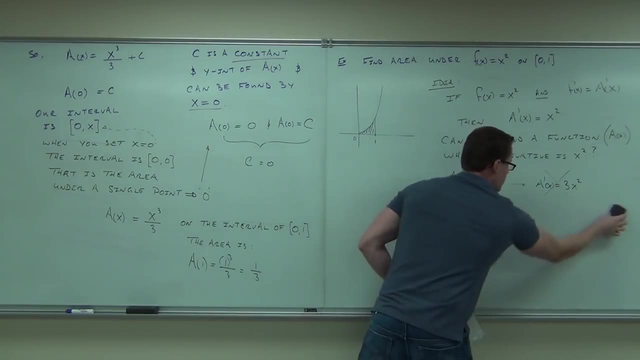 Show you how to get this, And later on we'll talk about how to do the whole thing together. So remember this was an introduction. So indefinite integral means that you're not gonna be able to find the area- definitely. That's why I'm calling it indefinite. 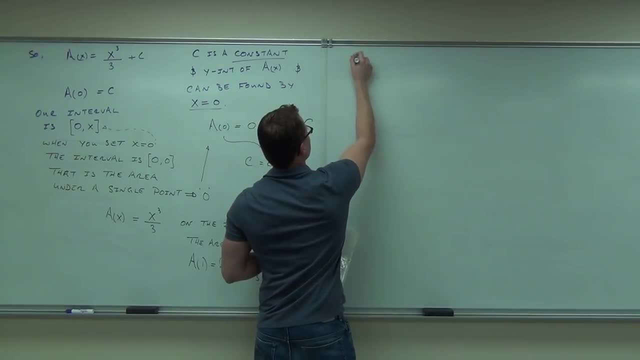 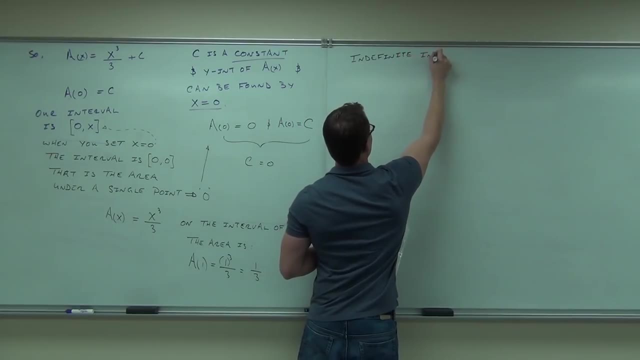 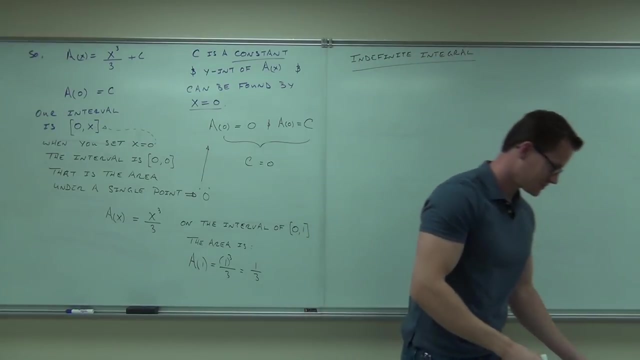 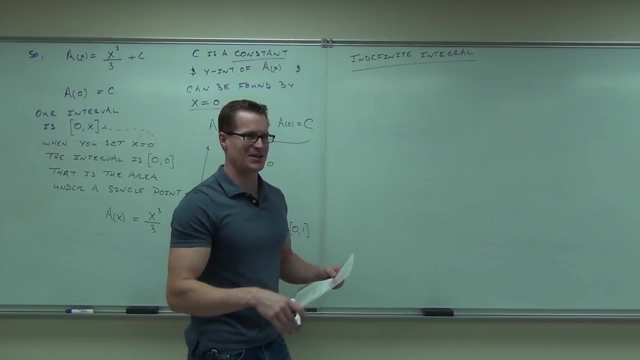 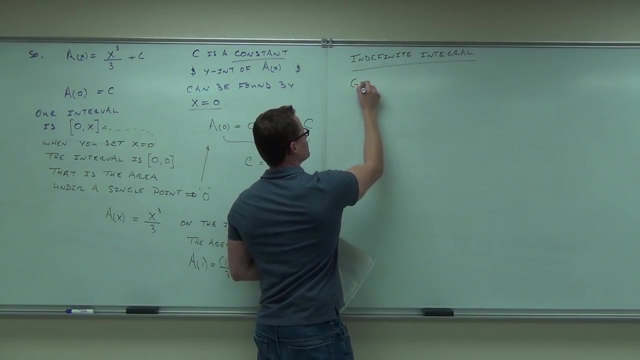 Oh yeah, I guess I should call it. This would be like a subsection. So there's a new word on the board: Integral. I'll bring down to what an integral actually is. It's not our concept. Given a function, let's call it f. 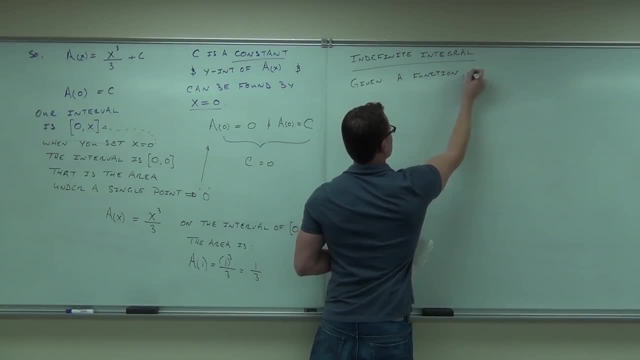 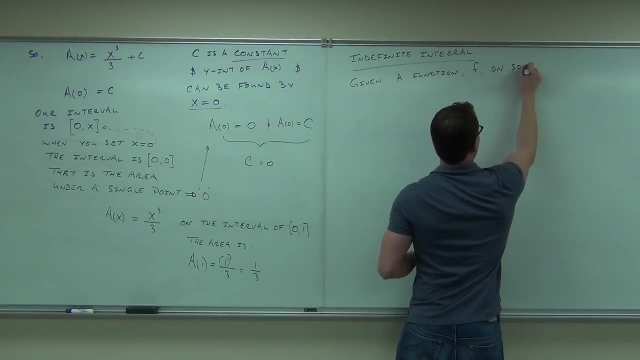 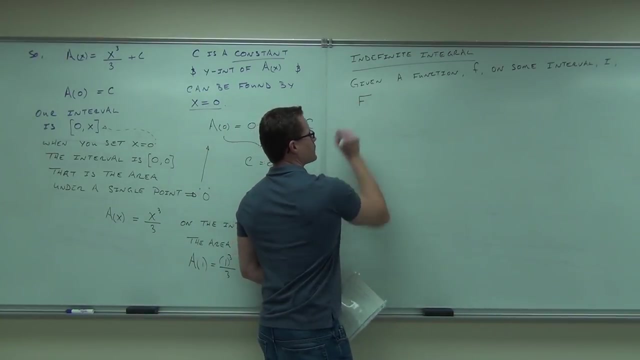 On some interval. let's call it i. I know this doesn't start out so fun right now. Okay, it sounds boring, It's not that bad, Just stupid. Given a function f on some interval, i capital. F is called the antiderivative. 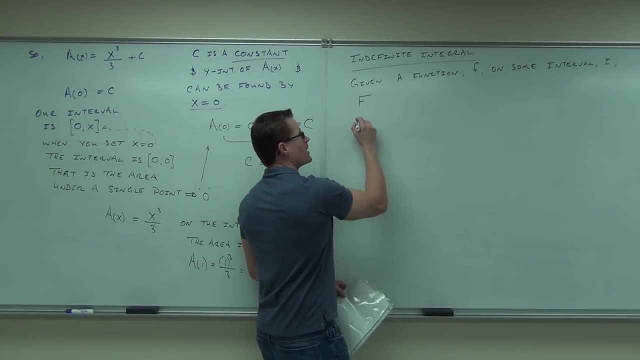 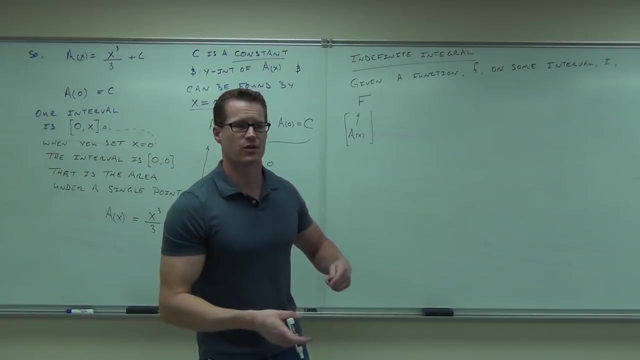 Please make a note here. This is also the area function. Okay, In general we call the antiderivative just the capital letter of whatever the function is. So if we have a function f, the antiderivative is capital F. That's all we're saying here. 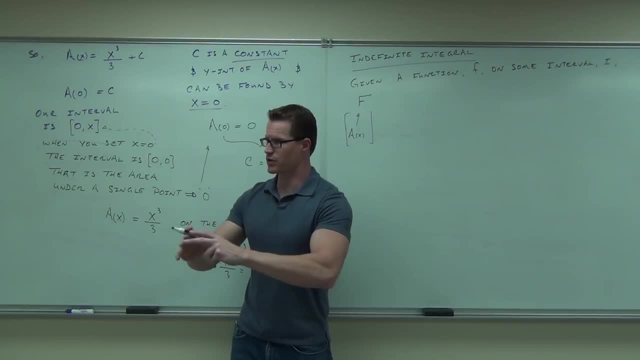 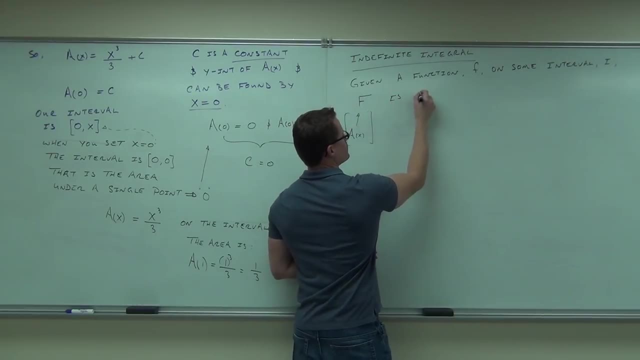 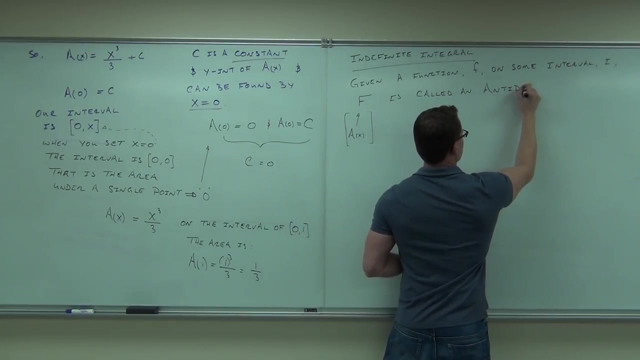 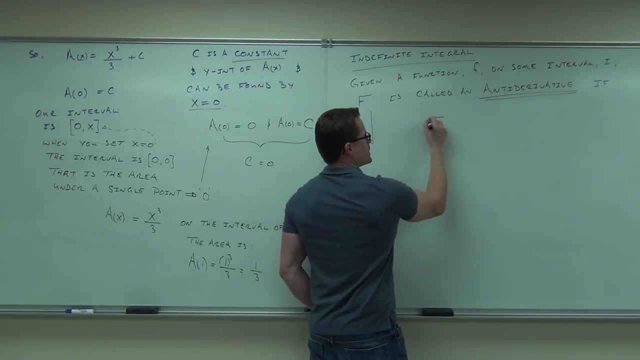 It will stand ultimately for the area function of your curve. Do you follow me on that? Now let's listen to what we'll stand for. F is called an antiderivative. If this is true, If you can take the first derivative of your curve, 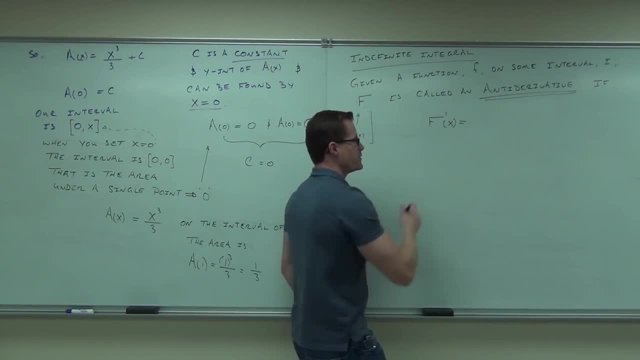 and you get the other side. if you can take the first derivative of your curve and you get the other side and you get the other side and you get the other side of your capital. F your antiderivative and it equals your number of x. 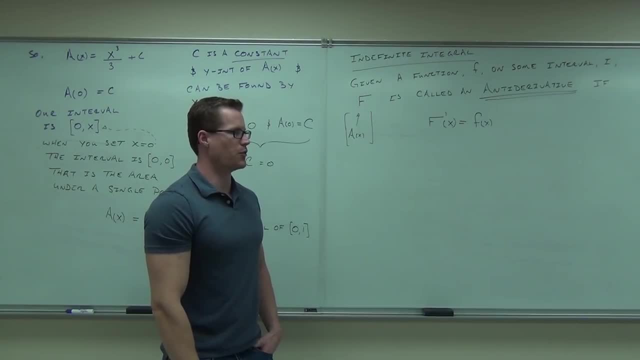 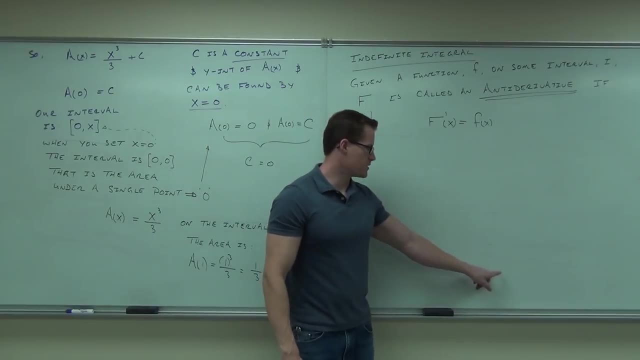 You'll notice I used the word and instead of the word the Think back to like 10 seconds ago- maybe like 30 seconds ago, when I said you had a plus c. You can actually almost see it in the purple writing that it doesn't quite erase that well. 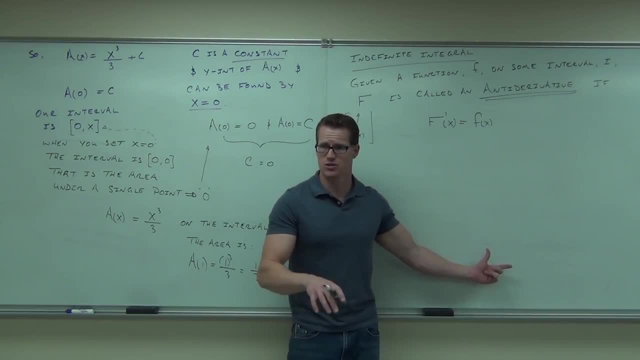 Remember how we had several, actually an infinite number of functions that you could take a derivative of, and it will give you your original function back again. That's why I say: and That plus c gives you a whole bunch of them, a whole lot. 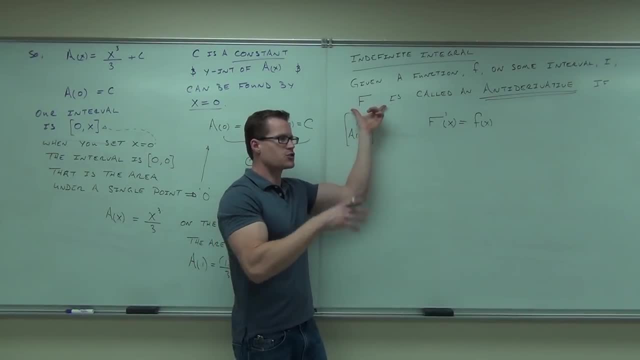 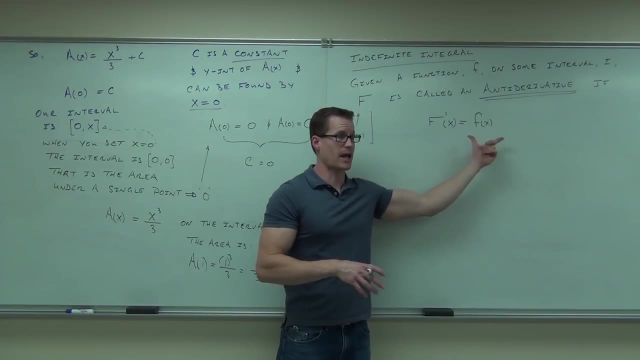 of them. And so what we're doing here is we're saying: F, F should be some function, that when I take a derivative of it it gives me my function. I'm looking at That's what happens. That's what an antiderivative is known as. 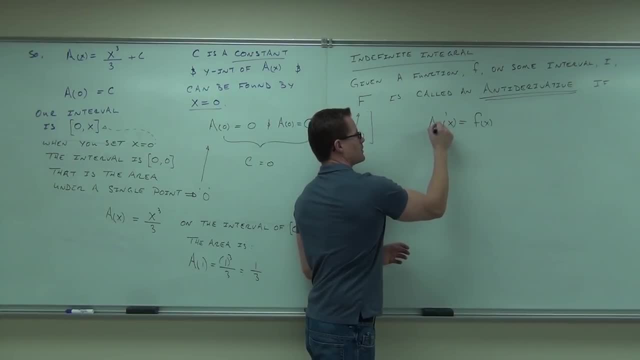 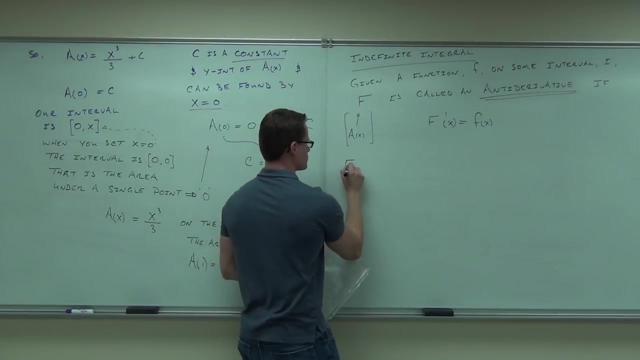 Now, we just talked about it like this: right Same stuff. A was the antiderivative, F is the antiderivative Same stuff, OK, OK, Let me give you the example that we just talked about. So capital F of x is the same as saying A of x. 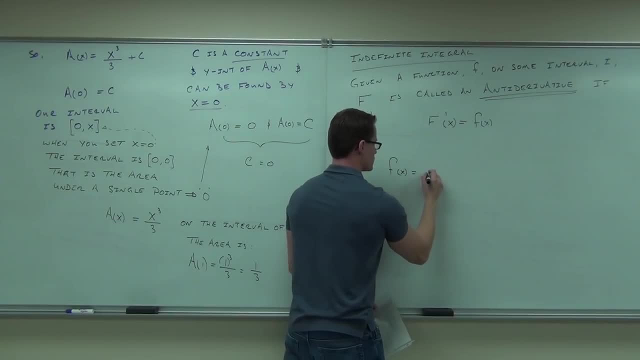 So it's the same as saying it's an area. OK, You remember this example right? In fact, it was on the board. It's on the board right there. Here's what we'd say for this. We would say that F of x has an antiderivative of capital F. 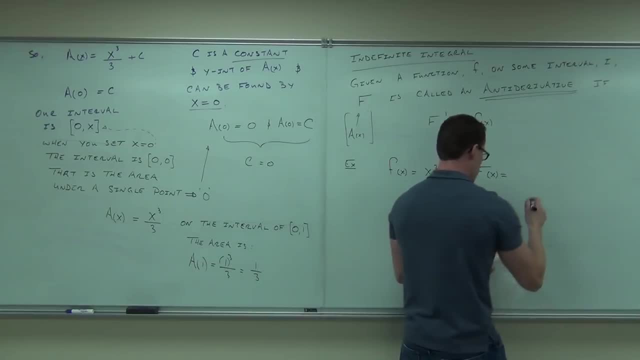 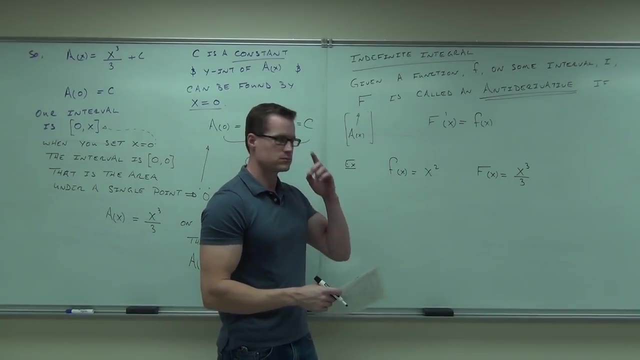 of x And capital F of x should be 1 third or x cubed over 3.. OK, You on it. Want to hear that again. You OK with this so far. You okay with it so far. You OK with it so far. 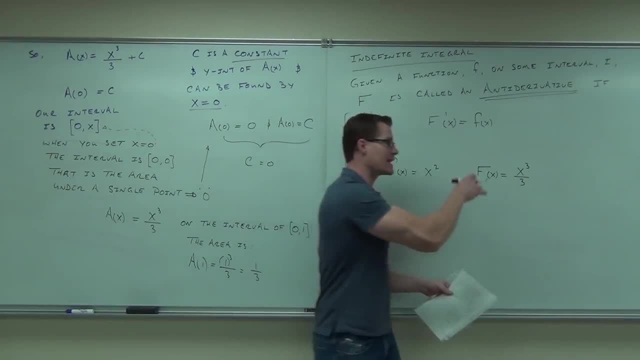 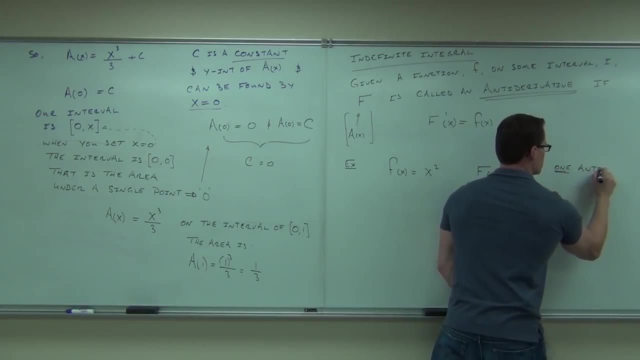 Is this the antiderivative or an antiderivative One of the many? It's one of many, It's one of many. This is an antiderivative. This is 1 antiderivative. I'm just saying anti-D. 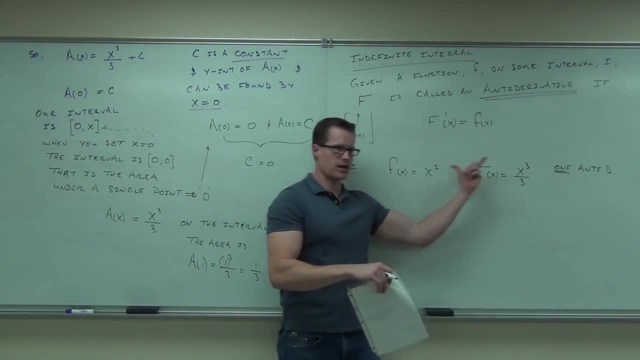 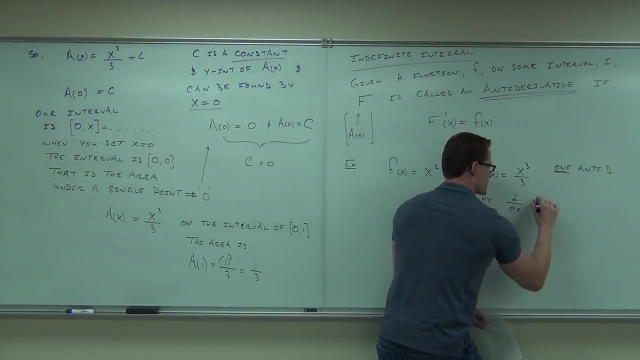 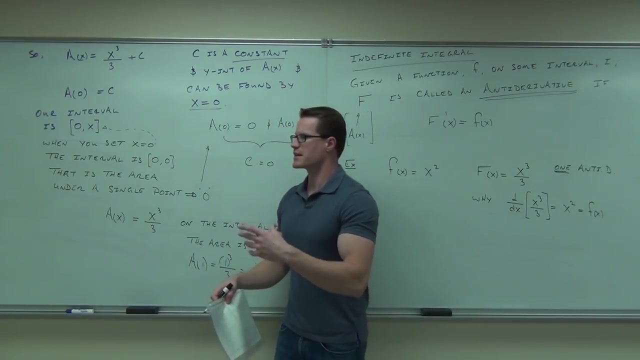 Why is it an antiderivative? Why, Antiderivative of this, does it not equal this? Why? Because the derivative with respect to x of this thing is this thing, which is f of x. That's why it works. This is all I'm saying here, folks. 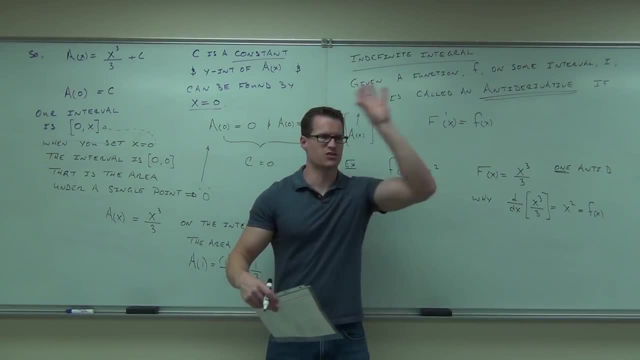 An antiderivative is this property. It says: I take a derivative of it and it gives me a function. That's what it is. This is one of those. Are there more? There are many more. There are infinitely many more. I gave you another one. 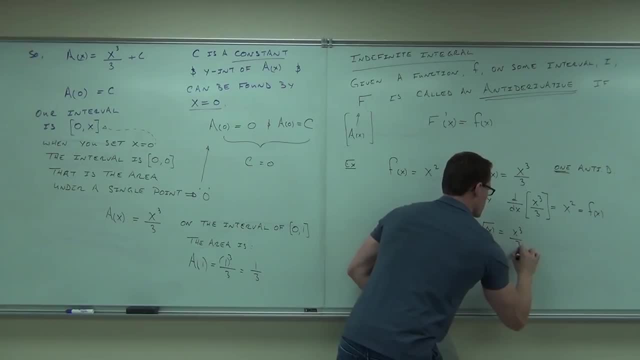 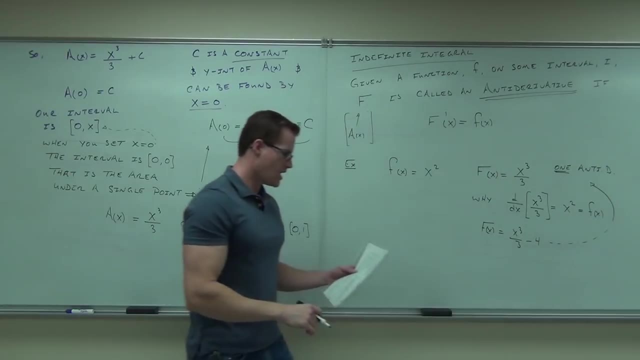 Another f of x would be x cubed over three minus four. Is that another one? That's another. That's another one of those antiderivatives. That's why, in general, all of them will have this form. That's why we have 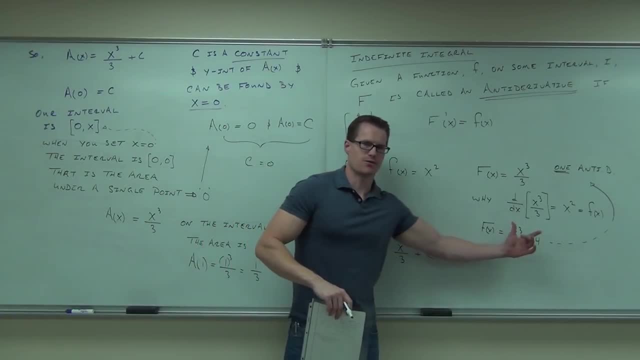 f of c to say: okay, you know what? I'm kind of tired of writing every constant over here. I don't want to write minus four, I don't want to write plus three, I don't want to write plus whatever. 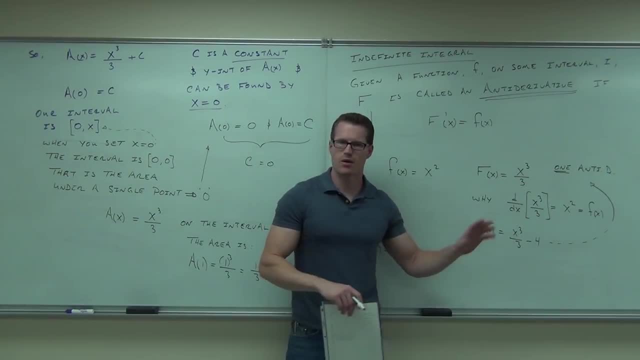 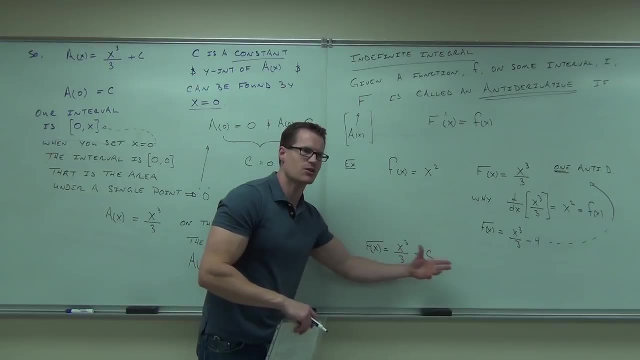 I don't want to write zero plus pi minus one half. That's all garbage. I don't want to write that. I want to represent this. This represents all of the possible antiderivatives. Do you follow me on that? I can't have any other x's. 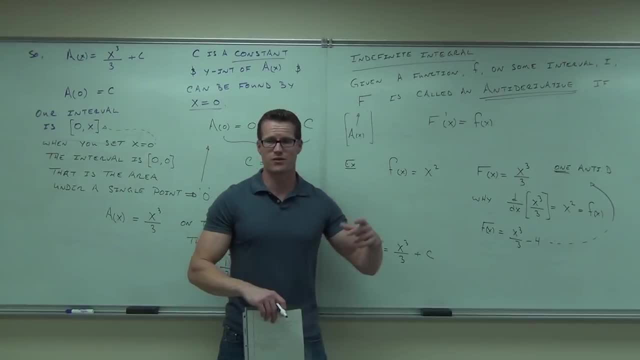 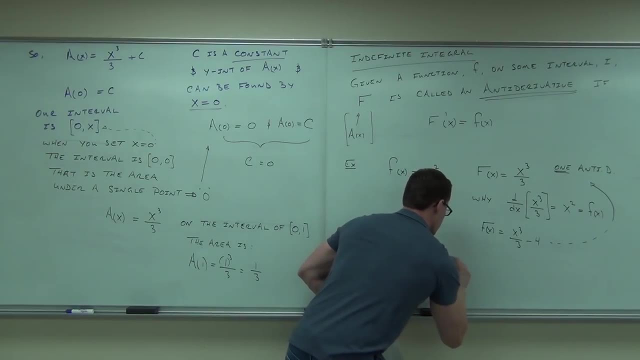 because that would alter the derivative, but constants don't, because we take a derivative of a constant and it gives you zero. So this right here is all antiderivatives, the family of all antiderivatives. I'll talk about that next time. 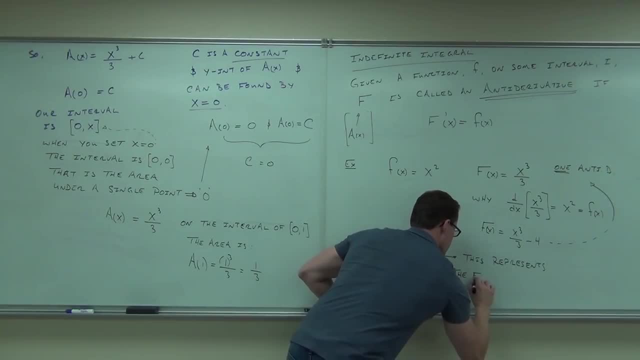 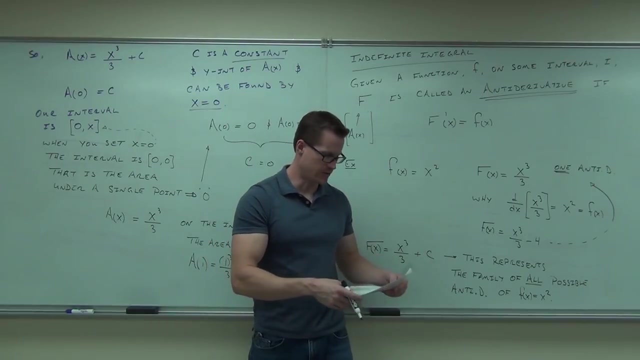 This represents the family of all possible antiderivatives for f of x equals x squared: All of the possible antiderivatives. Will other functions have different antiderivatives? Of course they will. Other functions have different derivatives, so they will have other antiderivatives. 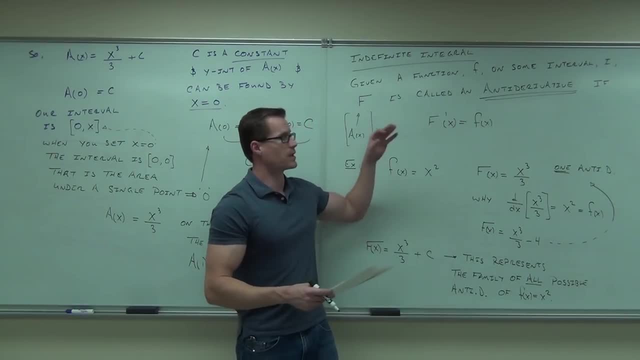 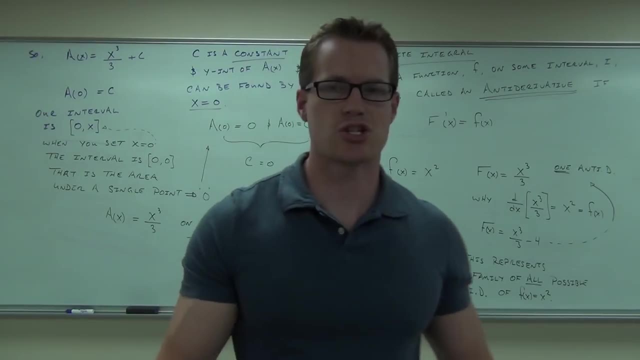 What I will do next time is I will talk to you about what an integral is. what an integration is. It's basically you'll find out, the same thing as doing antiderivatives, so I'll show you some notation and that will be where we continue. 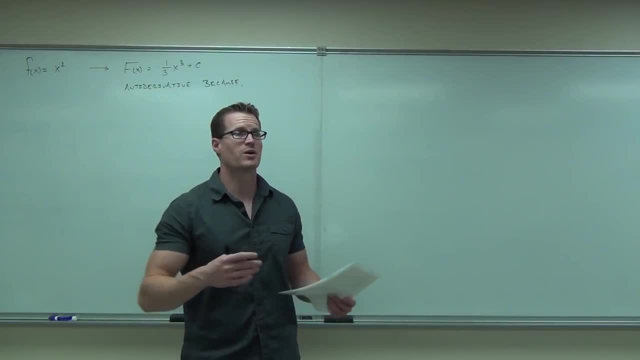 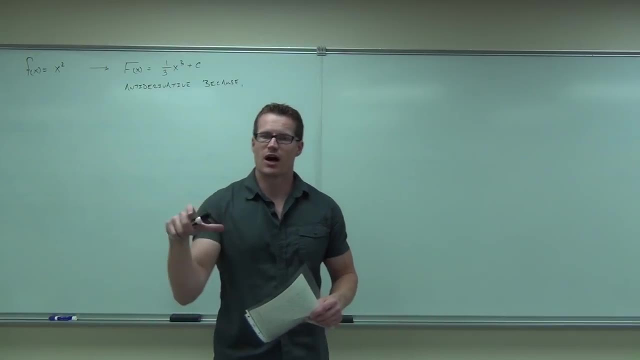 Our study of calculus has brought us to this point where we're not talking about derivatives so much anymore. In fact, we're basically doing the opposite of a derivative. From last time we learned that if a function has an area under its curve, 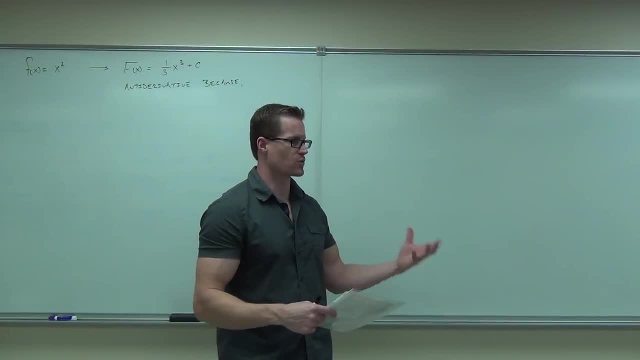 that's the area function, or in other words, that's the antiderivative. So basically, it's left to us to undo a function by pretending it's a derivative and saying: how can I reverse the process of taking a derivative? That process is called anti-differentiation. 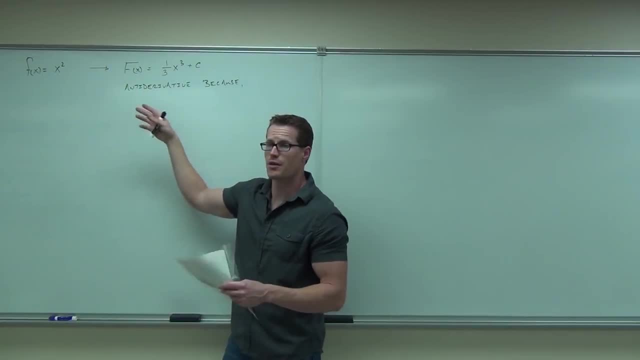 or finding the antiderivative. We left with this example: The antiderivative of x squared is one-third x cubed plus c. Why the plus c? Because there's any constant Good. The point of an antiderivative was, if I take a derivative of it. 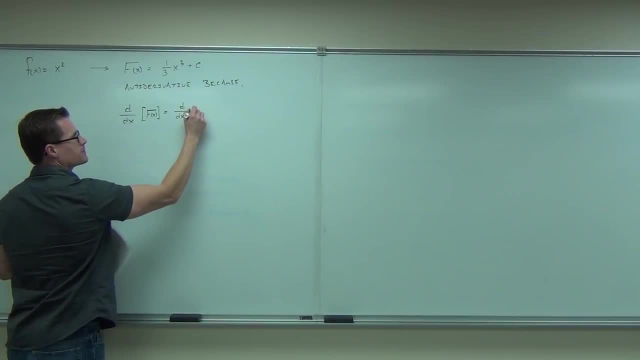 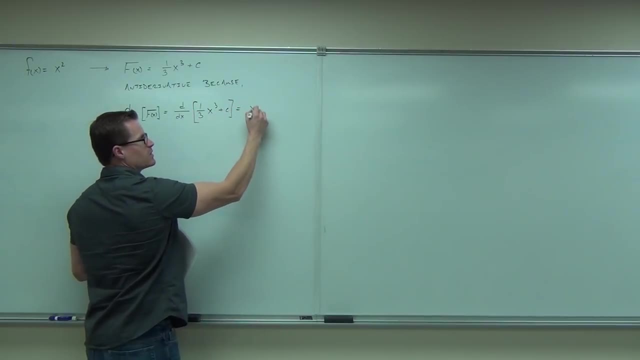 in other words, the derivative of one-third x cubed plus c. in other words, the derivative of one-third x cubed plus c. it will give me back my original function. That's the idea of an antiderivative. I take a derivative of it. 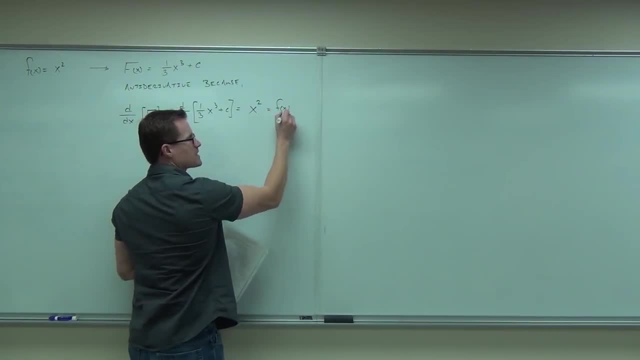 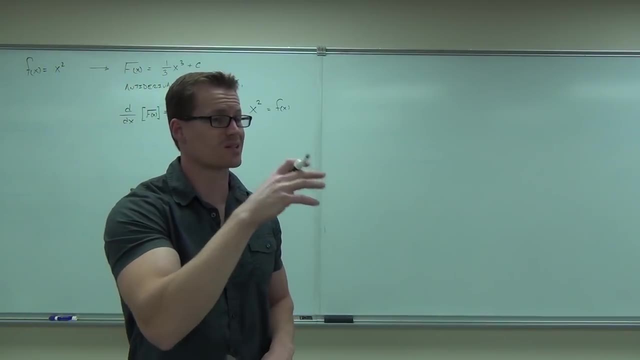 it gives me my original function back. Does that make sense to you? The plus c is there because, well, any constant's going to go away when I take a derivative. So that is basically a family of curves, a family of area curves. 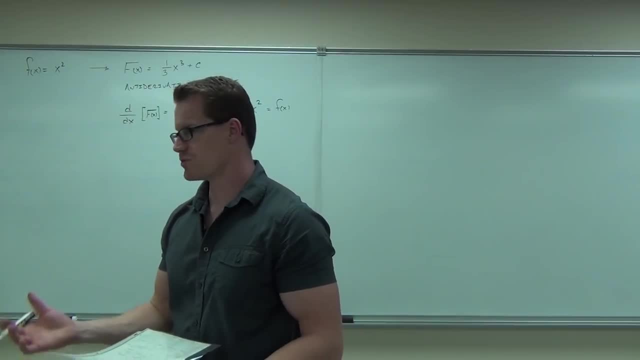 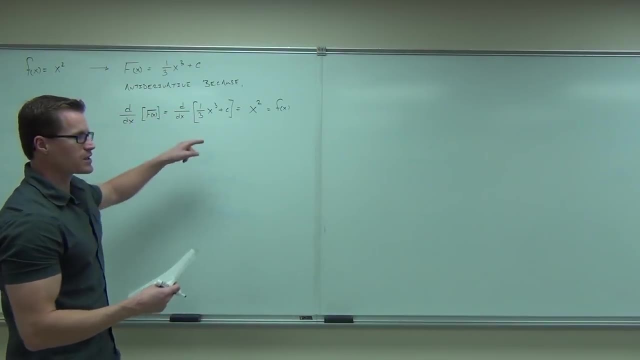 for which, when I take a derivative of it, it gives me my original function back. Did you understand that I'm going to go back to the last time? That's basically a last-time concept. Now the process of finding the antiderivative. 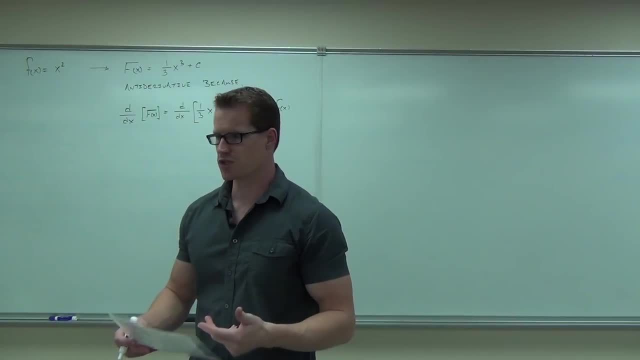 is also known as integration. So when you hear the word integration or find the integral, it means find the antiderivative. Does that make sense to you? So antiderivative and integral or anti-differentiation and integration synonymous. They mean the same thing. 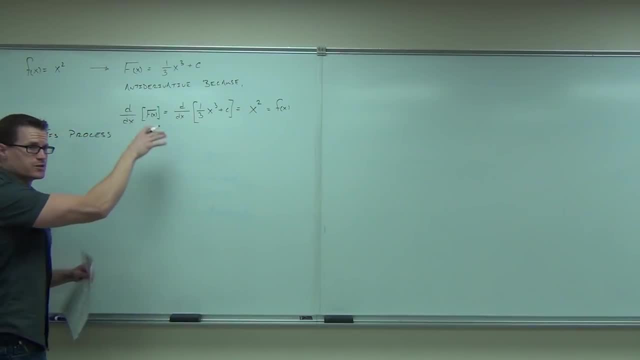 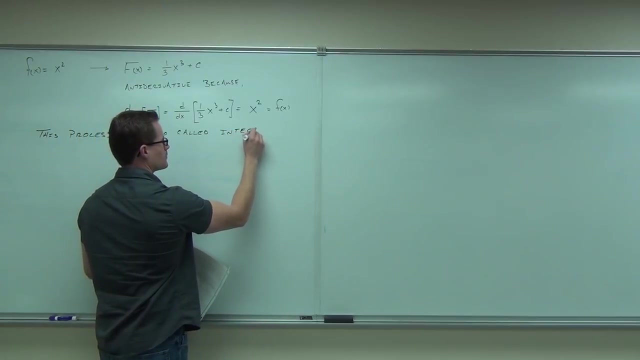 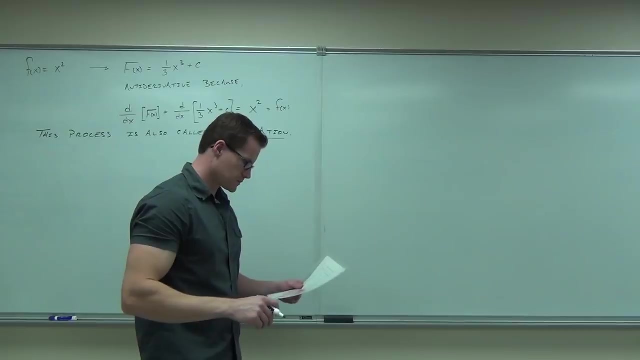 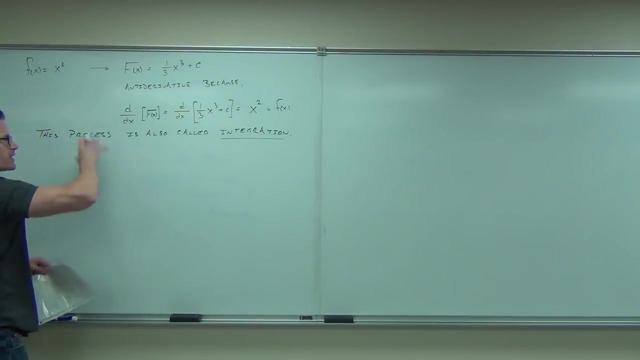 This process, and I mean the process of finding the antiderivative, is also called integration. Let me show you something. Here's basically our definition in a nutshell. This is really it. Our definition of an antiderivative is: if I take the derivative, 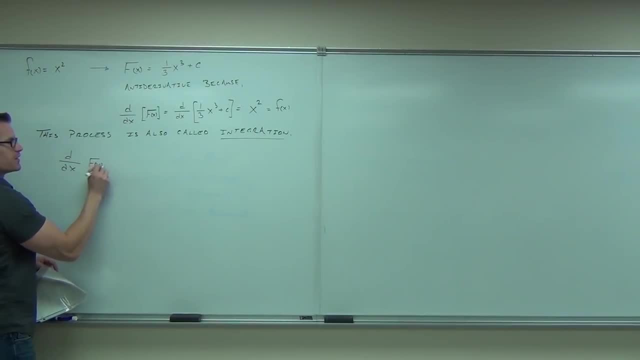 I even have it on the board already. if I take the derivative of my antiderivative, it gives me back my original function. Do you follow that? If I take the derivative of this thing, it must give me this thing. Do you follow? 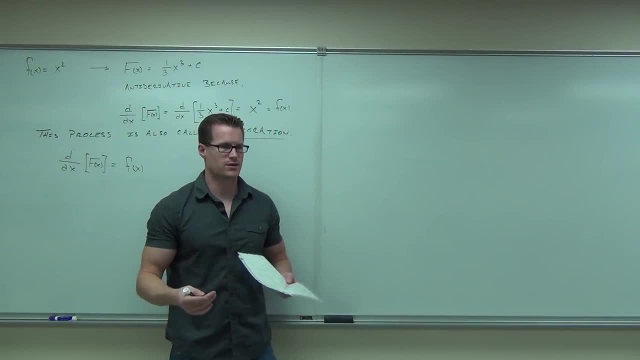 Okay, There's another way that we're going to write this. You see, this is kind of confusing, because this doesn't let us go from here to here, right? This basically just says: if I do this thing, it will give me this thing. 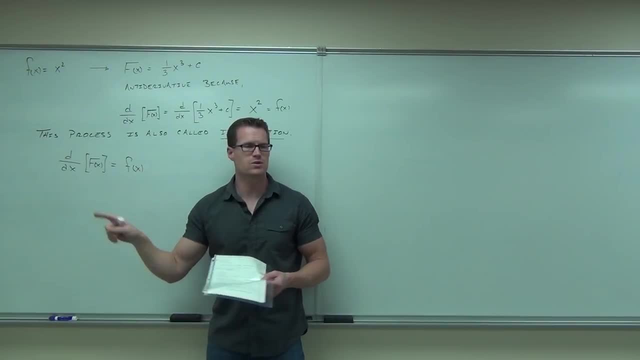 You follow. So we're going to write this a little bit differently. We're going to introduce a symbol called the integral. Remember, an integral means find the antiderivative or perform integration, which is to find the antiderivative. So this and what I'm about to write. 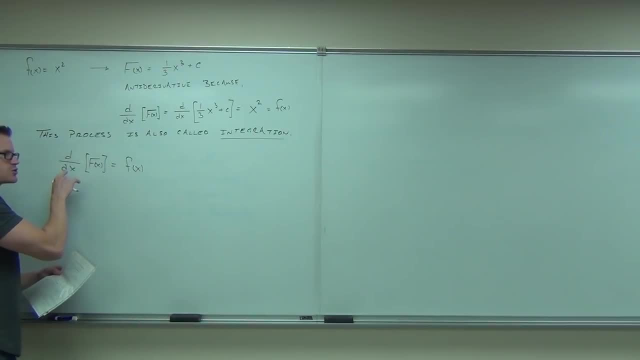 mean exactly the same thing. This says: if I take a derivative of the antiderivative, it gives my function. This says: if I find the integral of my function, it will give me my antiderivative plus C, Because we don't know the constant right. 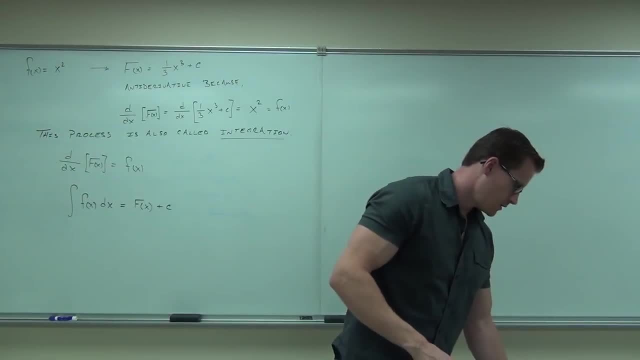 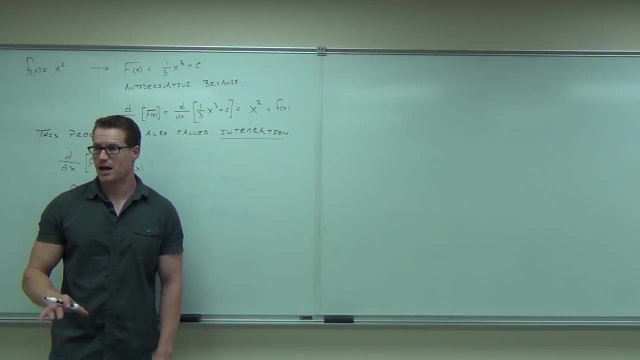 We talked about that already. It's a family of curves. By the way, is that C important, that constant? Yeah, that's two points on the test every time, So you have to have the C That represents. I don't know the exact. 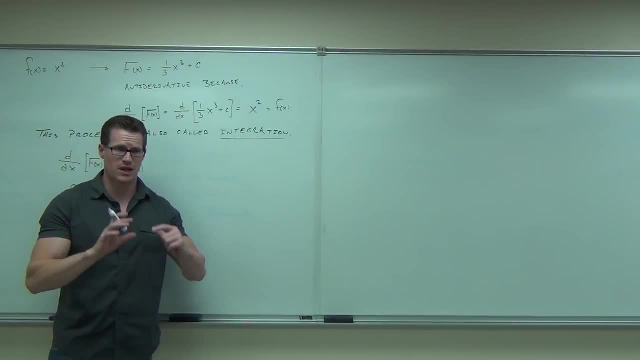 integral as far as the constant and it represents a family of curves for which I take a derivative and I get back my original. So this constant must be there And this right here is called your indefinite integral. I think I've referenced that before. 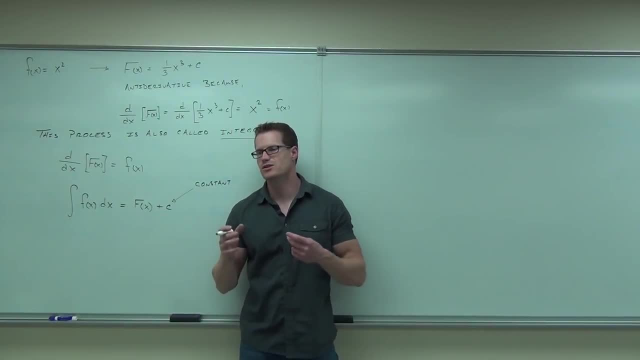 I said it's indefinite and indefinite integral, because you don't have any boundaries, You don't know where you're going. Basically, right now, all we're doing is finding the area function. It's very similar to this. You remember when I had you find derivatives. 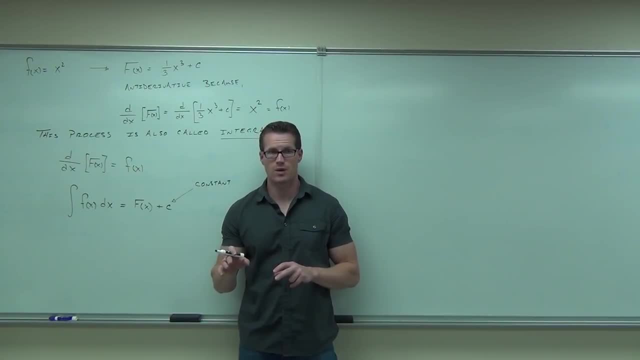 You ended with things in terms of x, right? So while that represented a slope, it wasn't an actual slope. until you plug a number in, Do you follow me? This is the same thing. This is going to represent an area, but it's not an actual area. 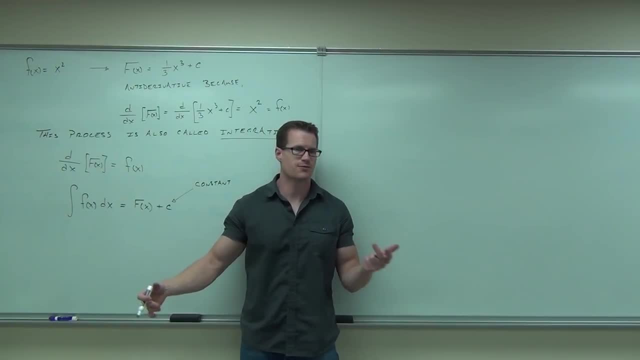 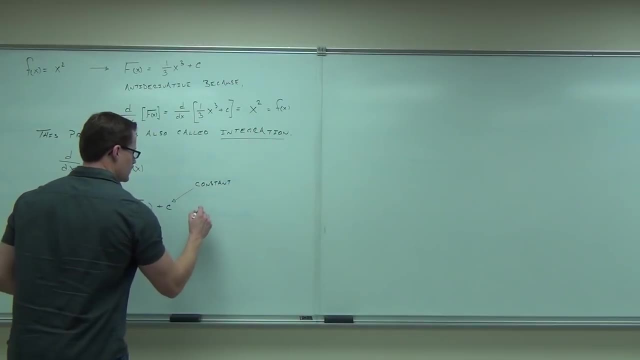 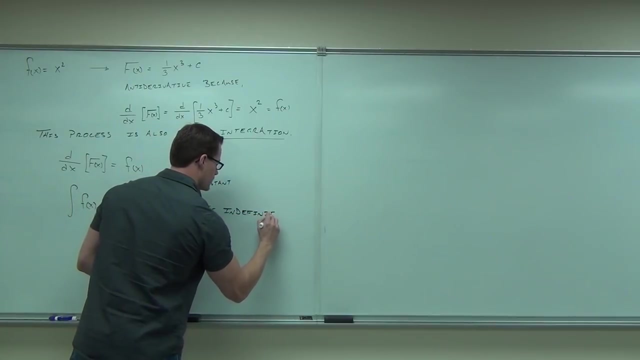 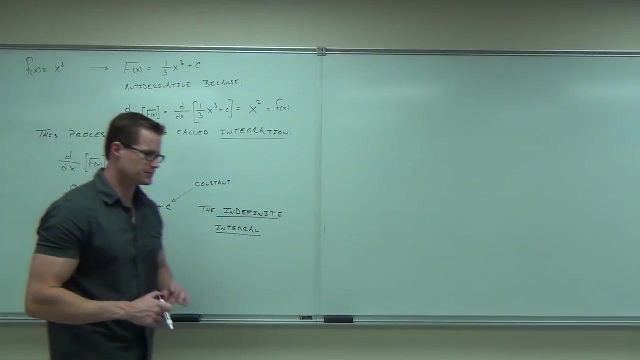 until you plug something into it, And that's why it's called indefinite and not definite. Definite would be: I'm able to plug numbers in and I get areas out. This is called the indefinite integral. The indefinite integral, The indefinite integral. 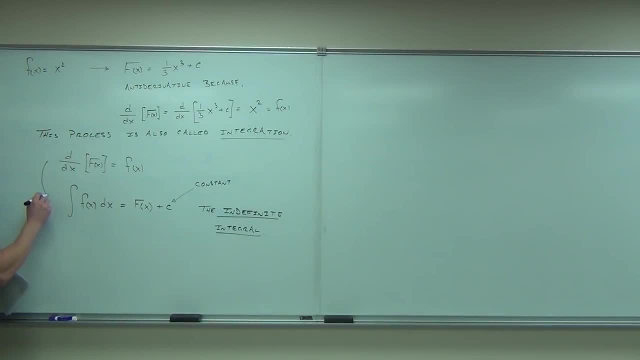 And these things say exactly the same thing: Interchangeable. This says: take a derivative of an antiderivative, you get the function. This says: find the integral of your function. What this says is this: It says: find the antiderivative to this. 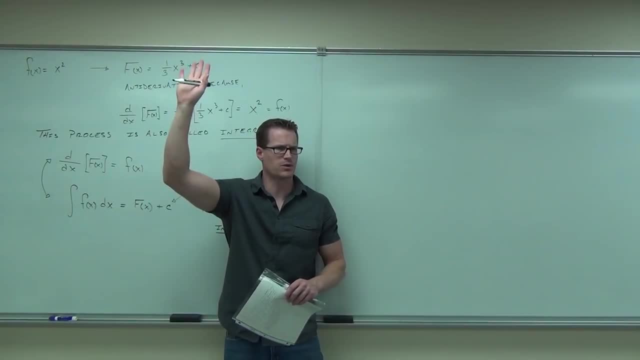 There it is. That's the whole idea. Do you understand the notation? we will do. What is the dx there? That's a good question. I'll get to that in just a second. That dx tells you what you're taking the integral with respect to. 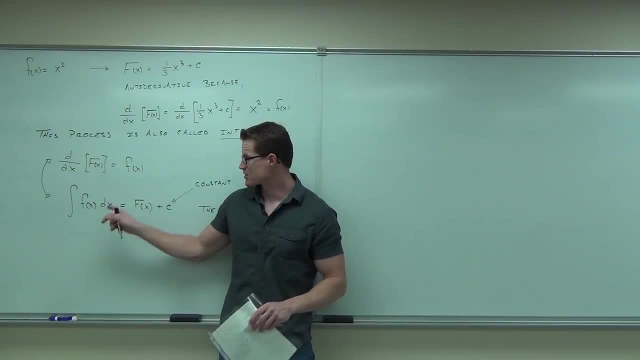 So what your variable has to be. So this dx right here says: I'm taking this with respect to x, So that variable has to be x. If it's not, we can't do it. Does that make sense? It's got to be there. 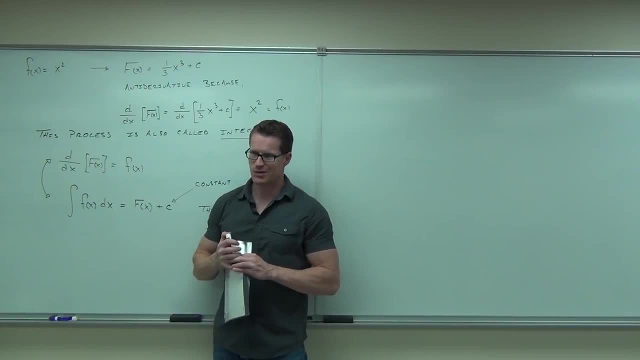 And we'll talk about this a little bit more as we go on and on. Basically, I want to get down to the names, the notation. What's that called? That's the integral symbol or integral. That's right. What this means is find the antiderivative. 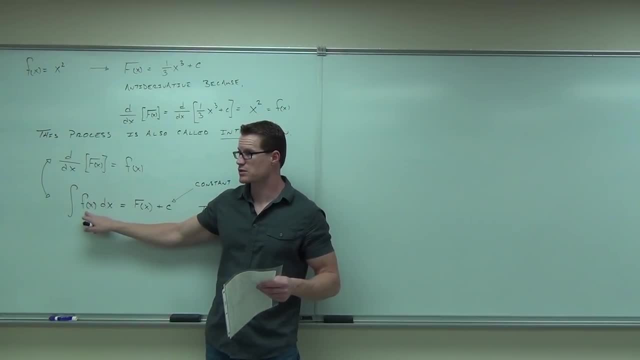 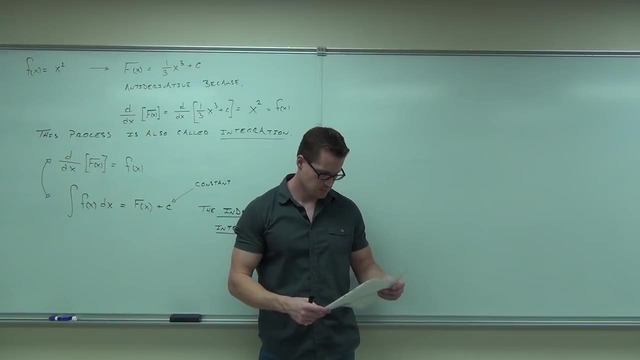 or undo this as if it were a derivative of something. So give me some function that I can take a derivative of and it will give me back what you started with. That's the whole idea right here. You okay with this so far. One note: this is also true. 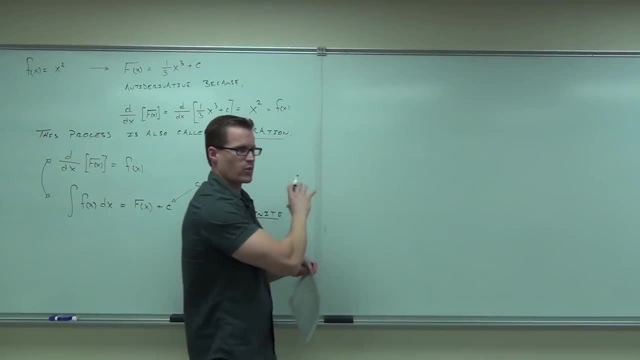 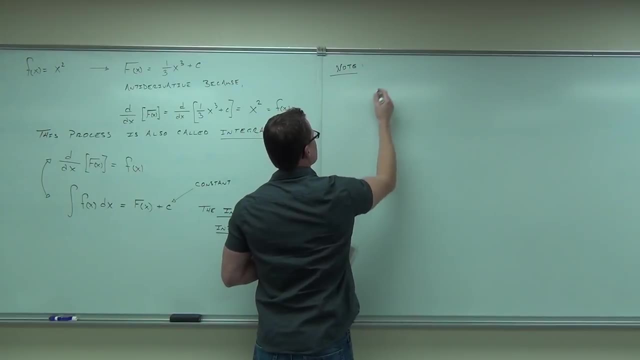 I hope this doesn't blow your mind, but I'm basically restating things a few different ways so that you see them a couple ways. Let's see if you can manage to do this. This is kind of critical thinking on a lower level. 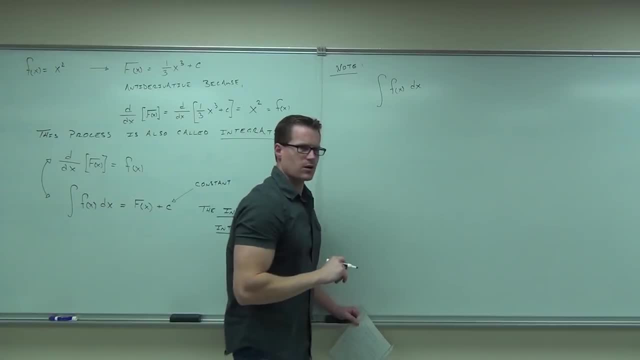 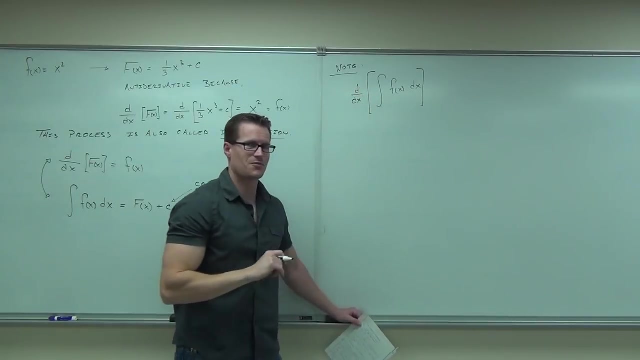 What's that stand for? Integral, Or what else? was it called Antiderivative? That's an antiderivative right. What would you suppose would happen if I took a derivative of the antiderivative? What do you think it's going to give me? 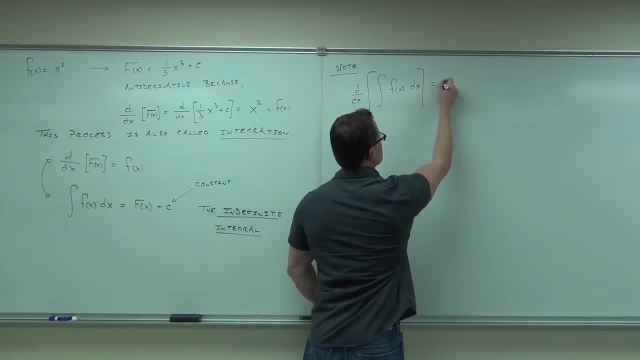 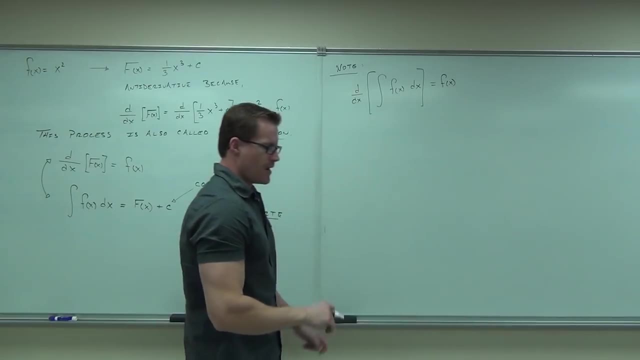 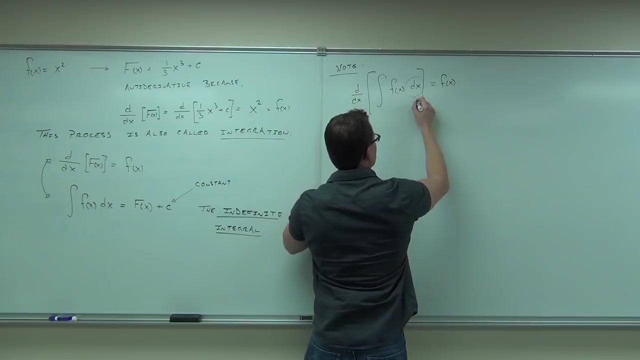 A basic function, A basic function F of x. This is true. That's a true statement as well. That dx- I'll make the note right here- that dx tells you what variable we are integrating with respect to. And this right here says: 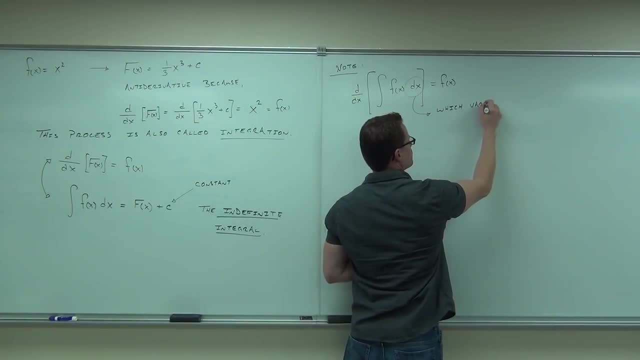 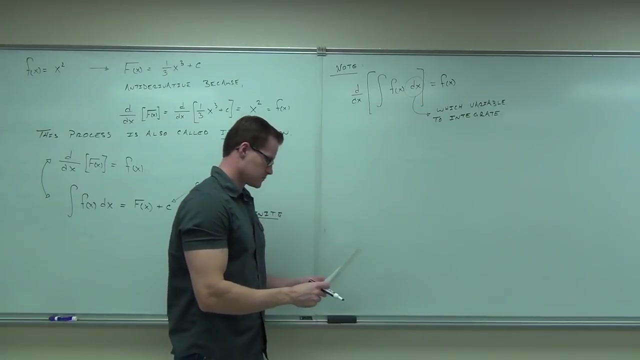 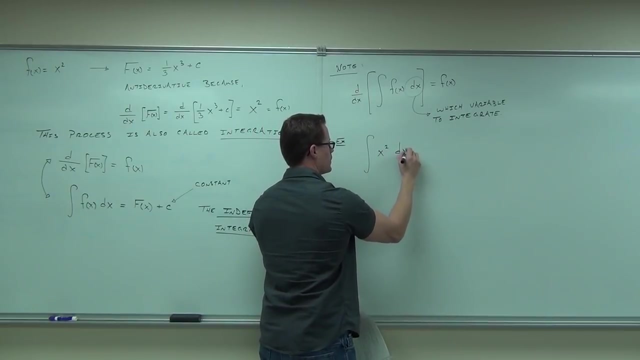 which variable to integrate, For instance. that's why, when we did this, now we can actually have symbols for it. Let's go ahead and try to do an example that we've had like probably five times, but just so you get the symbols down. 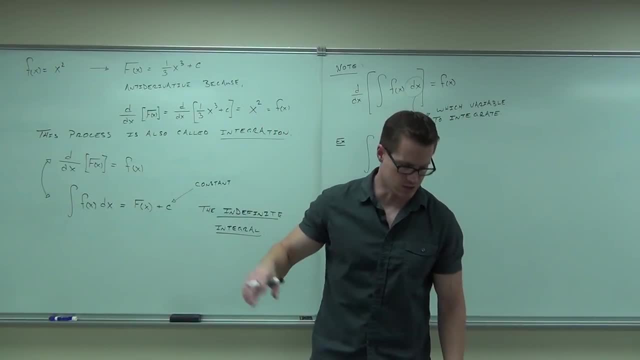 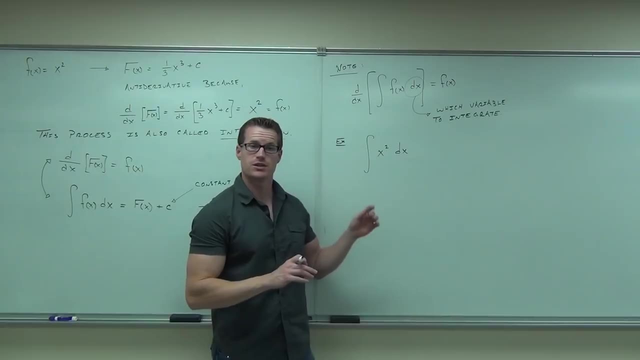 We've actually done this problem. I think we've done it. I've had it on the board several times, but we've actually done it twice. The integral of x squared dx says: I want you to find the antiderivative of this function. 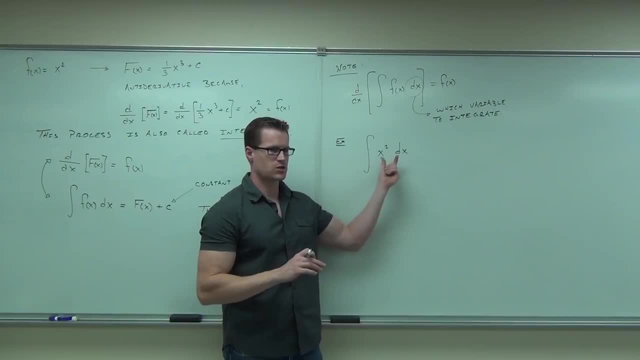 What's the function With respect to the variable x? That should match up. That has to match up for you to do it. You can't do it if it doesn't, at least not with our single variable calculus that we're doing. 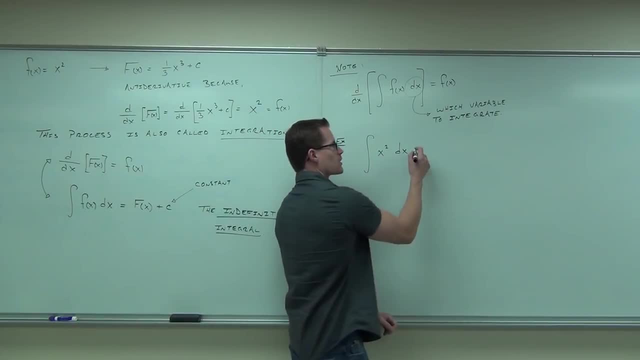 So if we're doing the integral of x squared dx, we're going to find the antiderivative of x squared. What's the antiderivative of x squared? Make sure we have that. Yeah, that's the one-third, Or x cubed over three is fine. 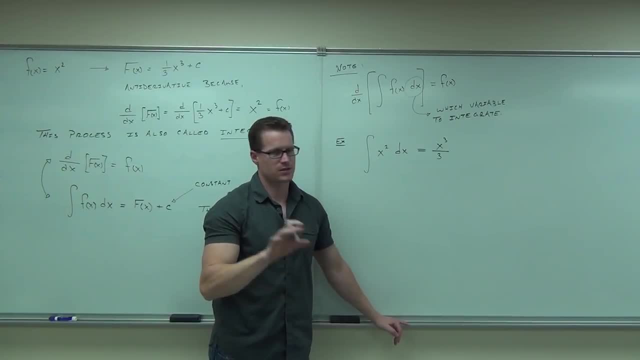 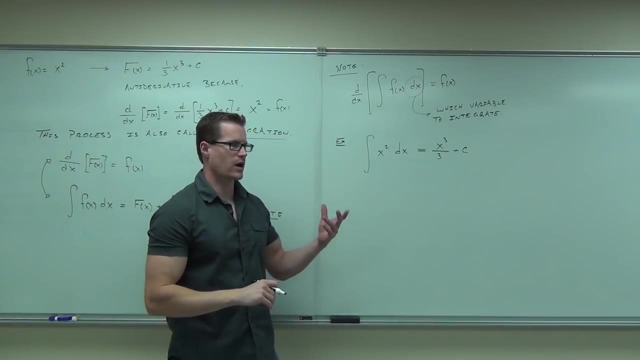 That doesn't quite do it yet. We also have to have- it's crucial, we've got to have that- plus c, Oh, minus c, right, And also minus c. Well, if you had minus c, you could write that as plus negative c right. 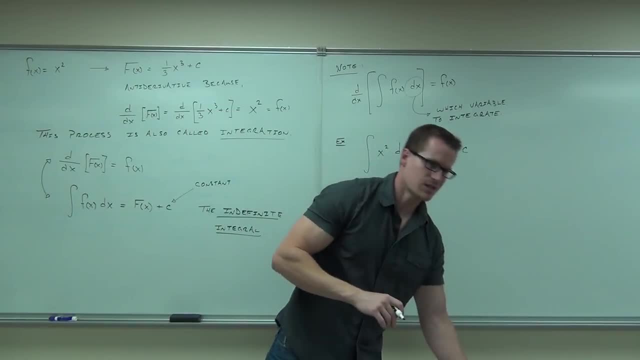 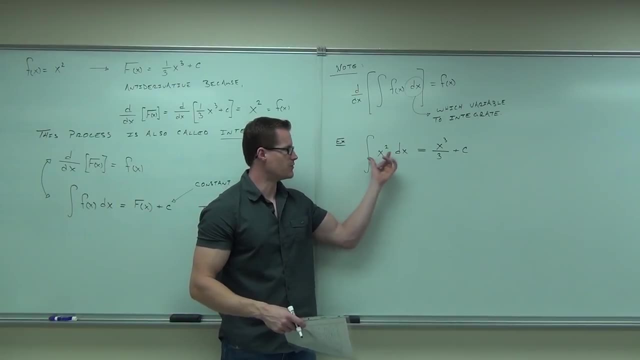 So you're always going to write plus c, So c is just some arbitrary constant that can stand for anything. That's how you do most of these problems right now. It says antiderivative of this function with respect to that variable, and we know how to do at least one of them, right. 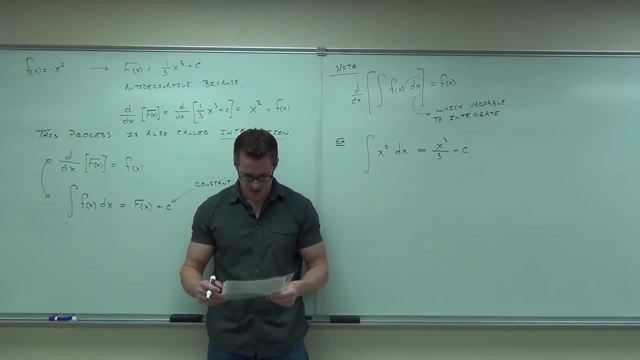 But we don't know how to do any other ones. So right now, what I'm going to do, I'm going to give you the basic integration table. Listen, If it doesn't fit in the basic integration table, you cannot do it right now. 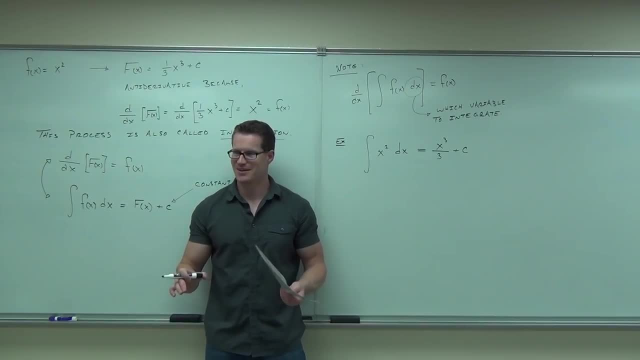 You can't create your own calculus here. If you do, you're better than Isaac Newton or Godfrey Leibniz. You invented this stuff way back in the day. That day was 1600s, So probably not going to happen. 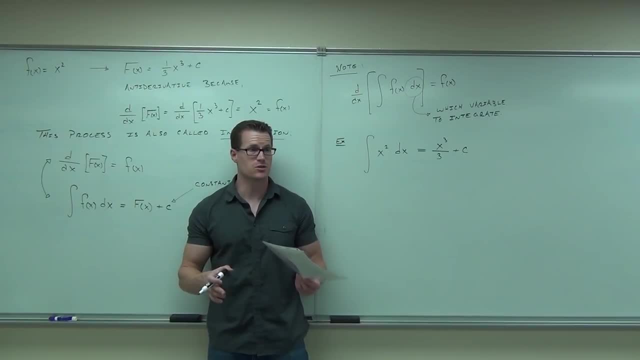 So don't invent this. Just follow the table. You do have to memorize it. I'm not going to put this on the board, but trust me, you will. The only tough ones are really the some of the trig ones that I'm going to give you right now. 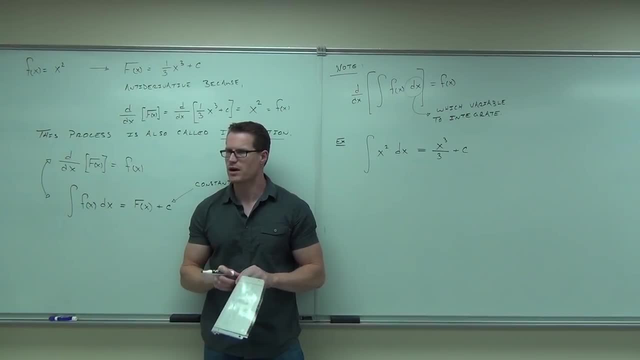 Some of the trig integrals are hard to memorize. But think of it this way: You already know the derivatives, right? We're just undoing them. So that's where all this stuff's going to come from. In fact, the table I'm about to give you. 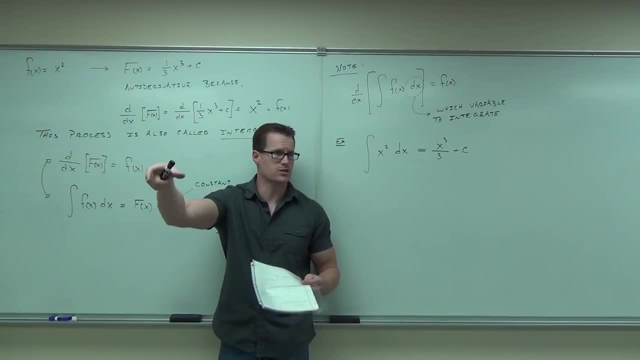 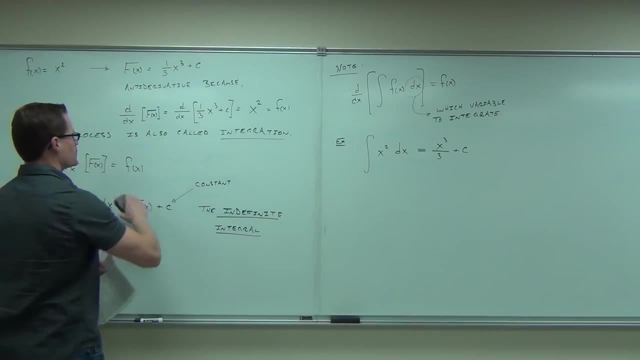 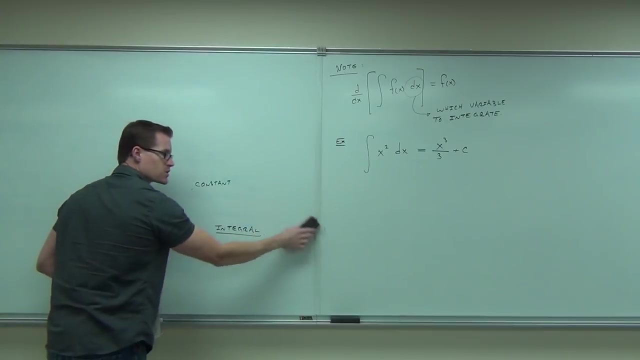 is going to have the derivative and then the integral that's associated with it. You ready for it? Okay, so This is called integration table. Yeah, basic integration table. You know there's a lot of them, There's a lot of integration tables. 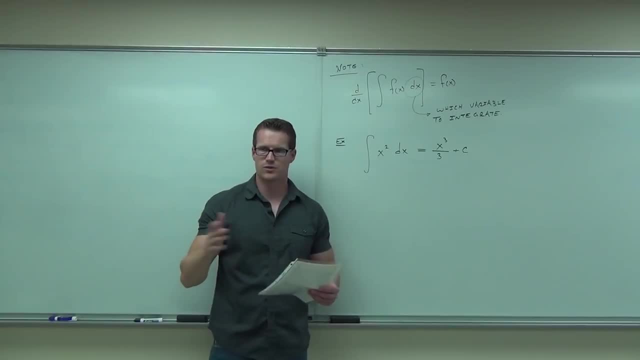 Yeah, most of the back of your book has just all those weird pages, right? What are all those The curvy things? Someone had fun just scribbling. No, no, no, Those are integrals and they mean something. 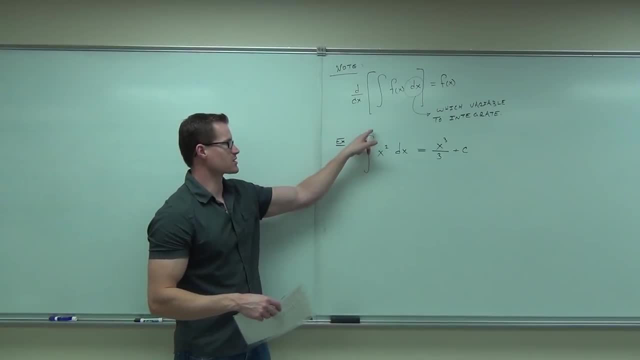 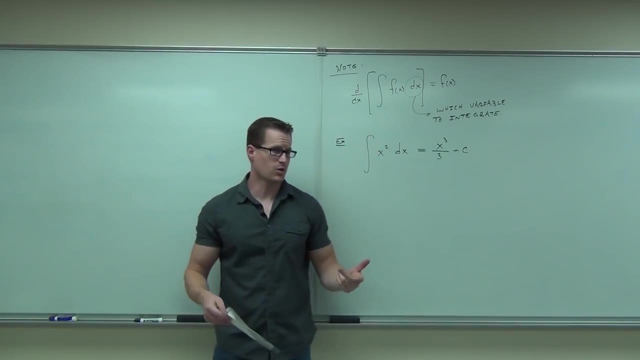 They all have different formulas, By the way, this long. what is that thing? It's integral, but what does it look like? What letter? It's an S? It's an S, and what we're going to come across in section 4.3. 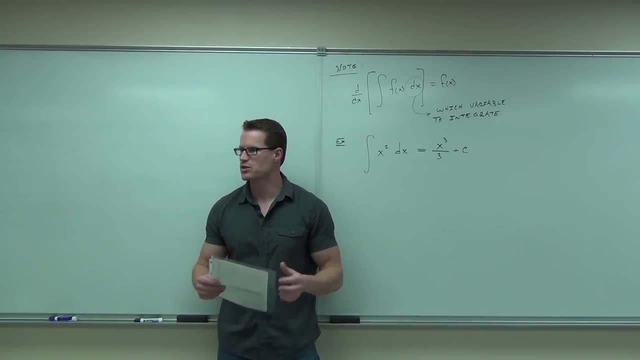 is that that's actually a sum. This is going to blow your mind, But remember how I told you that you can add all the rectangles together. That's what you're doing. It's a sum. It's a sum, A sum with a limit, basically. 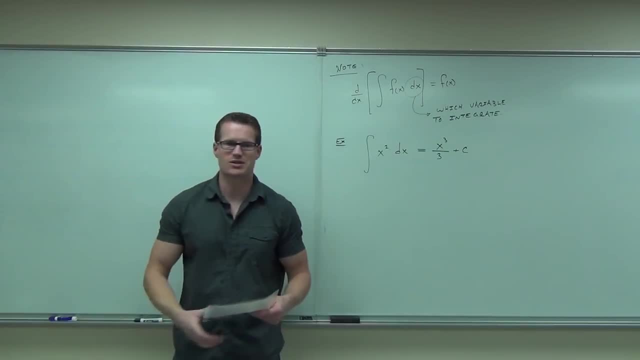 That's where the dx comes from. I'll show you all this. I'll make it very clear to you as we get there. but this is what we're doing. This is a way that you're adding all the infinite rectangles together and getting an area. 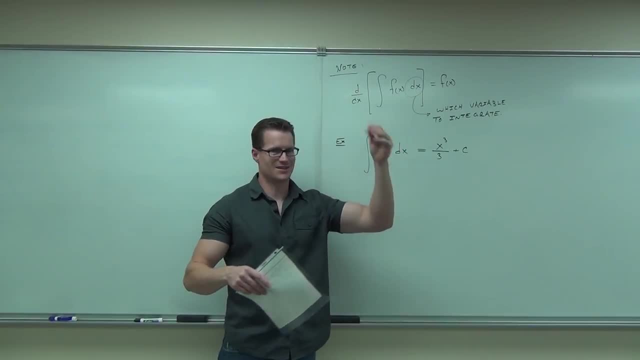 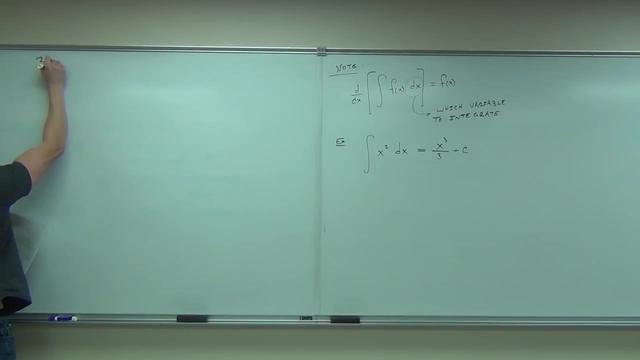 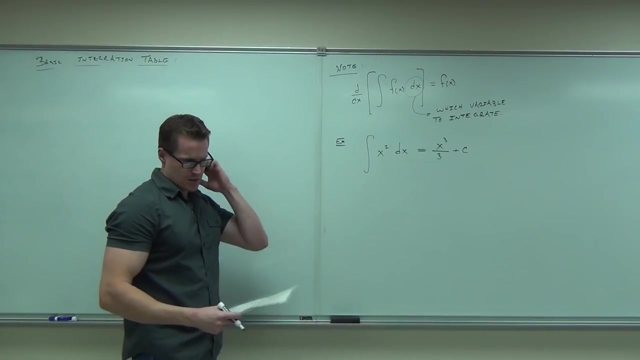 You get it Kind of cool, Kind of cool. It all makes sense in a little while. So basic integration table. So basic integration table. Like I said, I'm going to start you off with the derivatives and we're going to come up. 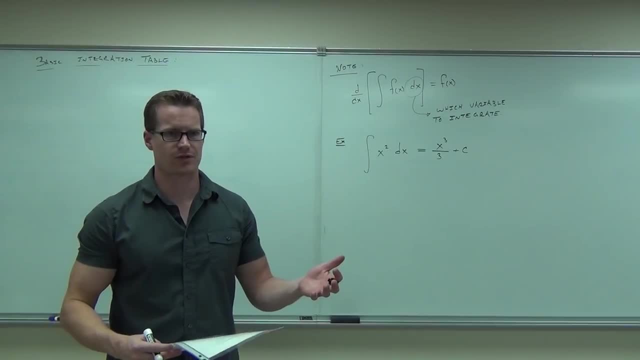 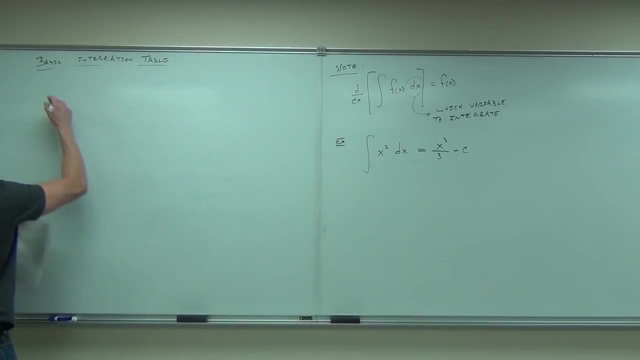 with the integrals that are correlators of them. because we know an integral undoes a derivative right. So if we know the derivative, we should be able to somehow manage to get an integral out of that. So let me ask you this: 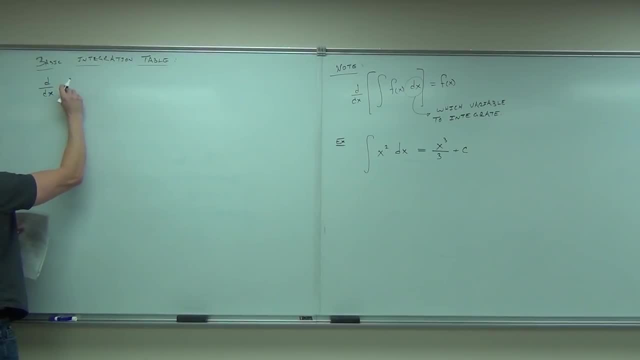 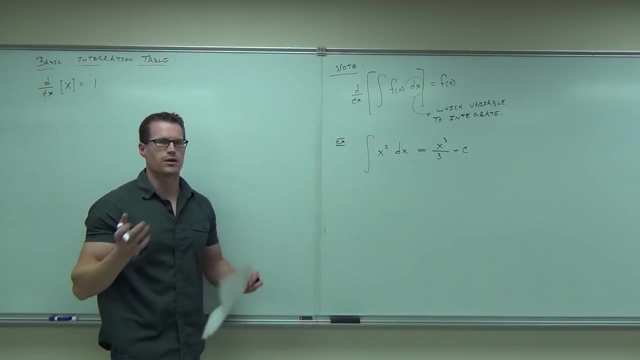 What's the derivative? We'll start very simply. What's the derivative of x with respect to x? One, Very good One. The derivative of x is simply one. The derivative of 2x would be two, 4x would be four. 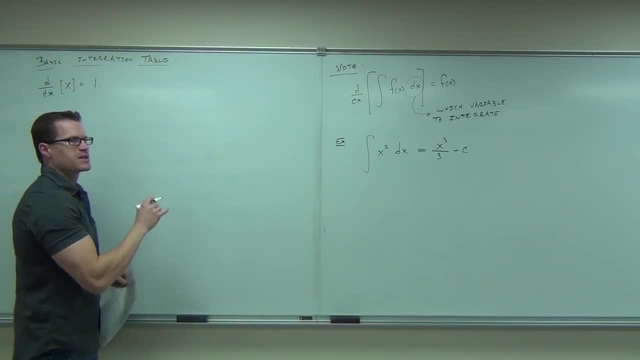 So the derivative of x is one. What that means is this: Hopefully you find out what I'm going to do here. What's the integral of x One? What do you think? If the derivative of x is one, the integral has to undo a derivative. 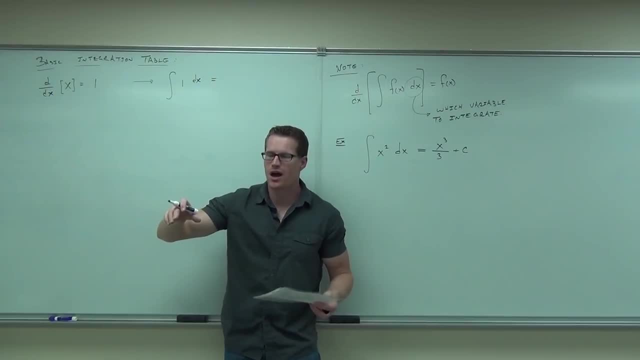 That's what this says here: A derivative undoes an integral and an integral undoes a derivative. So they have to go in reverse. They're like inverse operations, like division, multiplication, addition, subtraction, square root, square root- Same idea. 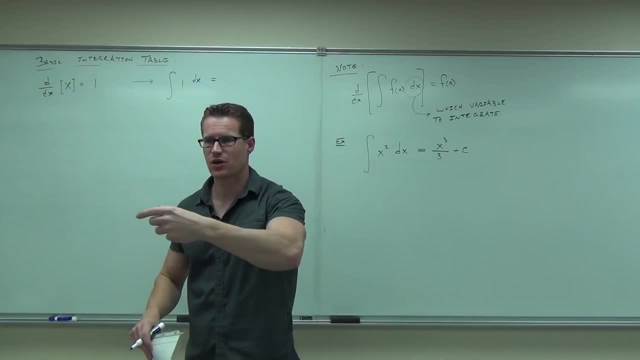 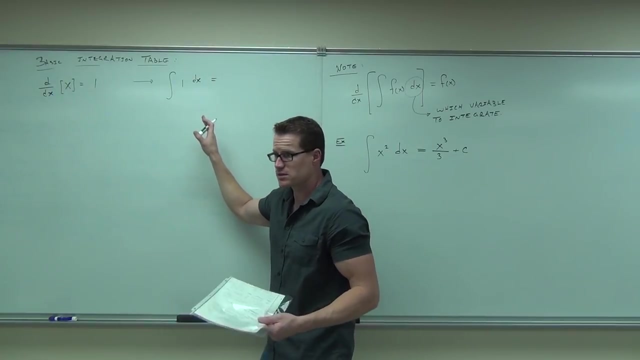 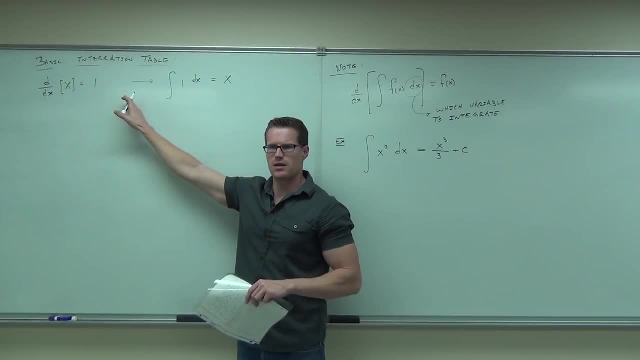 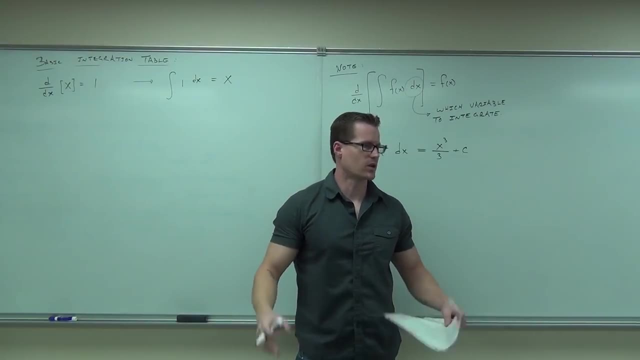 X, X, Sure, Why Think about it? You're undoing this like it's a derivative Right. That means, if you take a derivative of this thing, it should give you back. that Does it. Now we're missing something. 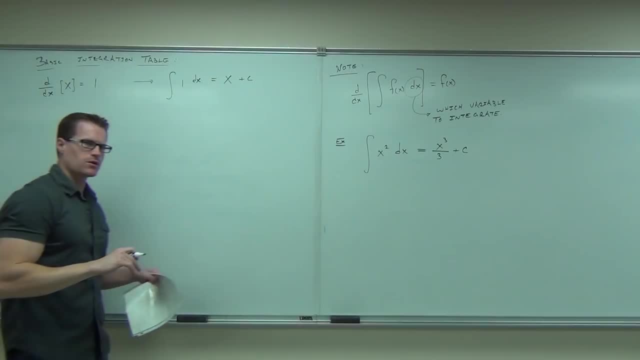 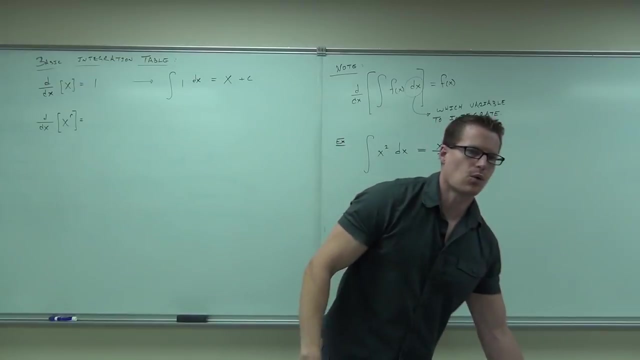 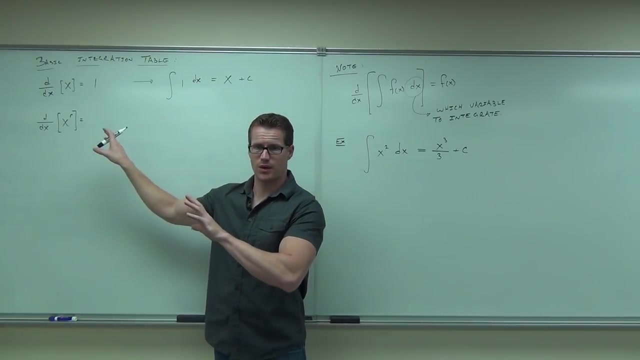 here. You OK with this so far? OK, What was the derivative of x to the r power? What do you do with that? What do you do? Add one to the. Okay, We add one to the. I'm sorry. 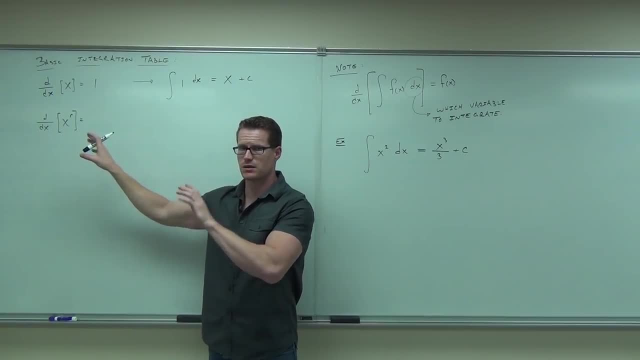 I'm talking about derivatives here. Derivatives, How do you take a derivative of that Minus r multiplied by r? Okay, Multiply it by r first and then subtract one from the r. Yes, That's cute, You'd have 3x squared. 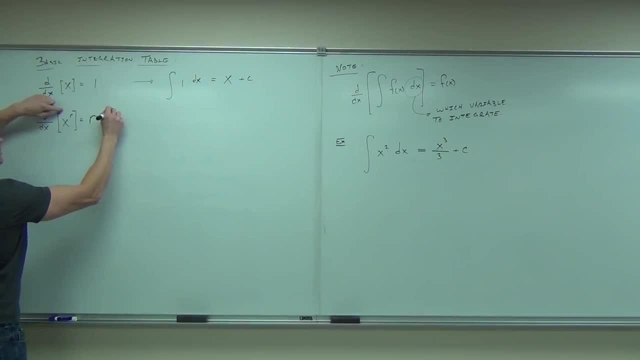 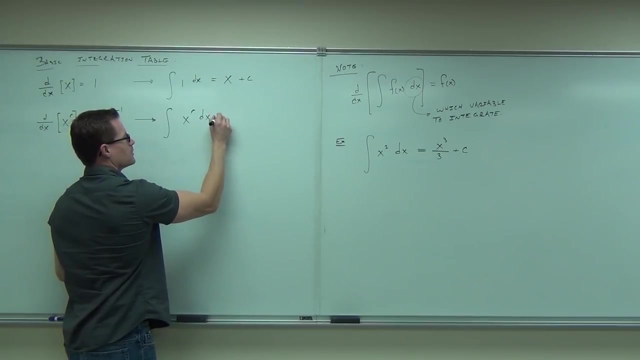 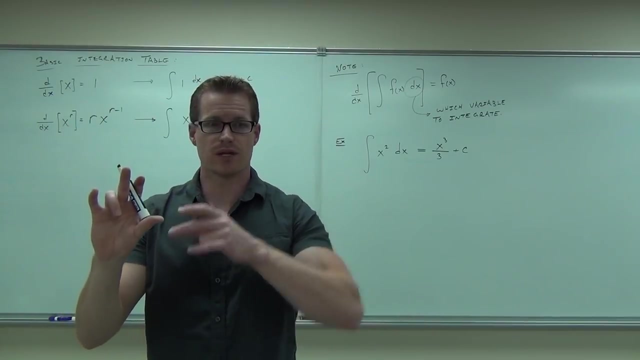 So this would be r x to the r minus 1.. You follow me on that. That means that an integral should go in completely the reverse order. So where we took a derivative, we multiplied and then we subtracted, right, The reverse order of that is: 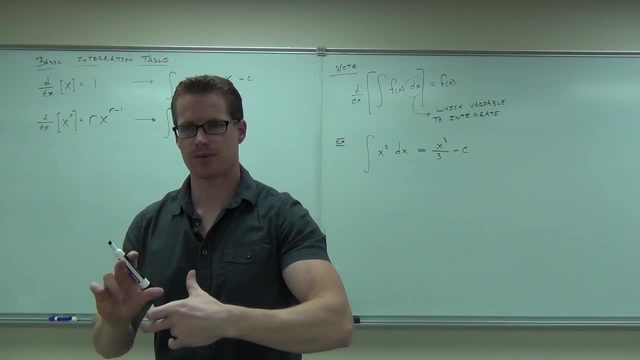 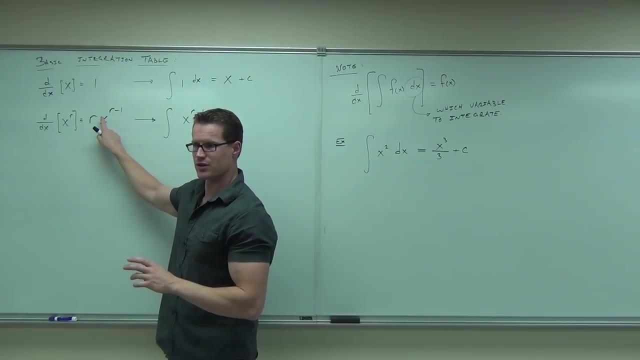 Add and then divide by that new number. Does that make sense to you? So here we multiplied first and then we subtracted For an integral that goes in reverse. that means you're going to add and then divide, Add and then divide. 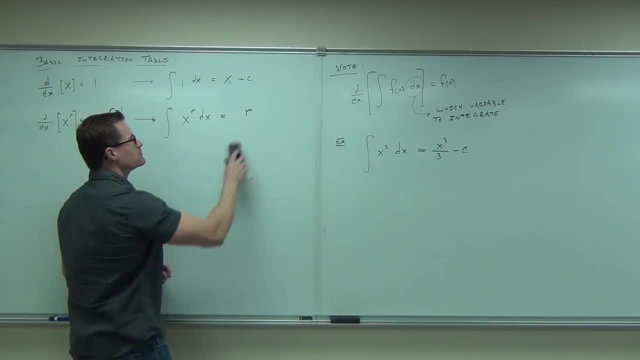 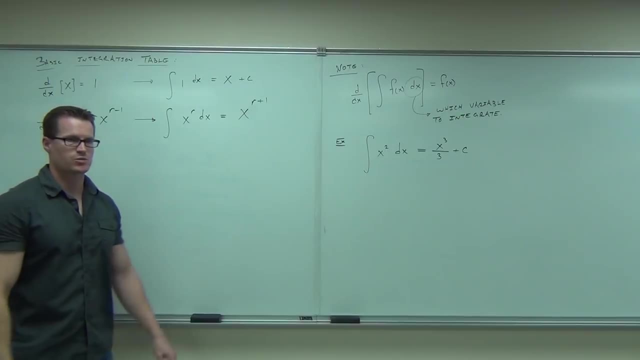 So our integral says: I'm going to take my x, I'm going to add 1 to that exponent, And what do you think? Am I going to divide by r? r minus 1? Or r plus 1?, r plus 1.. 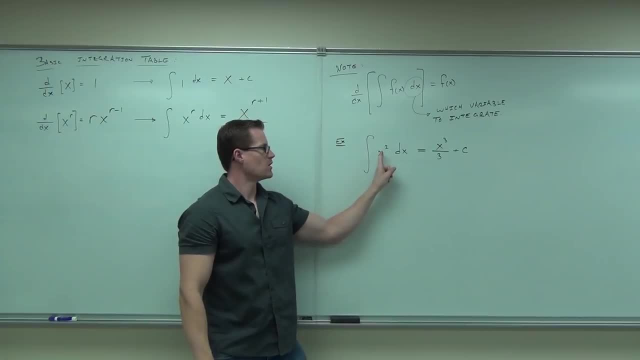 Look what you do here. Look, We actually did this right. How do you get from here to here? You add 1. But you don't divide by 2.. You divide by 3.. Why? Because when you take a derivative of it, the 3 has to match up with that to go away. 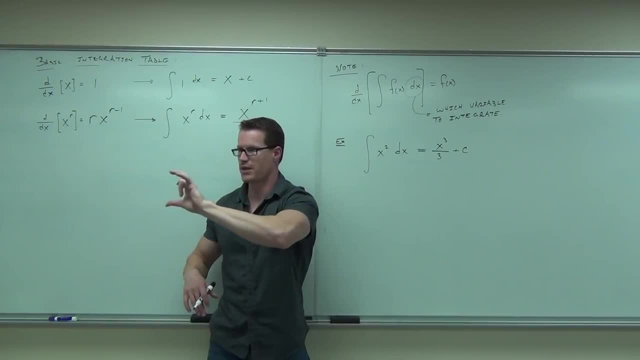 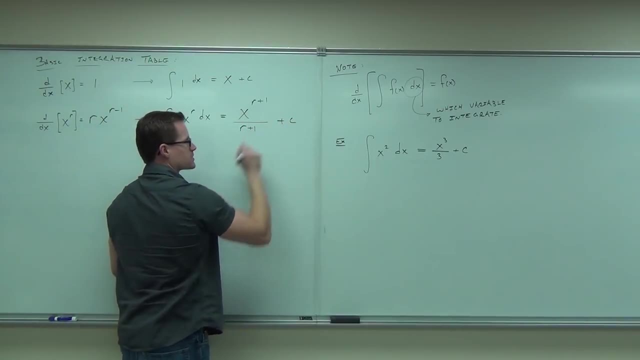 Right, So you're matching up the new exponent with that denominator. Do you follow that? So this isn't r. It's not r minus 1.. It's r plus 1.. Basically it says this in English: You add 1 to the exponent. 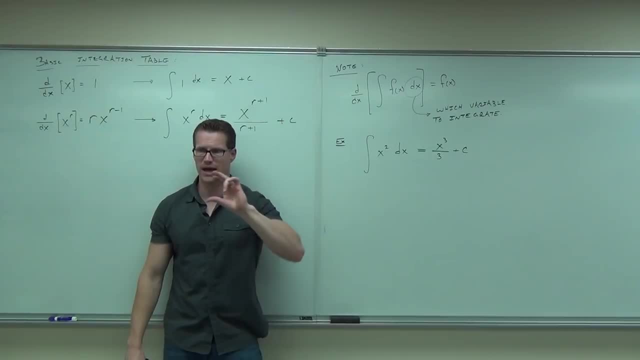 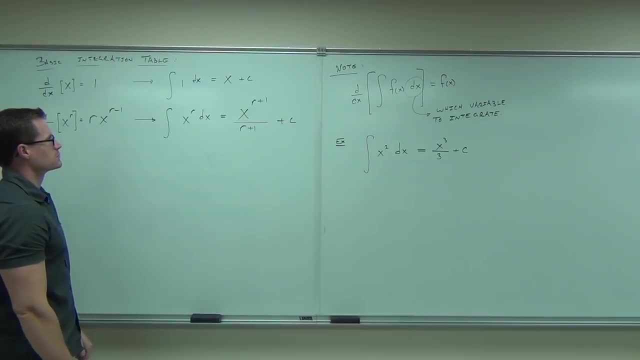 And divide by the new exponent. That's what that says in English. You add 1 to the exponent And divide by the new exponent. Shouldn't that be rx to the r minus 1?? This one, Yeah, Nope, No. 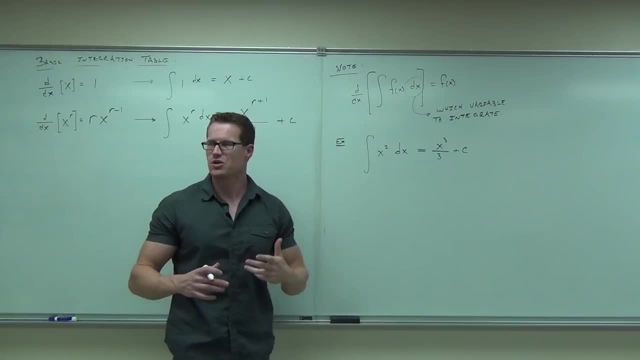 I'm kind of changing it here. I don't want to have this over here. I don't want to do the same thing. I'm just kind of using this as a template to what you're doing. You're doing this in reverse. 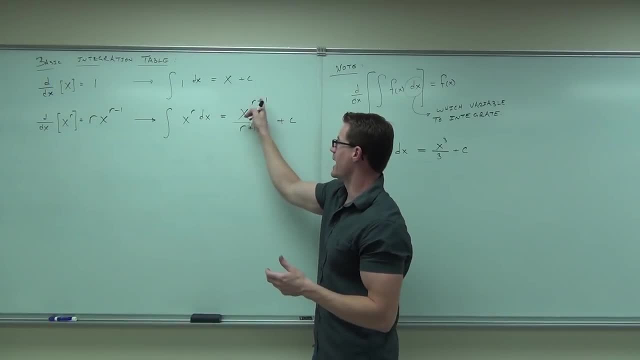 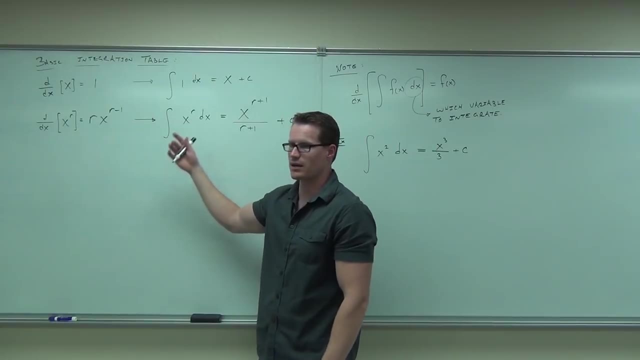 Right. So this says you're multiplying and subtracting. This says you're adding and dividing by the new exponent. I don't want to make it look exactly the same in this case. I know you can, But it's going to give you back x to the r. 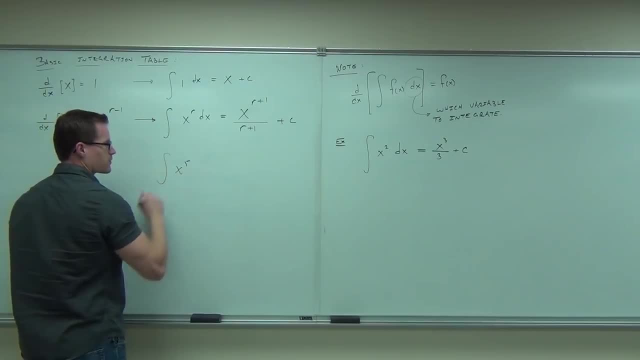 What I want to give you is things so you can do this. x to the fifth: Your integrals aren't always going to look like this. This would be way too easy. They're not always going to look like that. OK, Not going to do that. 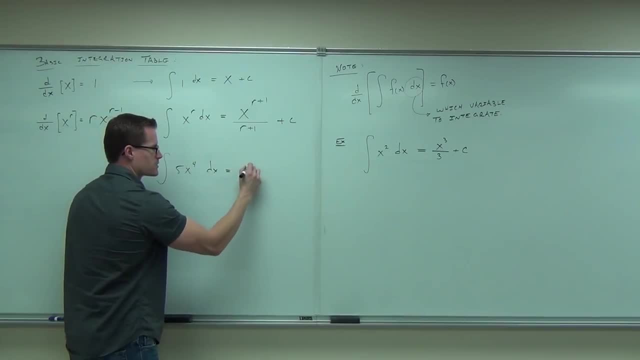 Yeah, no, This Sure, That would be x to the fifth, Easy. But what happens when you get something like this? Well then you have to know. I'm going to add one to that. I'm going to divide by the new exponent. 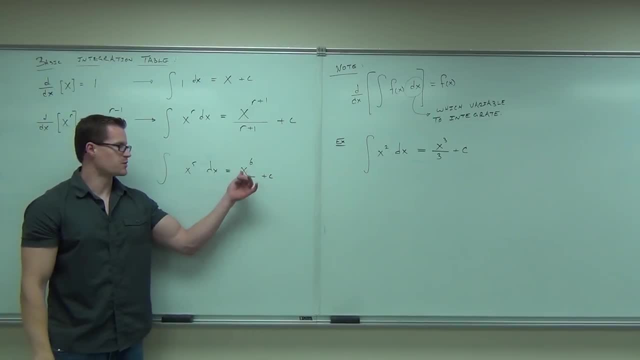 I'm going to put a, c And that's the correct thing. So when I take a derivative of this, it will give me back that. Does that make sense to you? That's the way this has to work. So yeah, I know that these don't match up exactly. 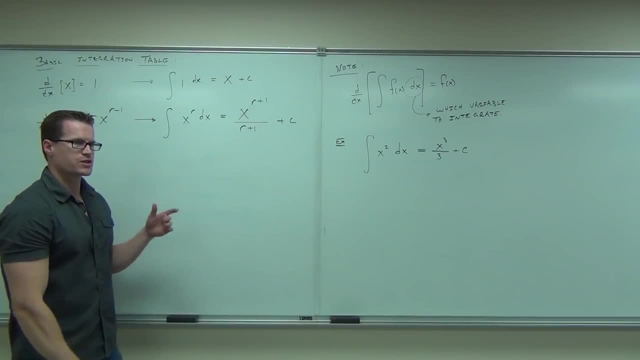 I know that Also. one more thing I do have to mention before we go any further. Notice that sometimes you're going to have this, It's not even going to have a one, Because really we don't even write ones most of the time in mathematics. 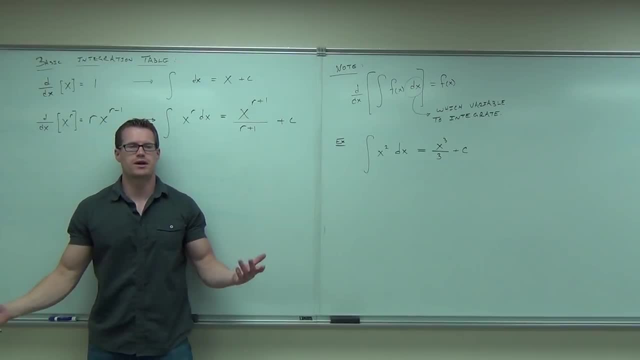 So if ever you see the integral dx, you go: what's in there? It's a one. It's a one Or integral of 2dx. Well, that would be 2x, But this that stands for the one. 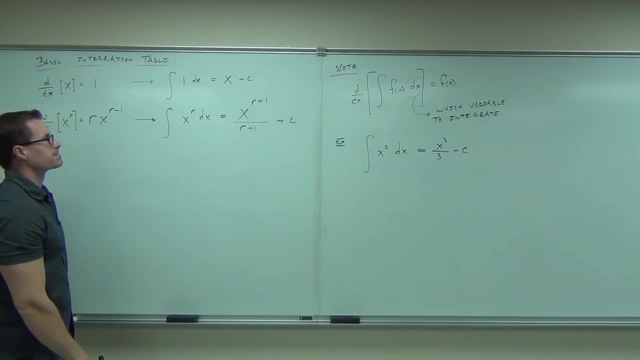 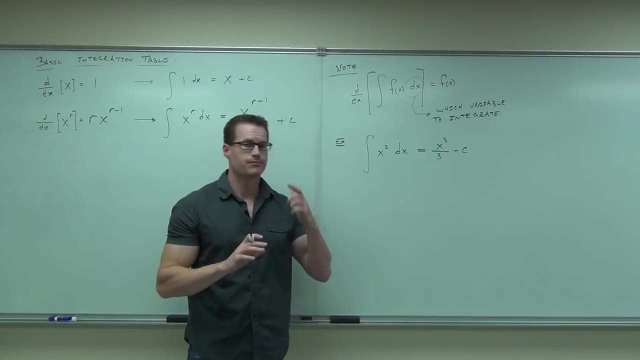 Between the function integrated and the dx. do you need parentheses there? You don't Not. unless you have a few terms. Do you have a polynomial in there or something You may or you may not? Oftentimes people don't put parentheses in there because it's implied that you're going from the integral to where it says dx. 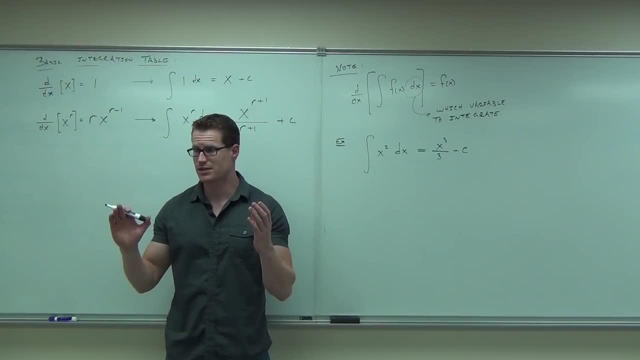 OK, Which, by the way, you must have the dx. If you don't have that dx, that says you're not even integrating anymore. You don't have respect of which variable You have to have. that It also closes off your integration. 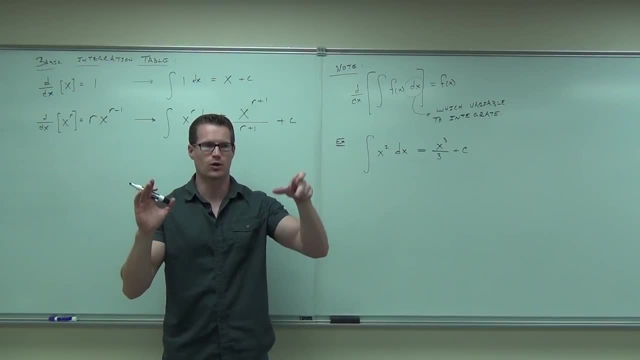 Does that make sense to you? It's kind of like the limit. Remember on the limits how you had to keep writing limit over and over, and, over and over again. If you didn't, I went. ha ha, ha, ha ha. 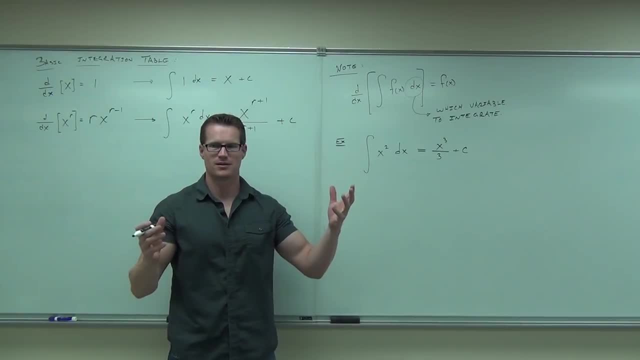 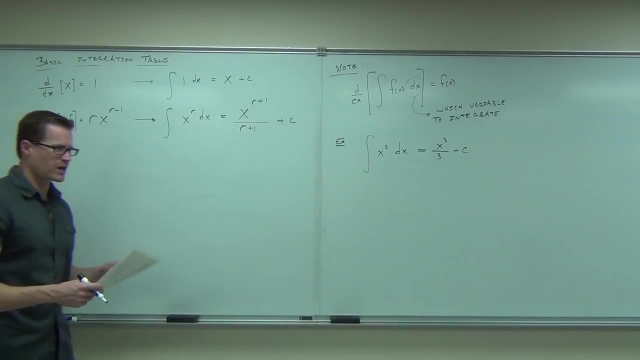 I laughed at you And I crossed out your papers And I burned them. Well, not really, But you had to have it. It's a must, because that's the same idea. Are you OK with these? so far? Some of you still don't like this. 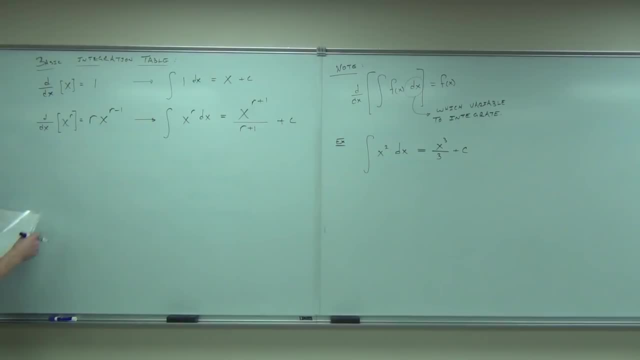 I know You're not used to it. If you don't like this, you're going to hate me on the next few, Not this one. That's too bad. Can you tell me what's the derivative of sine? Yes, very good. 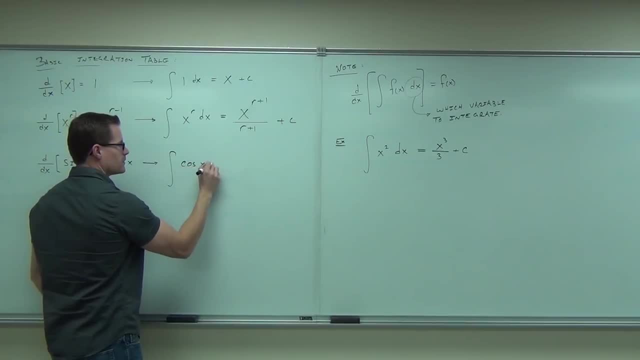 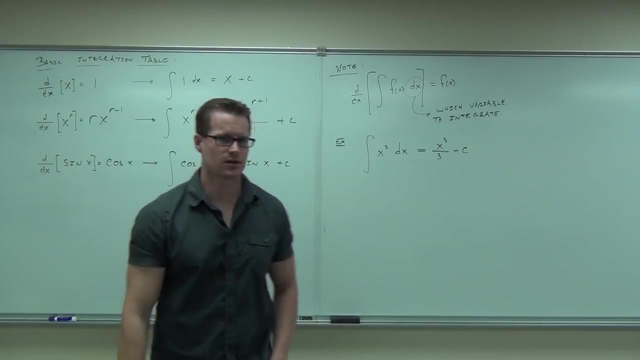 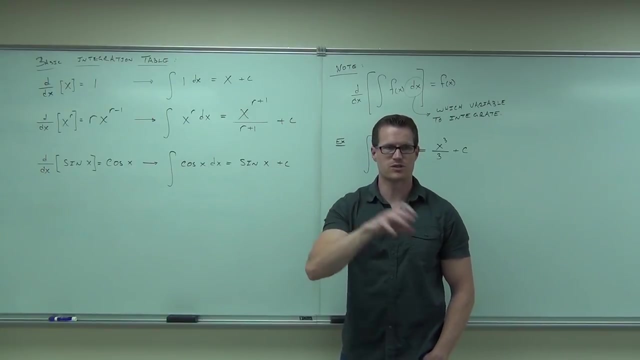 With that in mind, what's the integral of cosine? Sine x plus c. Sine x plus c- good, Very good. Do you feel OK with the integral of cosine? It's nice to think of these, as I'm looking for the reverse of a derivative. 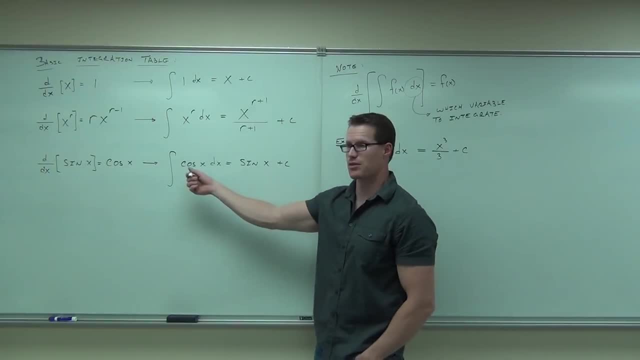 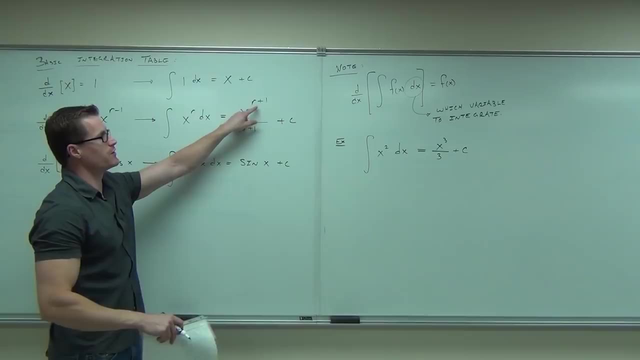 I'm looking for something that when I take a derivative of it, it gives me back that thing. Do you follow? That's what you're trying to do. The reason why we have it this way is because if you take a derivative of this thing, you bring down r plus 1.. 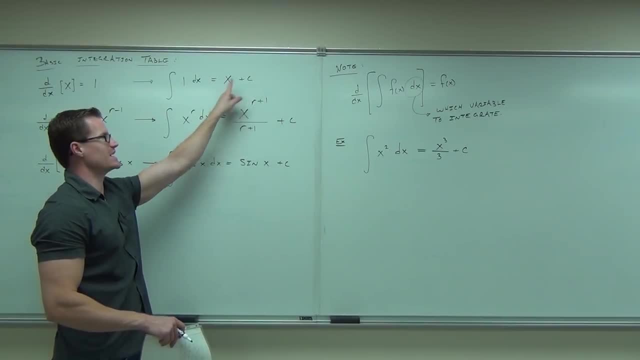 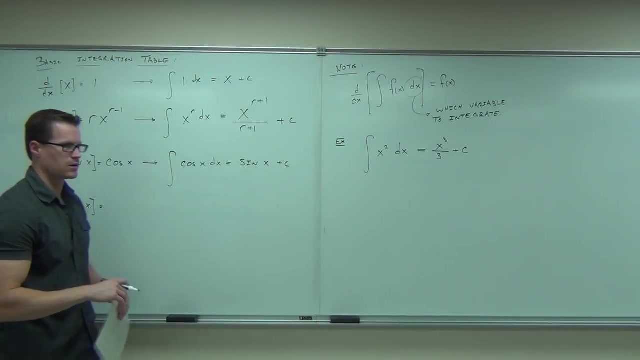 Those cross out. You subtract 1 from the r plus 1 and you get r. That's why we have it written that way. How about some more? We've got about five more to do. Please don't freak out with this, but I'm going to do this a little differently. 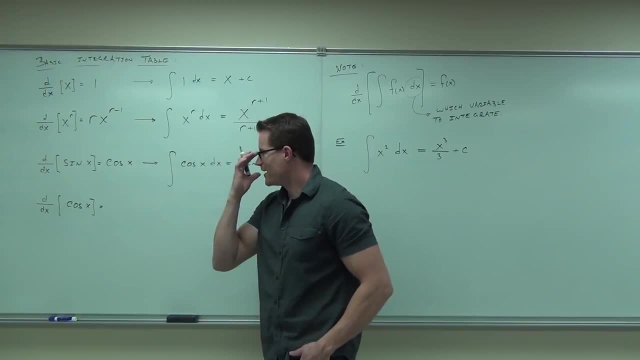 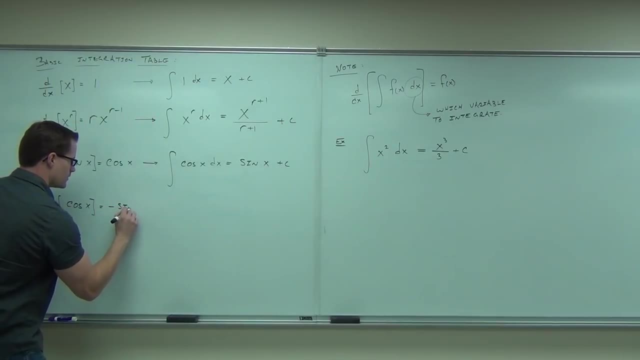 I told her not to freak out. The derivative of cosine. what's the derivative of cosine Negative sine? Now stop, Stop. I'm going to change this Because you know what we don't want to do. We don't want to have integrals of weird things. 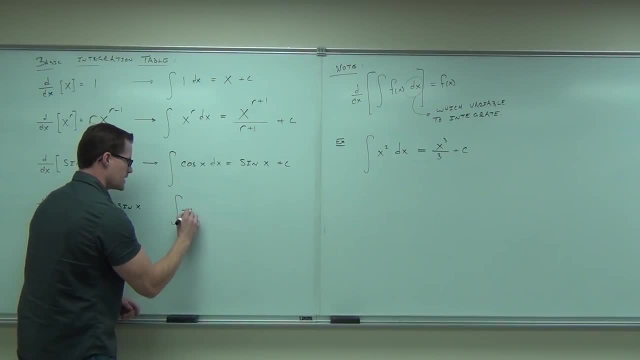 I don't want to know what the integral of negative sine x is, Because are you going to see negative sine x? No, probably not. You're going to see things like sine x, Do you get it? So I'm trying to make this thing into the thing that I have over here. 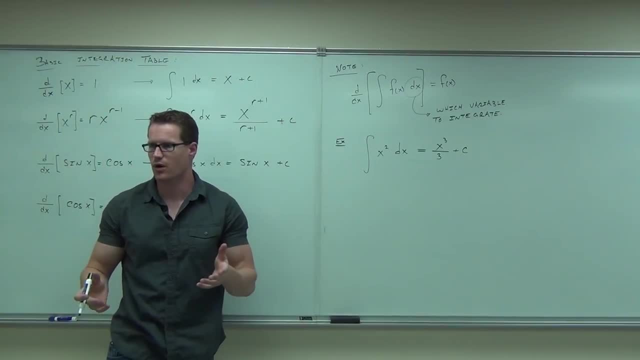 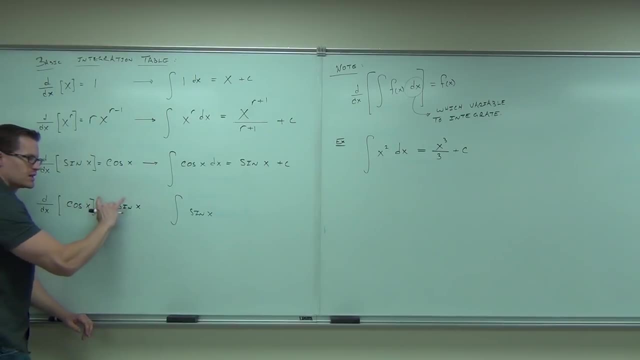 The only exception is that one. We don't write the minus 1.. We have it in terms of r, so you see it more clearly. But this, If this gives you negative, if the derivative of cosine gives you negative sine, what's the derivative of negative cosine give you? 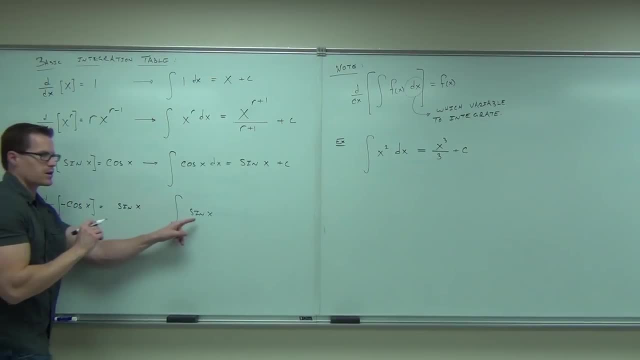 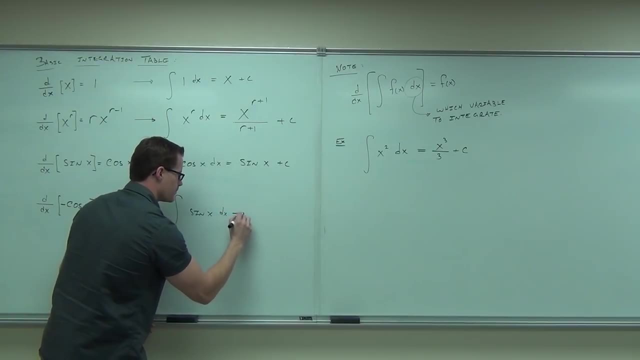 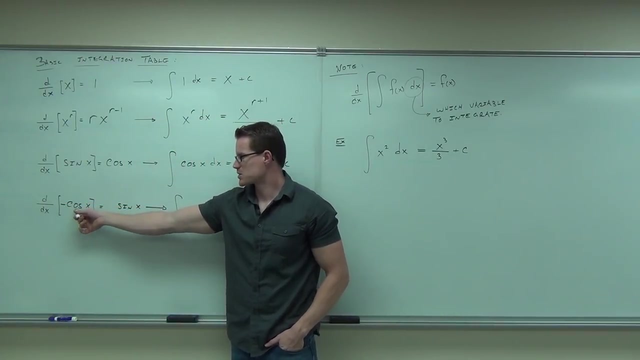 Sine, Sine, Do you get me? That's what I want here. I don't want to know the integral of negative sine, I want the integral of sine. That's why I changed that. Okay, You agreed that the derivative of negative cosine was positive sine. 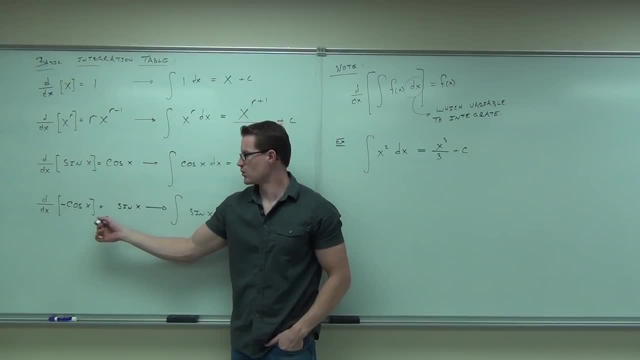 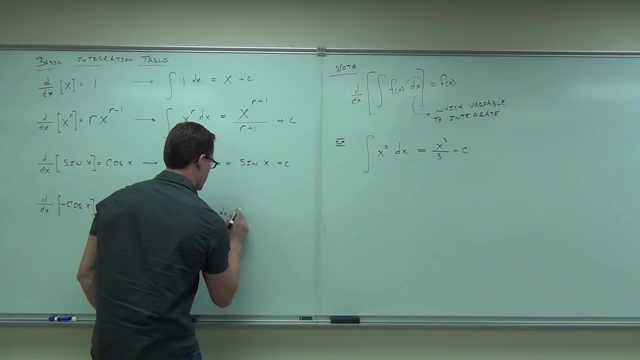 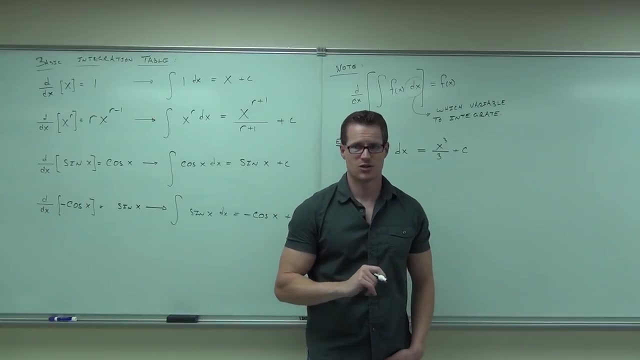 You agree to that? Yes, So what's the integral of sine Negative cosine, Negative cosine- Are these going to take some practice to memorize? You betcha, You betcha, You're going to reverse up derivatives- The opposite. 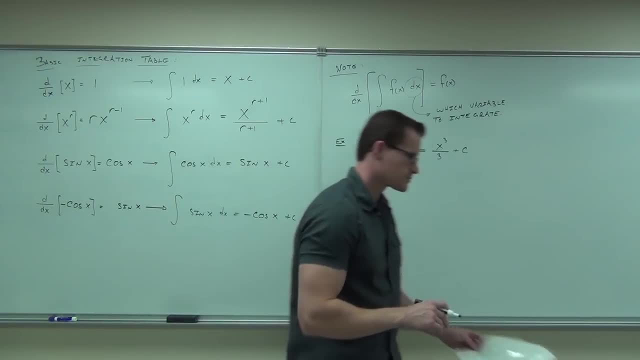 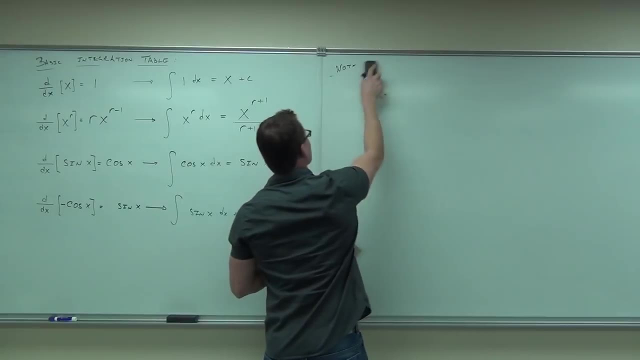 There's no such thing Backwards, No, No, You're lucky. There's no such thing as that. There's worse things, Oh no. Then where do we get lucky at? You don't learn in this class, That's next semester. 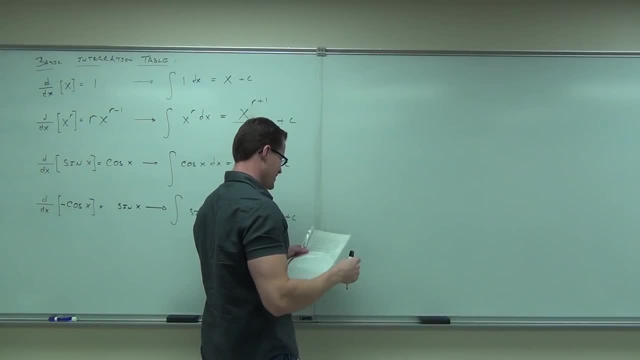 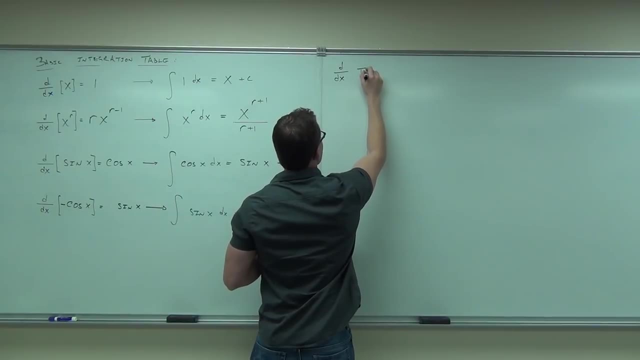 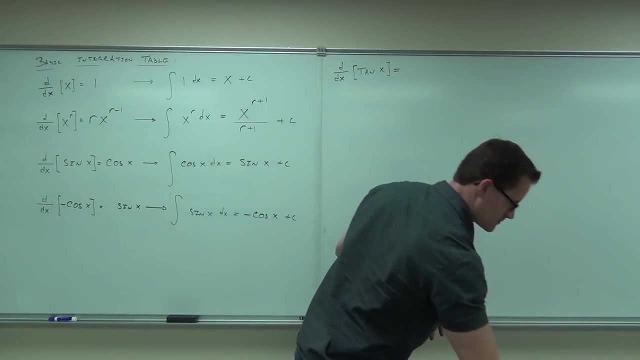 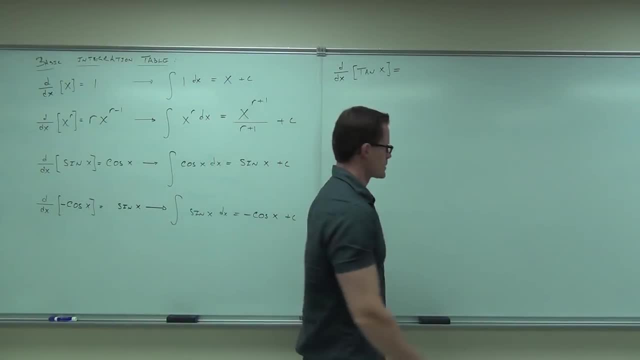 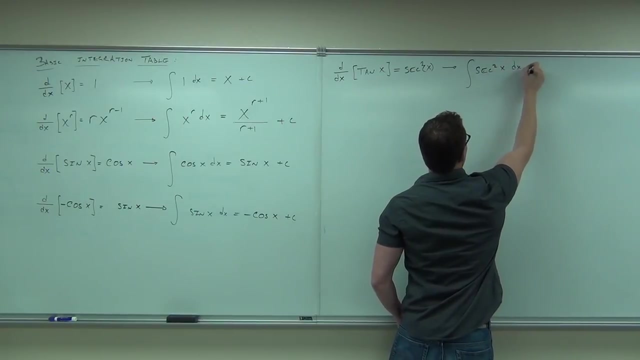 Okay, so derivative of tan x. What's a derivative of tan x? Secant squared x. Okay, This would be pretty painless. I mean painless. Now, this is pretty easy. That means what's the integral of secant squared x? 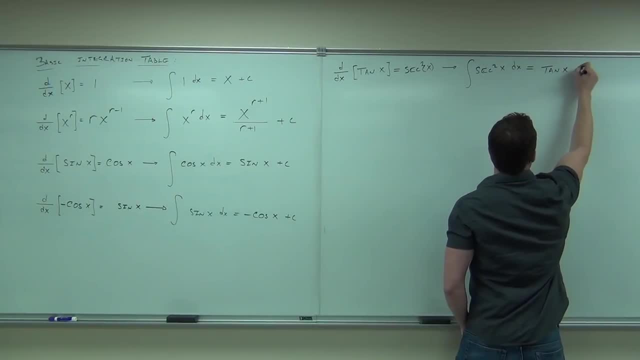 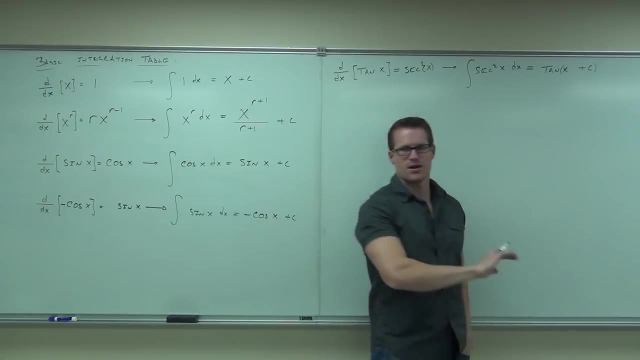 Tan x. I like the plus C. I heard it plus C, By the way. look at the board here real quick. Is it plus C like this? It's actually plus C like this. okay, Whatever the angle is. and then the plus C. 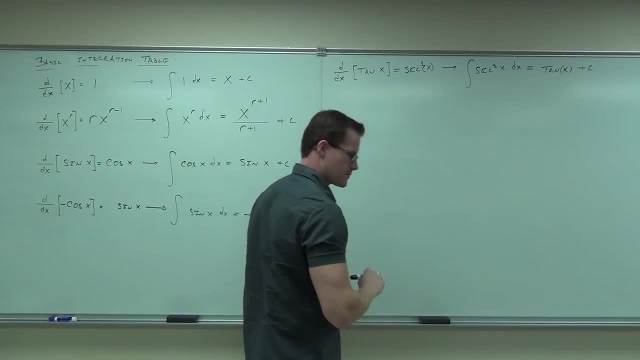 is the very, very end. Okay, three more. Well, let's see if you remember this one. Do you remember- and I'm going to change this, so don't get too excited yet- The derivative of cotangent Negative cosecant. 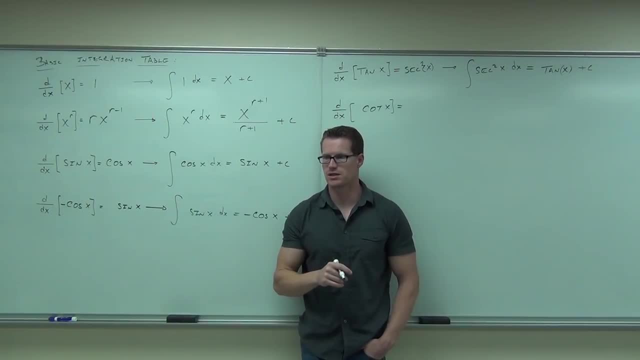 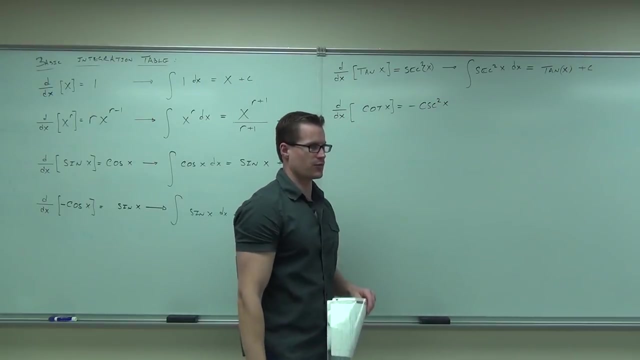 Negative cosecant. Yes, negative cosecant. If tangent is secant, cotangent is cosecant Square root With a negative, With a negative, With a negative. Do you know what I'm going to do? I'll bet you can see it. 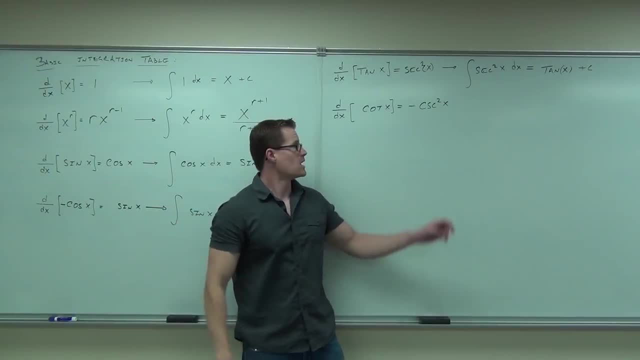 It's the same thing I'm going to do over here. All right, same thing I did over here. If I have cotangent, the derivative of cotangent gives me negative cosecant. what I want this to be is positive cosecant. 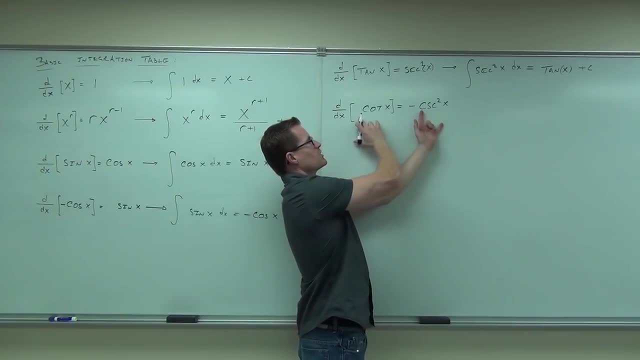 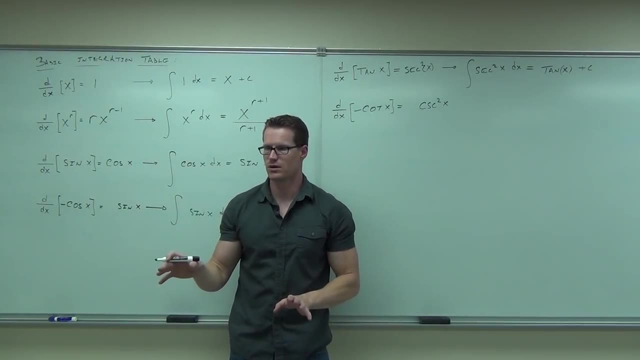 So look what I can do. I can say: okay, if cotangent gives me negative cosecant, negative cotangent should give me positive cosecant squared. Are you still okay with that one? So I'm just moving negatives around basically. 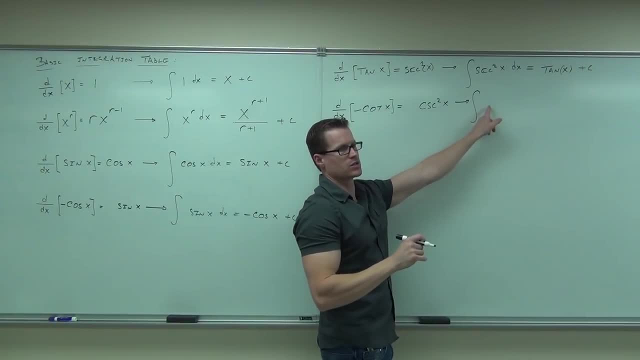 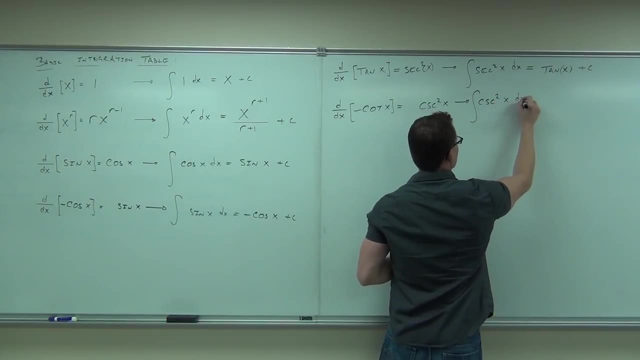 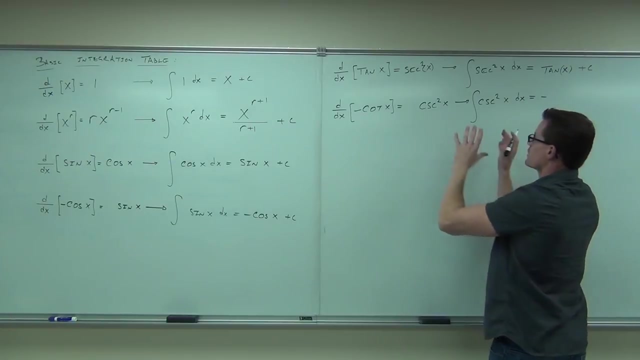 And the reason is because I want to have my cosecant here to be positive. I don't want to have the negative cosecant here. So what's the integral of cosecant squared x Negative? That's that The integral has to undo that derivative. 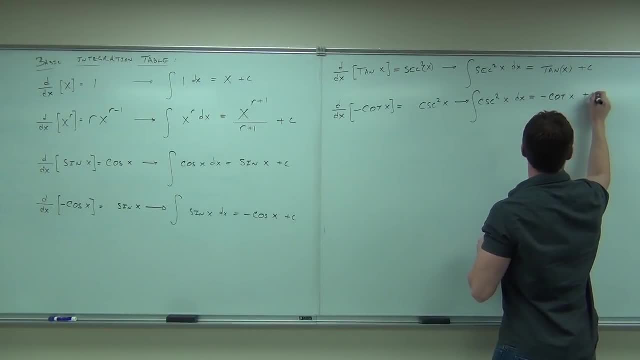 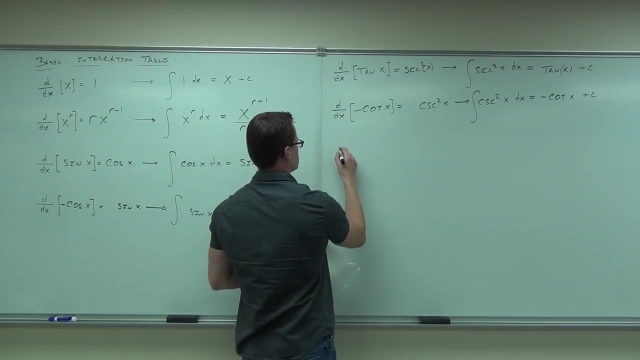 Plus c, Don't forget plus c. Two more Secant: Do you know secant Someone on the right side? do you know secant Right side, right side, right side, Middle. Yes, I've got some work to do. 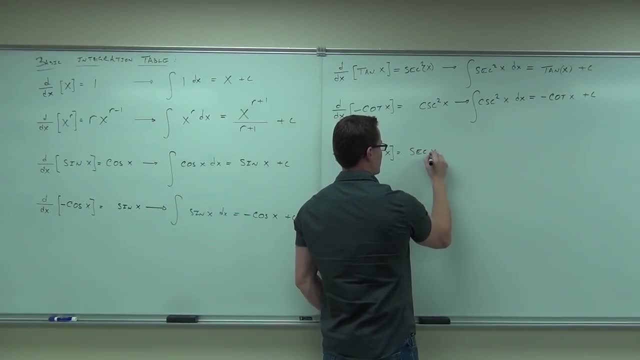 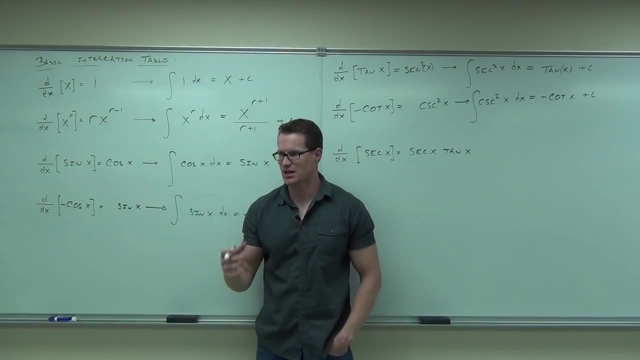 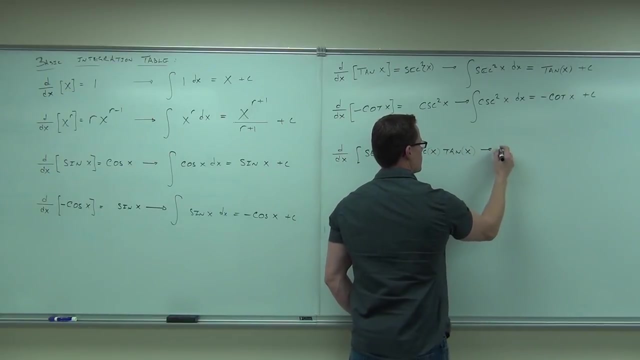 By the way, don't forget that x, It's not secant tangent x, It's secant x, tangent x, Secant x times tangent x. So this is like this: Well then, what's the integral of secant x, tangent x? 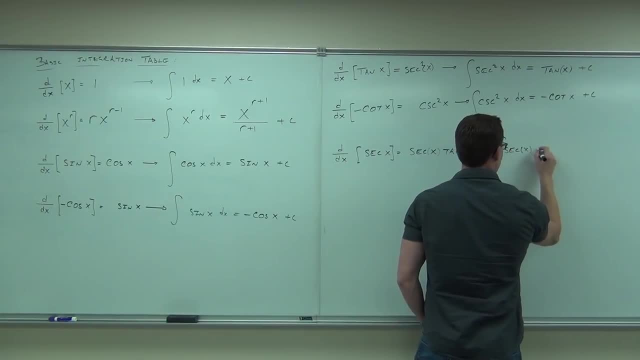 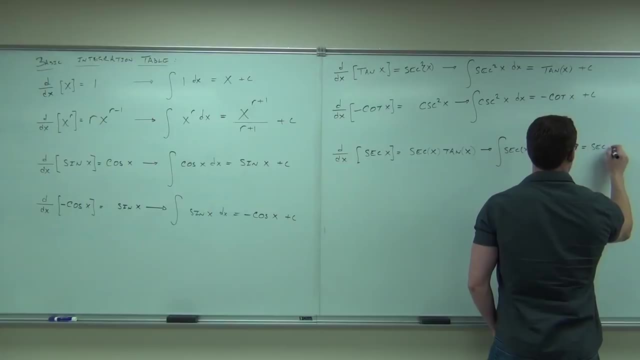 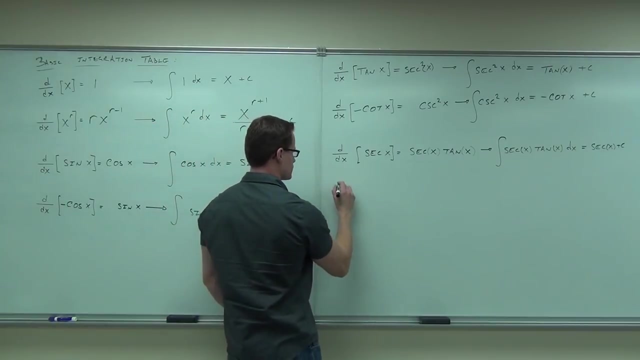 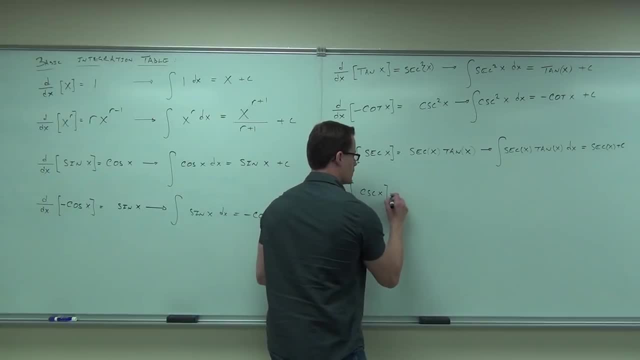 Yeah, Make flash cards up. Make flash cards up for something. You need these. You ever done flash cards before. There's just like cards that you flash, Not like blinker flash Right on the back side. Integral of integral of secant tangent. 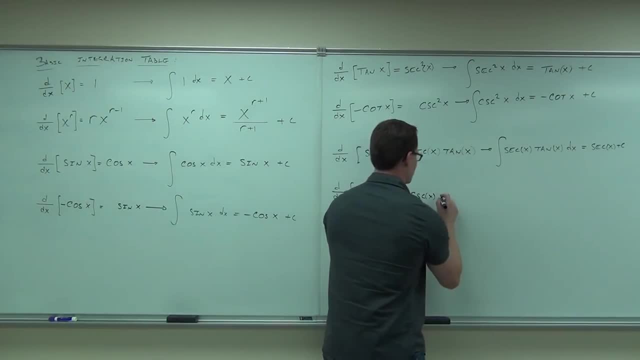 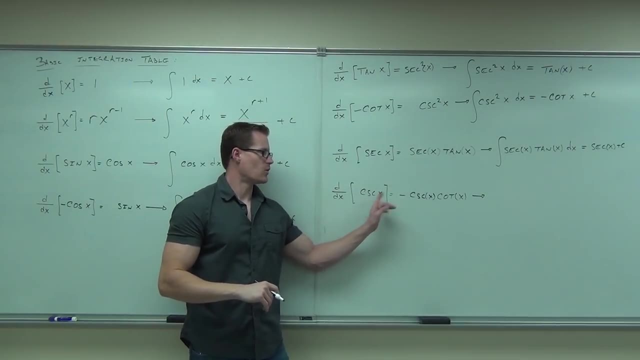 Secant squared. Oh yeah, No. Well, make sure you have them. You also probably know what I'm going to do with this one. I don't want that negative there, I want the negative here. So if the derivative of cosecant gives you negative, cosecant cotangent. 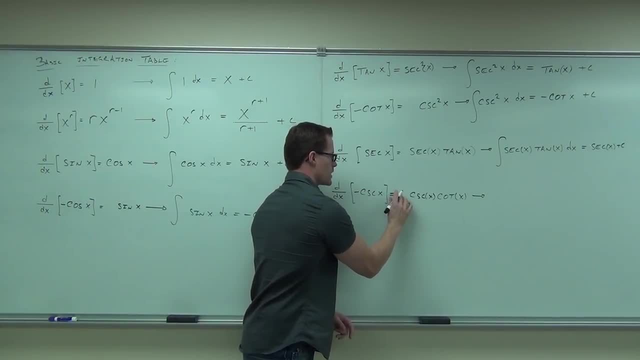 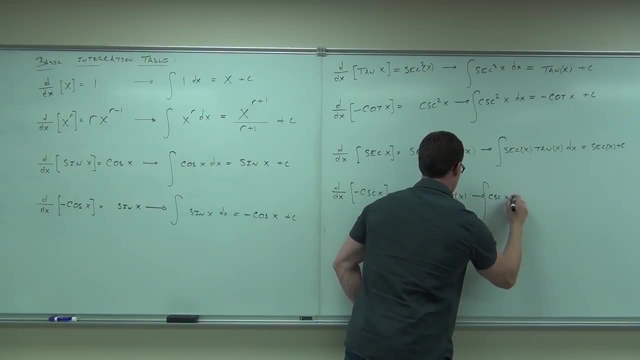 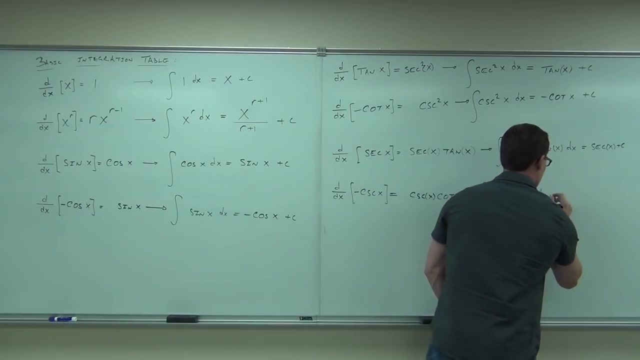 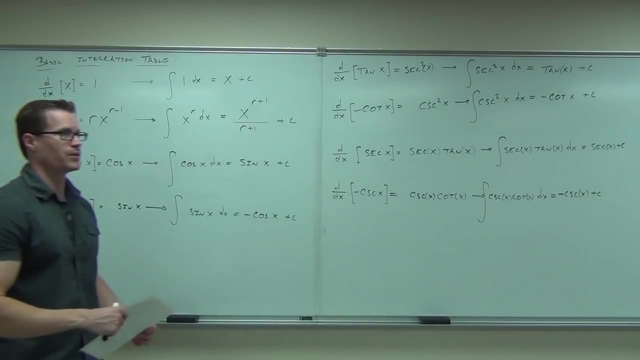 then the derivative of negative cosecant gives you positive cosecant cotangent. So I'm going to change that around. That way I have the integral of cosecant x, cotangent x, dx. don't forget, the dx Is negative cosecant x plus c. 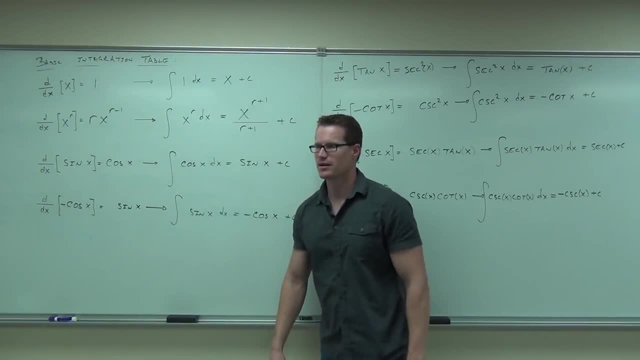 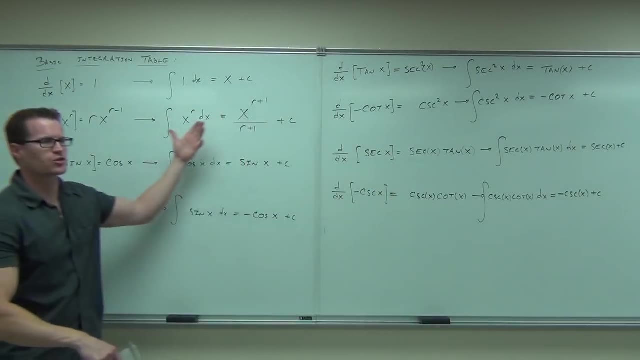 Isn't that fun, Isn't that cool. That's not too bad. Here's the bright side. The bad side is: this stuff sucks right. I mean this is hard to memorize, Especially these four, These ones. not so bad. 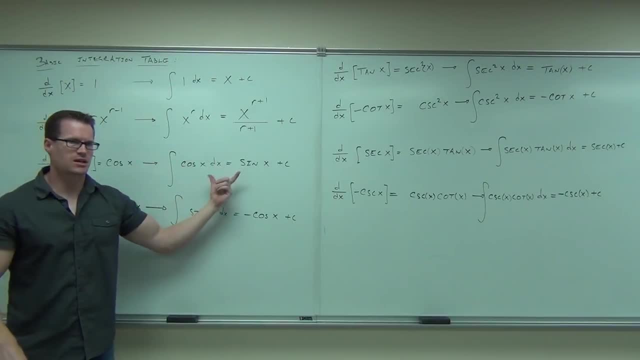 This is easy. This is easy. This is pretty easy because you deal with it. It's pretty easy because you deal with sine and cosine more often. This is okay. You know what. You know where people mess up. I guarantee you. 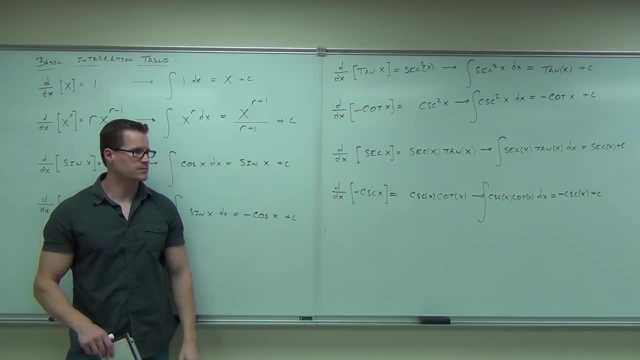 You know where people mess up, Where you're going to mess up if you make a mistake, Where do you mess up? The sines, The sines, The sine, Positive and negative, All the time, Because you're used to doing this. 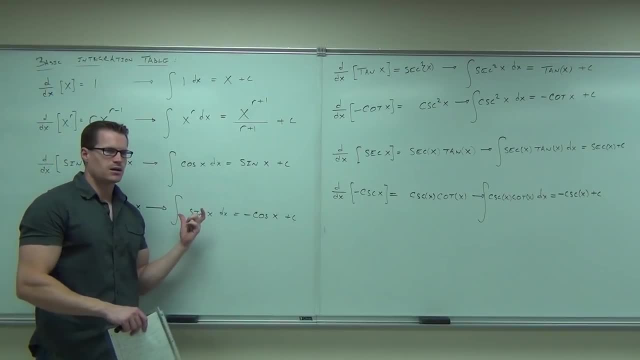 Just think about it. Think about it for a second. If the derivative of sine is cosine, the integral of sine can't. You can't have the same thing both ways, right? The derivative of sine can't be cosine and the integral of sine be cosine. 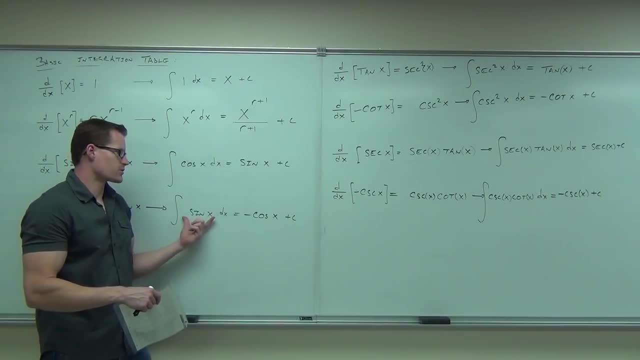 Something has to change there. So here the integral of sine. yeah, it's negative cosine. The reason is the derivative of cosine would give you negative sine. So the derivative of negative cosine would give you positive sine. You can think through it, but it's harder. 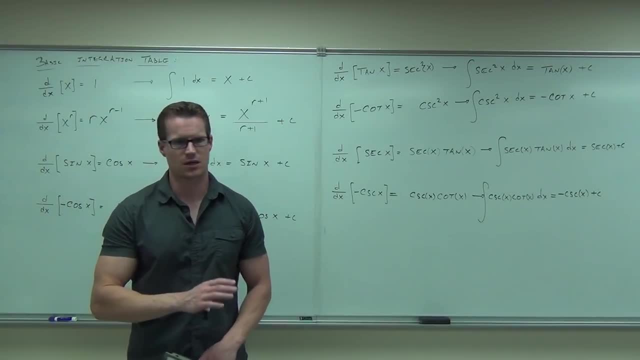 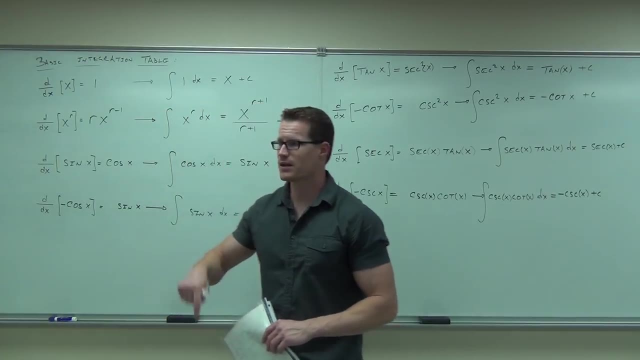 People make most of the mistakes with sines almost all the time. That's where all of it happens, especially that stuff. The bright side is: if it does not fit in this table, you can't do it right now. I'm going to show you one exception to that. 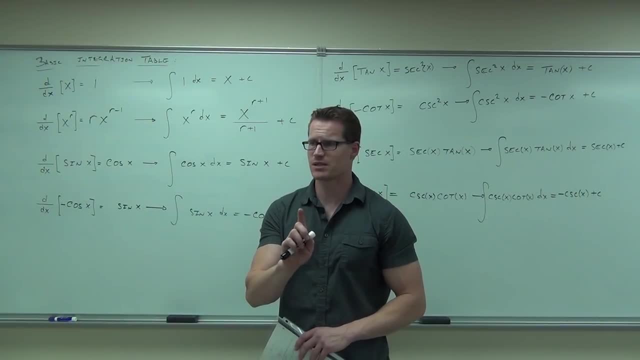 One. It's called integration by substitution. It's very easy, But again, what you get must fit in this table. If it doesn't fit, you can't do it. That's a good thing and a bad thing. Good thing, because if it's out of our realm, you won't even come up with it. so you know. 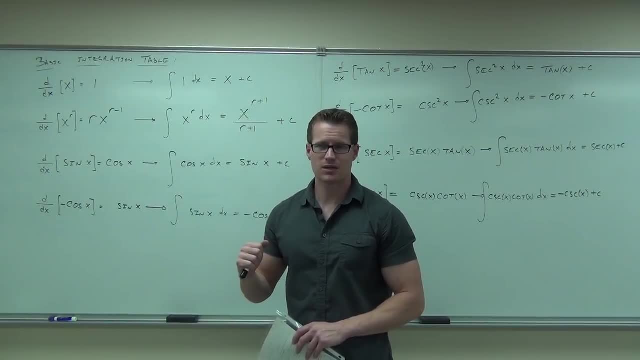 you're going to have an answer. It's a bad thing, because sometimes it's hard to make things fit, And so I'm going to show you some examples on this. But memorize these tables. I'm going to need to erase them. 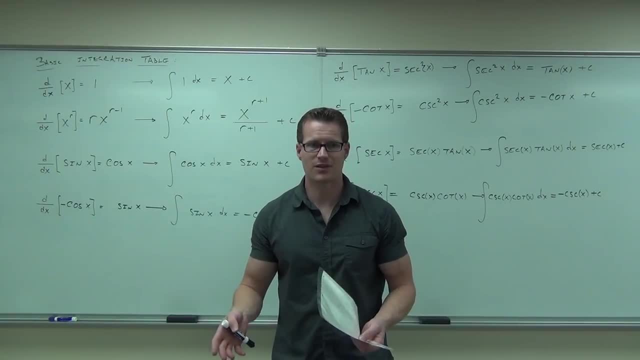 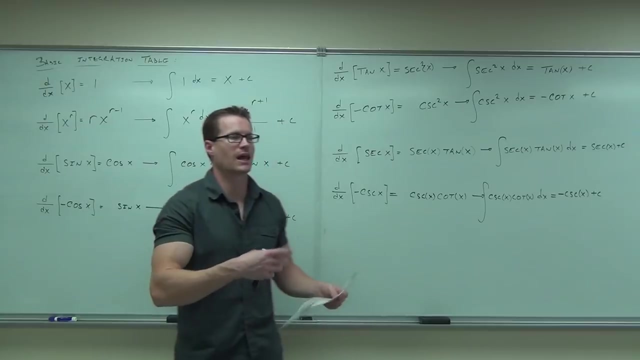 Are there any questions before we begin? Did you see how I got all of them? Basically, it's just undoing derivatives. It's the whole idea of integrals. It's why it's called an anti-derivative. It's the whole idea of integrals. 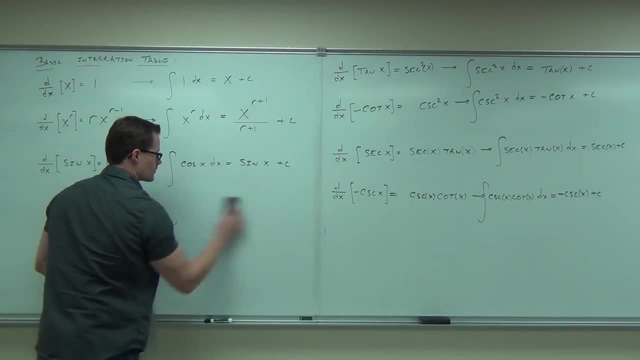 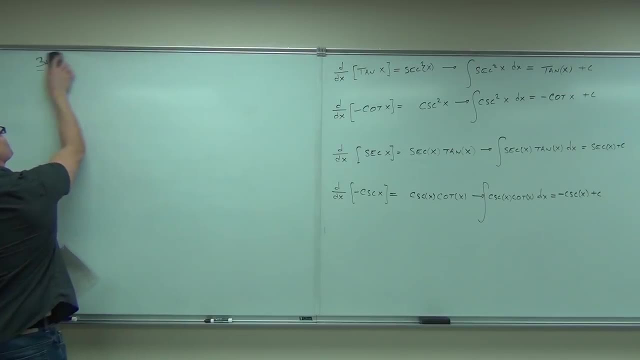 So those are going to be the only answers on the test right now on the board. No, No, That's a nice try, Good try. I'm not getting that one anymore. We dealt with that one four times. How about this one? 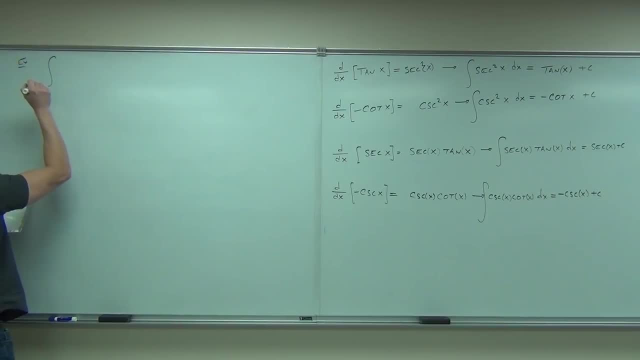 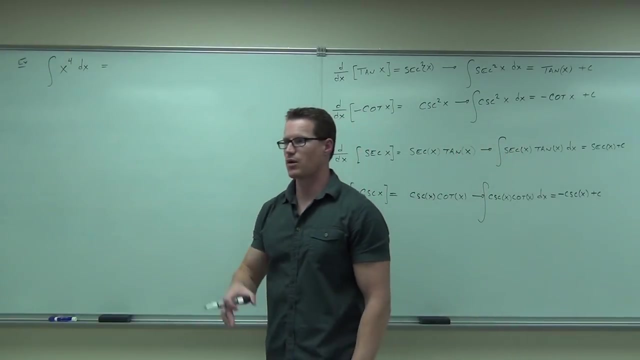 The integral of x to the fourth of dx. Does it fit your table? Yes, Yes, That's something to a power that fits your table. That's why I gave it to you this way. What are you going to do with this? 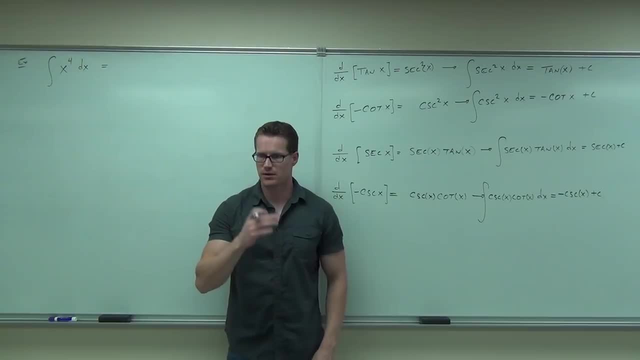 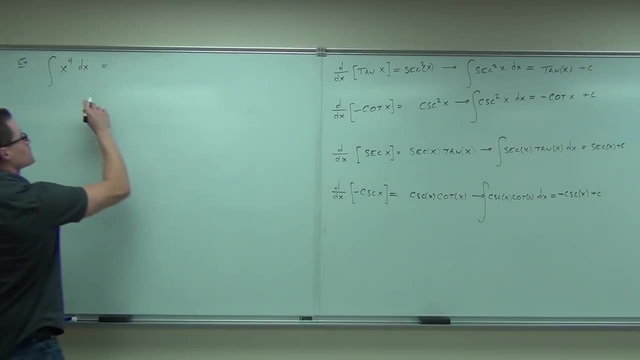 Subtract or add, Add, Add, Multiply or divide, Divide, Divide. You're basically going to do it in derivatives. So instead of multiplying and then subtracting, you are adding and then dividing. So, on our answer here, you're going to have x to the what. 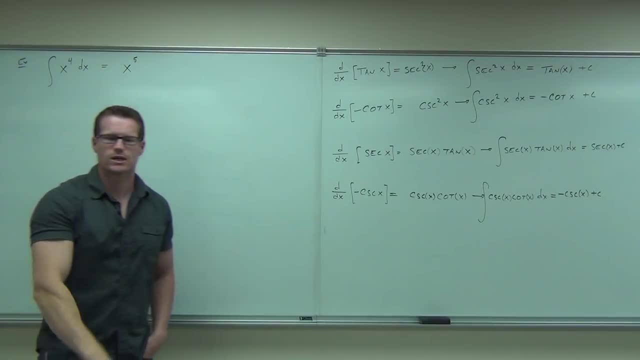 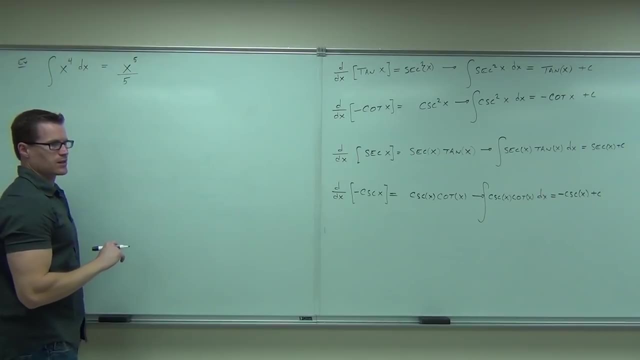 Five, Five. Yes, that's right. You add one, You add two And then divide by what Five Five? Is it okay if we write it as one-fifth x? Sure, Yeah, The book often writes it as one-fifth x. 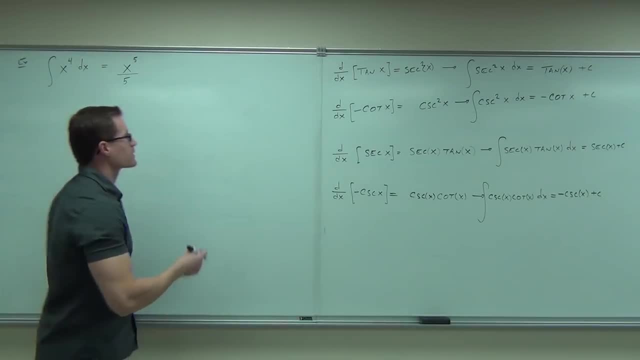 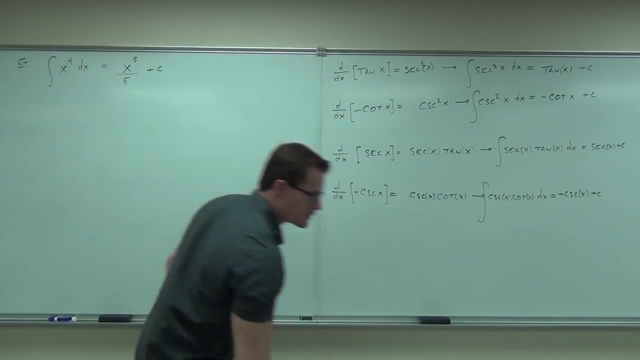 You know it's the same thing though: right x to the fifth, over five, or one-fifth x, And then Plus c. Don't you give me that plus c. Let's try this one. Notice how I have to always write my dx right. 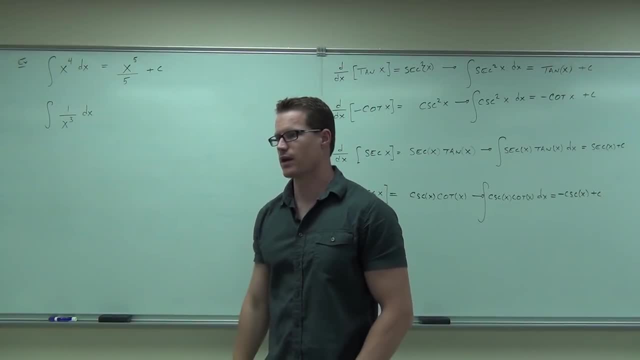 If you don't have that, it's not a good way to write an integral. You're missing something. Does that fit your table? Not quite. Here's what you can't do. You can't do this, You can't go, oh yay. 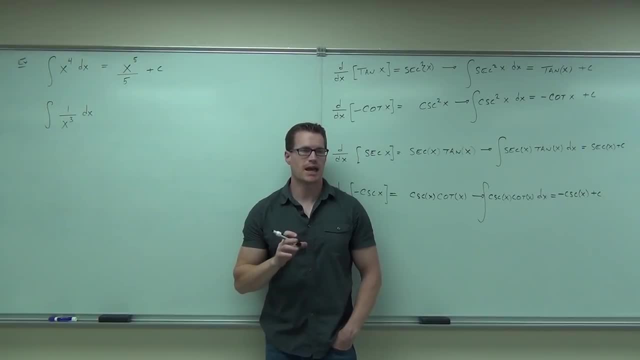 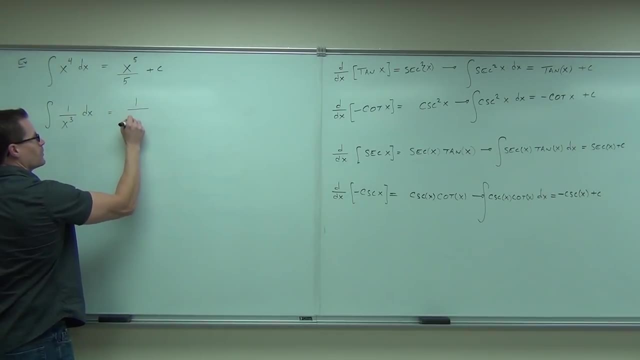 Not so much Plus c. Oh yeah, now you're right, No problem. now, Yeah, Could you break the quotient rule by just doing the derivative of the tau? Yeah, Yeah, Yeah, Yeah, Yeah, Yeah, Yeah. 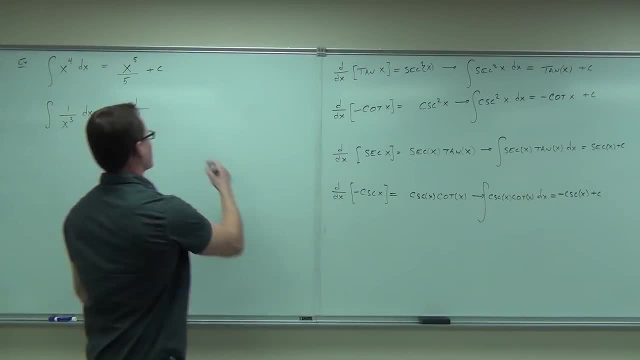 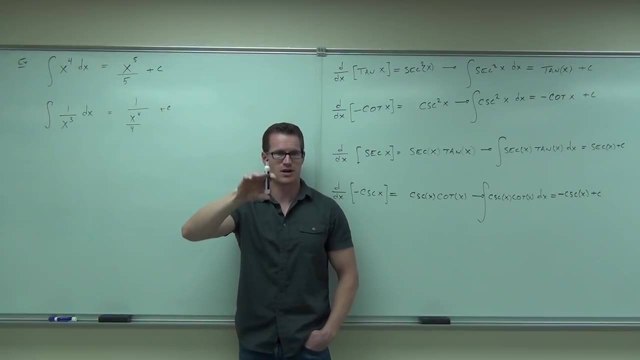 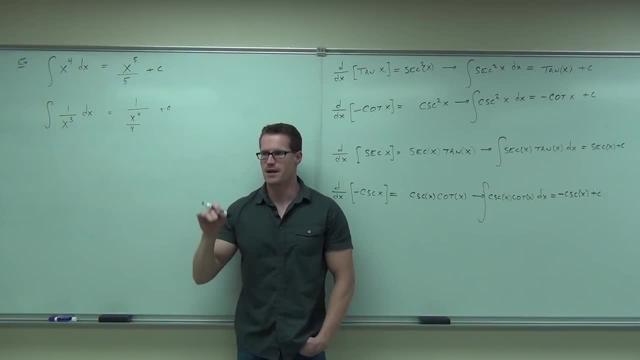 You can't do that. You had a quotient rule for that right. Well, we don't have things like a quotient rule. but note this What I said you earlier: it must fit your table precisely. I don't have anything in my table one, nothing. 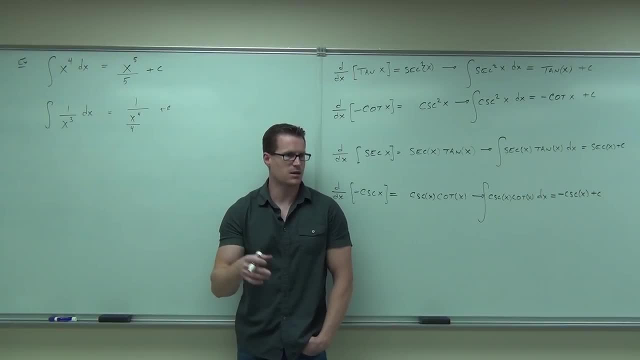 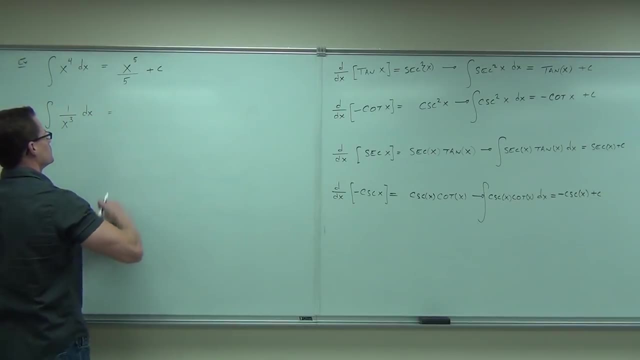 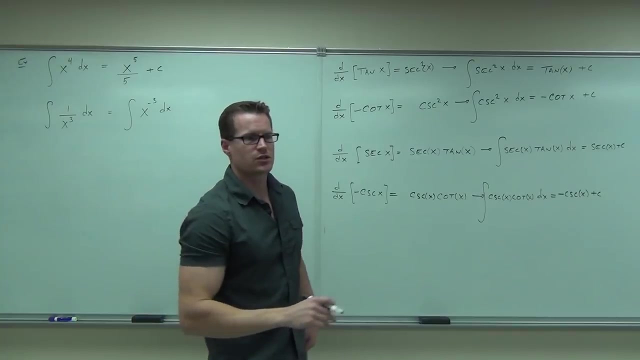 There's nothing one thing over that Is there. Make it a negative 3?. Make it x to the negative 3, that would fit my table. This, no, No, Oh dear, This is true. Yes, Make it fit your table. that's what you gotta do. 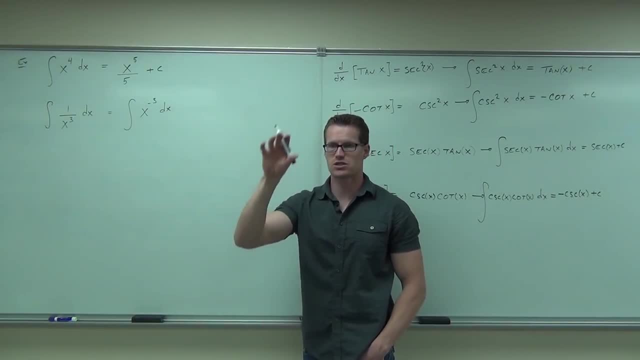 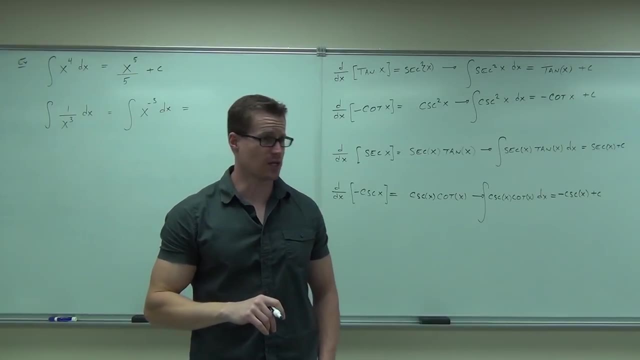 So x to the negative three. hey, now we have x to some power, now we can do it. Just be careful: when I say add, I do mean add, I don't mean get x to the negative four, because that would be subtracting right. 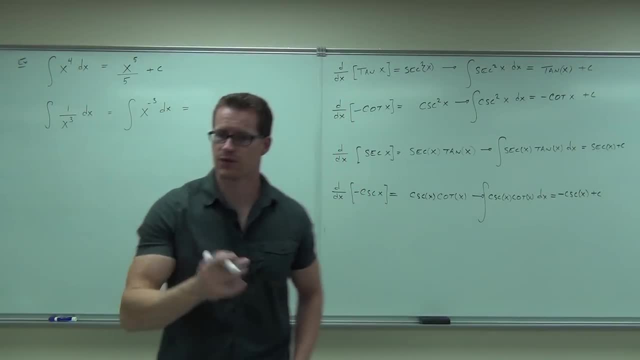 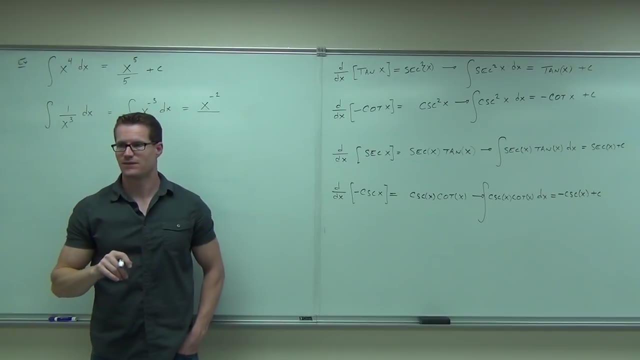 If we're adding to that, you're gonna get x to the Negative two. Negative two. very good Over what? Negative one? half two Over Negative two. Negative two. that's what you're getting over negative two. 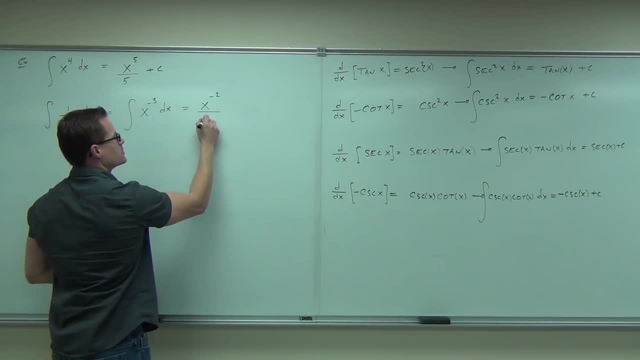 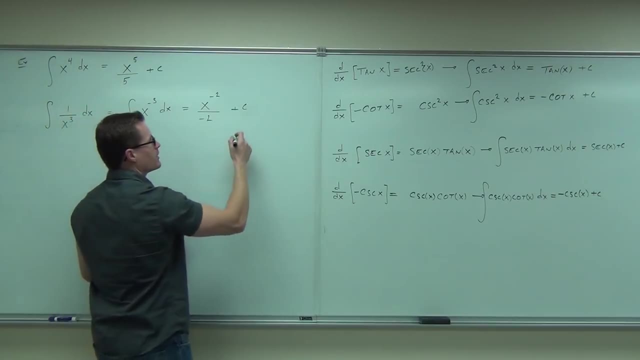 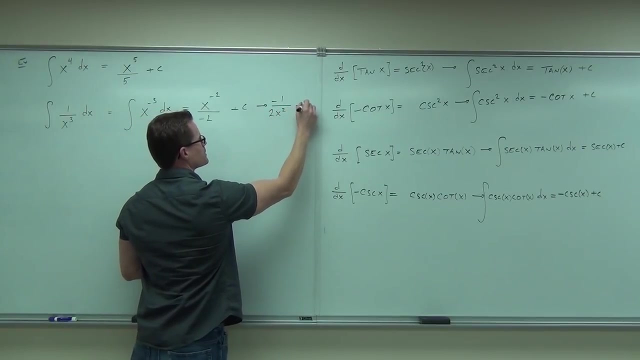 Yes, of course, because you take it over your new x squared negative two plus c. You might make this a little bit prettier. You can do negative one half. you can do negative one over two x squared plus c, which is probably the most appropriate way to write that. 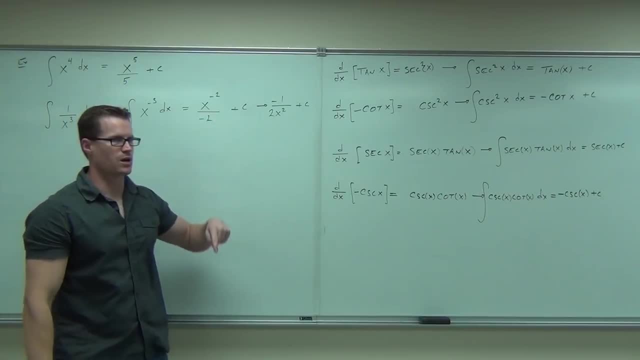 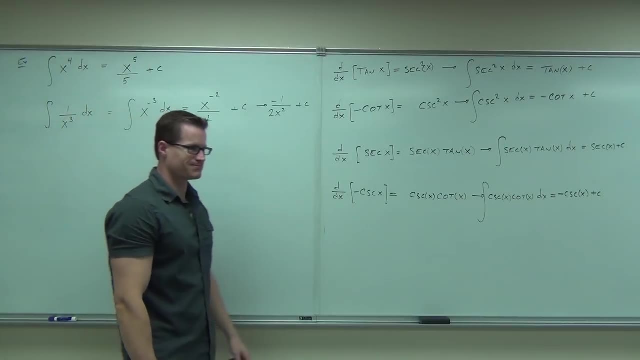 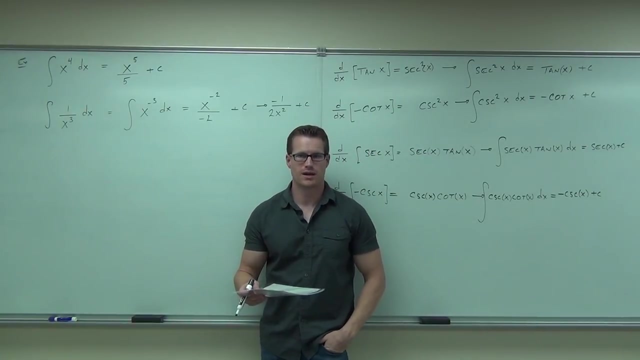 Do you see that? This goes down, that stays there. negative goes up. You okay with this so far? Any one of those would be: Is this acceptable? This is most acceptable. yeah, Now, by the way, could you check your work? 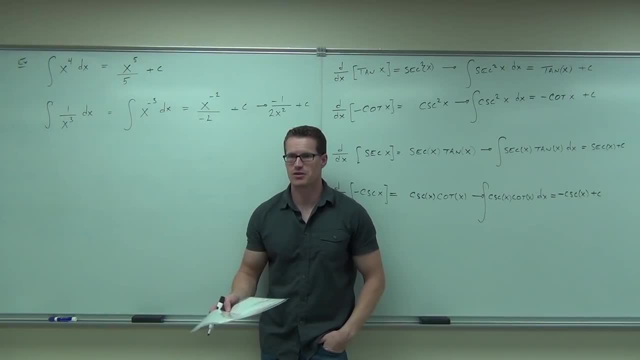 Hey, what checks your work? Derivative Duh, I mean. yeah, You should never get the wrong answer. You can always check your work, Unless you do it really hard on the rules. But most of the time you can check your work right. 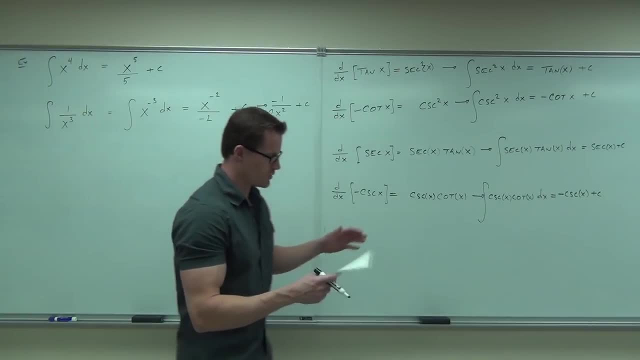 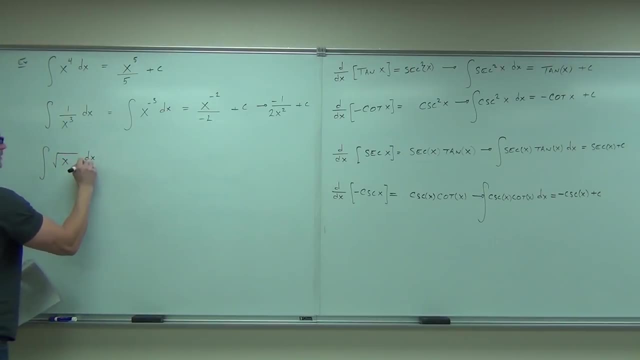 All the time you can. it just gets more difficult. But here with these easy ones, man, you should never get one wrong. You shouldn't ever get one wrong. You will, though. Some of you will, yeah, Some of you will- find a way. 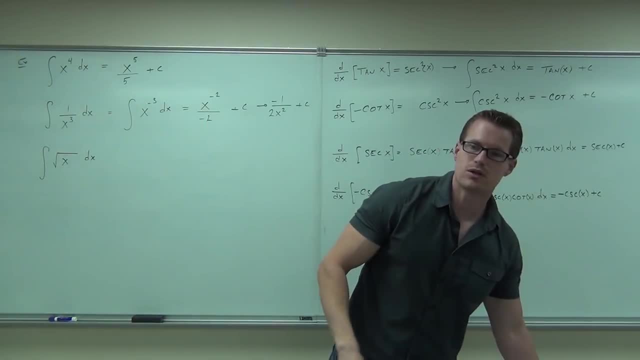 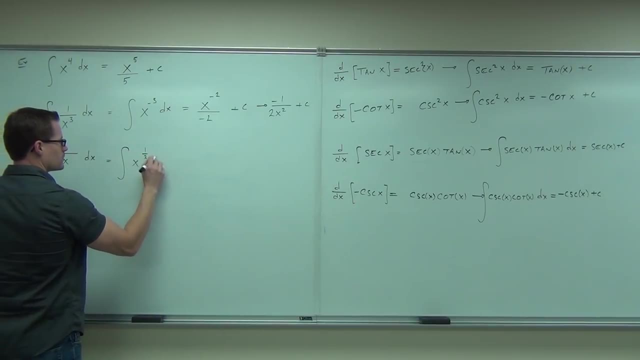 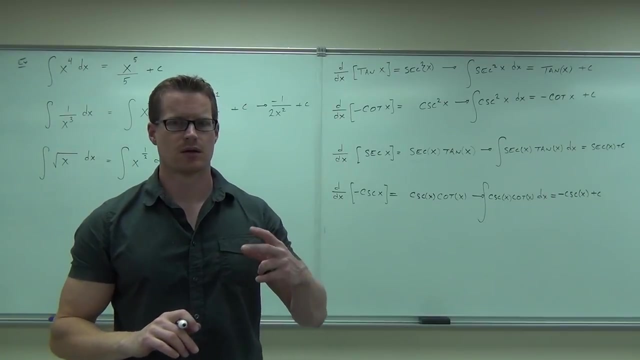 Okay, is that in your table? No, Make it fit your table. what do you do? So we got it. X to the one half. what do you do with the x squared? You add or subtract With integrals. you add. 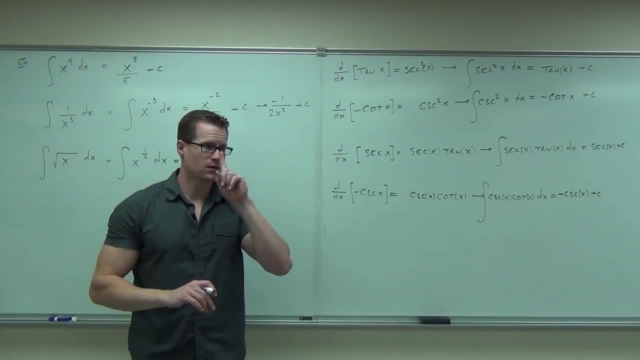 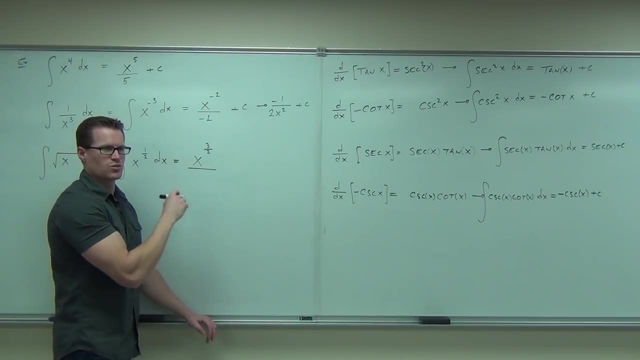 So we're gonna get what's one plus one half? Is it one? Three to the half? It's three to the half. So x to the three halves over. this is why I do the over, so you can really see this. 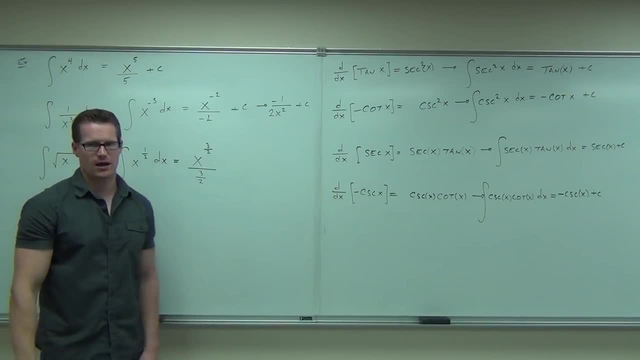 over three halves, right Over three halves. You got me That's x to the three halves over one, divided by three halves. If you, I'm never gonna do this again, but you can see it this way: X to the three halves over one over three halves. 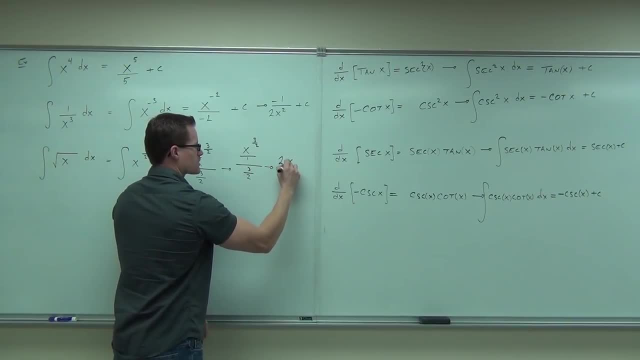 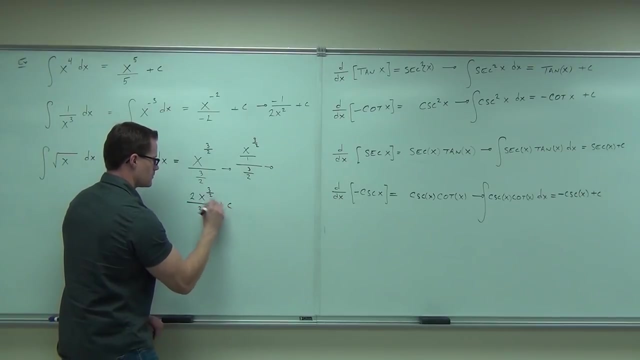 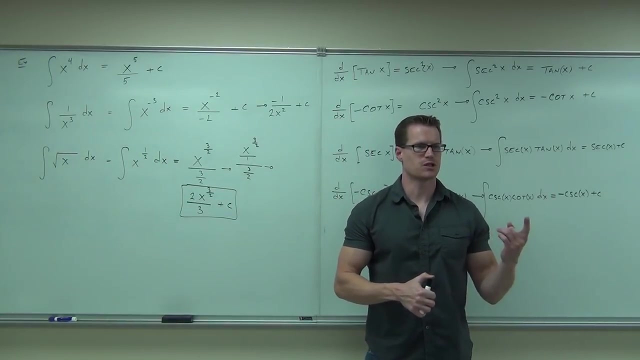 Reciprocate and multiply. What you end up getting is two x to the three, halves plus over three- I ran out of room, sorry. Plus c, Plus c. You notice a couple things about this. Firstly, did I put the plus c right when I did the problem? 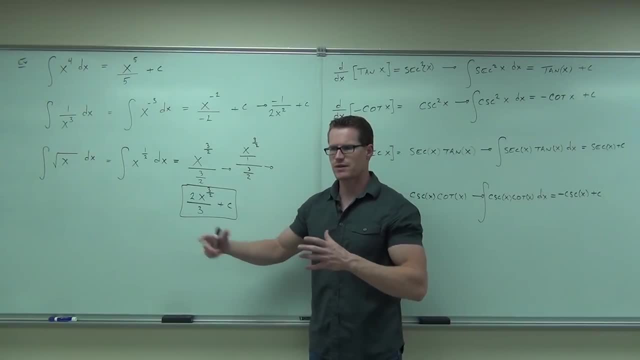 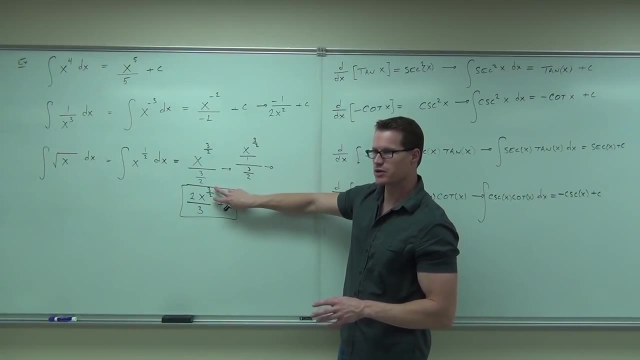 No, Not really. We only need the very end, just the very end. You can ignore it as long as you don't forget about it altogether, But the very end Also, could you check this with the derivative? Well, let's see. 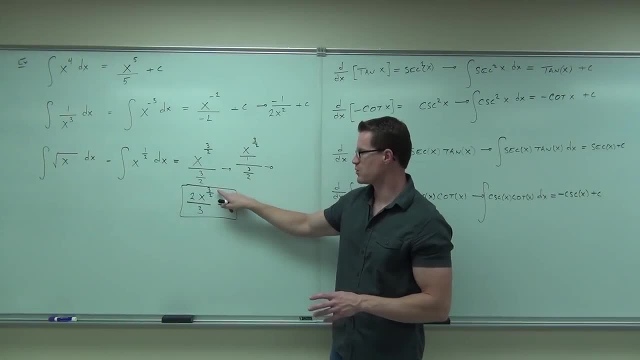 Derivative says you multiply by that, Hey, there goes the two thirds. Subtract one from it, There's the one half The c's gone because c's a constant. right Derivative of a constant is zero. That's the correct answer. 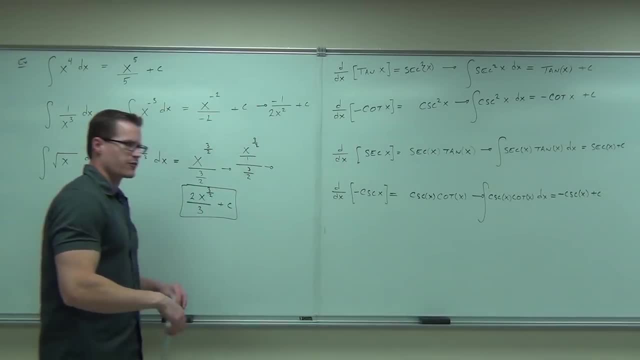 That's what we need to be getting Ready for. one more. I'm not supposed to do this one. Oh good, Let's do it again. What do you do first? Yes, Now play along. When you do this, you get. I'm going to do every step for you. 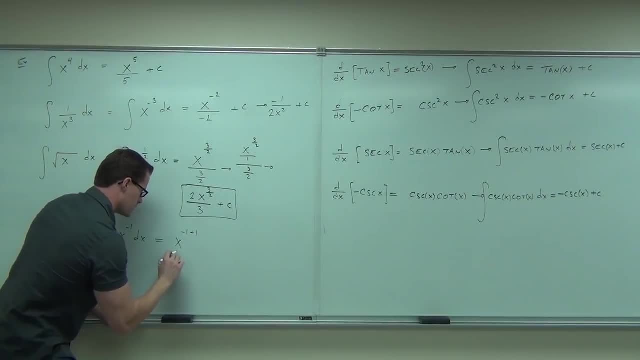 You get x to the negative 1 plus 1 over negative 1 plus 1.. Right, You get x to the 0 over negative 1 plus 1.. Right, You get x to the zero over negative 1 plus 1.. 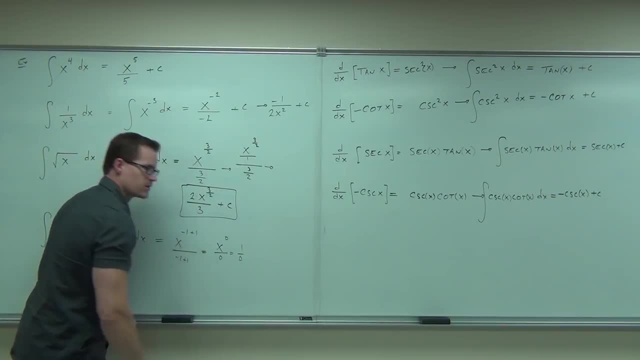 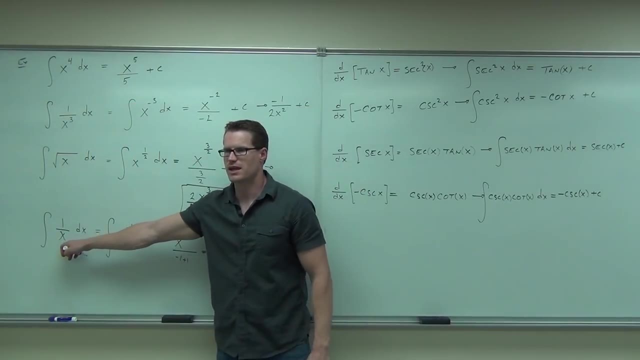 Right over zero, you get one- oh crap. you get- oh crap. Why, why? why, oh crap, you can't. So when you see this, can you actually do it? This right here is something out of the realm of this class. 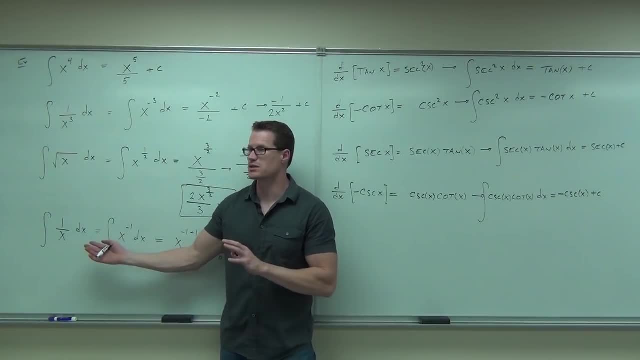 We do late transcendentals, we do functions like this later in 4B, which you're going to get this I'll give you a little hint. What this gives you is actually the integral of this is actually lnx, That's the integral of one over x. 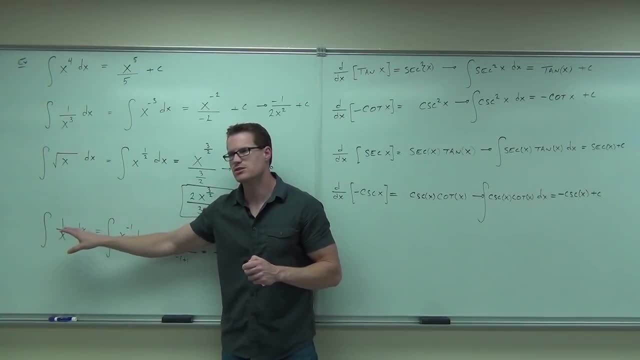 So when you see this, when you see one over x, you can't do it in this class. all right, You're not going to be able to do it here. I just want you to see it that, yeah, that power rule only works if your exponent is not negative 1.. 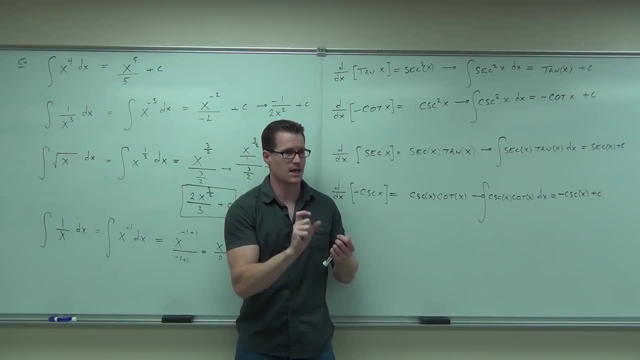 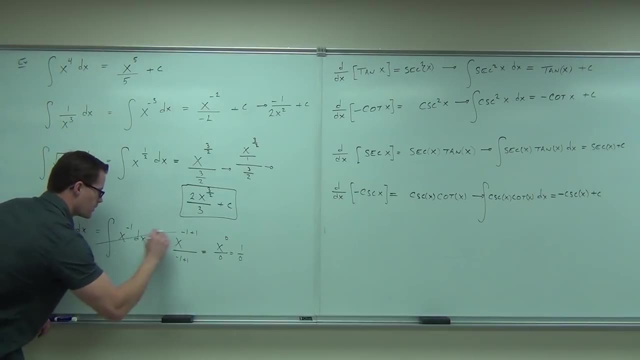 If it is negative 1,, you divide by a new exponent that is zero and you can't do that. So this one's off the table for us. We can't do that one, This one, if you really want to know this is can't do that. 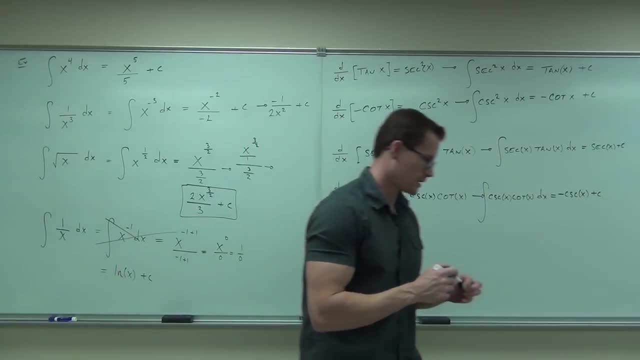 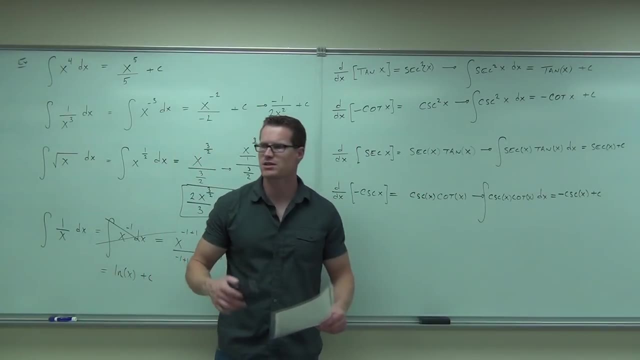 You're familiar with: x, It's ln. right Natural log: Natural log- It's lnx. Let's cover a couple properties before we go any further, and then we'll start just practicing some of these things, getting more and more used to taking the integral. 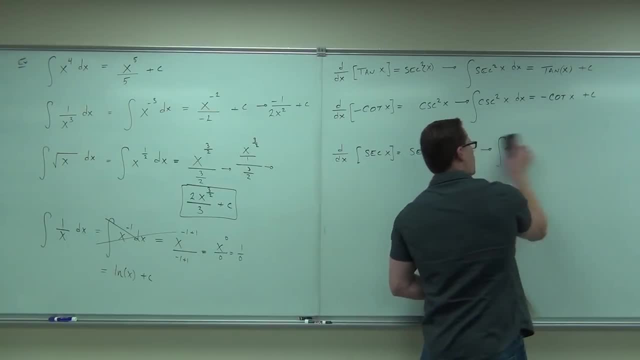 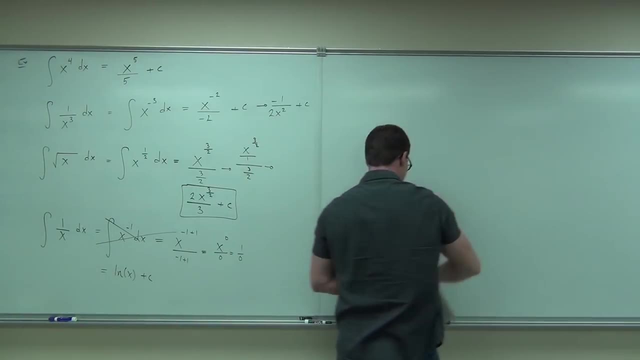 finding those anti-derivatives. The properties you're going to find out are very, very similar to the properties of derivatives. I'm just going to state them for you. You'll see them, because they're exactly the same as derivatives. You're like, oh yeah, that makes sense. 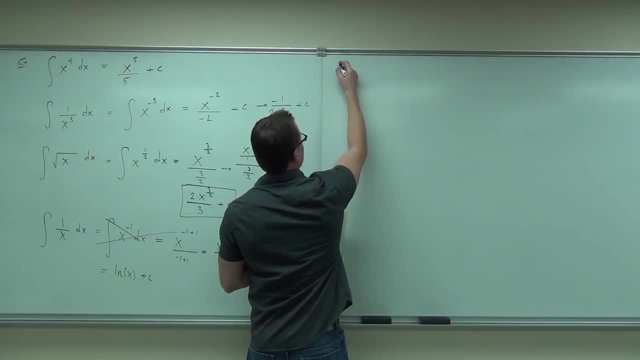 First one is: if you take so properties, If you take and have an integral of a constant times some function that has an x in it, what do you think you can do with that constant? Take the constant outside of that constant, We can. 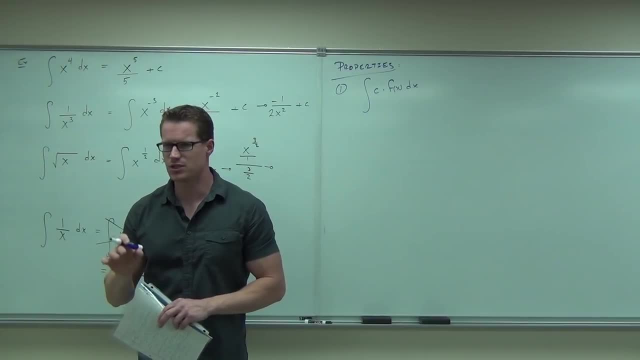 And typically you see this a lot more with integrals, With derivatives. we didn't really do that, Remember. We said we could, but we ended up just multiplying With integrals. you really do, You do it a lot. 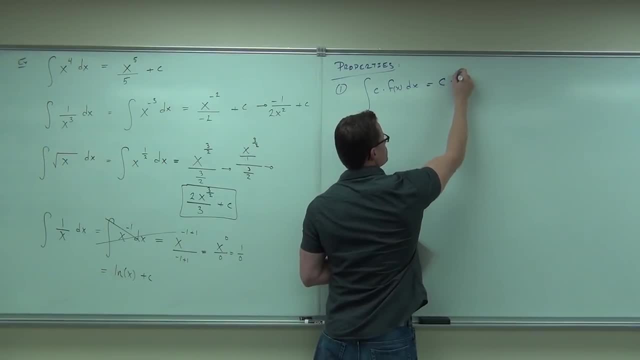 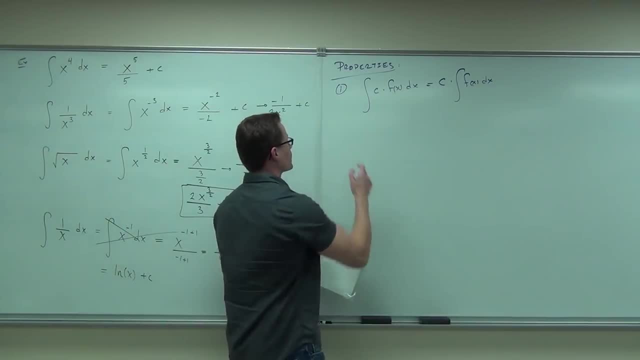 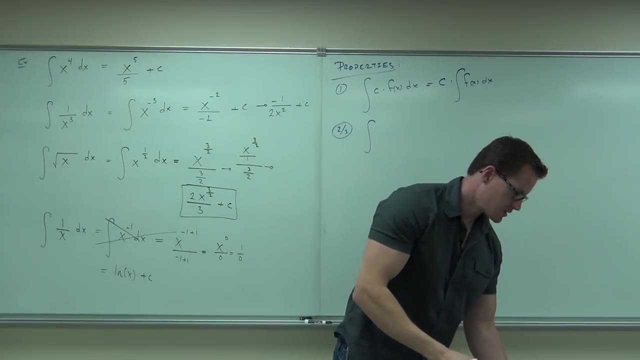 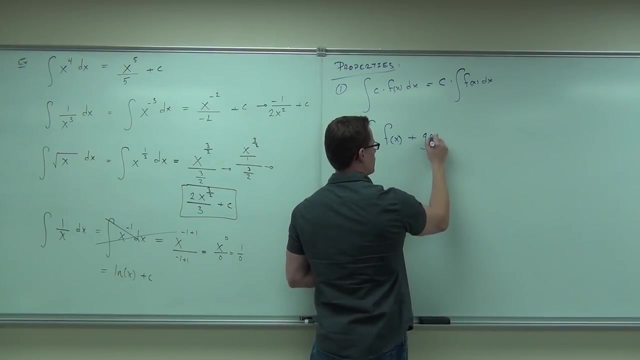 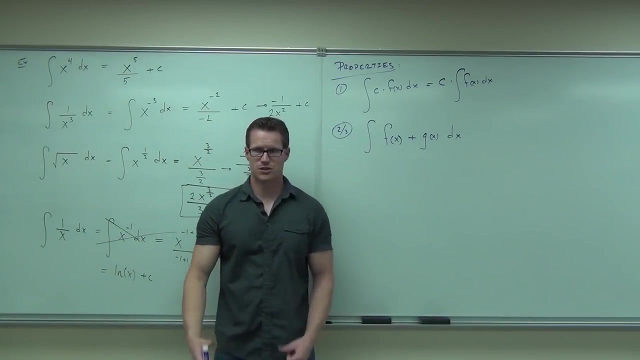 Yes, I'm going to put 2 and 3 together. Here's 2 and 3.. 2 and 3 say. let's suppose that you had two functions being added together within your integral, like that, with derivatives We could separate those, couldn't we? 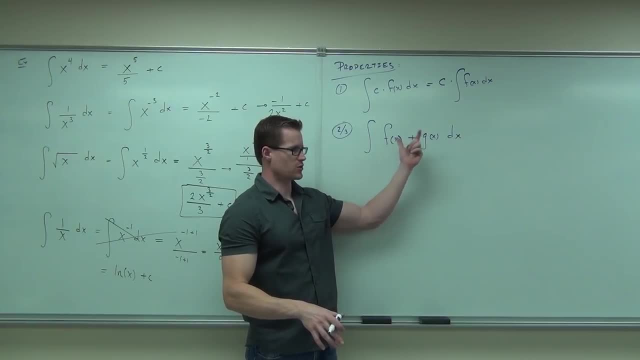 We could take the derivative of the first one plus the derivative of the second. That means here: that works as well. You did the integral of the first one plus the integral of the second. What we couldn't split up was that right. We still can't. 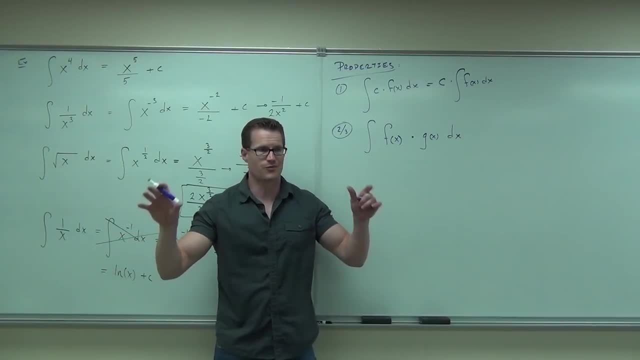 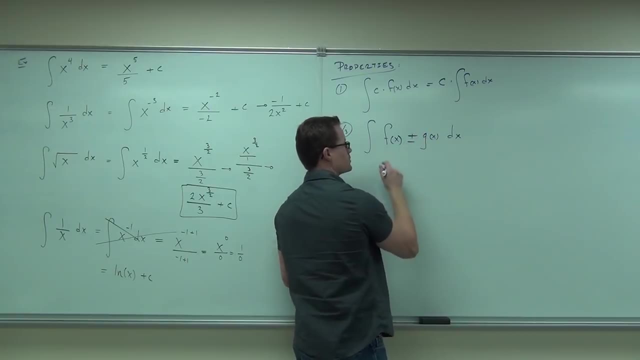 We still can't do that, So you can't split up two integrals like that either. It's very much like derivatives, because you're going backwards from a derivative, So you can't do that either. But this you can, and this is 2 and 3.. 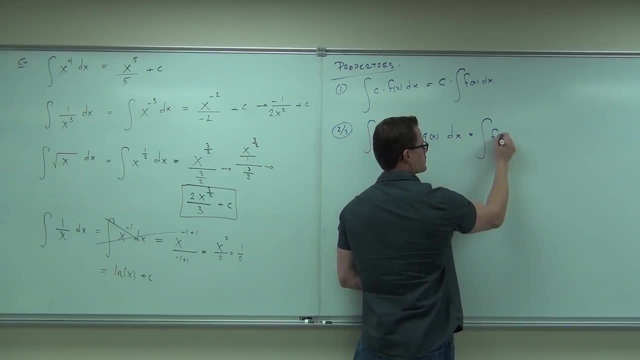 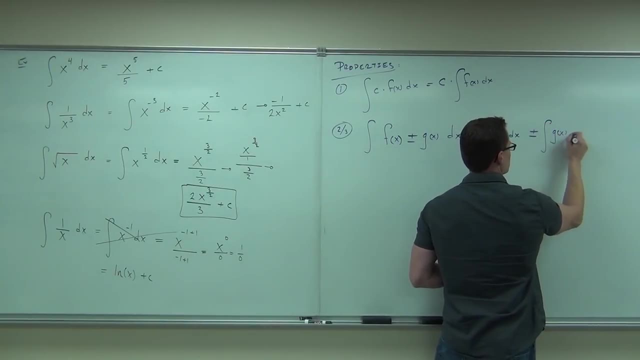 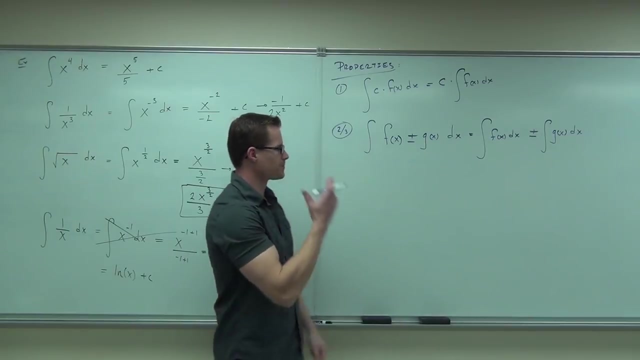 This says you can take the integral of f of x d x plus with plus, minus for minus g of x d x. It says I can take the integral piece by piece. basically, That's what that says. This one is not true. 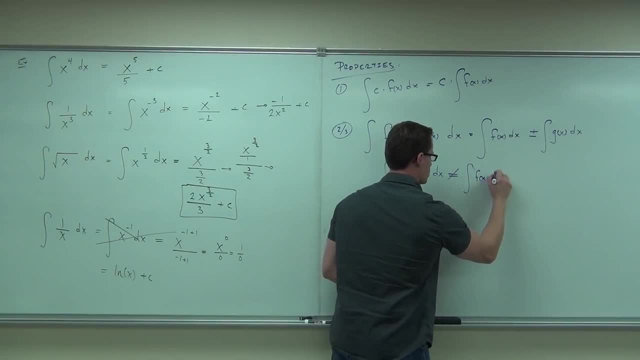 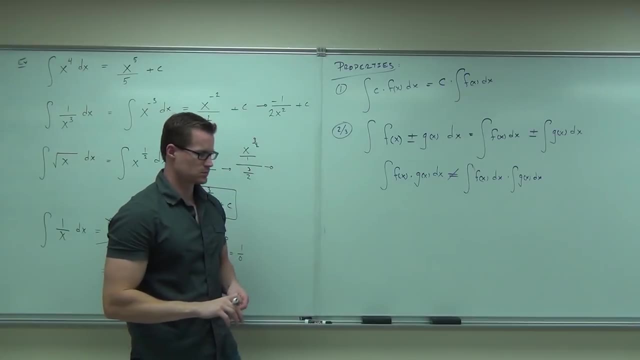 Not true. Still, okay, Let me caution you about the c's. You know we have to have plus, c's right. Let me caution you on how to do the c's. I think I mentioned this just like 20 seconds ago, but I want to make sure you see an example. 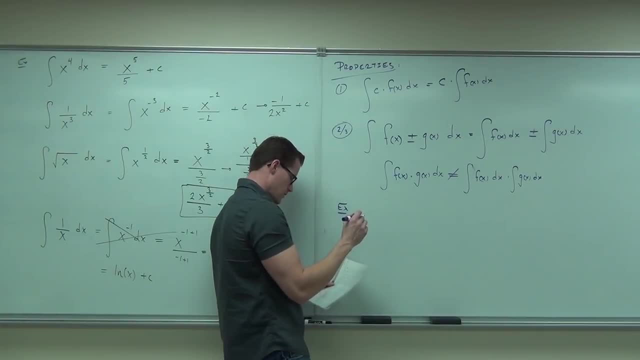 Let me give you a real quick example on this. Let's say I had the integral of: let's just do 2x. Note that 2 is a constant 2. I should be able to pull out in front of my integral and I can. 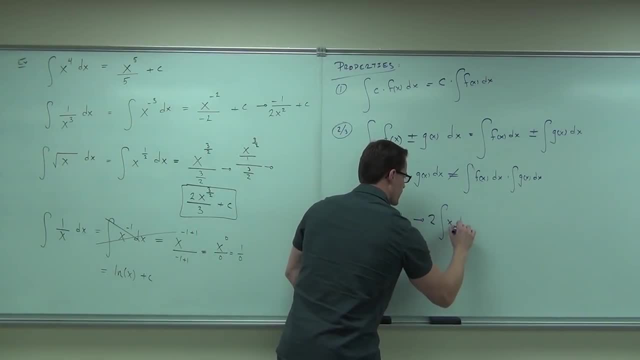 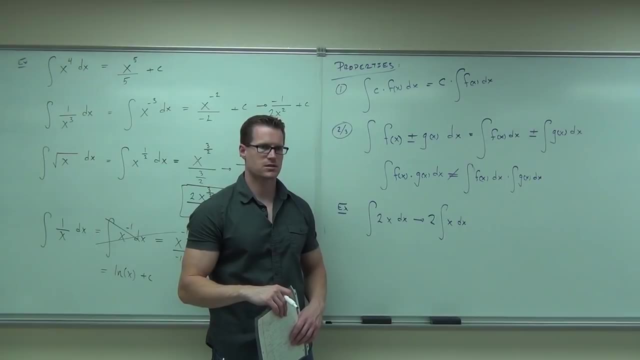 So this would be 2 times the integral of x. Remember, I said, your integral has to fit your integration table. This does What's the integral of x? 1.. 1.. Oh dear, Are we doing derivatives? Think, think, think. 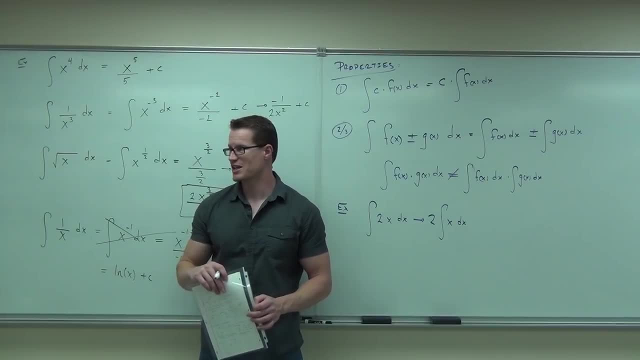 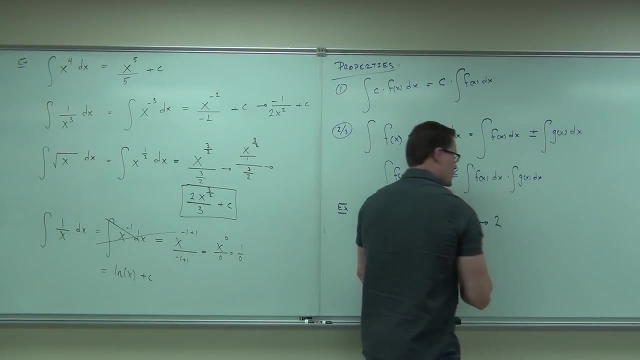 x squared over 2 is correct. Oh my gosh, I erased the integration table and you all forget. I did 2, 2,, 2,, 2.. x squared over 2 plus c. Does that make sense to you? 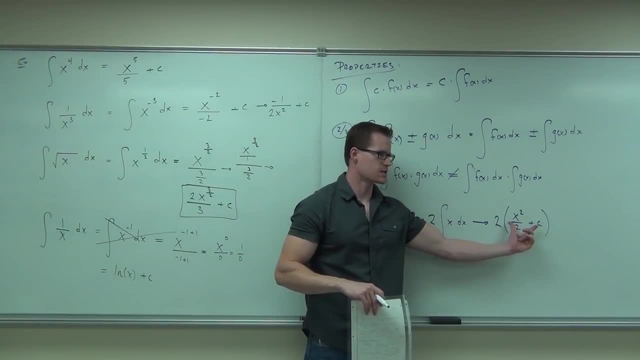 You have the 2, you have the x squared over 2 plus c. Now, For those of you who have written it like this, for those people who think, oh, I need the plus c immediately, well, that gets confusing. 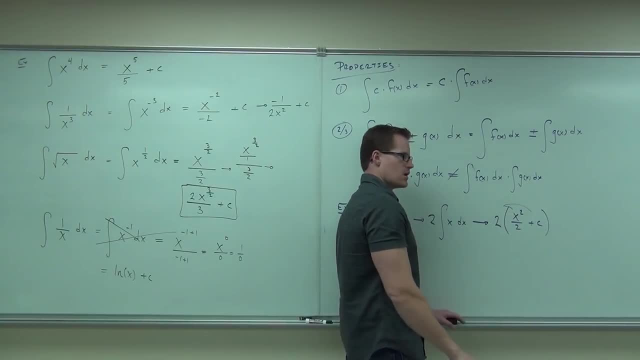 because what are you supposed to do? Do this, If you do that, what do you get? What do you really get? You get x squared right. You get x squared Plus 2c, Plus 2c. However, what is plus 2c? 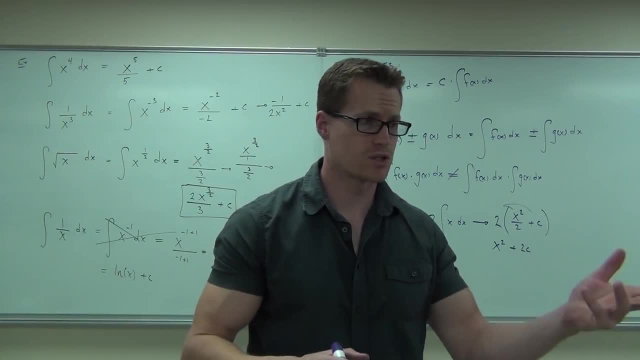 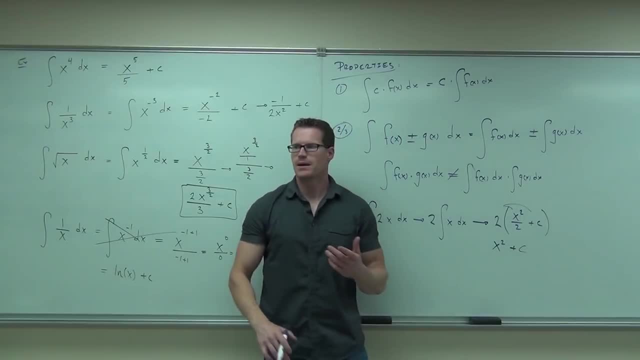 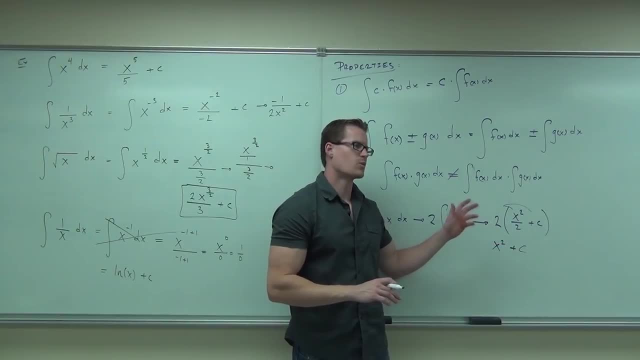 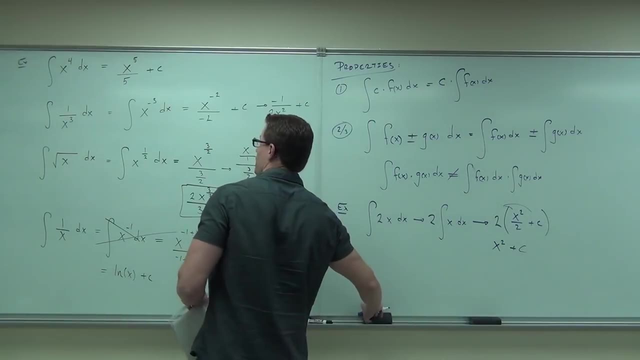 You can put the plus c immediately and be careful on it, or really just ignore it and put it at the very end of your problem. Can you do that for me? Here's another example about why this is kind of useful. I'll give you one more. 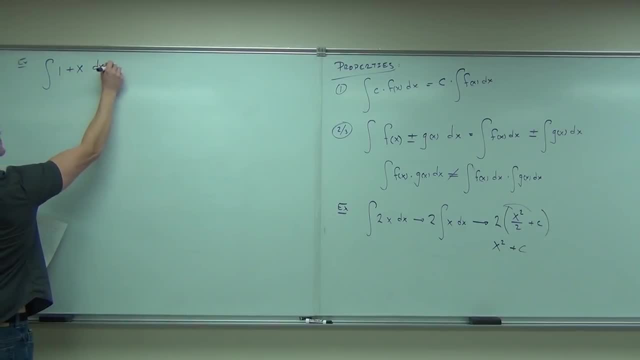 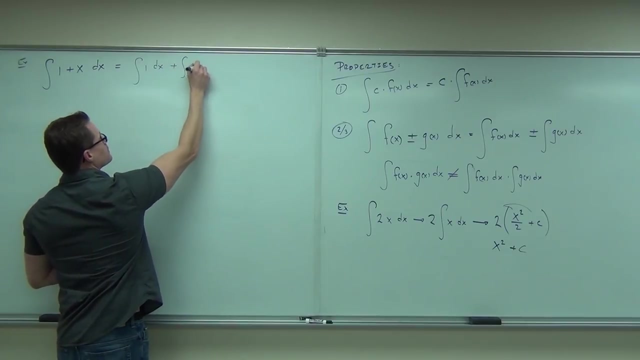 Integral of 1 plus x dx. Can I split that up? Yes, That's the integral of 1, dx plus the integral of x dx. Here's what I mean about the c's. Just watch, Just watch. 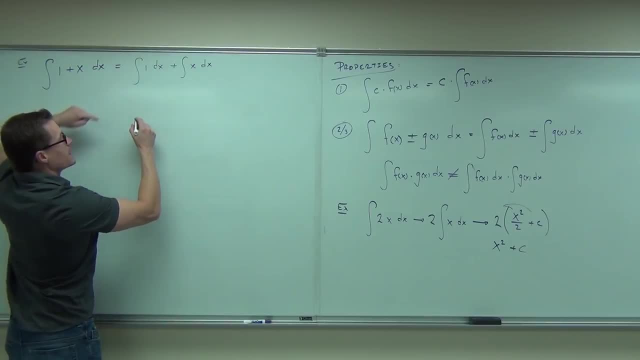 Okay, watch for a second. You write down later The integral of 1, dx is x, True, Yes, So if you said oh, x plus c, you have to call it c1, because it's going to be another. 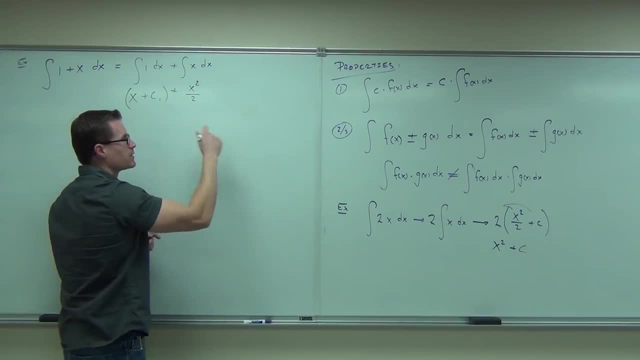 constant Plus this is x squared over 2, yes, we just did that- plus c2.. But then when you add them together you get x plus c1 plus x squared over 2 plus c2.. And you get x plus x squared over 2 plus c1 plus c2 by re-commuting those things. 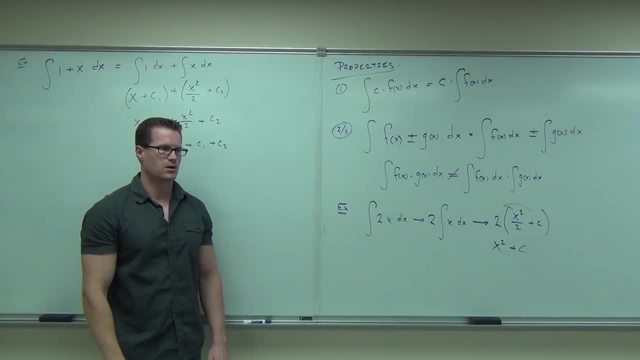 Follow that: How much is c1 plus c2? It's a constant plus a constant. It's not a constant. Who cares what it is, It's going to be a constant. Does that make sense? So here, ignore the c1 and the c2.. 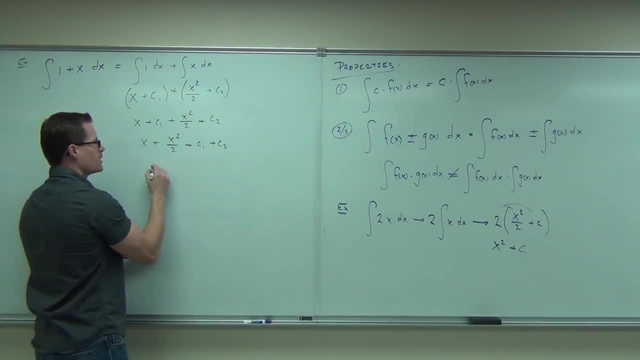 That's too hard to deal with. So basically you'd have x plus x squared over 2 plus just c. It's just going to be a constant there. You're not adding together different c's and going oh crazy. It stands for any constant. 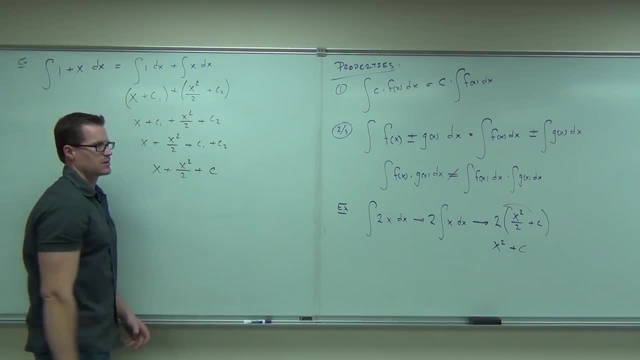 So any constant could be c1 plus c2, but who cares? No, I mean integral, So you have to line up. You just always end it with plus c. You're going to have 1 plus c at the very end of your problem. 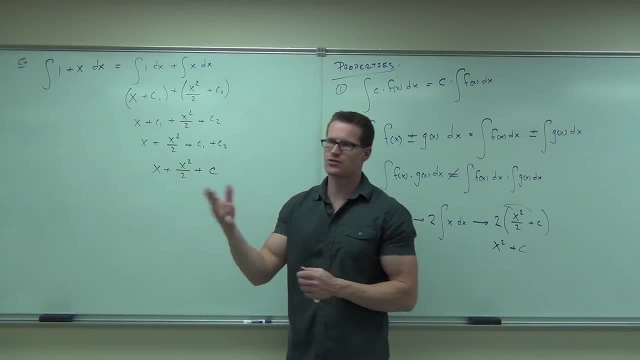 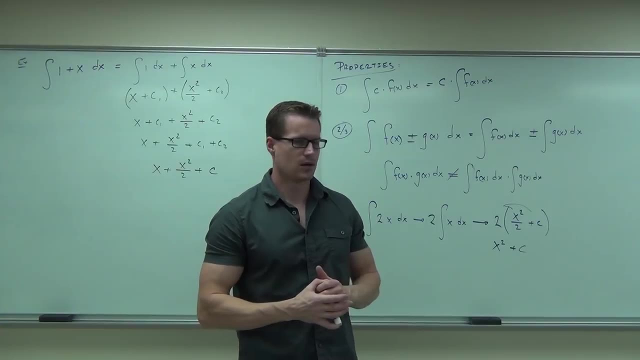 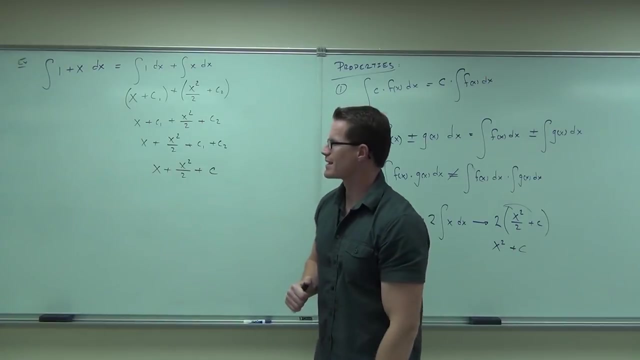 That's for indefinite intervals. That's what you're going to do. That's what you're going to do. That's what you're going to do. Now, one last thing. Do you remember how, with derivatives, when I said I want you to take the derivative of 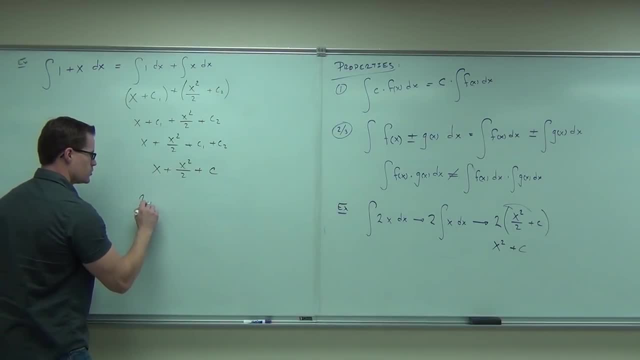 2x squared. don't write this down, just watch. minus 4x plus 3.. You didn't split that up, did you? You did 4x minus 4 and then zeros. Right for derivatives. you can do the same thing with integrals. 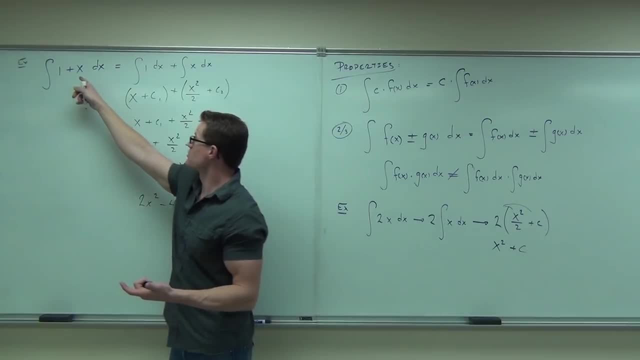 So here, could you split it up? Yes, you can, But could you get directly from here to here? Sure you can. What's the integral of 1?? What's the integral of X? X squared over 2.. Where's the C coming from? 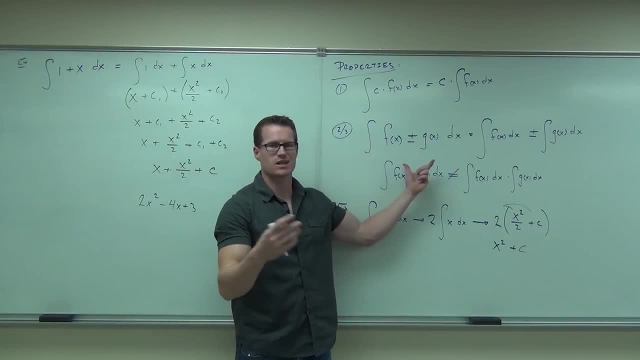 You need a plus C. That's the same thing. I'm just saying that this is possible, just like you did with derivatives. this is possible. Therefore, you can go directly from here to here. You with me on that. What you can't do is this again: 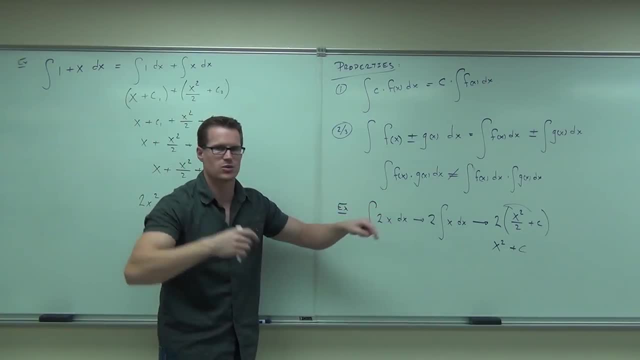 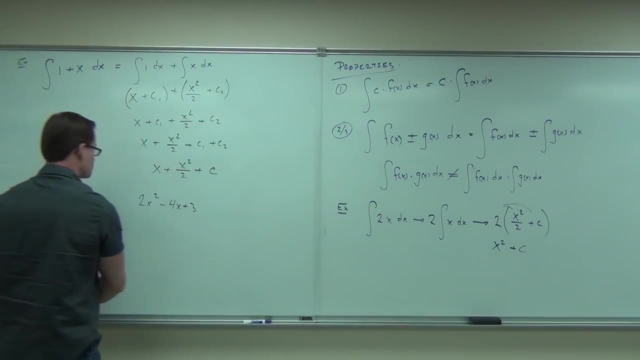 you can't break the multiplication thing, You can't do integral of this times integral, That doesn't work. So when you have functions of X multiplied together like this one, is there a special rule for that? Nope, Yeah, kind of. 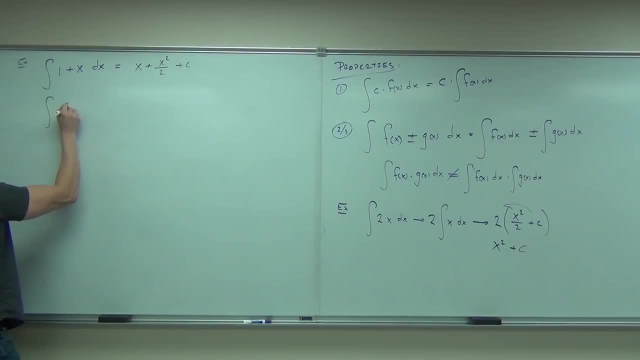 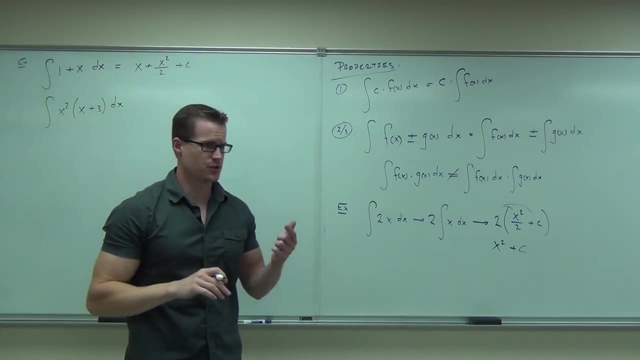 You can go directly from there to there, But something like this: What you could not do, you can't take the integral of this thing times the integral of that thing. That doesn't work. It doesn't work at all. What could you do? 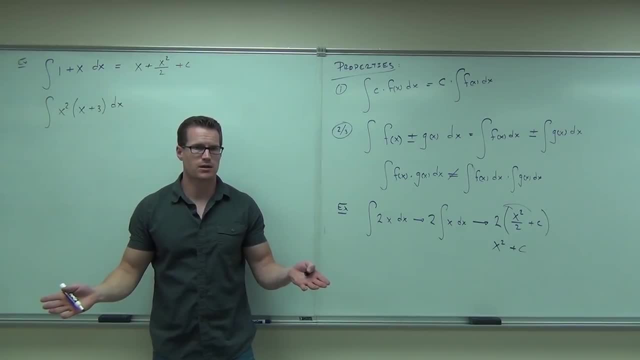 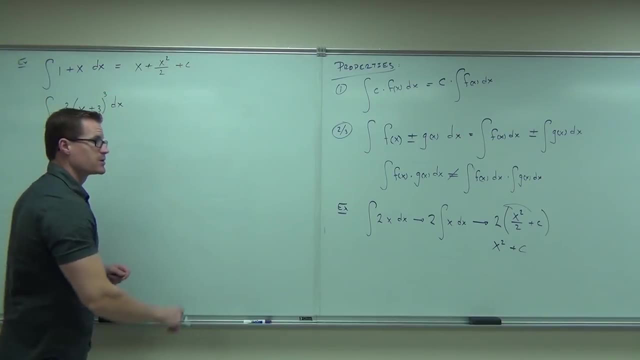 Distribute, Distribute, You could distribute. That would save all your problems right Now. you could do that with that. all right, You can't do that, That wouldn't be possible. But I'm going to show you ways that on certain cases. 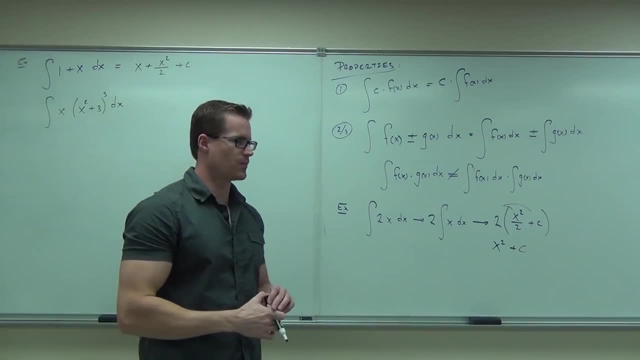 like this one. I will show you how to do that particular example. all right, Some integrals are going to be off limits for us in this class. You get that 4B, But a lot of them we're going to be able to do. 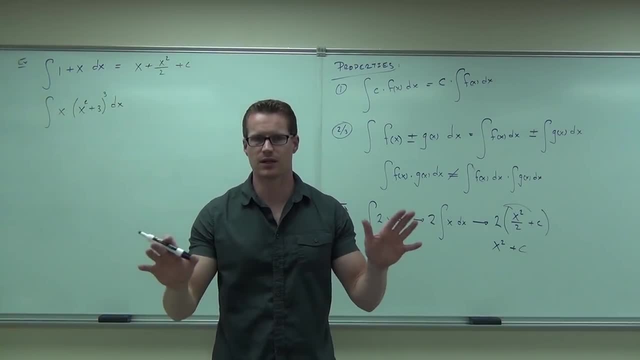 But they must absolutely, with everything else failing, fit your integration table. They have to do that. So, whether you need to distribute, whether you need to do something else with it, make it fit your table somehow. That's the only way this stuff works. 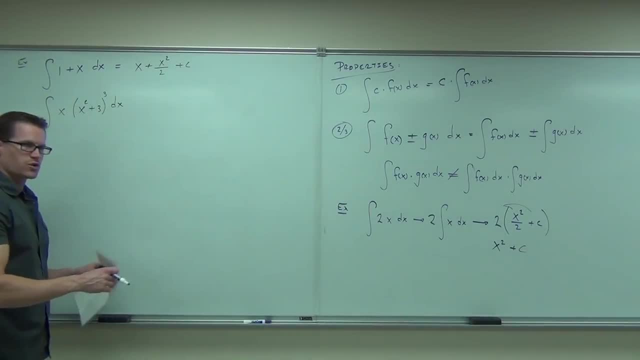 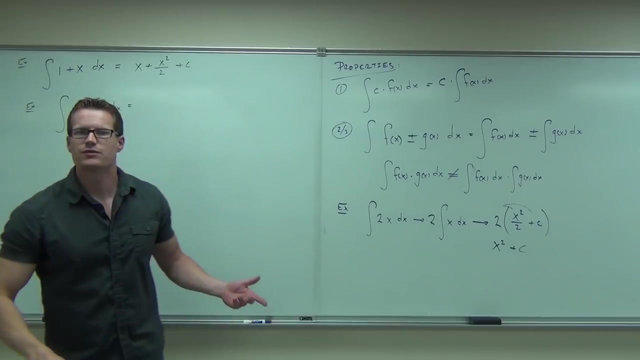 Still okay, Shall we try a couple more and then call it a day. Yes, So that one we can't do yet. Integral of 4, cosine x, dx. let's see what do you do with the 4? Constants. we often do that. 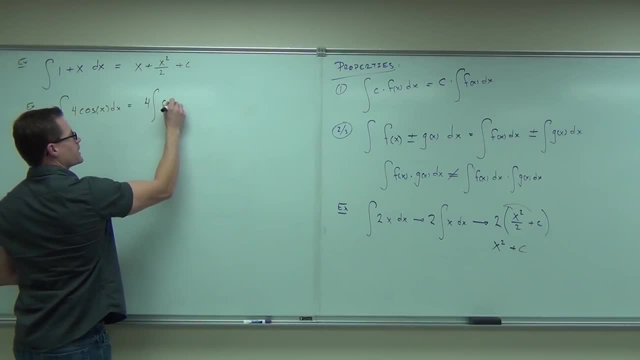 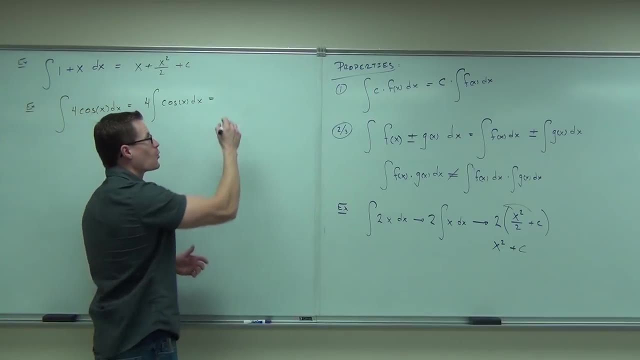 We really do. We say this is 4 times the integral of cosine x- dx. That makes it fit our table. That's easier to recognize. Just don't forget about the 4.. You've got the 4.. The 4 should be there, being multiplied. 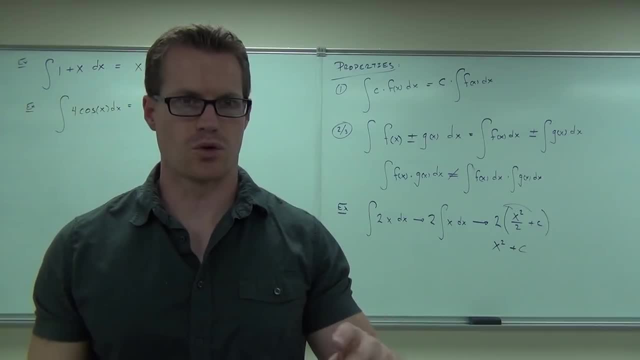 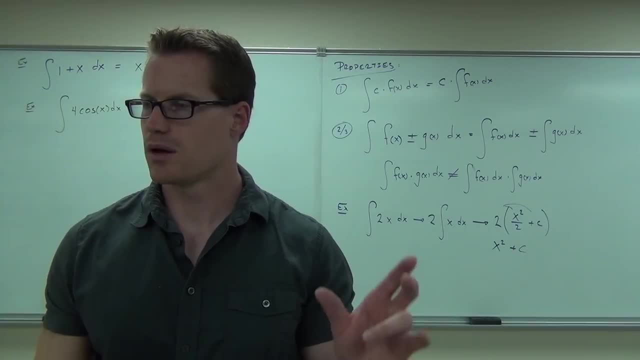 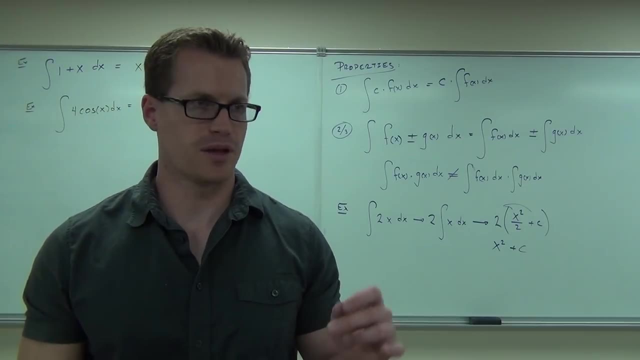 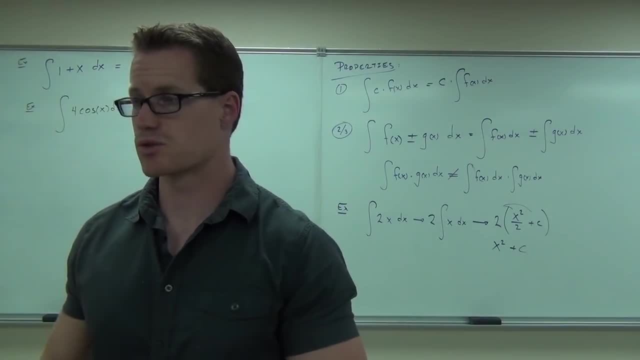 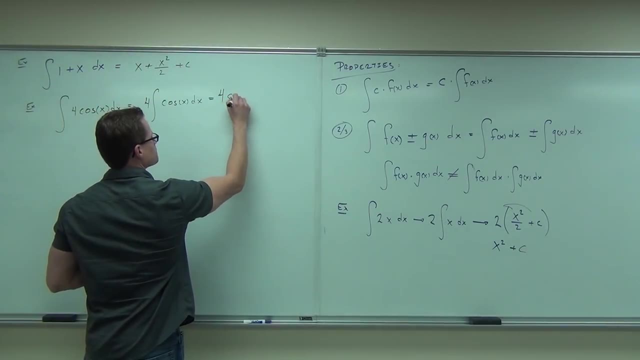 When you take a derivative of it, does it give you positive cosine x? Because that's what you're looking for, Was it sine x or negative sine x, Positive sine x. Remember you can always check your work. No sense in getting the wrong answer here. 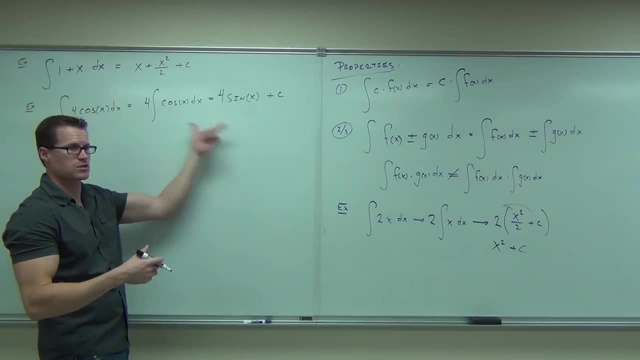 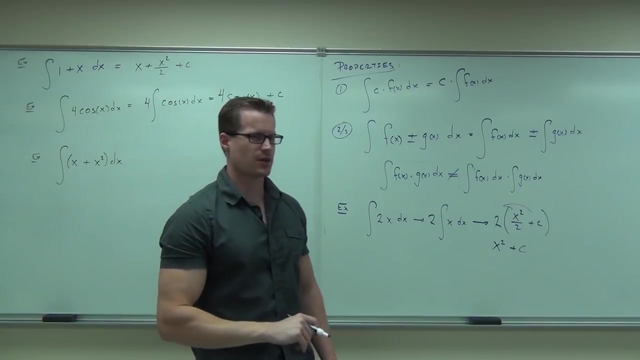 The derivative of sine x is cosine Positive cosine x Positive cosine. that works. That's what you want to get out of that. OK, If you ever see parentheses around that, it doesn't really mean anything special. It just means you're taking the integral of the entire thing. 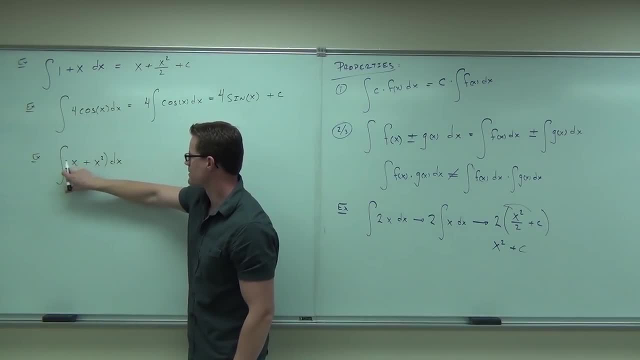 So this basically means the same thing as what I've been writing, as this: Those parentheses just say everything's included in that. Do you see the difference there? There's really no, There's no. It's just grouping them, It's just saying this integral of the entire thing. 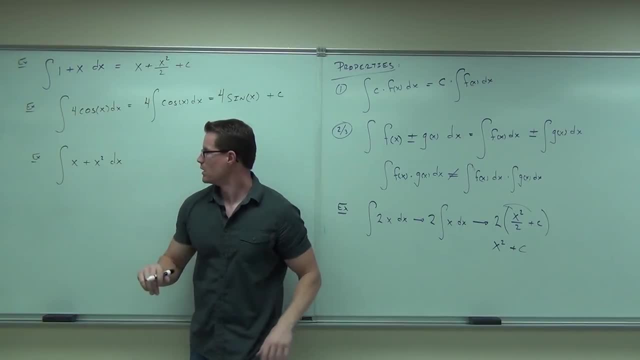 it's not making anything special. no special multiplication or whatnot. Can you take the integral of x? Do that now on your own. Take the integral of x, Write that out, Just do it. You don't have to say it. 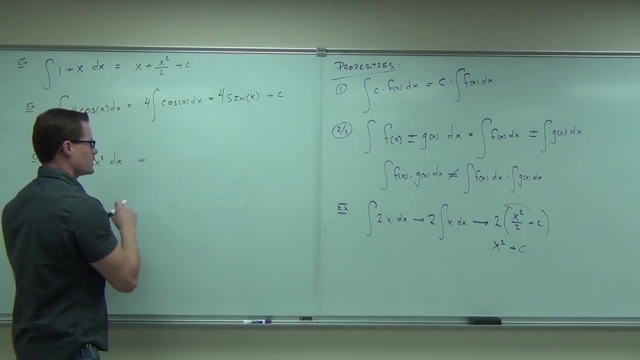 Just write it out: Integral of x is 1. True or false? False, What is it? 1 half x squared. You can write 1 half x squared or you can do x squared over: 2. Plus, Plus, Plus. 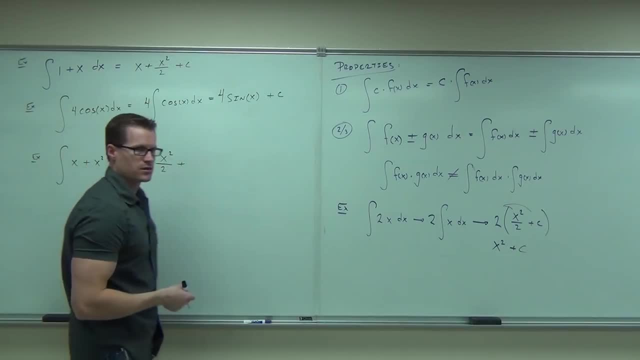 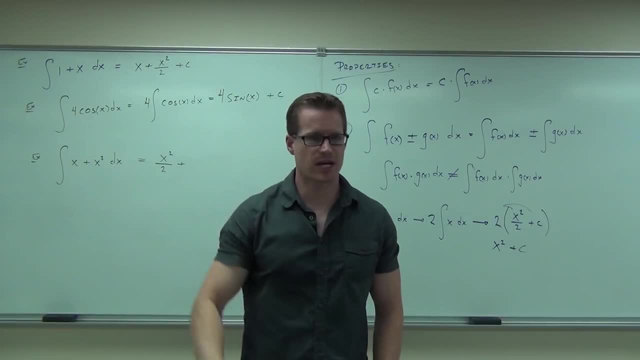 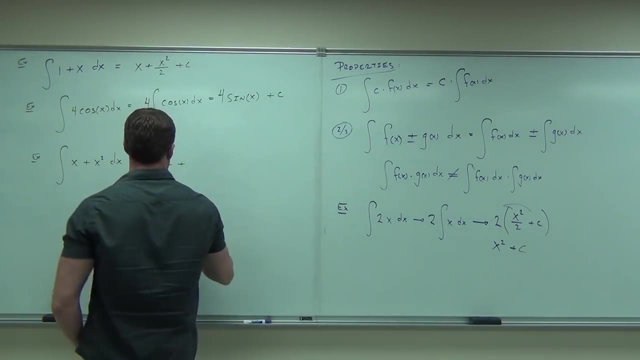 if they're being added or subtracted. Not multiply, divide it, but add and subtract it. Integral of x squared- What's that? I'm going to assume your mumblings were x cubed over 3.. I think some of you said that actually. 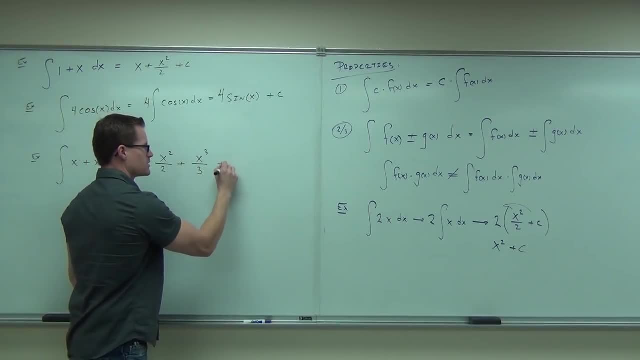 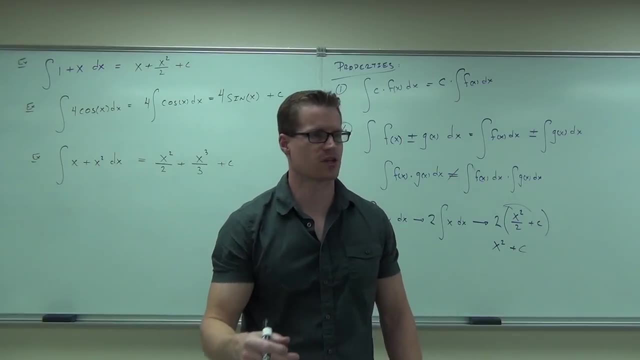 And then what? No two, c's just plus. That's all we want. That's pretty much it. How many people understand the basic idea of integrals? We're going to practice a whole lot more of this. I'll show you things we can and can't do next time. 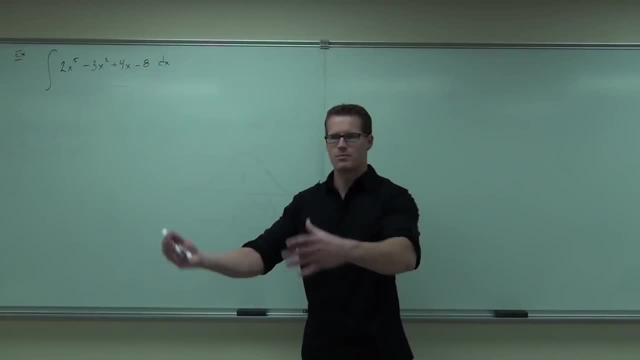 All right. So we're still doing some integrals, our anti-differentiation going backwards from a derivative, backwards of what a derivative is. So let's go ahead and talk about that problem. That's what we're going to start off with. 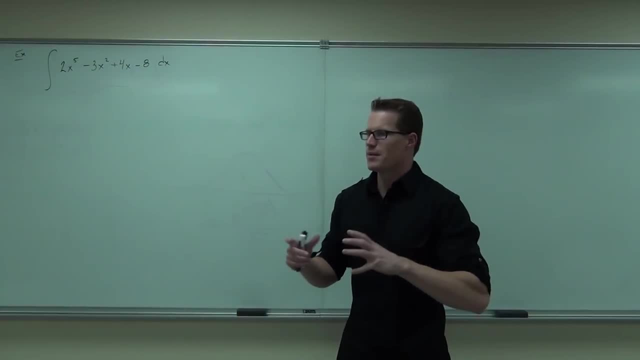 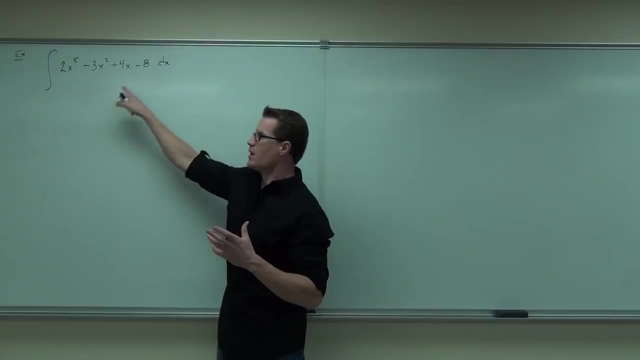 so you get our brains a little motivated. When it says an integral, that means find the anti-derivative of whatever function in terms of this variable that I give you. So this says with respect to x, so our function has to be in terms of x. 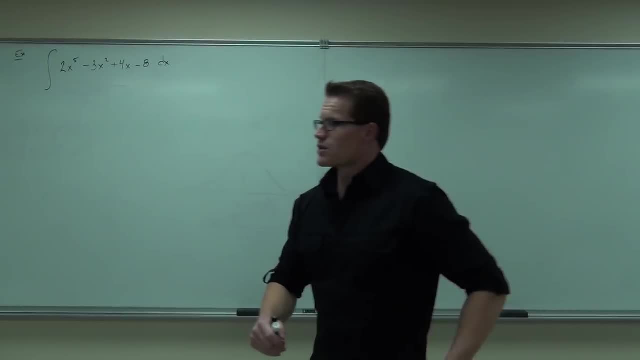 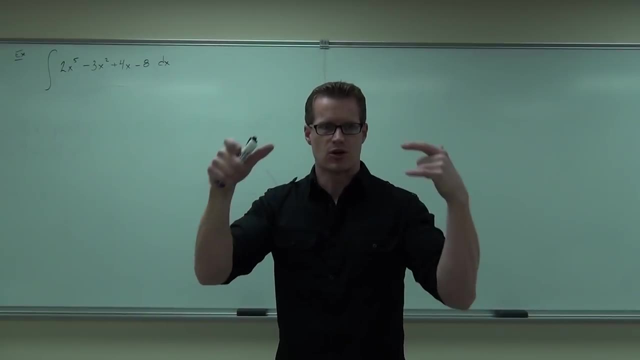 That's what we're integrating with respect to. So when we have 2x to the fifth minus 3x squared, plus 4x minus 8, do I have to necessarily split that up term by term, or can I just find the integral of each little piece? 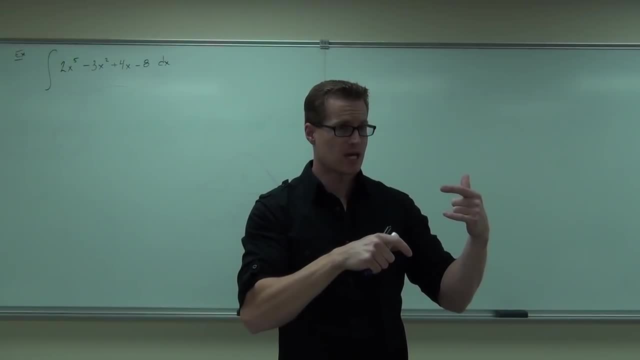 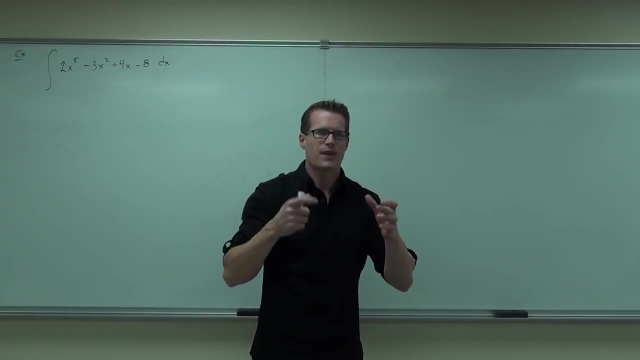 With addition and subtraction, each little piece is fine. With multiplication, division, each little piece is not fine. We knew that integrals, just like derivatives, were separable by addition and subtraction. What that says is: it allows you to do the integral of this piece. 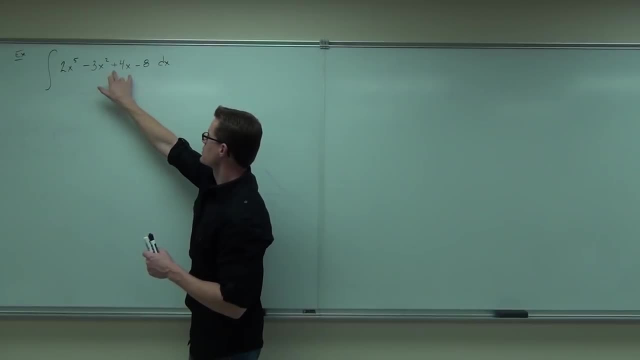 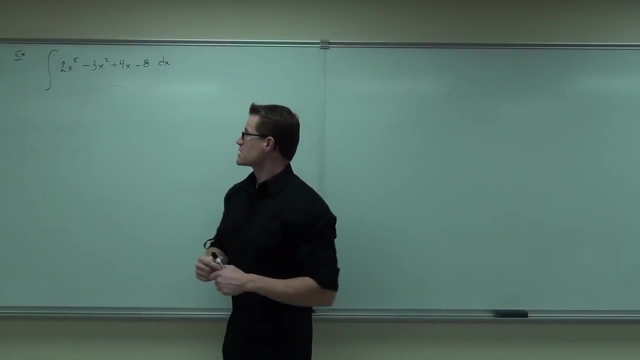 minus the integral of this piece, plus the integral of this piece, minus the integral of this piece, and then jam it all back together. You follow me on that. Let's go ahead and let's take this integral: What's the integral of 2x to the fifth? 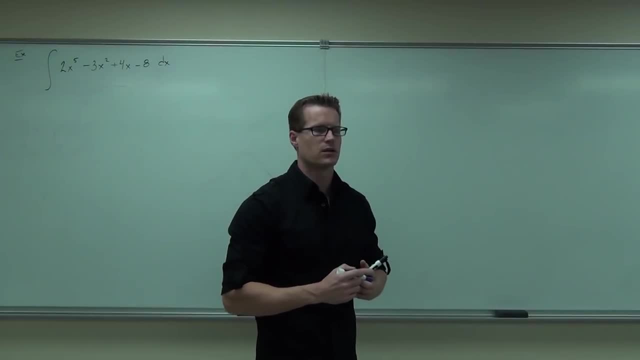 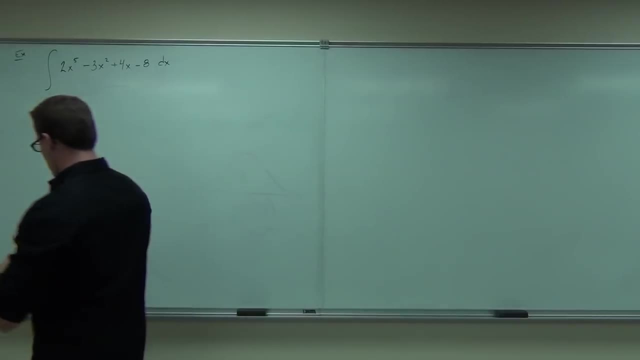 Can you tell me x to the tenth over 10.. Oh no, not quite 2.. 2 times the tenth over x is 2.. Okay, Is the 2 still going to be there? No, Well, you're going to reduce it out. 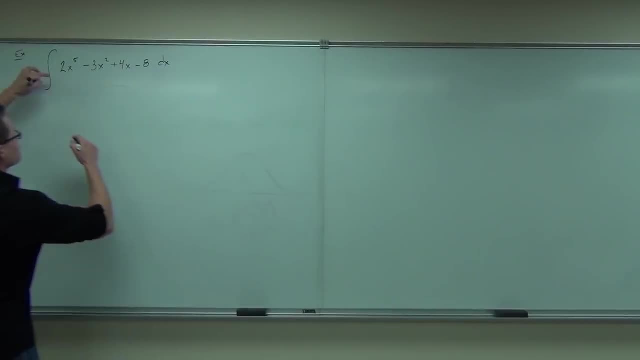 Okay, but is it going to be there when we start? Let's do that, This little piece, that 2 is a constant, right, When we take an integral, just like a derivative, the constant doesn't do much. In fact, if you were to break this up, 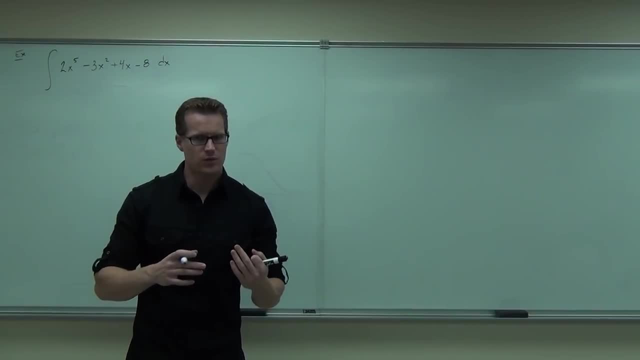 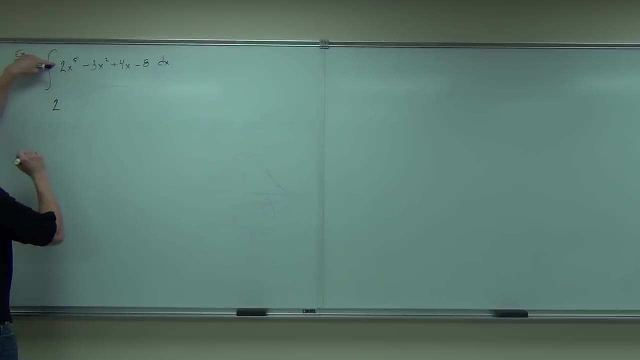 you'd write your constant in front of your integral. Now we're a little beyond that. We just do the integral as we did derivatives. We look at it and do it piece by piece. So we say this is a 2. No problem. 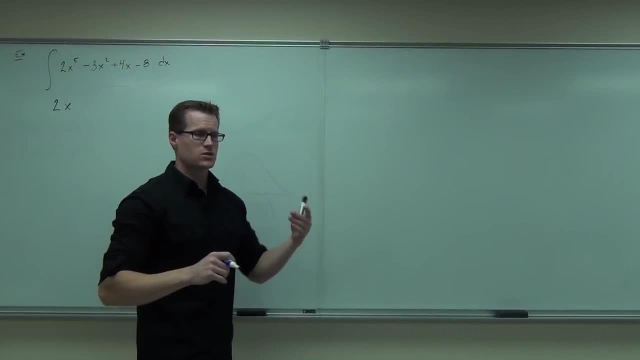 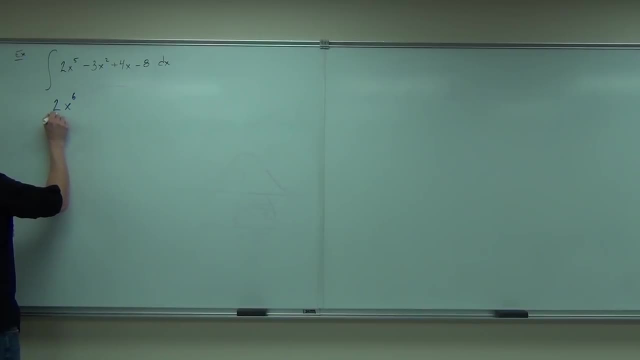 The x to the fifth. what's the x to the fifth become x to the fourth or x to the sixth? y, sixth, Yeah, Over what Six? Yes, The new exponent is what you divide by. So we're going to get 2x to the sixth over the sixth. 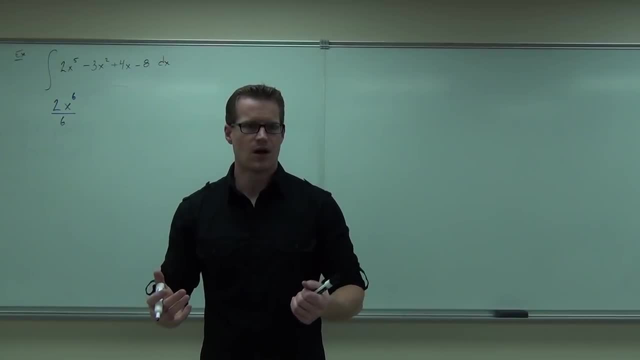 before we start simplifying, Are you following me on this so far? Again, you know what. It's probably useful to check this with a derivative at some point. If you took a derivative here, notice you're going to get 2x to the fifth. 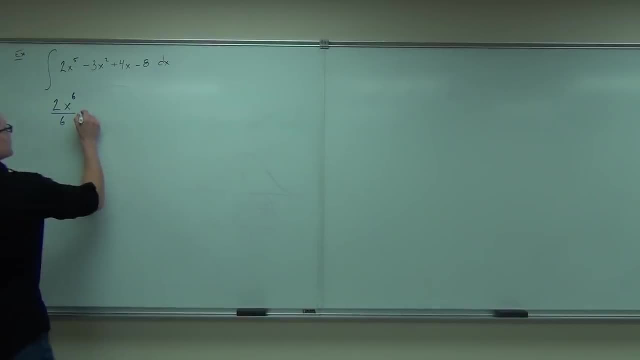 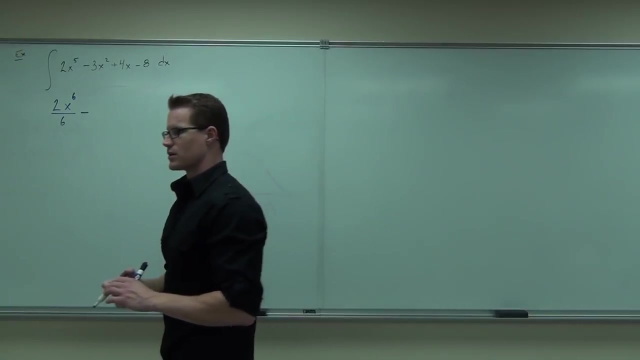 That's nice. You can check that. Make sure you have this right. Minus, Let's do the next piece. How about 3x squared? What's the integral of 3x squared? Okay, I like the way you said. 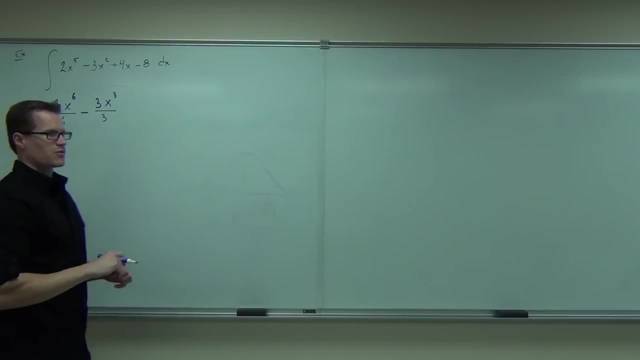 3x to the third over 3, because I'm going to simplify it in a moment. I'm going to write out the integrals just like they are and then I'll simplify it just a bit. We okay so far, Plus, plus what? 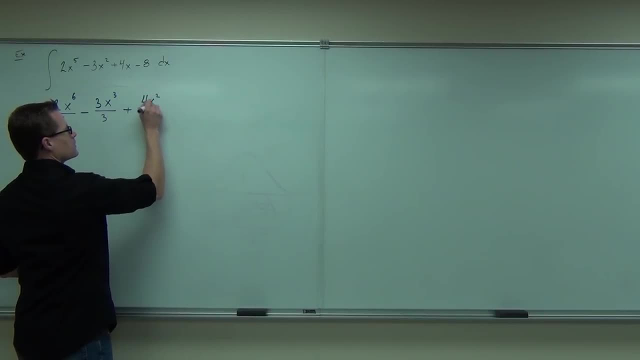 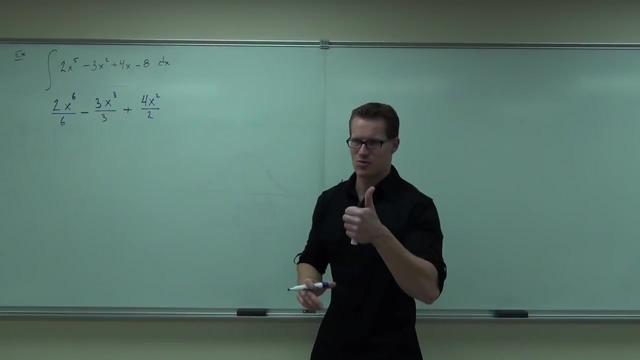 Very good, You sound like my little drums today. 4x squared over 2, that's good, No emotion, but at least you're right, Fantastic. And then the minus 8 goes to 0, right, Because all constants go to. oh wait, 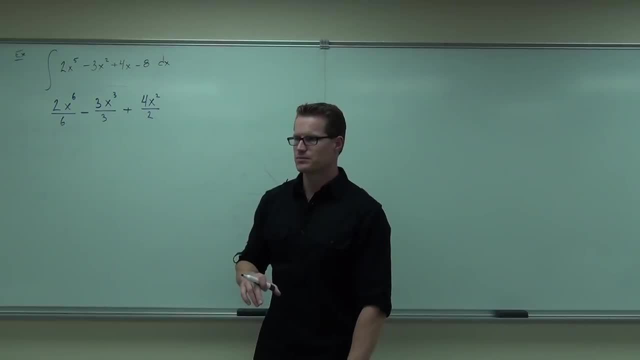 No, When do constants go to 0?? We're not doing derivatives, We're going backwards with that. So if a constant goes to 0 in a derivative, a constant goes with an x in an integral, So this goes minus 8x. 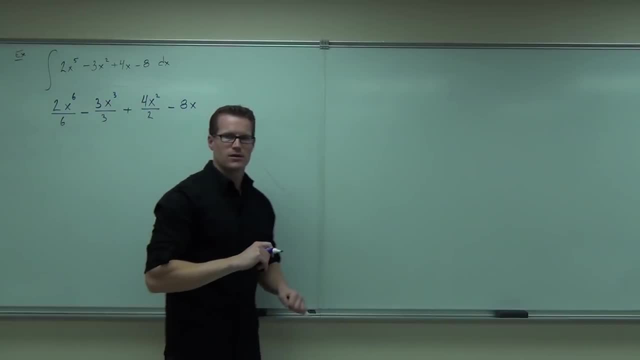 And that's it right. Over 1.. Over 1, I guess you could if you really wanted to. We don't need to show the over 1. But we are missing something very crucial: Plus c, Plus c, mm-hmm. 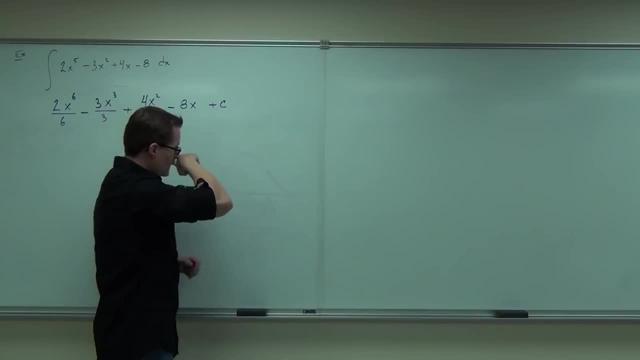 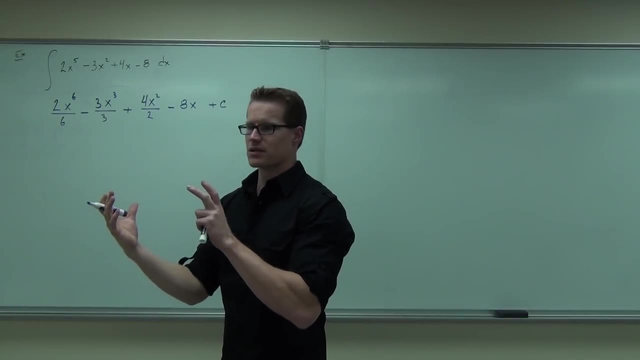 Yeah, plus c is important. Again, what we're finding is a family of curves or, I'm sorry, a family of area curves. basically, from this, This is a family of all the curves, such that when I take a derivative of it, it'll give me that. 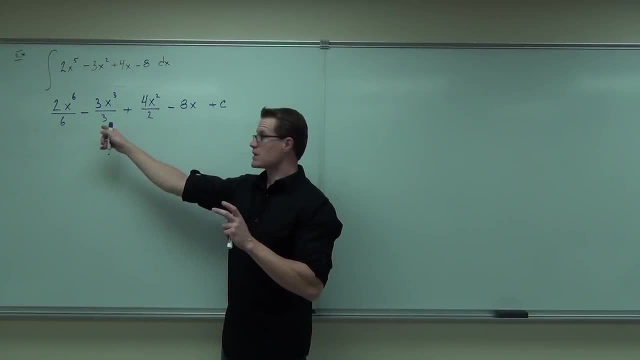 That's what we're talking about. Are you with me? By the way, if you take a derivative of this, will it give you that? Certainly, That's how we found this in the first place. That's why it's called the antiderivative. 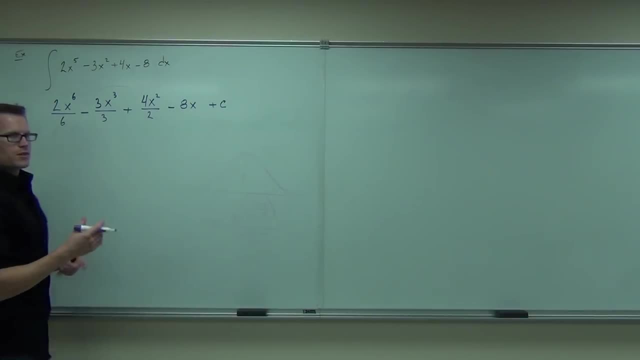 Now we're going to simplify it a little bit. Some of you already told me This is one thing: One-third x to the 6th or x to the 6th over 3.. Minus x cubed, plus 2x squared, minus 8x plus c. 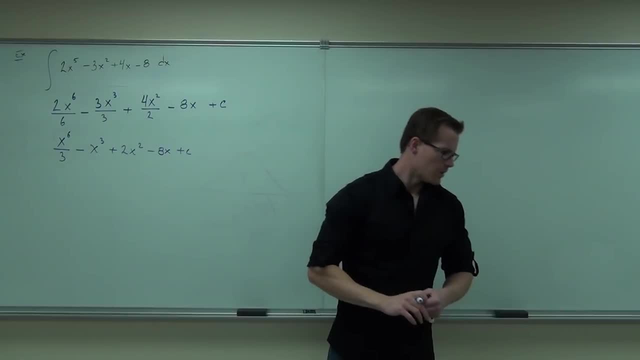 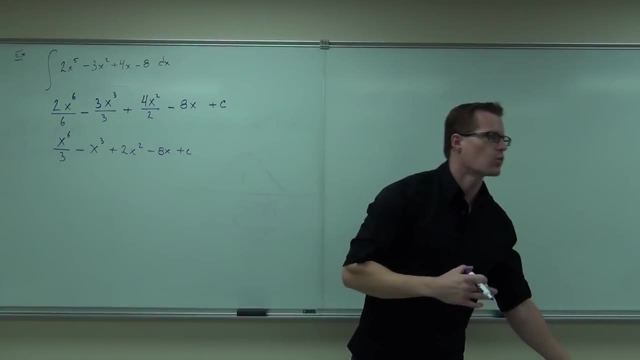 That's our, that is our integral. Can I show my hands, Tell me if you're okay with this example? Kind of a basic example, right, Not too bad. I am going to show you some ones that you do have to do some work to. 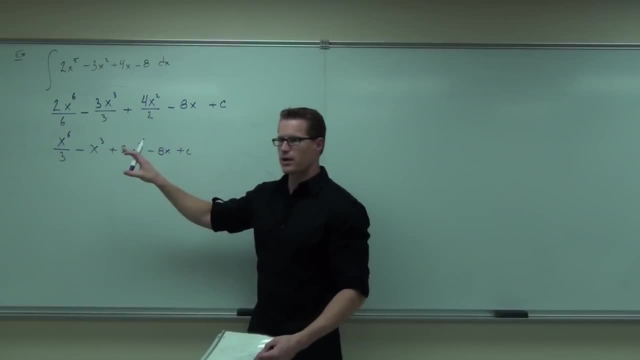 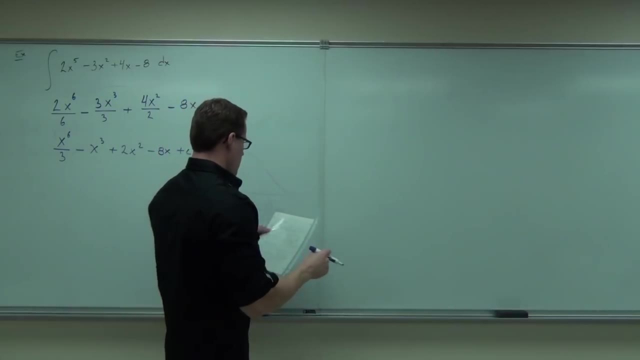 This one was nice because everything fit in our integration table right away, But there are some cases where that is not true, So we'll take. would you like to see a couple of those examples? Yeah, Okay, I think I gave you one last time that I'm not going to give you again. 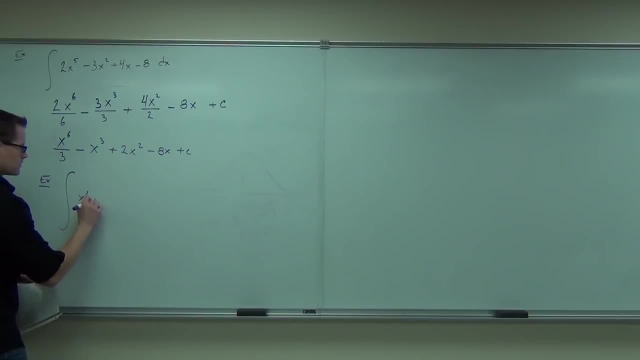 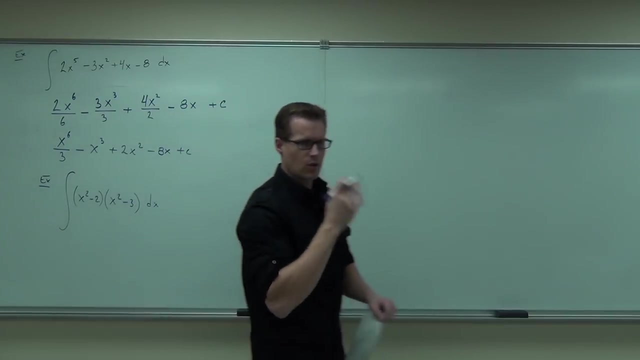 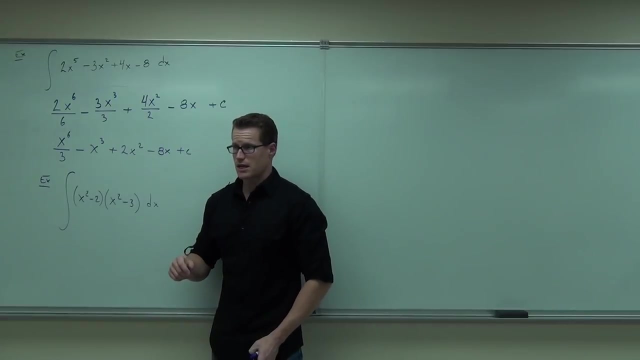 but I want to talk about it Like that. We're not going to go all the way through this, but I want you to look at it. I gave you examples similar to that before. Can I just take an integral of this and an integral of this? 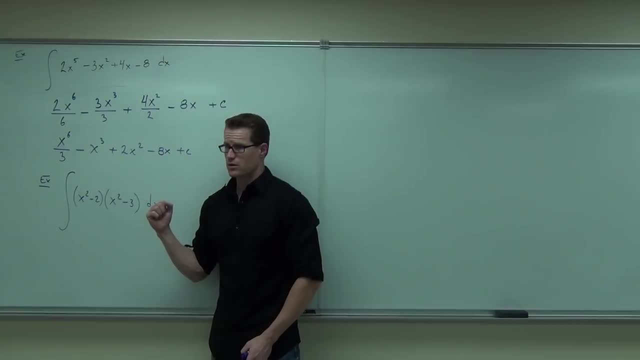 Yeah, Yeah, Yeah, Yeah, Yeah. Can I just take an integral of this and multiply it together? Does that work? No, No, It only works. separation by addition, subtraction. So if I gave you this problem, what's the only way you have to do it right now? 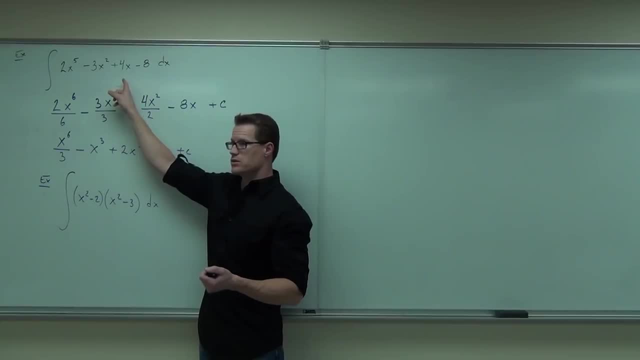 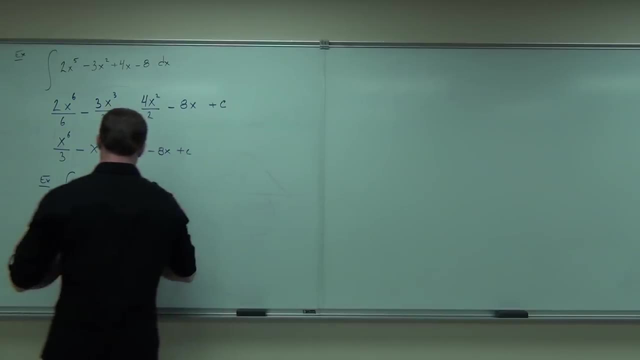 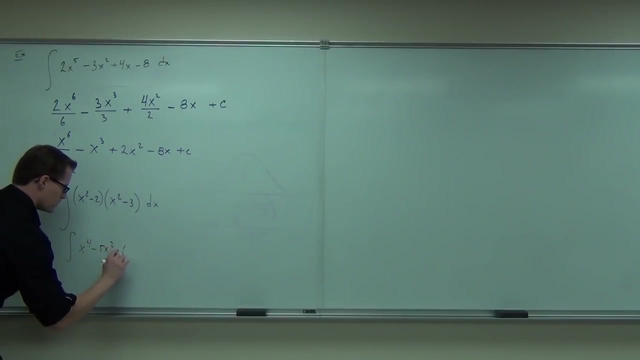 Distribute it, Distribute it, Distribute. Make it look like this, and then you can do it. Does that make sense? You get like x to the fourth minus 5x, squared plus 6. At least I hope so. I guess we can go all the way through it. 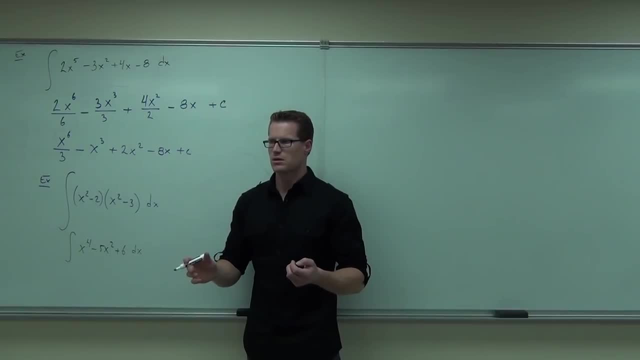 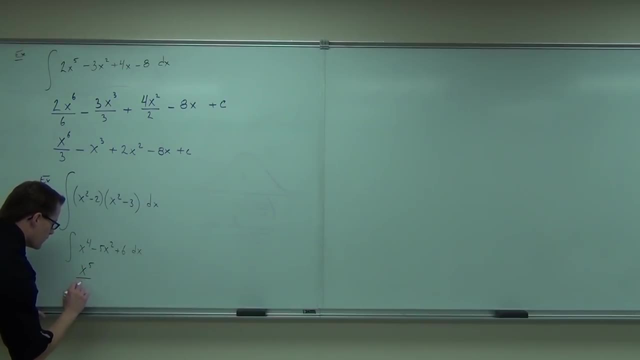 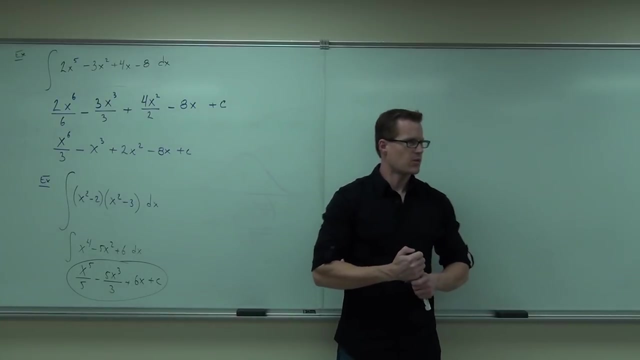 It's not that hard, But once you do, do you see the distribution there? Once you distribute, then you can take an integral. It's fairly easy after that. That's what we're going to get You. okay on that one. 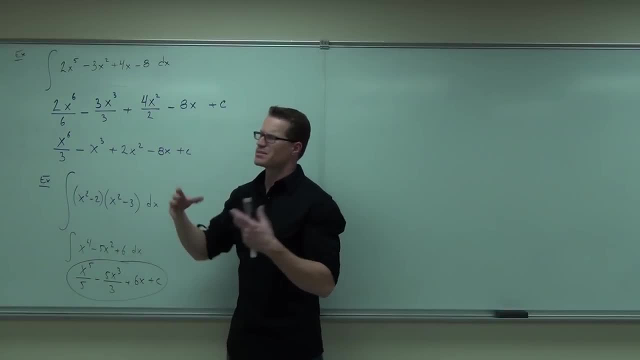 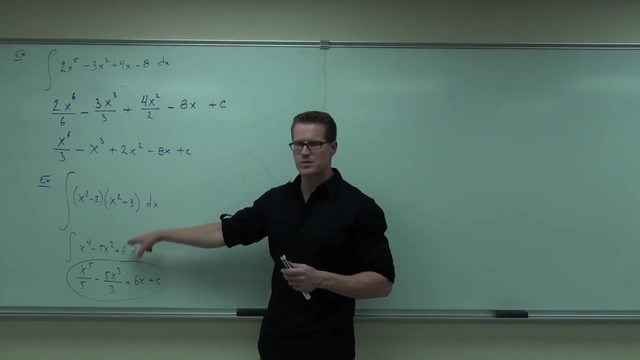 So, even if it doesn't look exactly like this, sometimes you can make it look like that by some distribution Or some working with our fractions Or manipulating some trig functions- We'll see that on the next one. Are there any questions on this particular one? 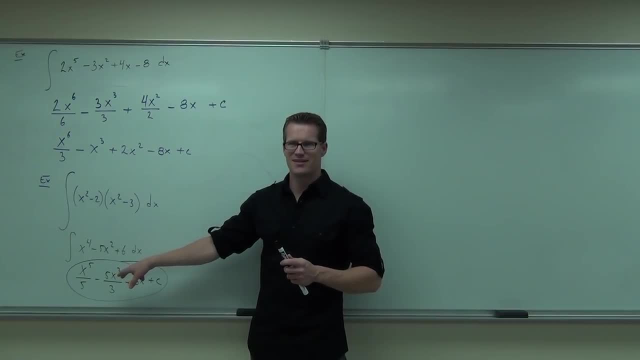 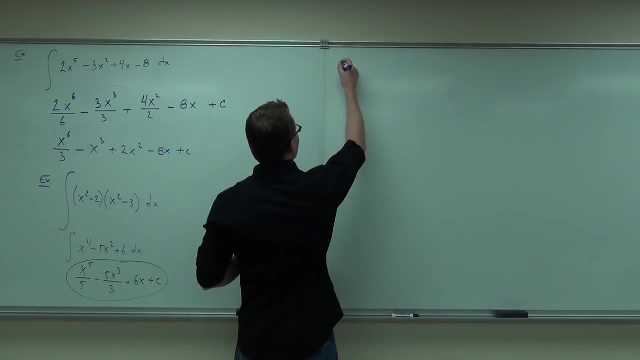 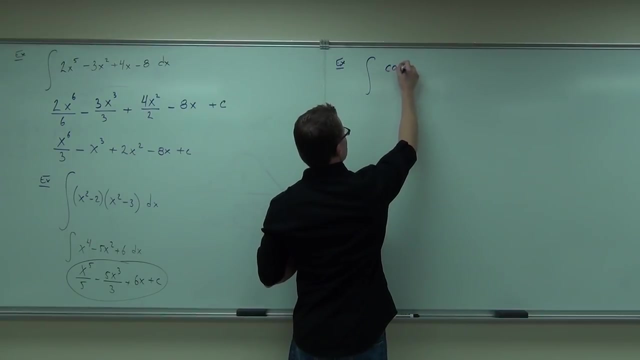 You guys alive today out there? Oh yes, Okay, You're freaking me out. Do you remember me telling you that with your integrals, they absolutely must be exactly the same, Exactly like on an integration table, Or otherwise you cannot do it. 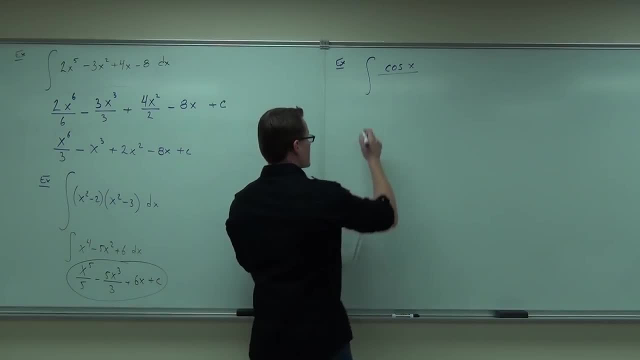 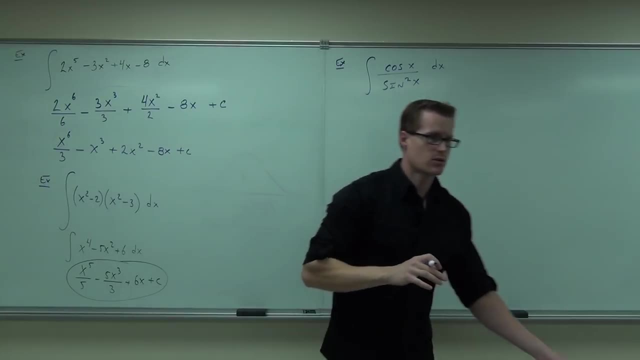 That was not a lie. Okay, That's a true statement. So when I give you something like this, is that right there on your integration table? Then you can't do it the way it is. That means you have to manipulate it somehow. 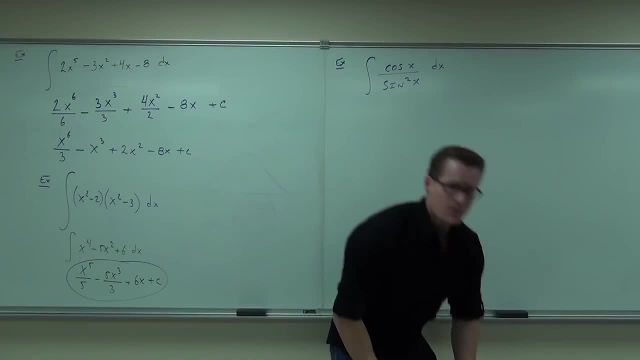 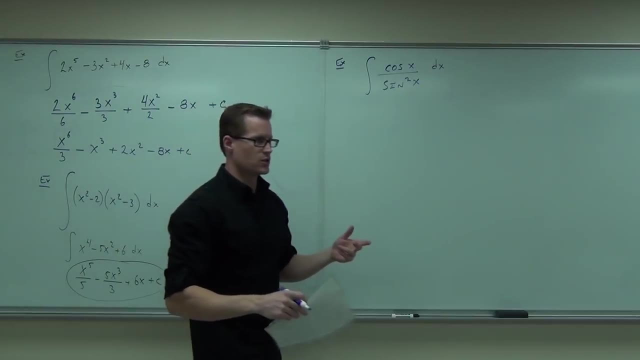 So when we look at this, what we're constantly trying to do is somehow figure a way to make this fit something on our integration table. That's the idea. These fit because they're polynomials. They're very easy to do With trig functions. they've got to match exactly. 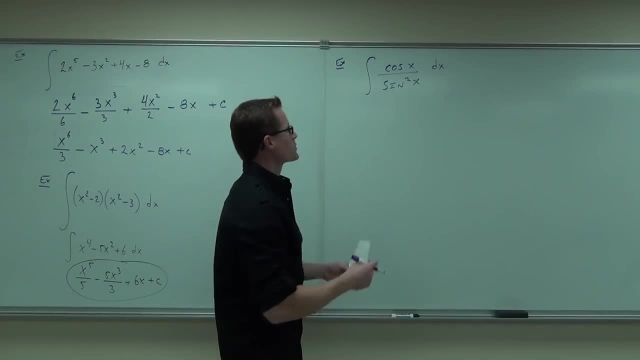 Well, you can't even be missing a little piece. We've got to make them match up. So when you're dealing with things like this, it's often nice to break them up and see if you can manipulate around those trigonometric identities that you know and love. 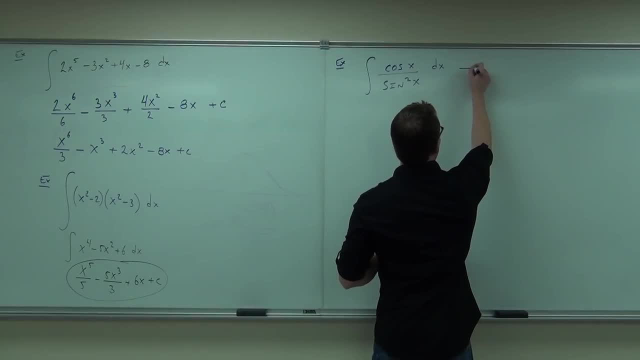 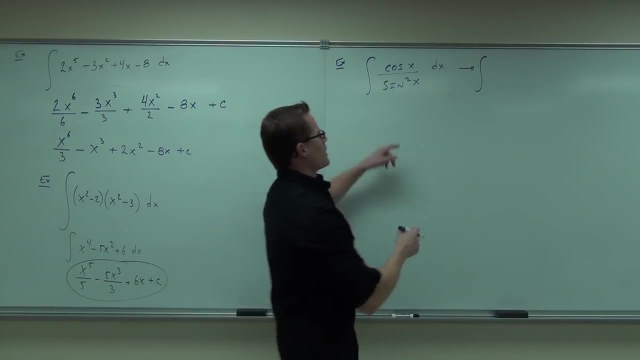 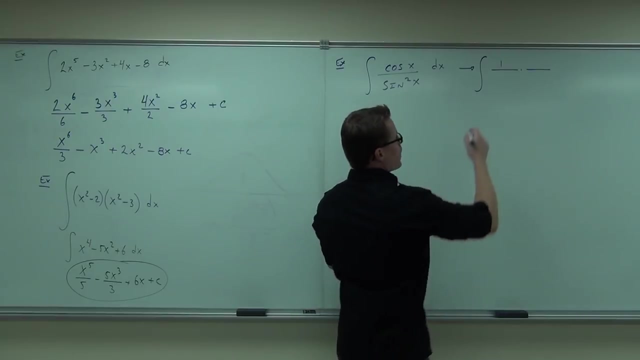 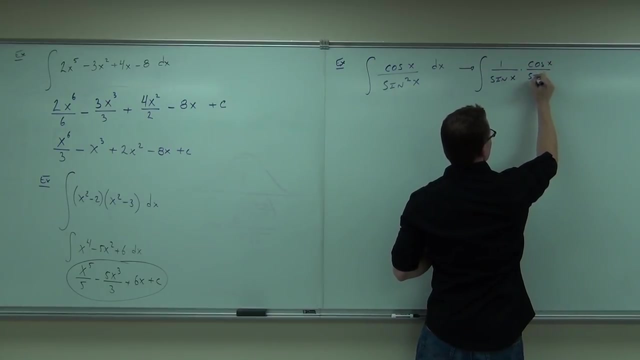 Maybe not love, but at least hopefully know. So, for instance, let me give you a method on how to do some of these. One method would be okay. let's say I split this up as 1 over sine x times cosine x over sine x. 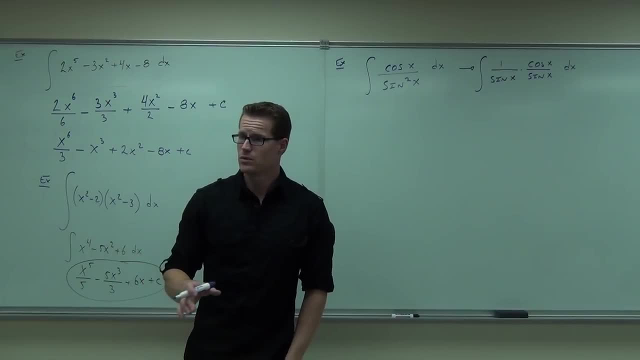 Are we okay on that one? Do you see it's legal to do That's still cosine x over sine squared x, right Now, why am I doing this? Well, firstly, because I'm pretty good at it, right. I know what this is going to be. 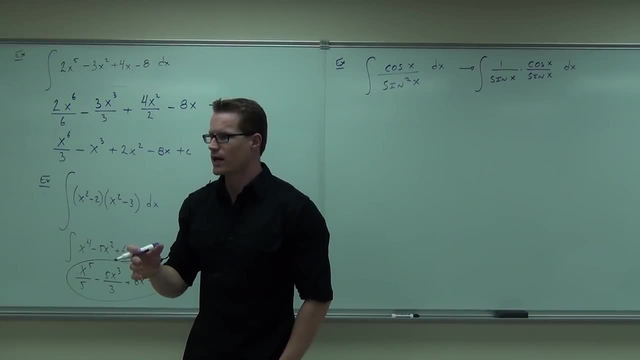 But secondly, because I'm trying to do this, I'm trying to do this, I'm trying to get some other identity, because I know right now, cosine x over sine, squared x, that over, do you see the over? There's nowhere to be found in your integration table, is there? 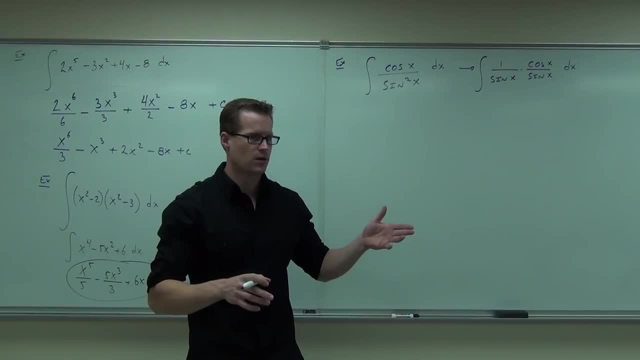 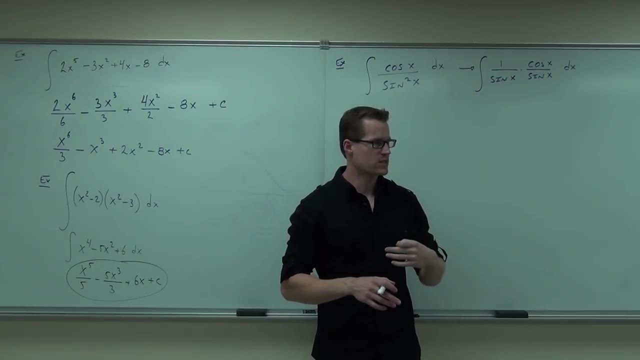 There's no over, There's no fraction on your integration table anywhere, right, But what there is is when you have something over sine and something over sine. you can oftentimes translate those into some other trig identities that might be on your integration table. 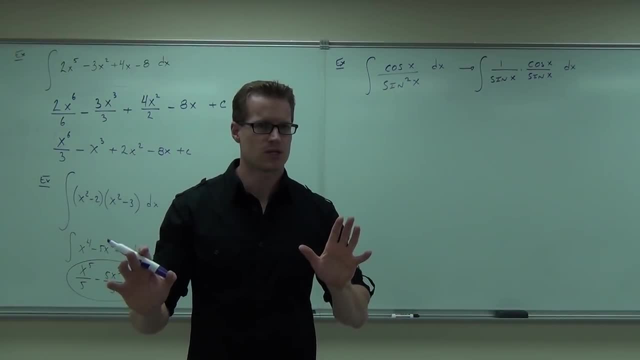 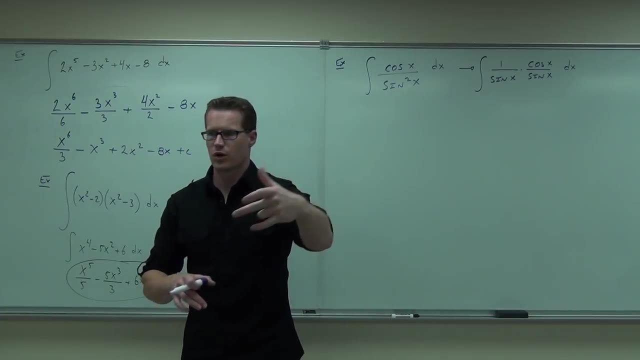 So if you see an over, that's not a good thing for you right now. If you see an over right now and later on, I'll show you something. I'll show you some other ways to go about doing this. Method one is well, manipulate it into something you can work with. 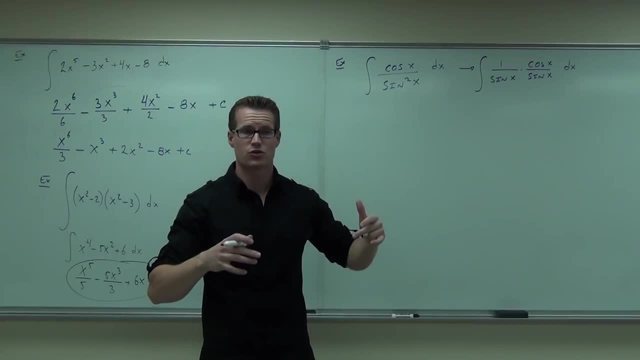 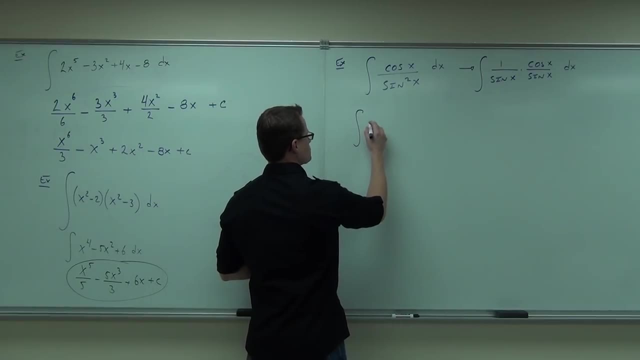 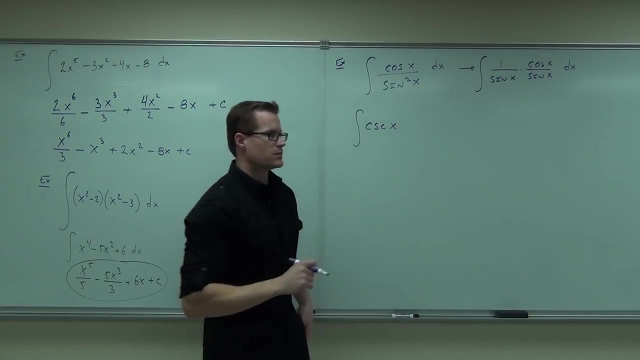 If you have something over sine, over sine, translate that back into a different trig function and then see what you have. What is one over sine? That's cosine times, not tan Cone, Cone, Cone, Cone, Cone, Cone. 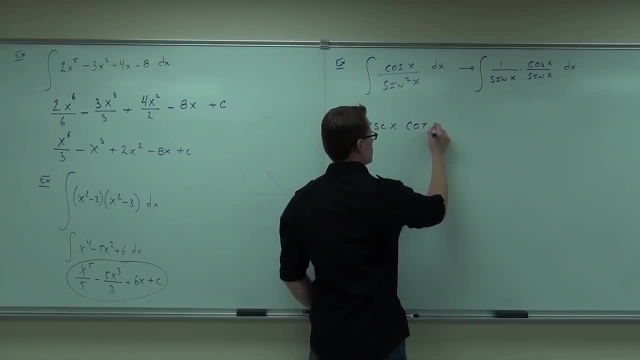 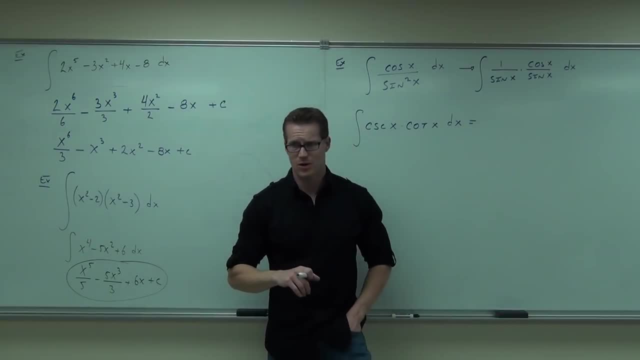 If you haven't memorized that integration table, which I'm guessing you probably haven't in one day- why don't you take out your notes and look at it? Find the integral of cosecant, cotangent. Cosecant x- cotangent x. 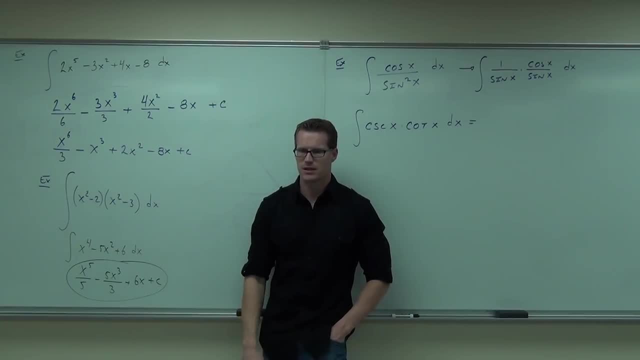 Negative cosecant x plus. I want you all to find it, Get it in your at least, read it on your own, Find it. Reading something like that reinforces the idea even more, besides just hearing it from somebody. So I want you to. 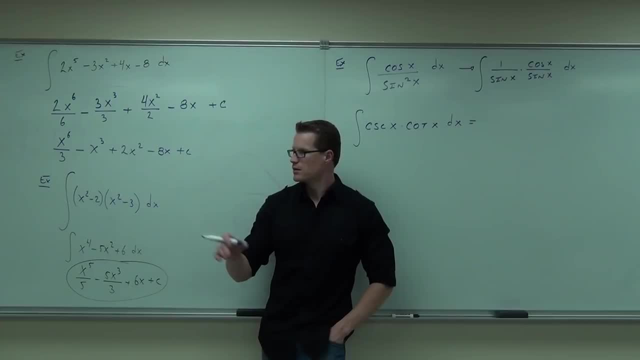 Find it, Look at it and identify that they're right. I wrote them on the board. Oh, They're on the video. They're also in your book, Did you all find it Okay? So, cosecant cotangent, I gave you a nice one, because that's actually in there. 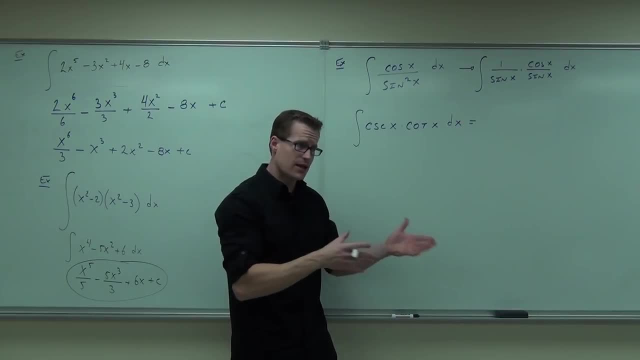 If it wasn't, you wouldn't be able to do it. It has to be there. It has to. So that means you're going to manipulate this around until you find something that's exactly in your table, which I guess is kind of a nice thing, isn't it? 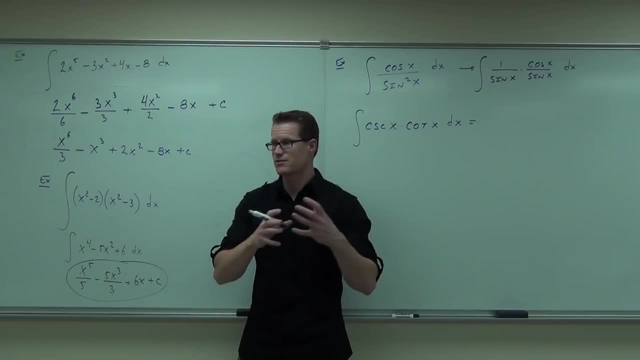 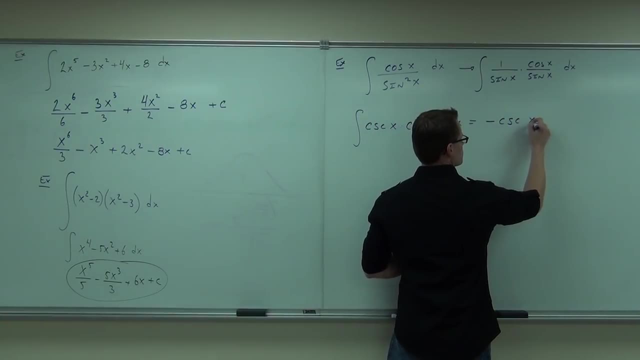 If it's not there, you can't do it. Sometimes, make it, Make it If it's not there, it's barely part of those. So this one you said negative- cosecant X: Yes, Plus, Plus, Plus, Very good. 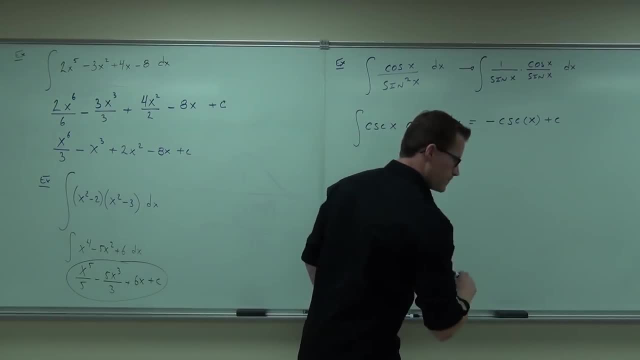 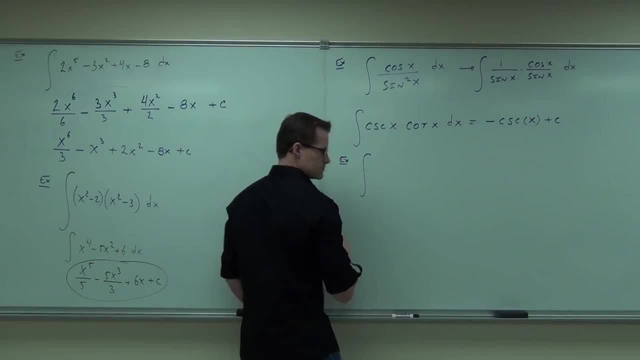 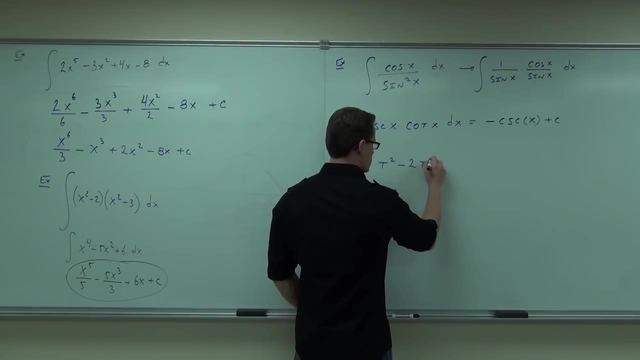 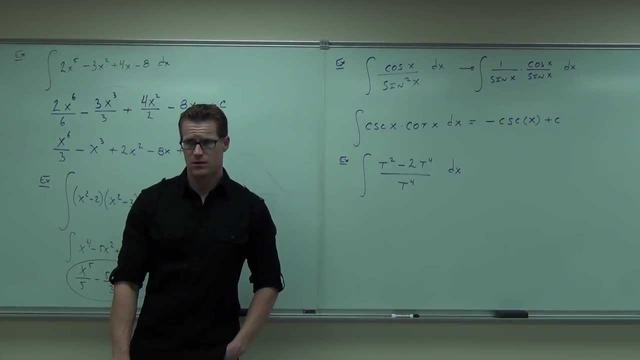 something that is wrong with that integral. right now It's with respect to x, but the variable is t. Say that louder for me. It's with respect to x, but the variable is t. Do you see the discrepancy? If I'm asking you to take an integral with respect to x, my variables have to be x. 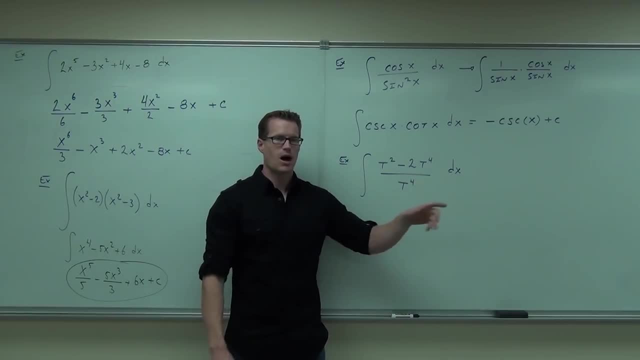 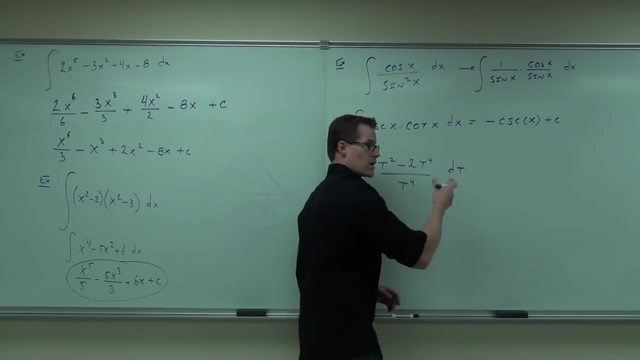 If my variables are t, that needs to be a t. If it's not, then you can't do it the way this is. You have to have that in the same variable. So that's correct. That's fine. Don't forget your dt. 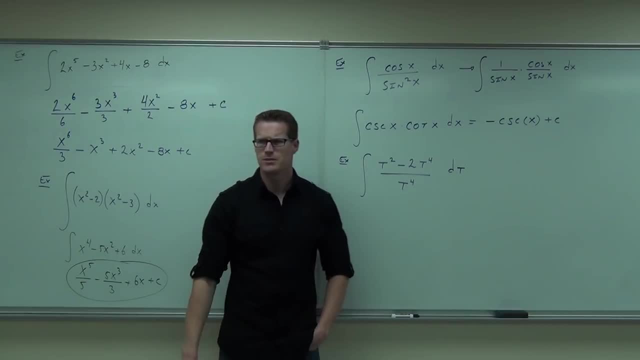 That's important. Now, OMG, is that in my integration table, No, Heavens, no, No, I'm not taking over anything in our integration table, so this can't possibly be. Now one more question: Can I take the integral of this, the integral of this and the integral of that? 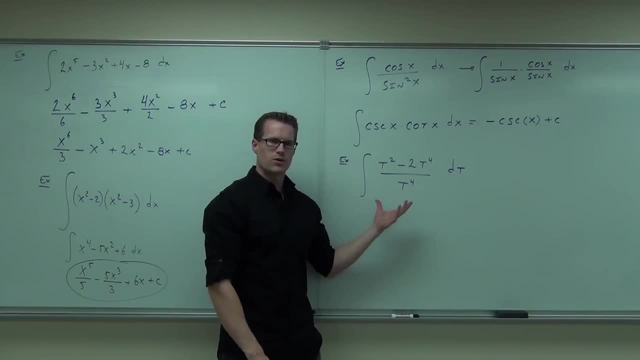 Does that work? No, No. Is there a quotient rule for integration? No, No, Make it fit. Make it fit in your integration table. So manipulate this somehow. Someone on the right-hand side of the room give me an idea about how I can manipulate. 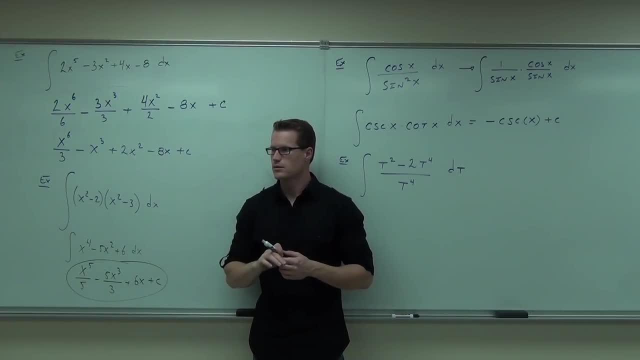 this to make it look. maybe better Say what t to the negative 4.. Okay, I can't quite just move that up there. I can't just move that up there whenever I want to because it's being subtracted, but you're on the right track. 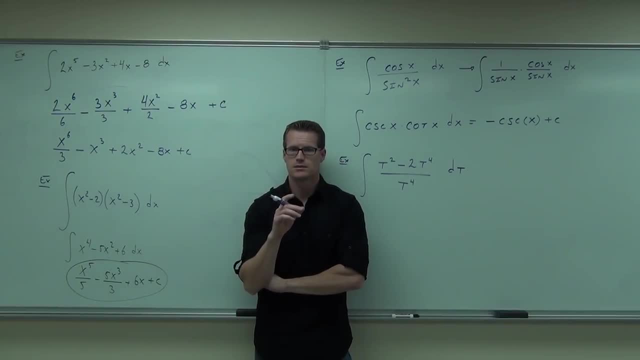 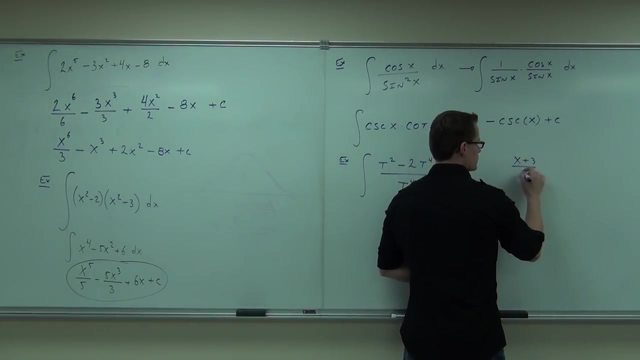 I like the thought. Can you factor stuff out, Factor stuff? What do you mean? factor stuff out Factor, Factor, Factor? Wait, say that again. Break it apart When you deal with things sometimes. it's often nice occasionally to be able to do. 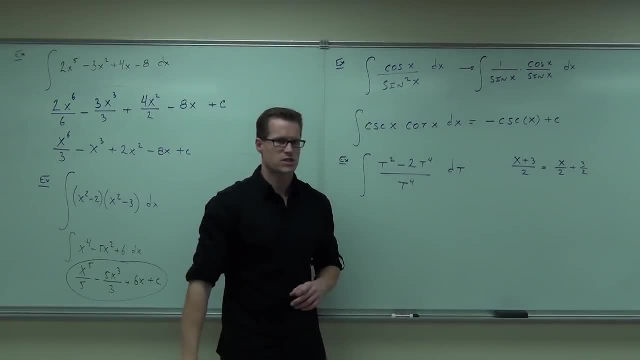 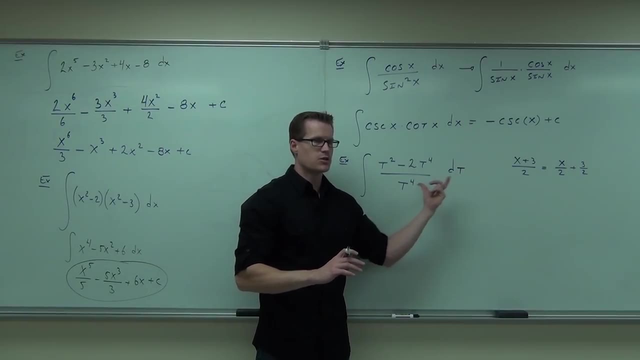 this to it right, Which is a true statement. Notice that if I do that- and this is a very big hint- whenever you have one term on the denominator, that's possible, right, Two terms not possible, But one term, you can always do that. 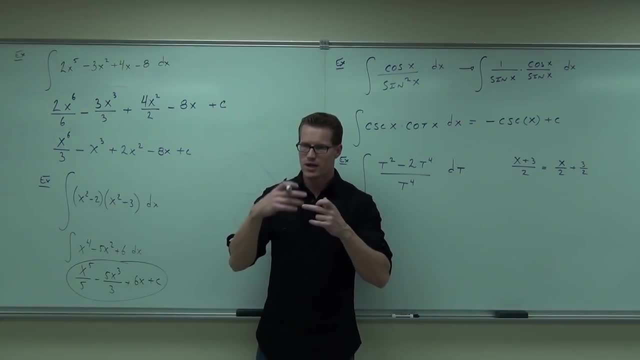 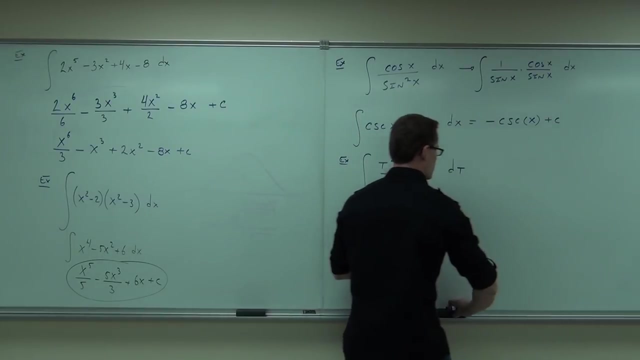 Do you see what I'm talking about? If you break up each individual numerator term over the denominator factor, you get all these different fractions, each of which will be simplifiable, each of one. So yeah, absolutely correct, Let's make this. 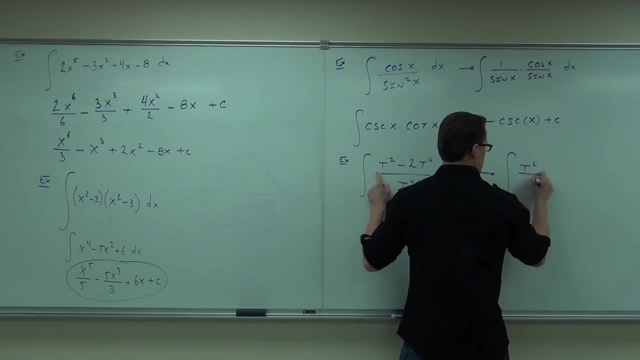 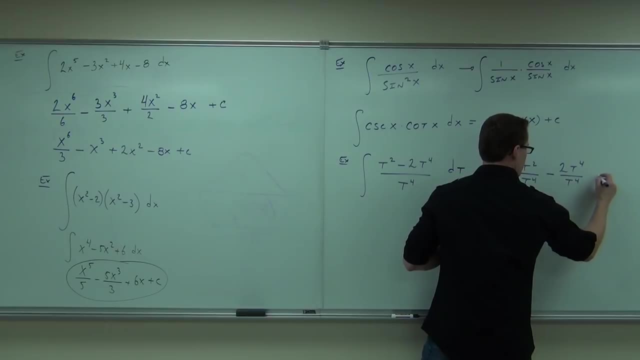 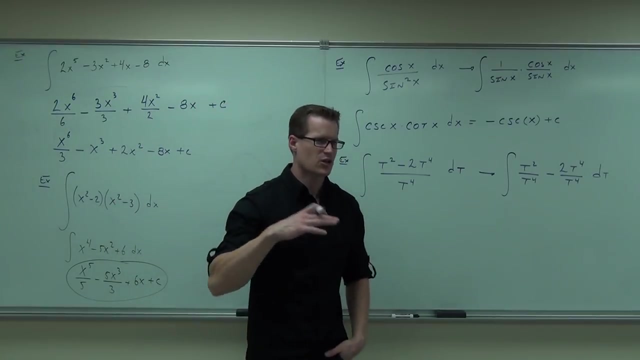 I'll show you every step here. Let's make this simple: Minus t squared over t to the fourth, minus 2t to the fourth over t to the fourth, and there's still a dt. By the way, don't try not to overthink these things. 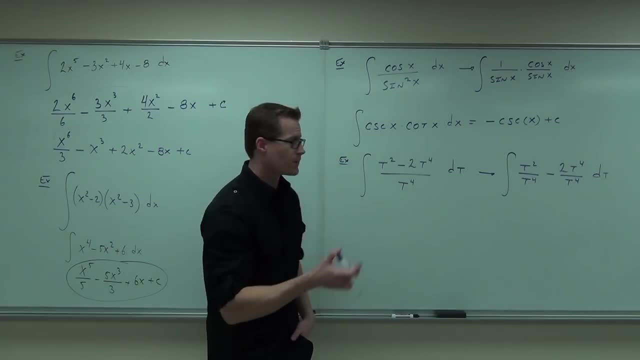 Do the simplest thing that will work, not the hardest thing. Do the simplest thing that will work. That's the simplest thing that's going to work. Why is that the simplest thing that's going to work? I don't know. You tell me. 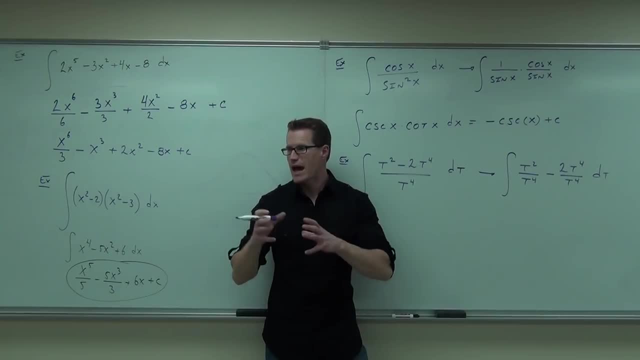 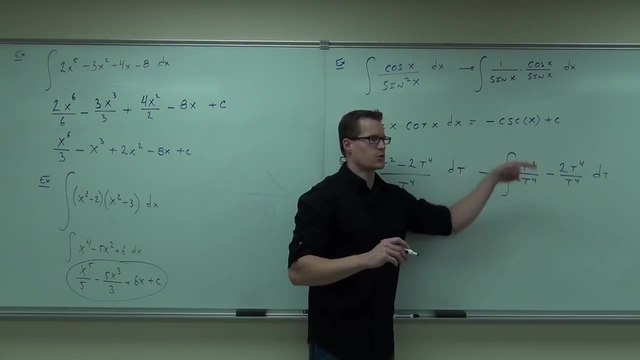 Simplification. Can you simplify each of those fractions? No, Absolutely, And they're not going to have any denominators in here. So when I have t squared over t to the fourth, well, I know that we subtract exponents when I divide like bases. 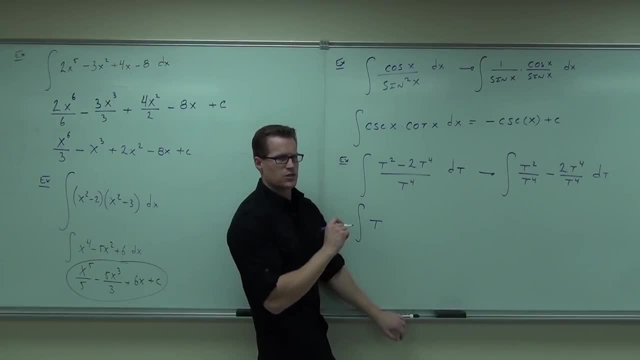 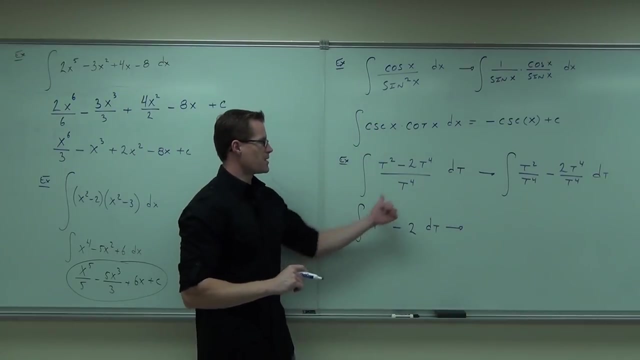 So that's going to give you t, squared t to the negative 2 minus. how about the last one? What was it? Oh, that's great, I love that. Does this look a whole lot better than that one? Yeah, for sure. 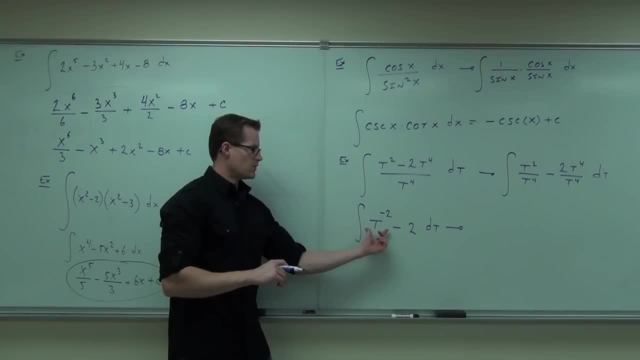 It fits our table. That's what we needed it to do. So let's do the integral of 2, sorry t- to the negative 2 minus 2.. Do it on your own. See what you get out of that, Okay. 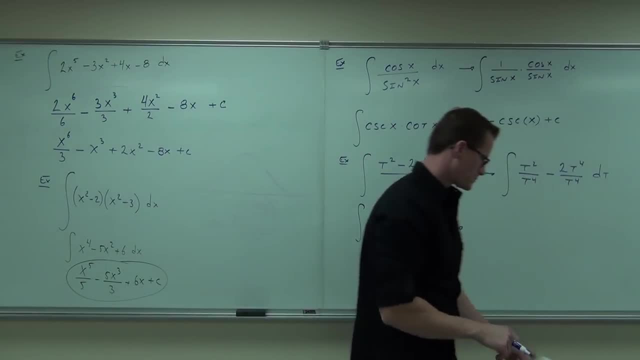 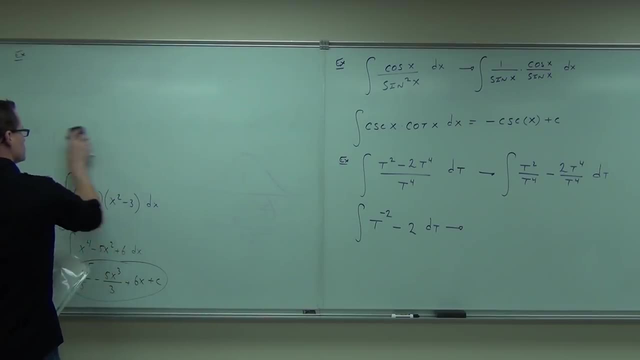 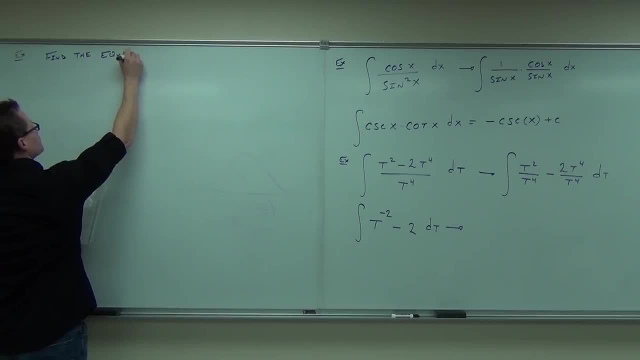 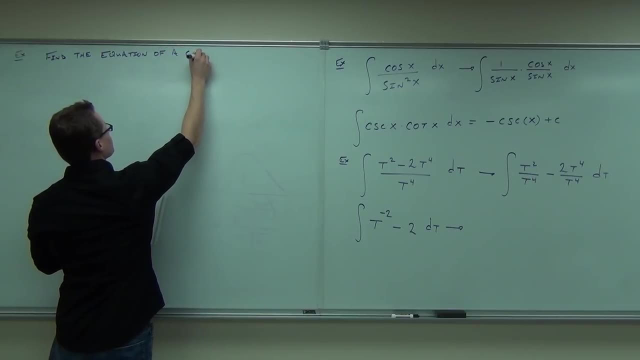 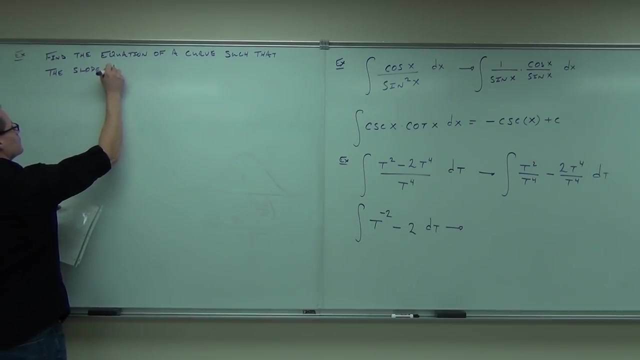 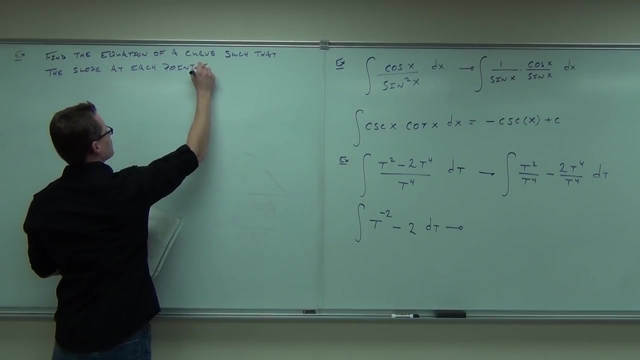 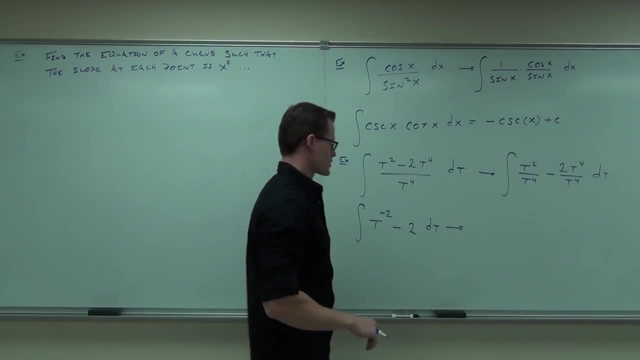 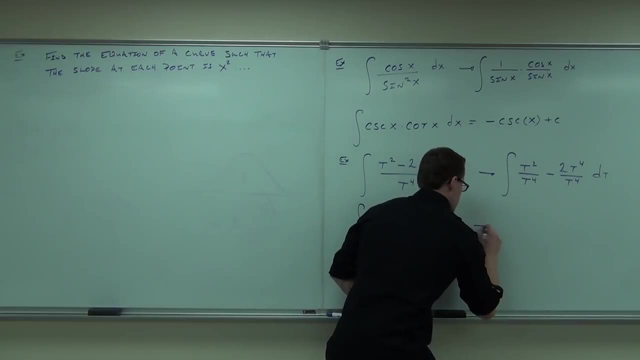 we solve the first part. Before we get there, let's look at this part. We're going to do the integral of t to the negative 2 minus 2, well, hopefully you got t to the. is it negative 3 or negative 1?? 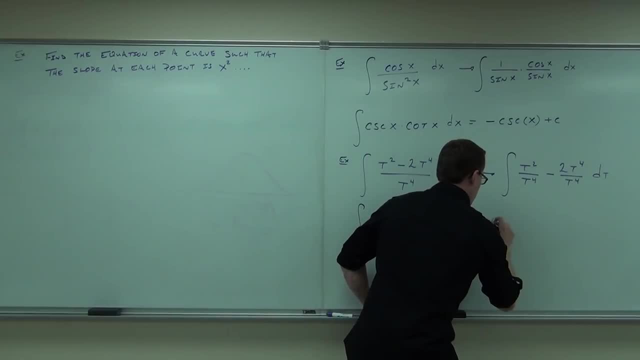 You're adding 1 to it. negative 2 plus 1 is negative 1 over negative 1, did you make it that far? Minus what? 2t, 2t cool, Maybe plus c at the end. 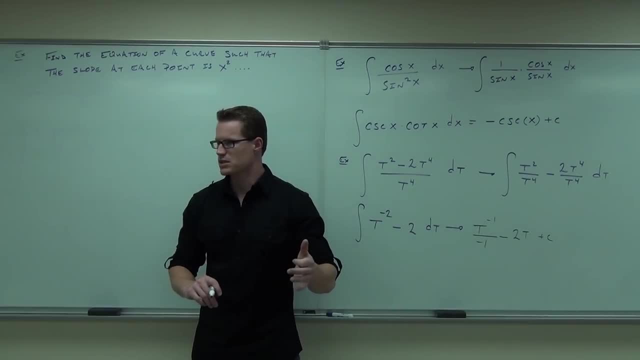 Now you can hold on to the plus c until the very last step if you want to, as long as you have the plus c. We found out that plus c- that's a constant- really doesn't matter where you have it, as long as you have it at the end, it's just a constant. 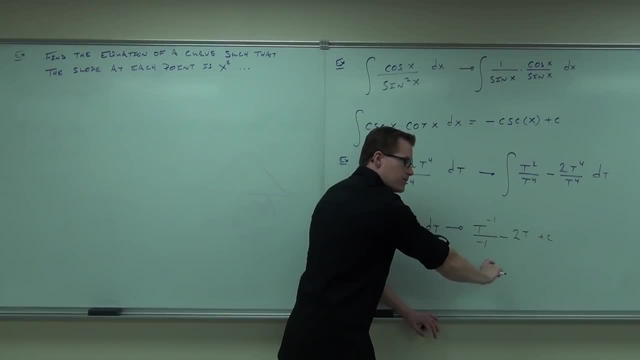 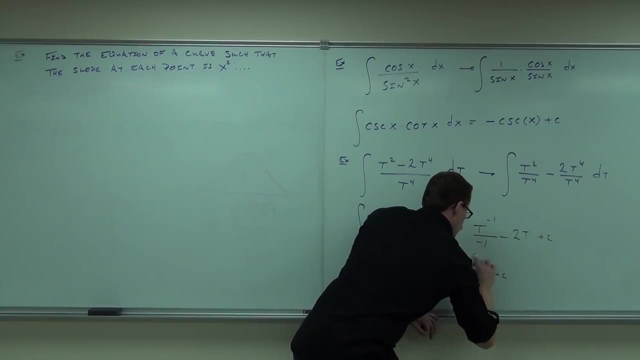 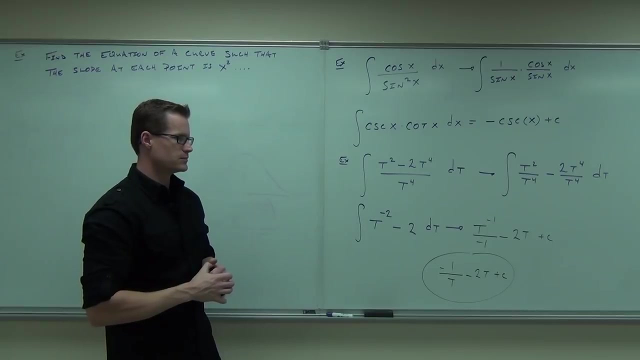 Now I will make this a little prettier. I'm going to move that exponent to the denominator. that'll be negative: 1. Over t minus 2t plus c. Whenever we have negative variables, we should at the end move it down. a negative exponent. 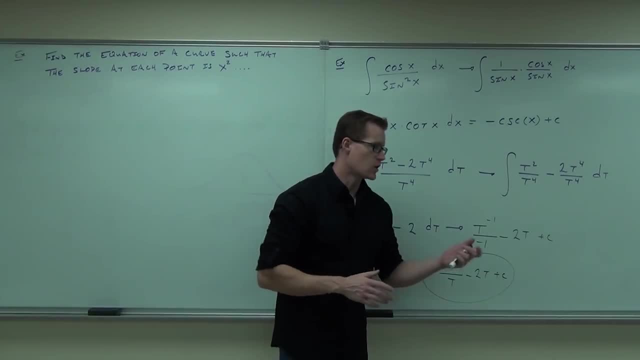 Yeah, typically yes. Are there cases where you don't? Yeah, there are, but typically yeah. Would you wish me if you got that one Good for you. fantastic Integrals versus derivatives: so far easier or harder, Harder. 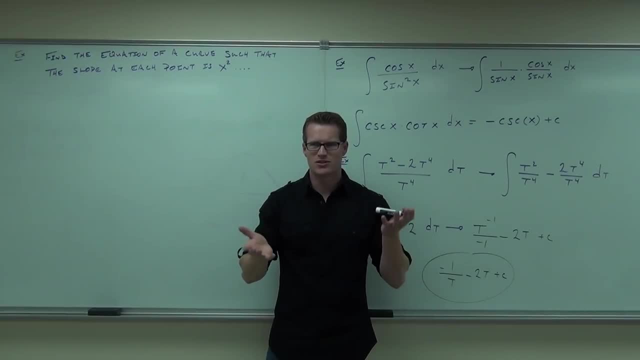 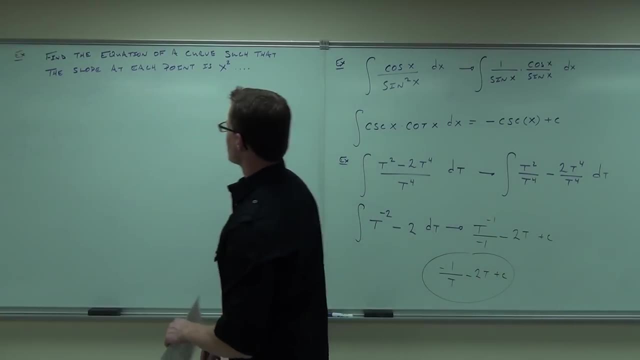 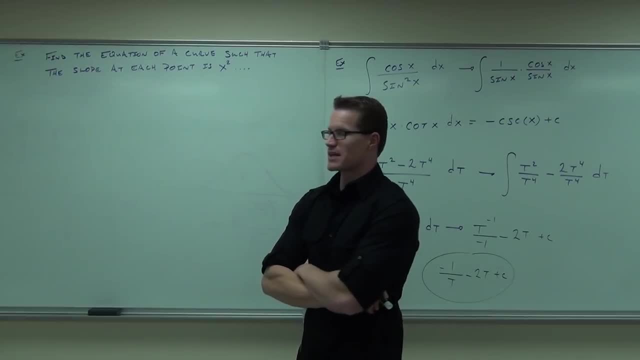 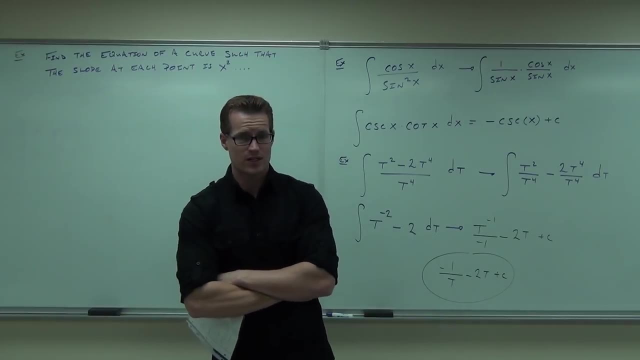 Find the equation of a curve such that the slope at each point is X squared. Let's think about what this means. Find the equation of a curve such that the slope at each point, the slope at each point, is X squared. What gives you the slope of an equation? 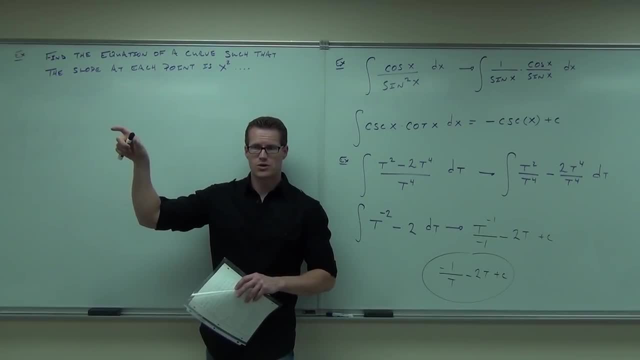 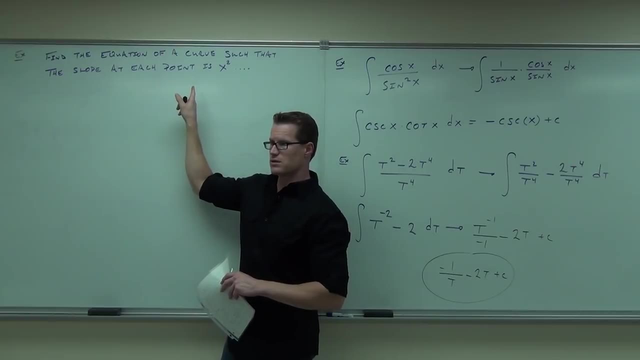 So basically it asks this: Give me an equation. When I take a derivative of it, the derivative is x squared. do you got me? That's basically asking for the anti-derivative. That's what this question asks. It says: give me an equation so that when I take a derivative of it, when I get the slope, 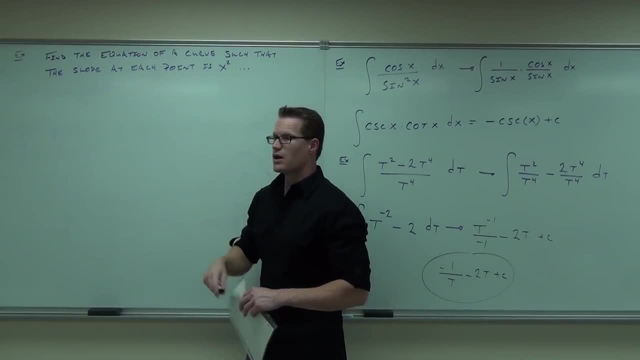 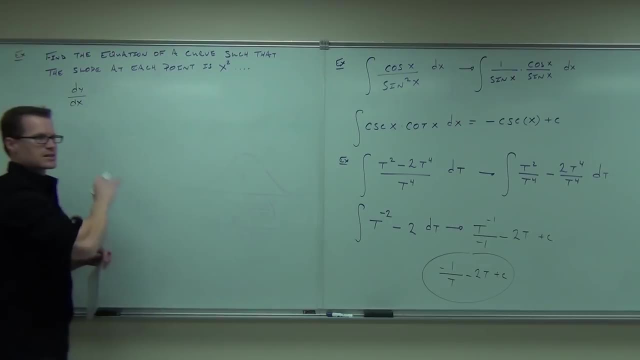 at any point that's a derivative. that's going to give me x squared. So this question says: okay, here's what you know: the slope at each point. recognize that's a derivative right. The derivative means a slope at any point. that is dy dx. 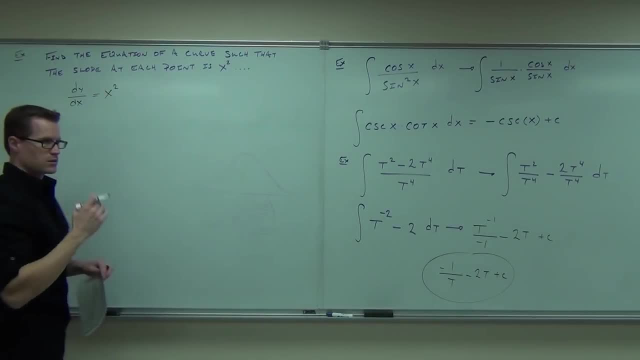 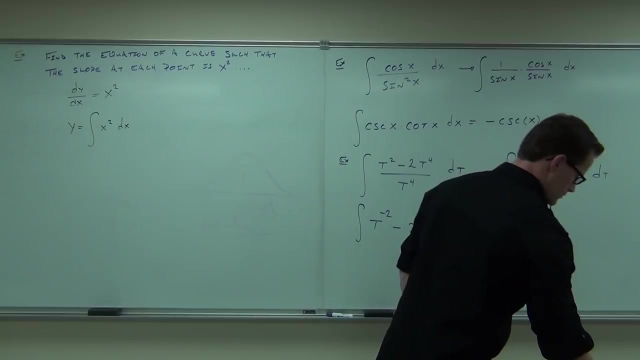 The slope equals x squared. true, The slope equals x squared. How do you undo that? Well, how do I find the equation that's going to give me that? Take an integral of x squared dx. You're going to notice some weird things, and this is kind of the way it works. 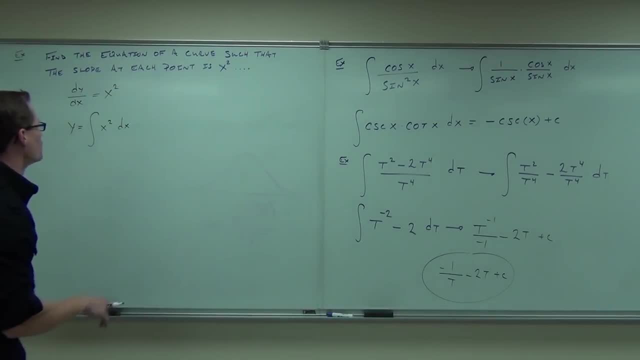 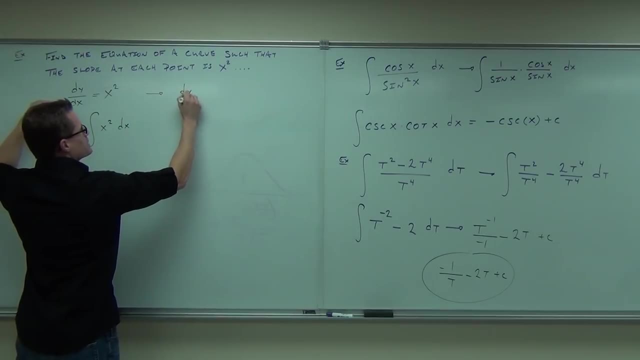 It's interesting. I can show it to you a little bit later where all these symbols come from. but do you notice something? This is weird. But do you know something about this? If I treat this like a variable and I multiply, I get dy equals x squared dx. 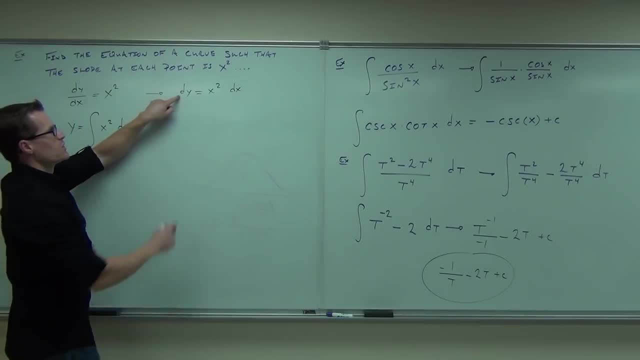 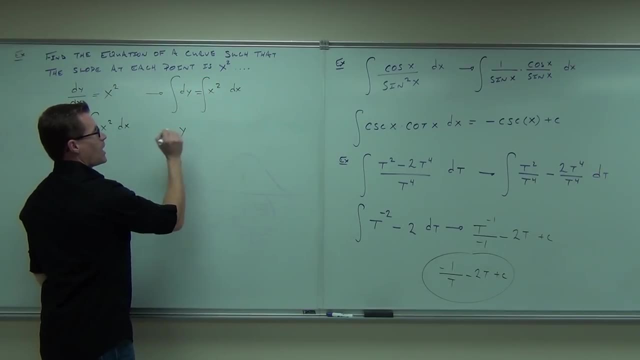 Do you see where the dx is Interesting? huh, If I want to undo a derivative, an integral undoes that. An integral undoes that. on both sides, Integral of dy is y. Aha, look at that. That's 1 dy, right. 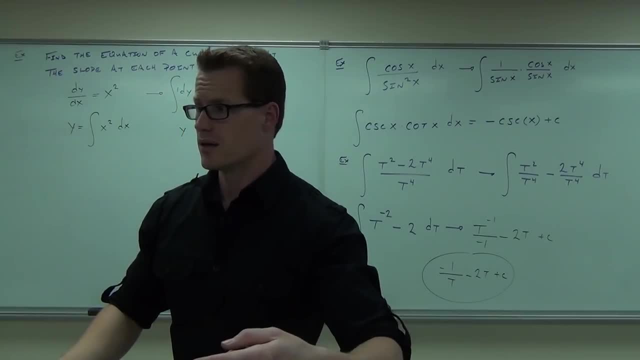 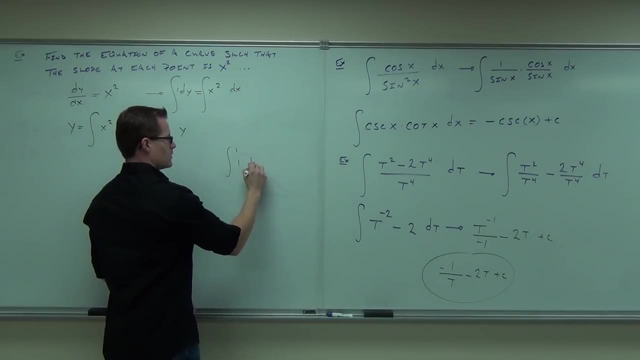 With respect to y: 1 dy. with respect to y. will give you y. Does that make sense to you? Did I lose you? Yeah, Do you remember I lost you? Yeah, What was this? I don't know. No, no. 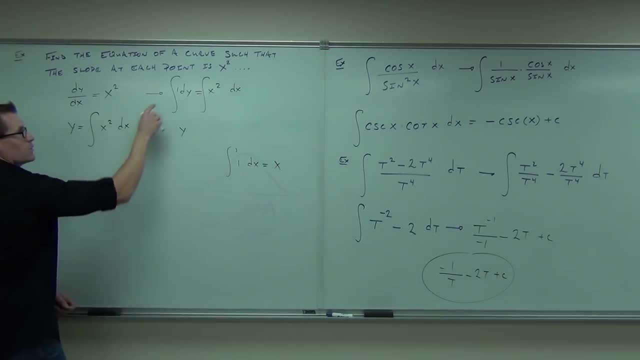 What was this? Oh, x. Clearly, With respect to y, it is 1.. Oh Equals the integral of x squared dx, which is exactly what we have right there. That's very interesting. It says: undoing a derivative gives you an integral. 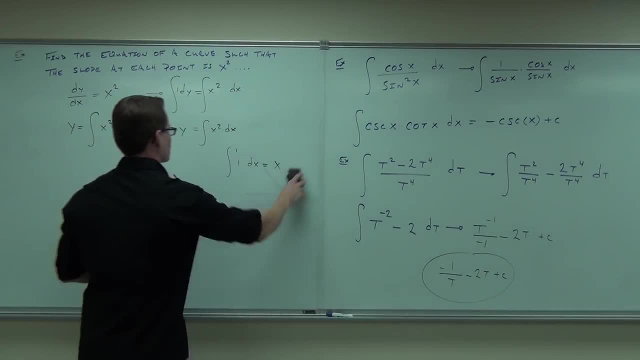 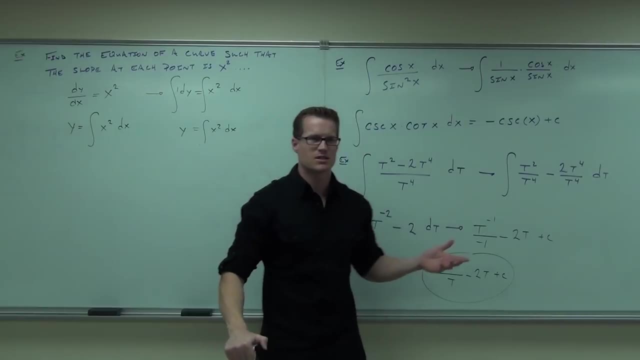 Crazy, Crazy, Cool. Anyway, that was a side note beyond a little bit of the realm, but it's interesting how that works, right, Because some of you were asking where's the dx or maybe thought where's the dx coming? 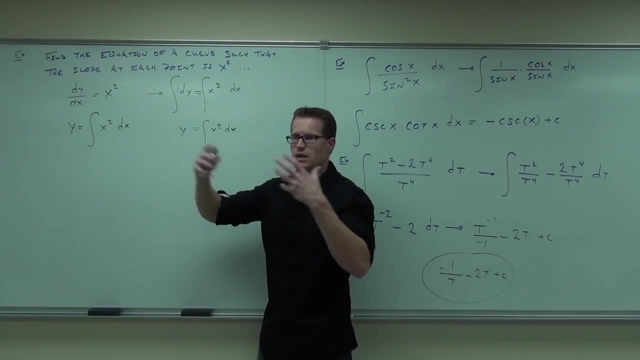 from. Why do we have that? It's from doing that. Doing this idea. Undoing a derivative says: well, you work it this way: Integral of 1, dy, that's y. Take an integral of both sides, you get an integral of x squared dx. 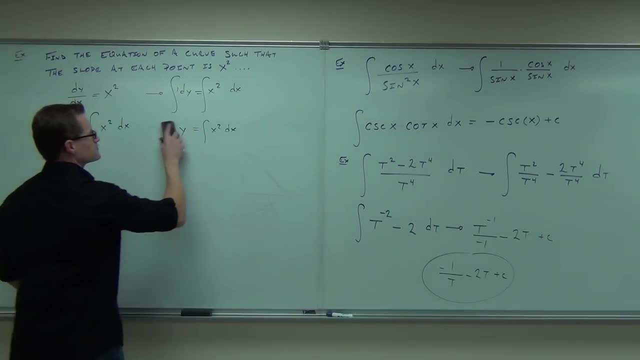 Okey dokey, That works Cool, All right, Thank you Bye. OK, now back onto this. Did you need that? Do you want me to write that back for you? No, You have it right, It's on video. 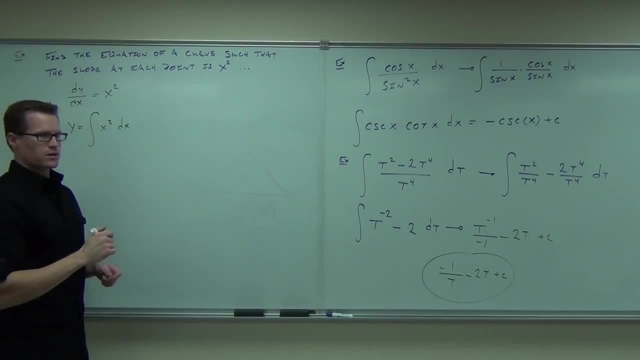 You can watch it again. What is the integral of x squared dx, x to the third? So are you saying that that's the equation, right? What does that represent, right there? The family, Family, Family, Family. 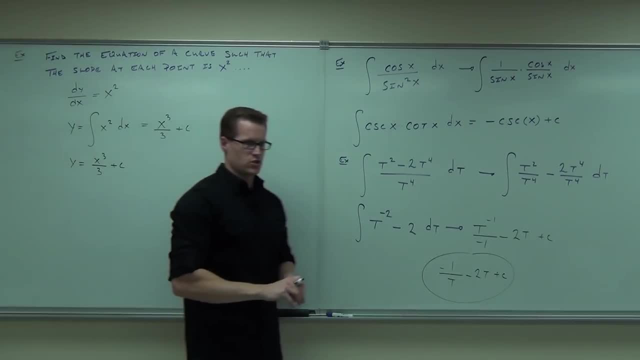 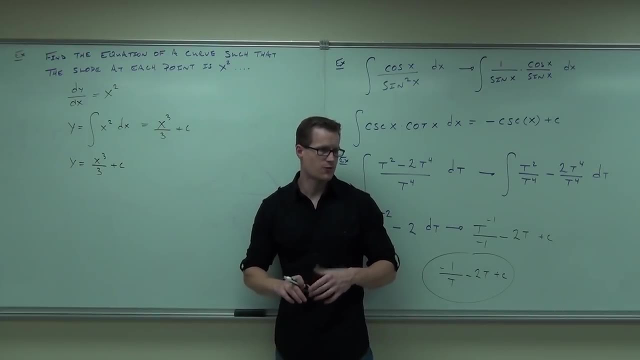 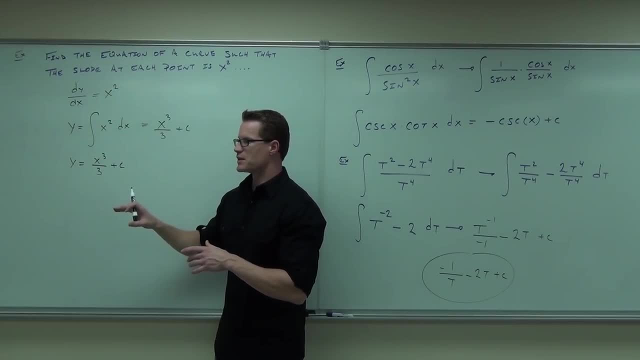 Is that true For sure? Any constant. Now, can I be specific? Can I give the equation in this terminology? Can I do that with this problem right now? No, not right now. Not right now because I haven't been specific on the c. 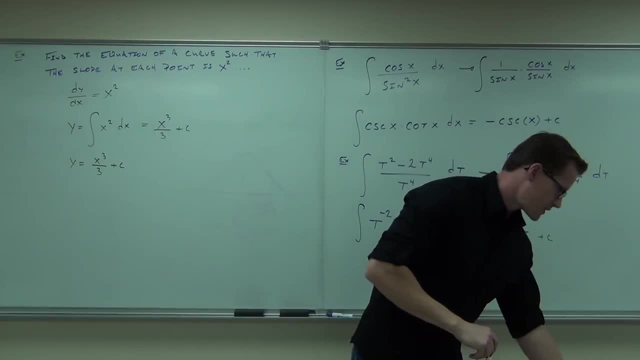 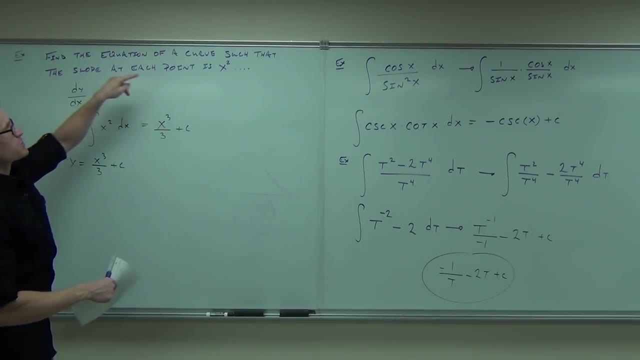 But if I change the problem just slightly- and here's what I'm going to add on to it- I'm going to say: let's find the equation of the curve such that the slope at each point is x squared. And that's why I added dot, dot, dot. 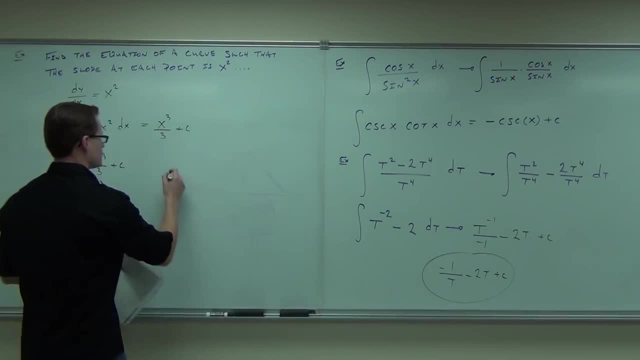 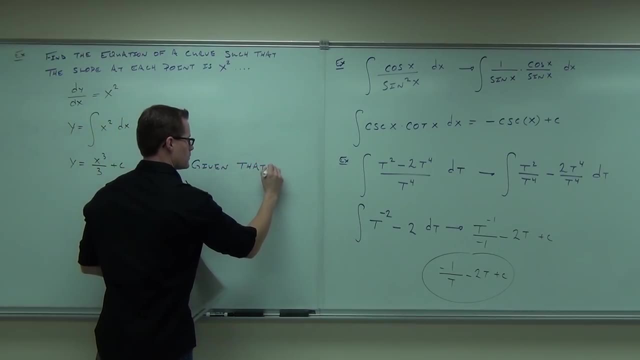 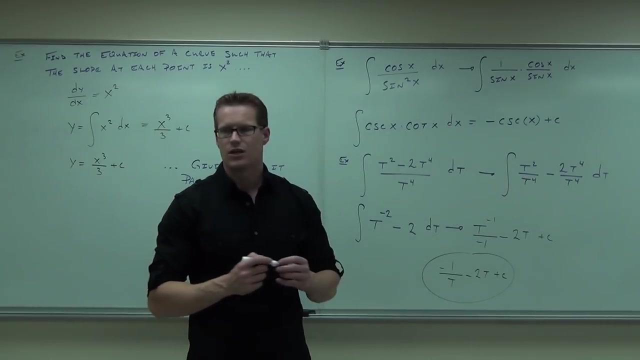 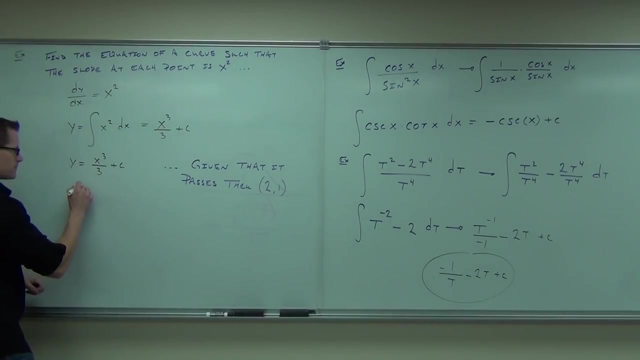 Given that it passes through the point 2, 1.. You know what? it doesn't make it any harder, It really doesn't. What this says, what this says right, here is this family, All the x cubed families you can think of, right. 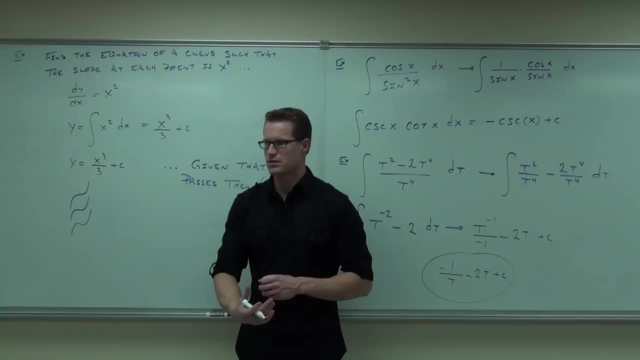 It says any of them that are shifted up and down along the y axis. Do you notice that There's no other x's? This is just x cubed, shifted up and down the y axis. So that's what I'm going to do. 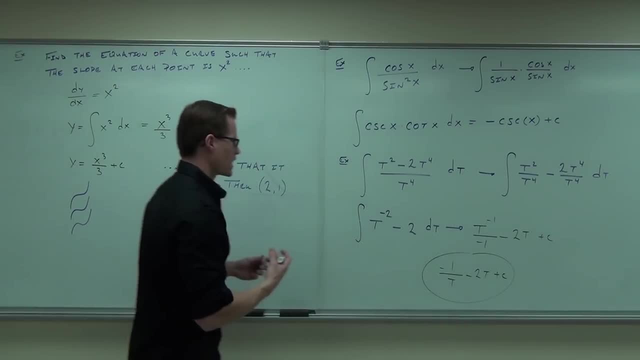 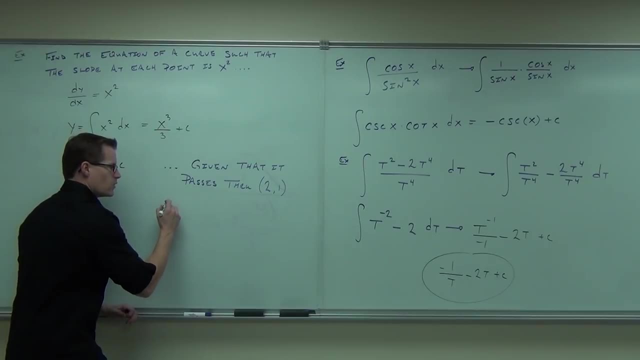 This is just x cubed, shifted up and down the y axis, so your y intercept is different. What we're saying is now: ah, choose a specific one and now tell me what it is. So the way to go about this is you can say: all right, well, I know for a fact what we just found. 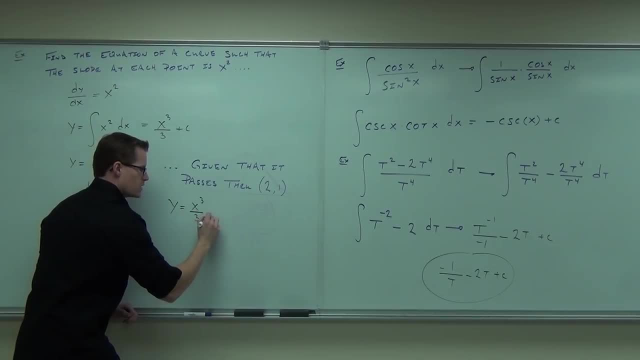 out is that y equals x cubed over 3 plus c, not e, c. Right, That's what we have. Hey, do you have an x? Do you have a y? Plug them in. You're going to be able to find c. 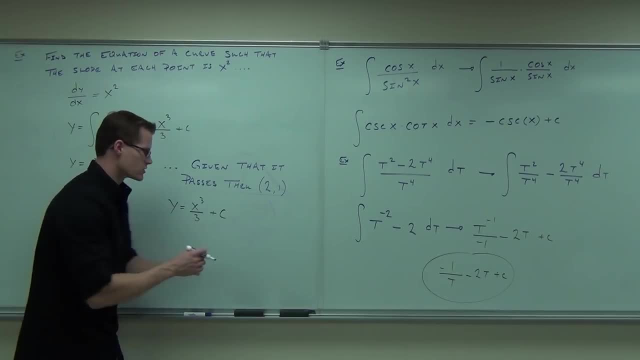 That gives you a specific, Specific equation, Not a family, but a specific equation. So when I plug in my 1 for y, my 2 for x, let's just solve for c. If I subtract 8 thirds from both sides, what do we get? 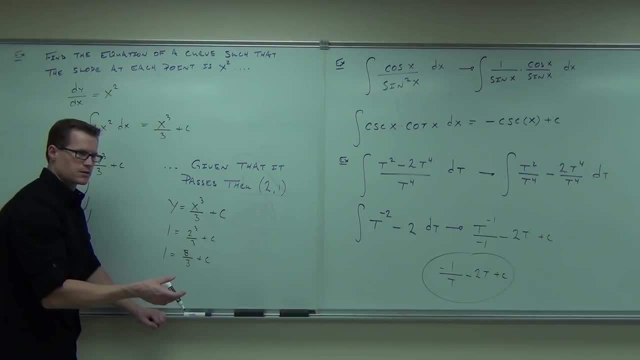 Negative 5 thirds, something like that. This number 2.. Yeah, All right. All right, So that's what we're going to do. So when I do that, I get c equals negative 5 thirds. Can you see that down there? 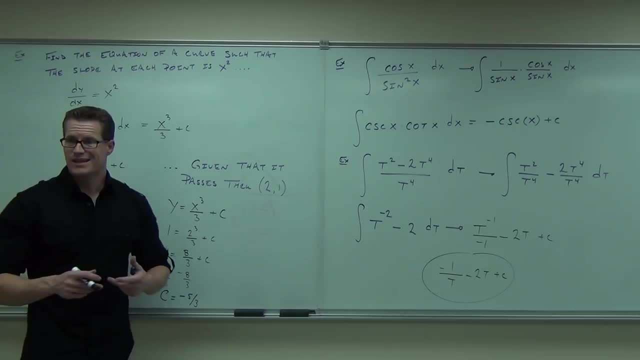 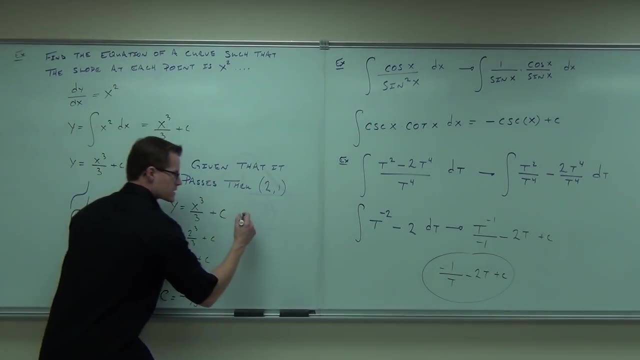 How do I finish out the problem? Well, it's not that hard, It's. you now know what c is right Here. we were stuck without a c, so if I want to finish this off, I go back up to here. 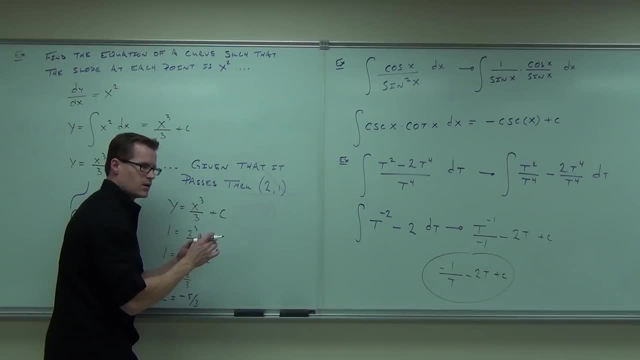 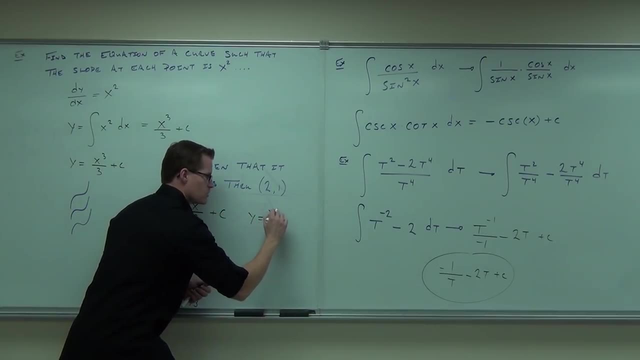 I say: all right, I know the equation, so that when I take this off, I know what c is. When I take the derivative of it, it gives me x squared. when that happens and it goes through this point, it's: y equals x cubed over 3, and then what? 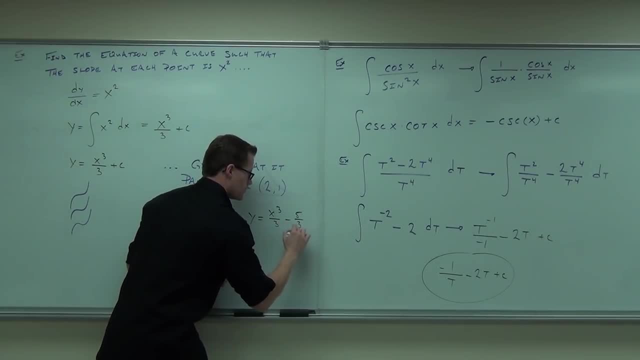 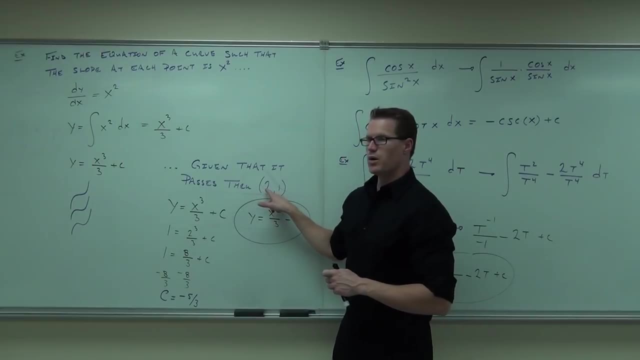 Minus 1.. Minus 1.. That's right, Let's verify that. for a second, Is this going to go through the point 2, 1?? Sure, That's how we found c. When I take a derivative of this, does it give me x squared? 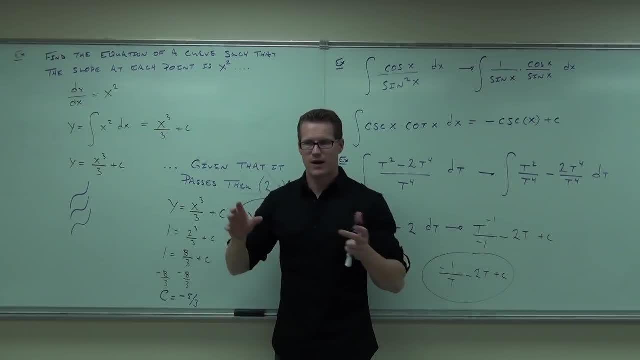 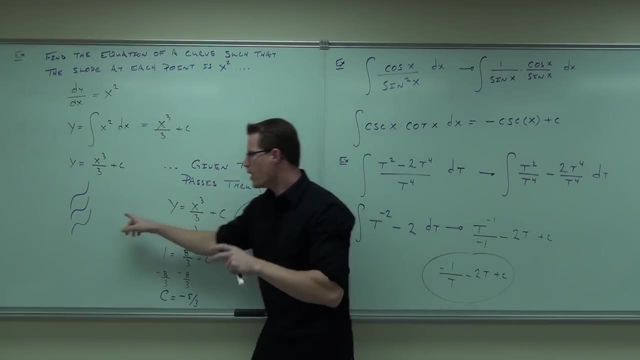 Mm-hmm, Then this is the only equation, So that when I find the slope, at each point it's x squared and it goes through this. That says it's not a family anymore. We've narrowed it down to 1 of these graphs. 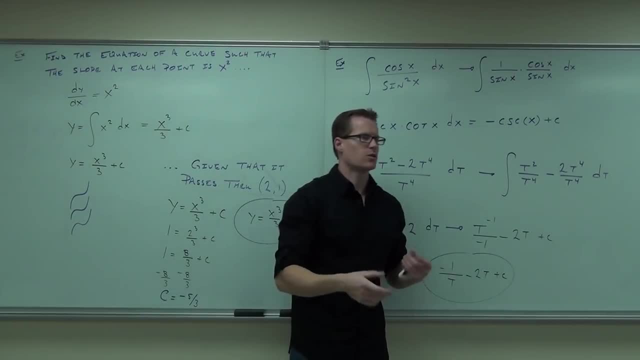 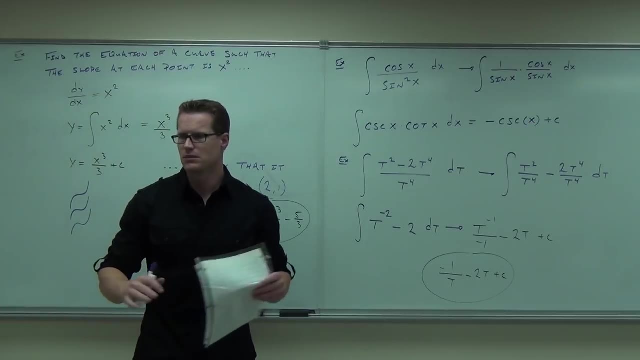 How many of you feel okay with that one? That's the idea. This is very similar to what's called the initial value problem that we're going to study right now. We're going to talk about differential equations. Just an introductory, not anything too drastic. 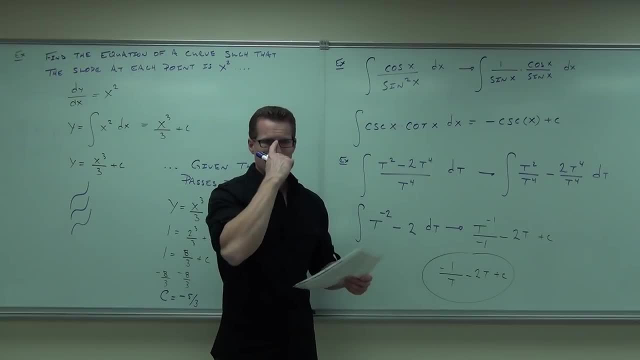 They have a whole class on differential equations. right, I'm giving you, like you know, when you get a new thing, ice cream, and you open the lid and you get the ice cream on the top, you're like, oh, I bet I'm going to get ice cream on the top. 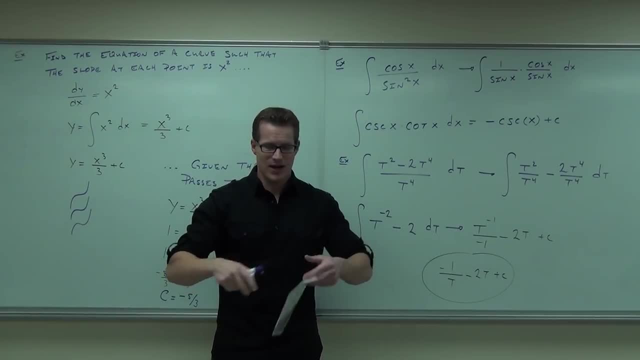 You're like: oh, I bet I'm going to get ice cream on the top. You're like, oh, I better get that stuff because it melts real quick. You know that The ice cream is differential equations. I'm giving you the stuff off the top. 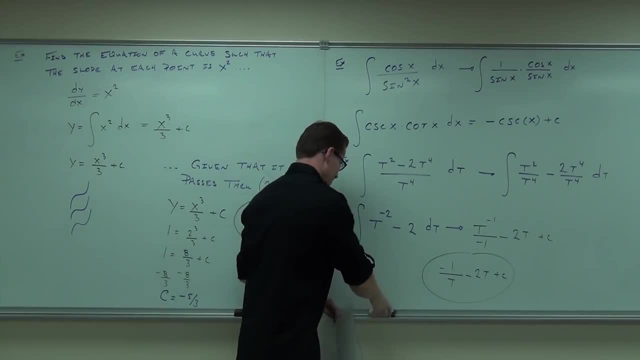 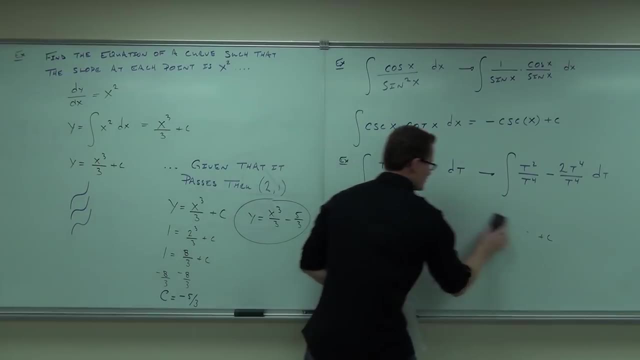 That's it. That's the skimmest tasting of ice cream. It is really sweet, but you get more of the good stuff in the actual class. okay, It turns bitter. It doesn't have to be bitter, It's fine. 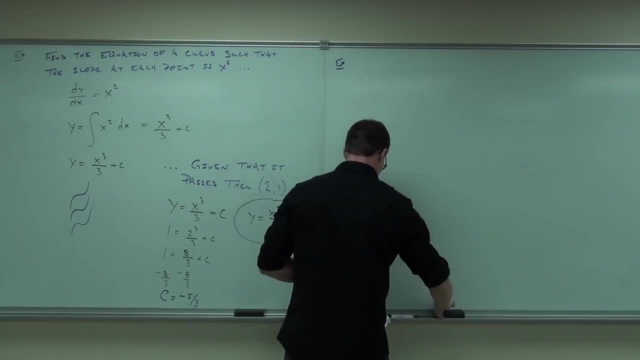 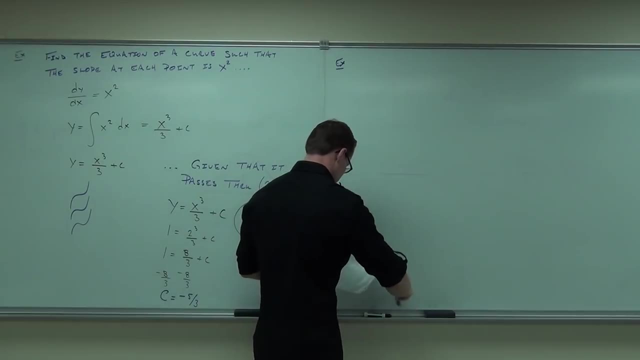 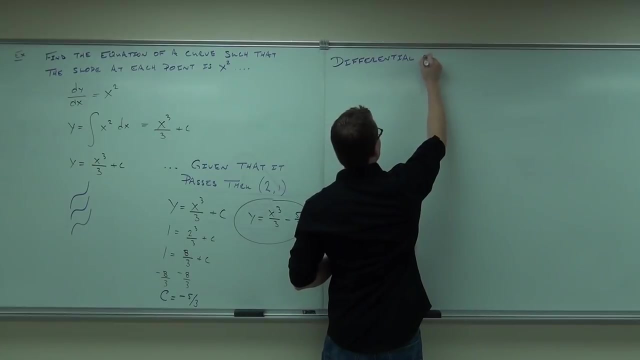 I don't know what kind of ice cream you're talking about, so I don't know what you consider. fine, You ever had garlic flavored ice cream. It's actually pretty good. It's not like that, It's an acquired taste. Yeah, so don't go home and say, oh, I learned all about differential equations. 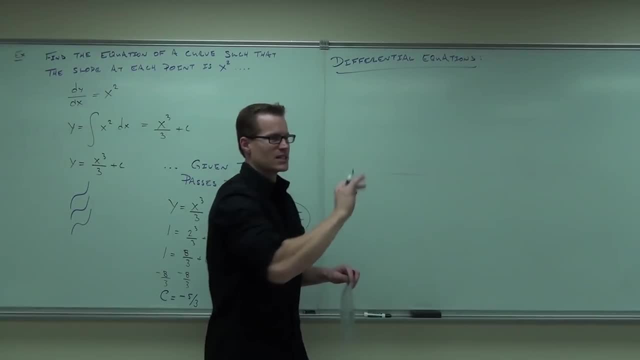 No, you didn't. All right, this is just the little little, teeny bit of it, but the idea is is there and we're starting with a basic idea. Let's pretend for a second and this was basically it. 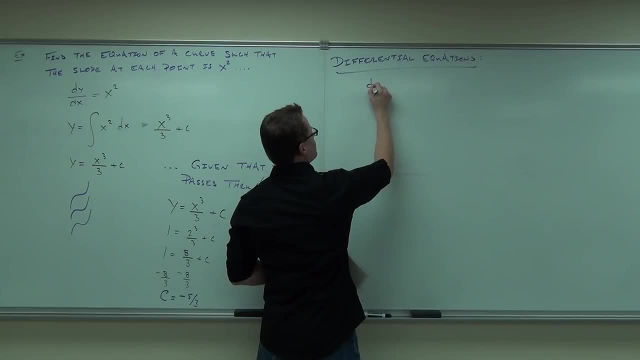 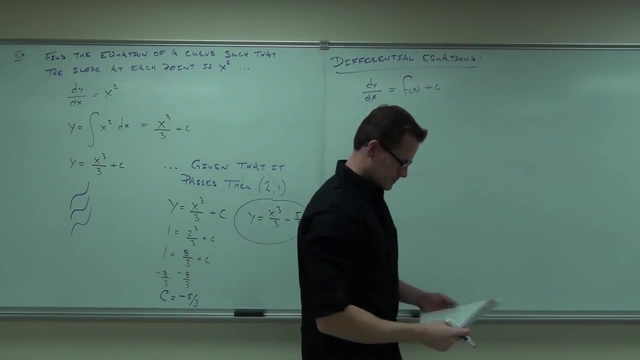 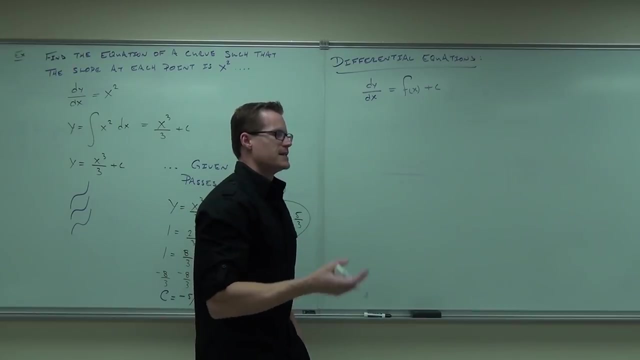 I'm just kind of going to illustrate a little bit more. Let's pretend that I have a derivative that I know like that. The idea is this: It's basically the same thing we were doing here, It's: can you find a function, an anti-derivative, so that the derivative gives you this? 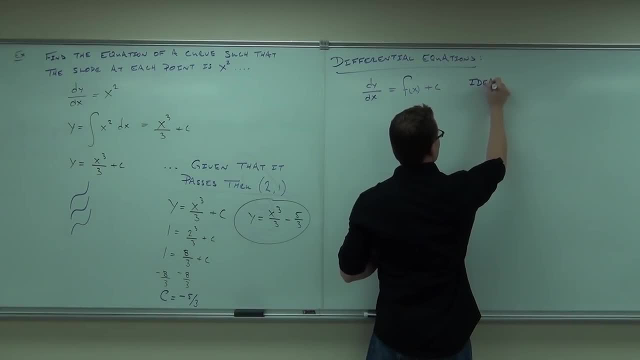 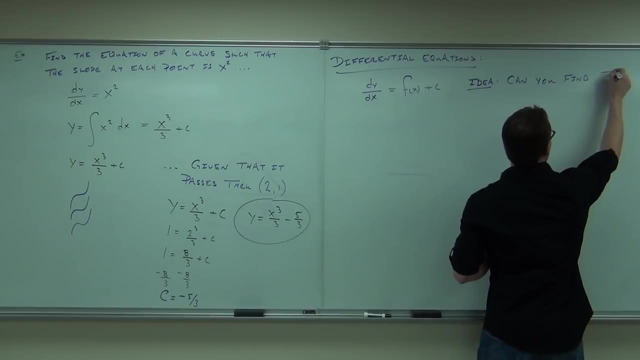 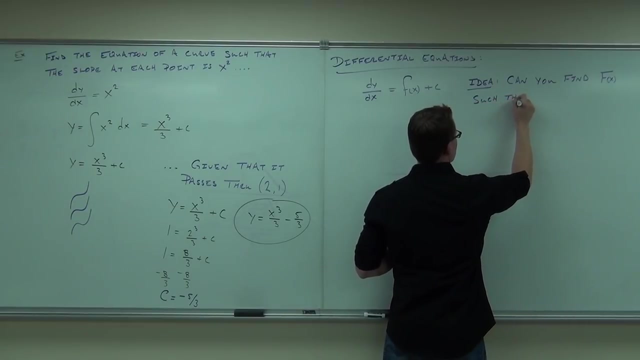 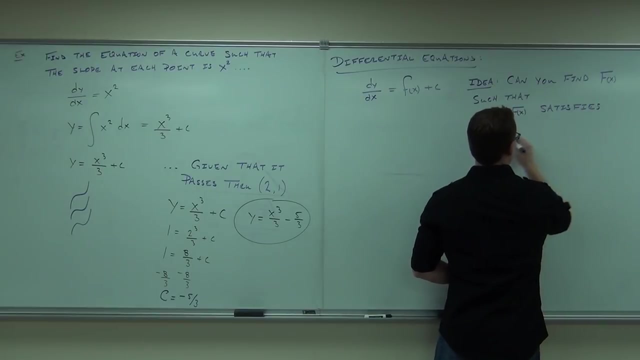 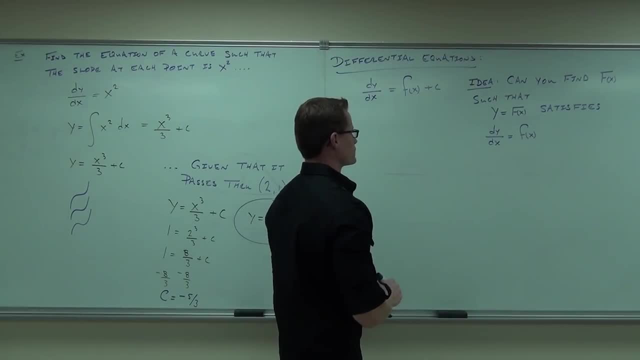 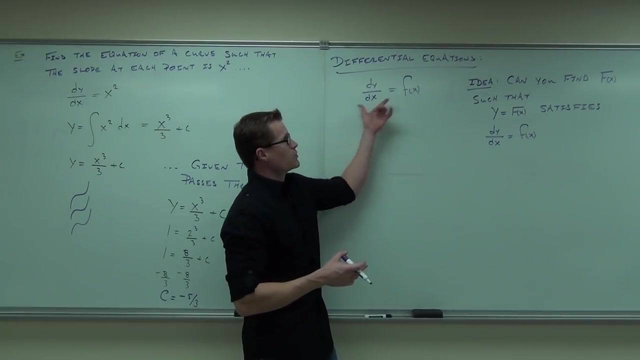 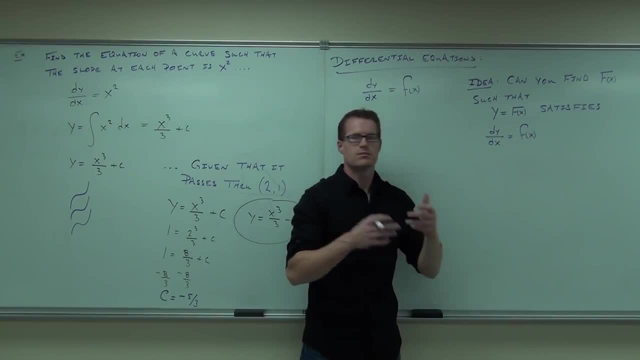 function so that when I take the derivative of it, it gives me original function back again. That's the idea. It's essentially the same as this. Let me show you how this works with what's called an initial function. I wanna make sure it doesn't break. 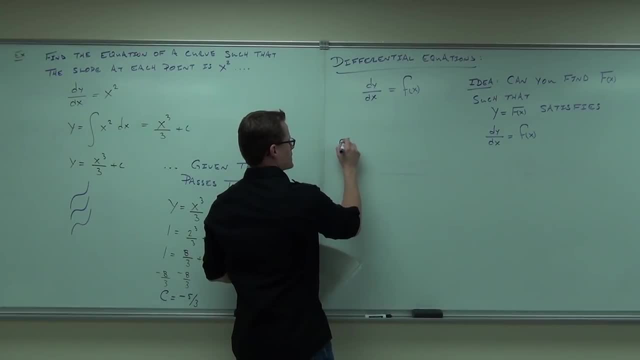 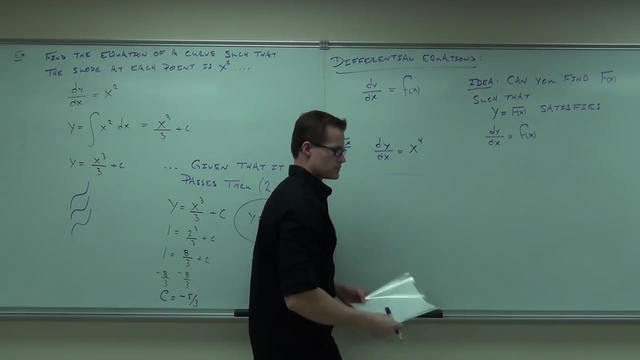 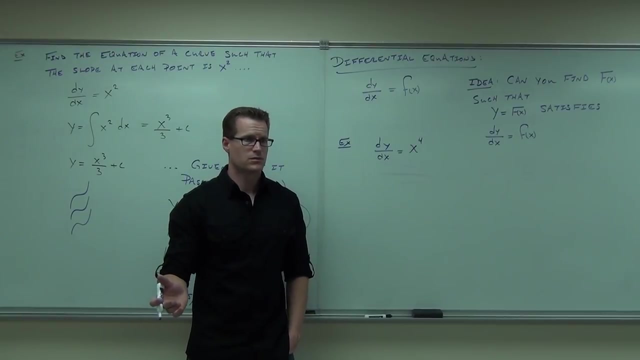 after we do one basic example. Let's say that dy dx equals x to the 4th. Can you tell me what y equals? If the dy dx equals x to the 4th? can you tell me what y equals? One-fifth x to the 3rd? 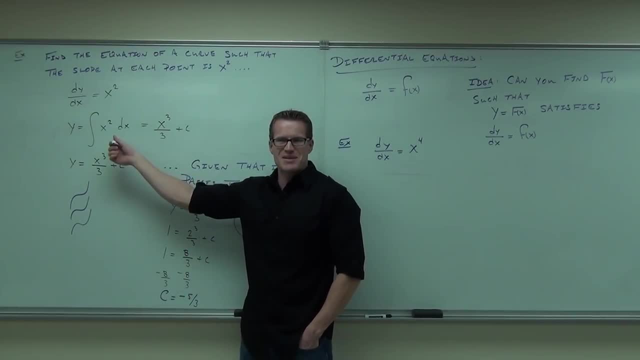 That's what it would be. It's the same question here. Do you see how it's the same question? It's interesting, isn't it Same thing? I asked you here. Find me an equation so that the slope is this. That's what it says. 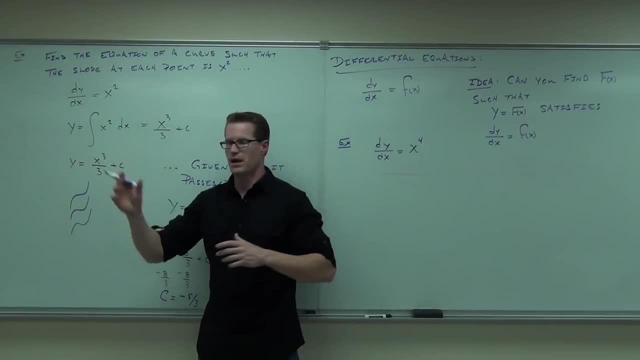 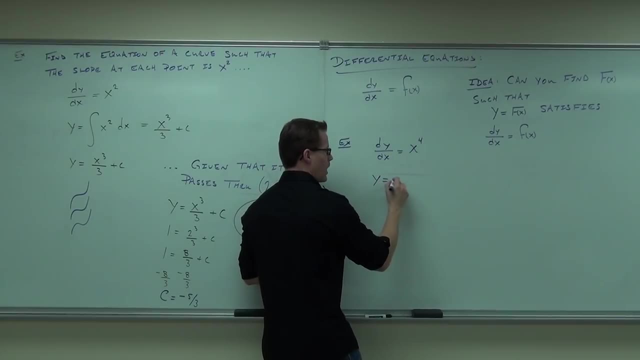 Find me an equation so that the derivative is this: Instead of slope, I now have the word derivative, But it's the same idea because slope is a derivative. So here it says: well, I know that y is going to be the integral of x to the 4th dx. 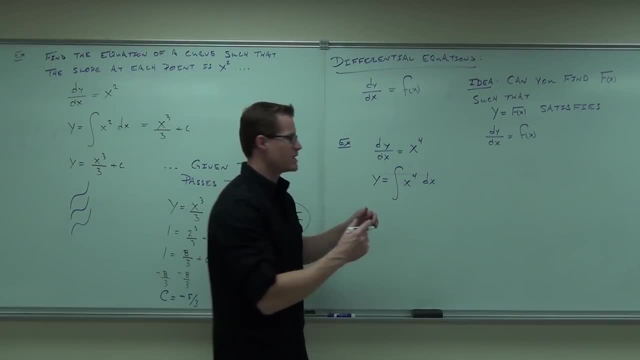 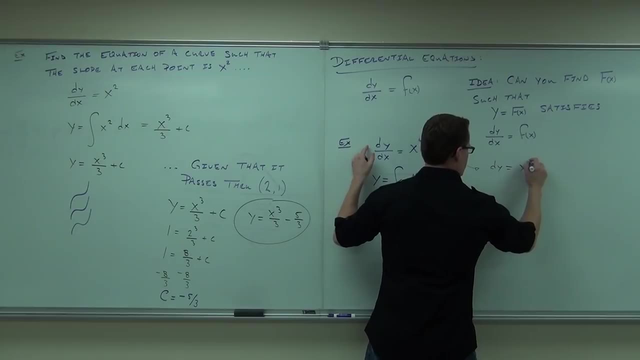 If you want that proof again, here's the proof again. Well, not even a proof, but here's a minute. I'm going to do a calculation of these variable parts. If I separate them, I get dy equals x to the 4th dx. yes, 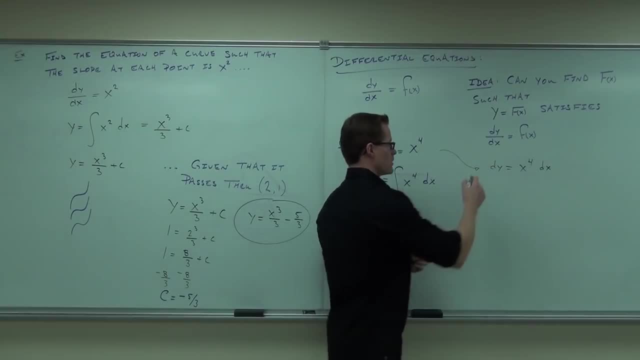 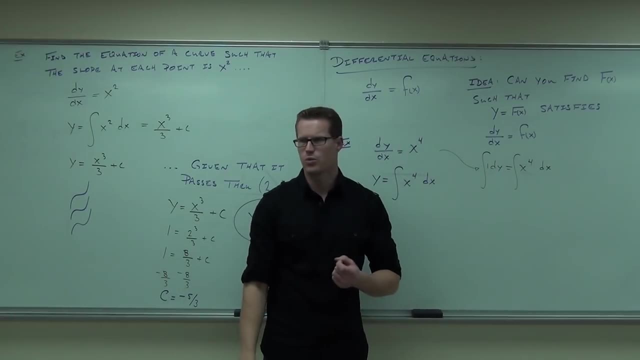 To find y I have to undo a derivative on both sides. Undoing a derivative is called an integral, The integral of 1 dy. I can put a 1 anywhere that I want to. The integral of 1 dy is y. 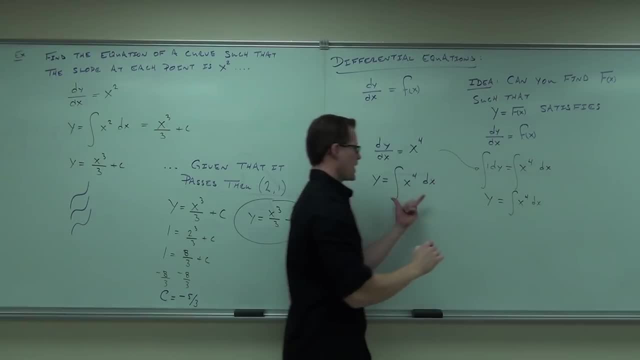 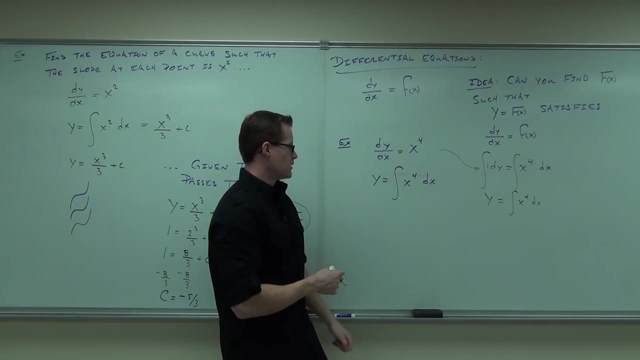 The integral of x to the 4th dx is exactly what I have here, And that's why we're coming up with this. That's how you find the anti-derivative. That's that. Does that make sense to you? Can you follow that? 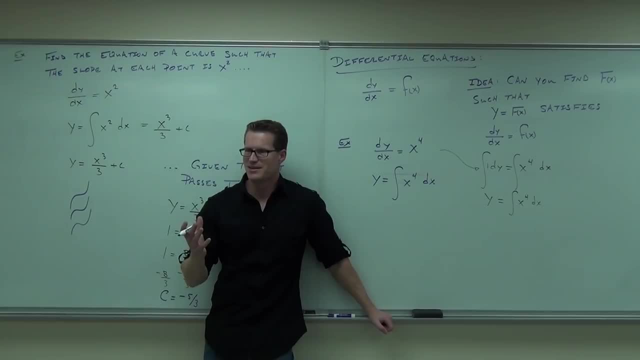 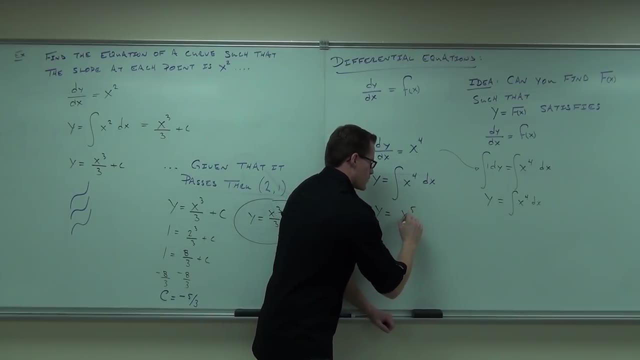 Have I blown your mind like a mine grenade? Are you with it? Yeah, All right, And Joe was right. x to the 5th over 5, or 1 5th. x to the 5th plus c. Don't forget the plus c. 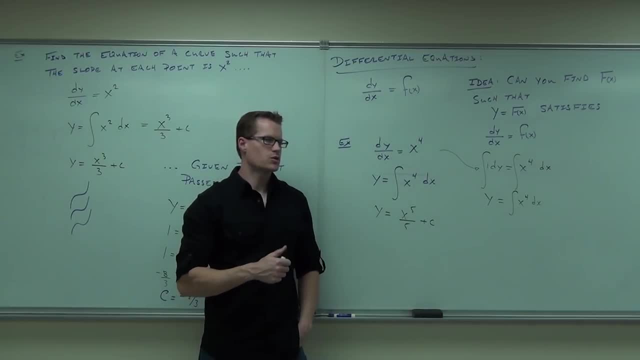 Everything's not working. Everything's not working. So what's a solution to a differential equation? It's actually not one. It's solutions to differential equations, just like we have solutions for a family of curves. before I put this little piece into it, 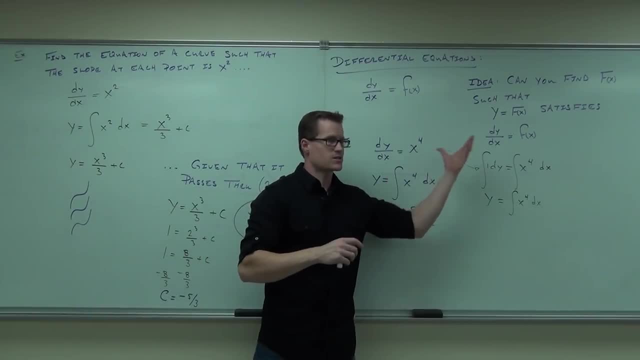 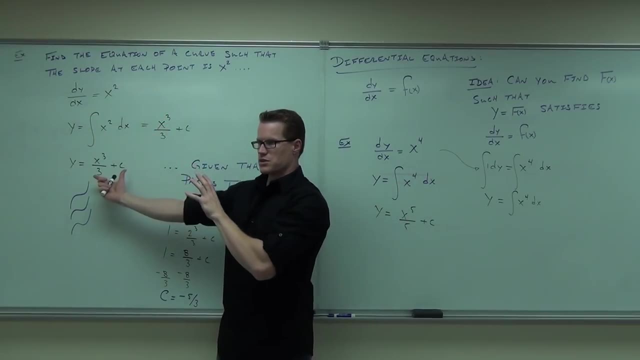 The reason why I gave you this first is because this problem is a differential equation. It's asked in the same concept. This right here is a differential equation. that's a family of curves. You got it. This right here would be an initial value condition, and that's what I'm going to introduce. 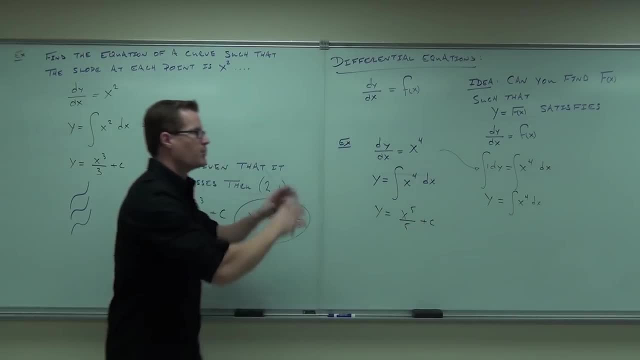 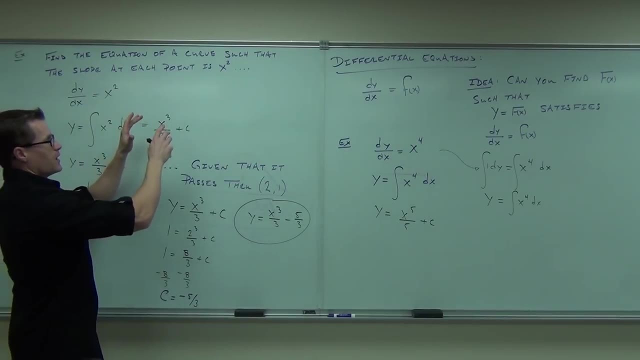 to you over here. in the terms of differential equations, Both questions are the same. Give me the slope, give me the derivative. I'm sorry, give me the slope of. if the slope is this, find me a function so that the slope is what I've given you. 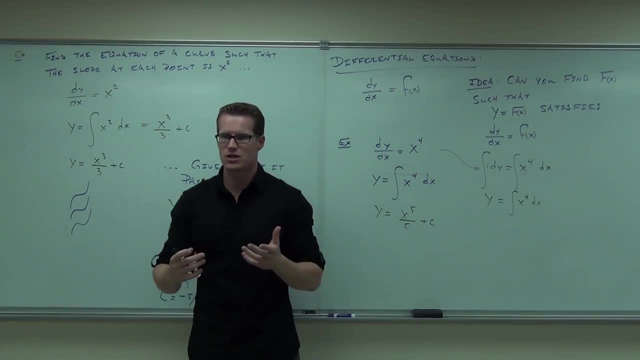 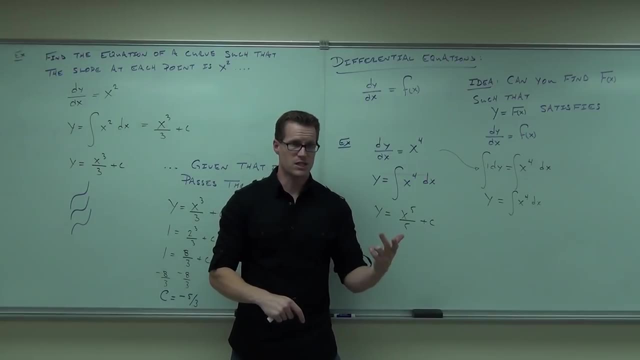 Find me a function so that the derivative is what I've given you. It's the same exact question. Then I can add pieces onto it. Here's a condition that lets you solve for c. I'm going to give you an initial value problem that lets you solve for c. 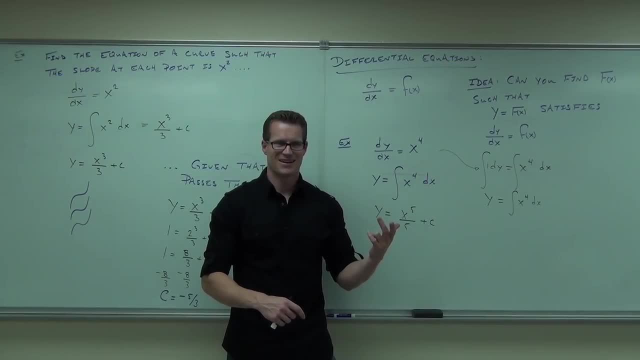 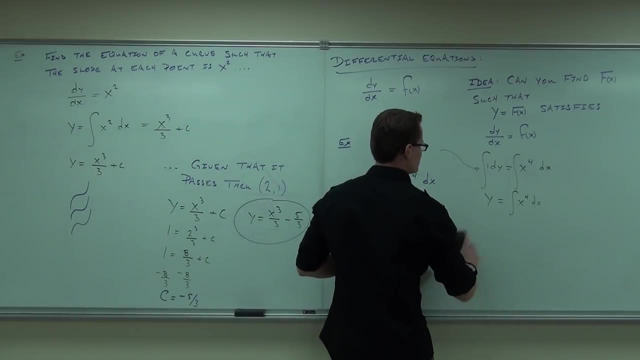 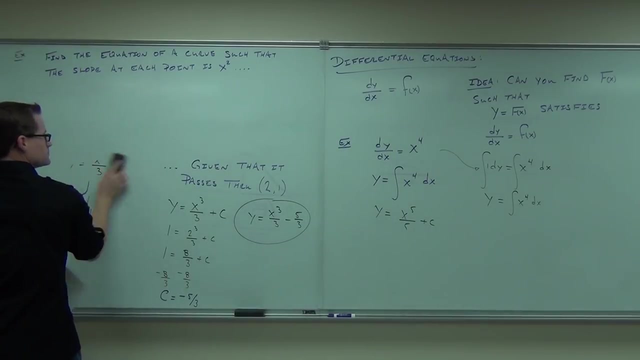 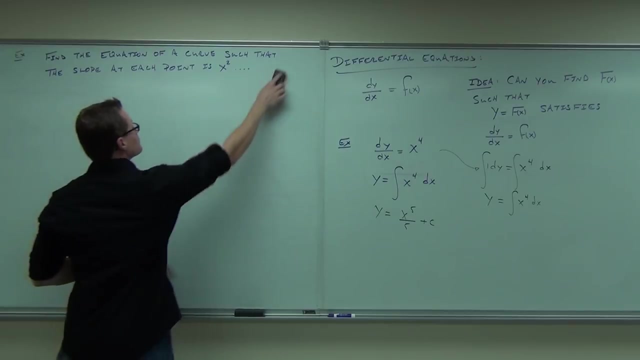 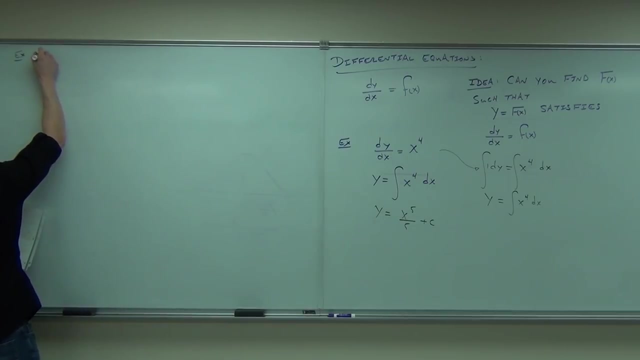 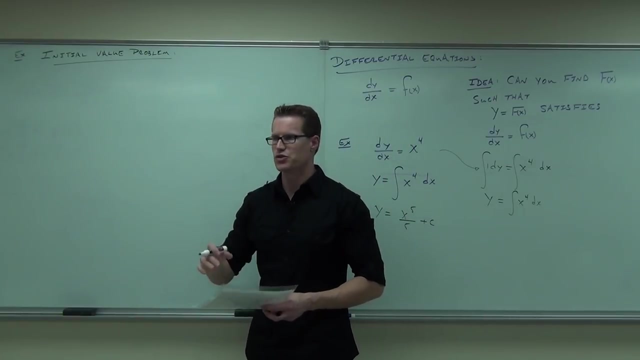 Would you like to c one of those? Totally, That was funny. Thanks, I'll leave that. How is that? This is basically when you only need one solution based on some initial condition. So this is the family of solutions right here. 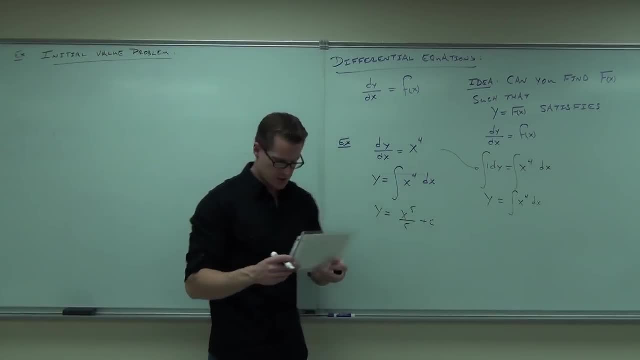 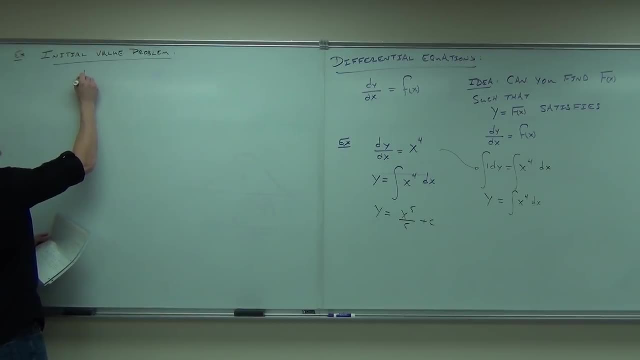 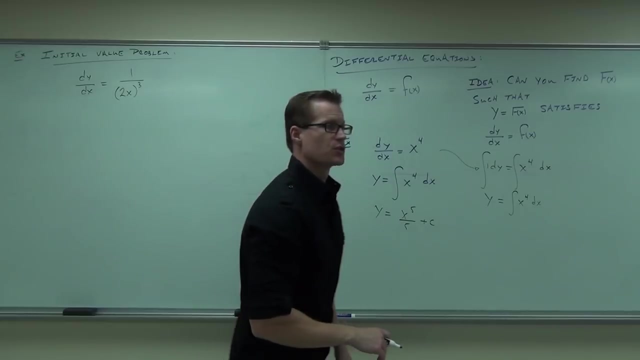 We're going to say, well, we only have one, We need something to fit a specific purpose, and that's what we're going to do here. So, basically, here's an example: If you have dy dx equals 1 over 2x to the quantity cubed, an initial condition looks: 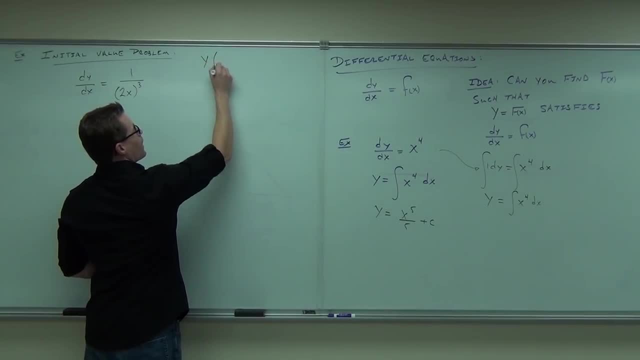 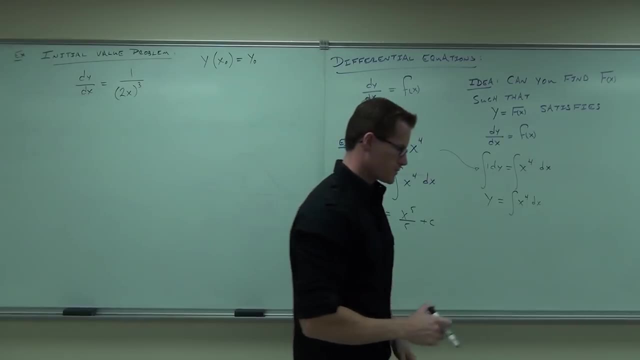 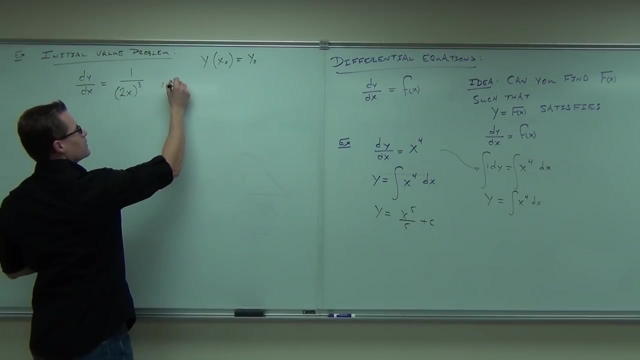 like this: It says: y of some initial x value equals some initial y value. That's what that says, And here's what I'm going to do. This looks pretty complicated, but here's what it says in real life. It'll give you like something: y of 1 is 0.. 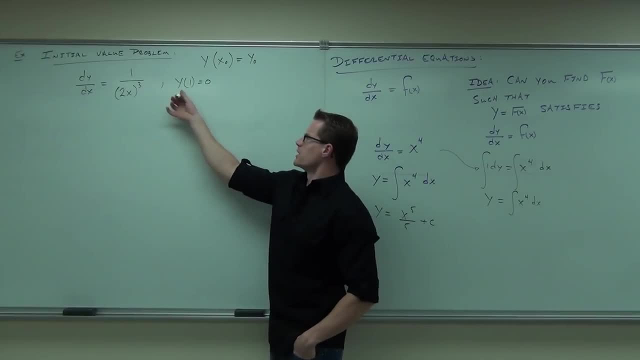 That's what it would be. Can you tell me what is your x coordinate here? What's your x? The 0 or the 1? The 1.. The y would be the 0.. This says, when you plug in 1, you get out 0.. 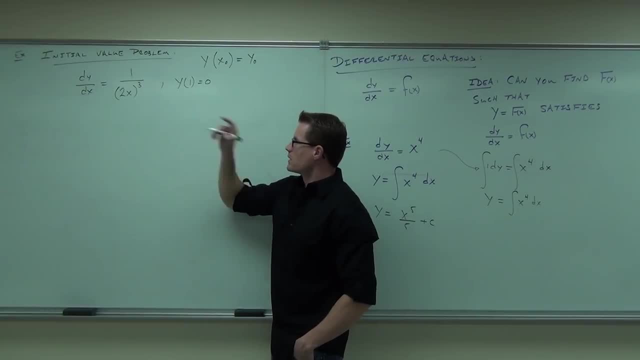 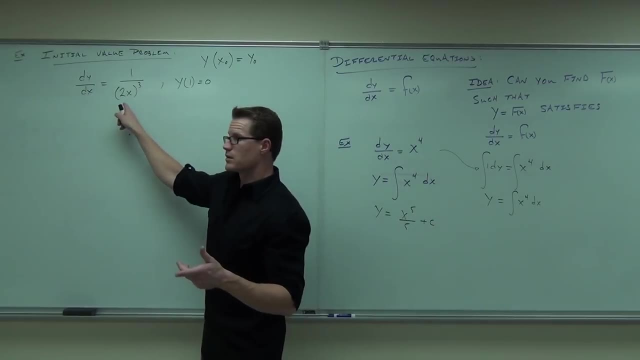 Does that make sense to you? That's what that says. So can you first undo the derivative. Secondly, can you use this to solve for c? That's the two parts of our problem. So firstly, can you do that for me? 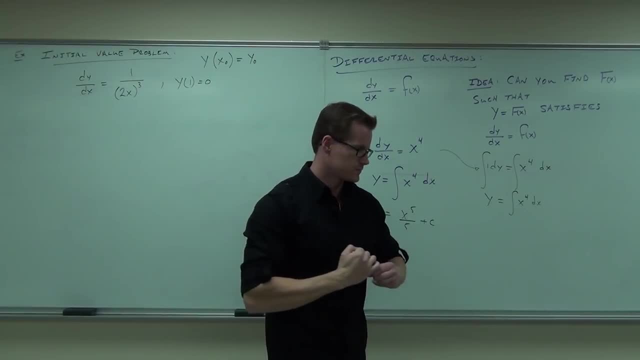 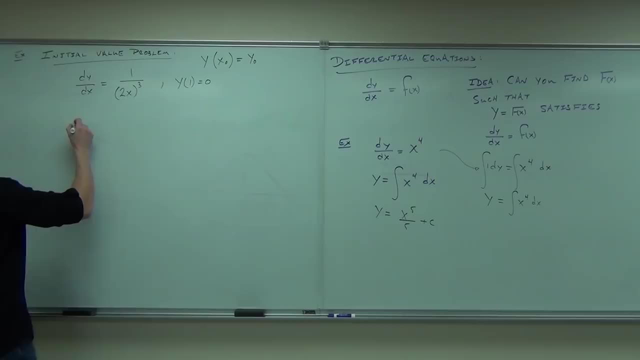 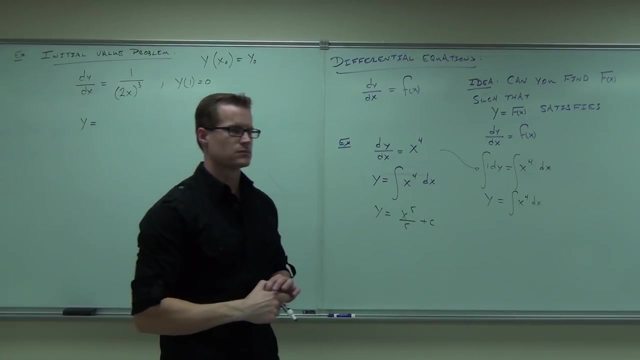 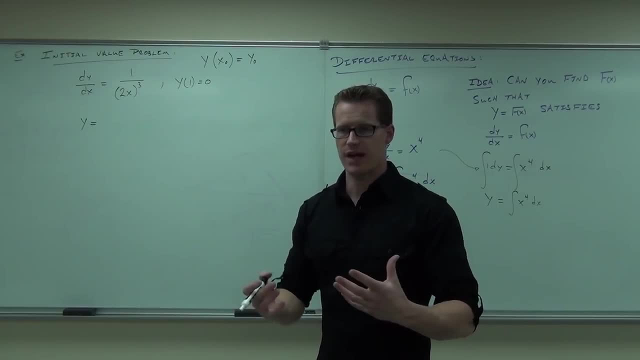 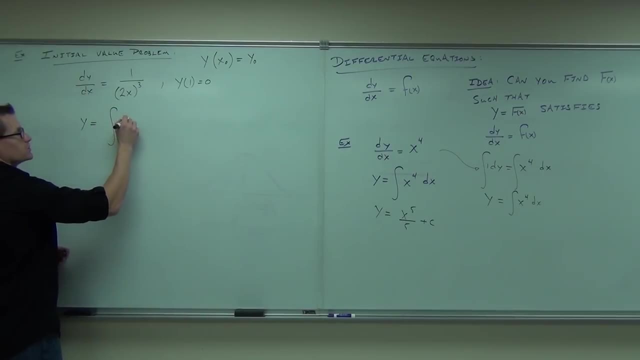 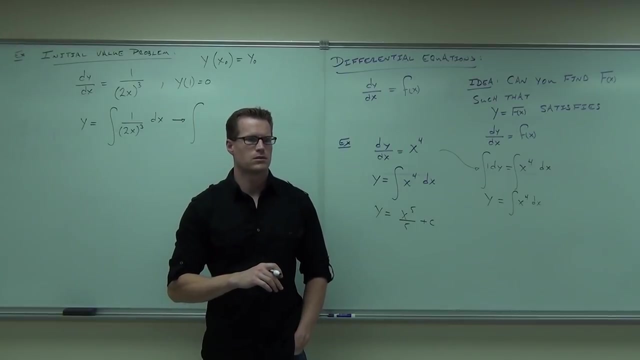 What's the derivative of y? What's the derivative of y? We need to undo that derivative. That's the integral, That's the antiderivative idea. So what we want is to undo this thing. Tell me, maybe the first thing that you would do. 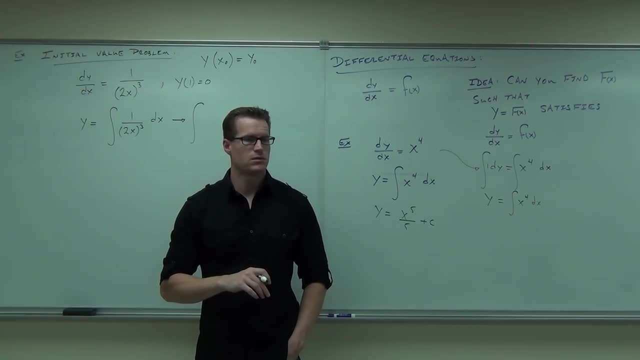 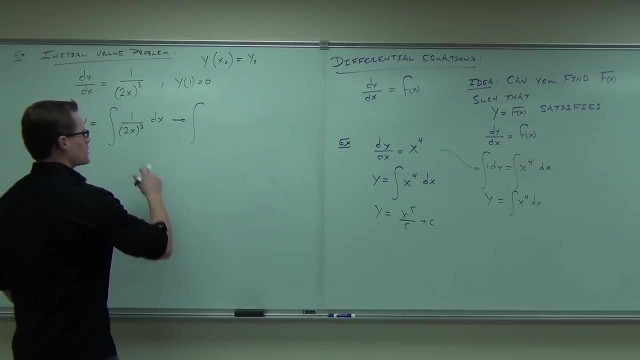 Make it fit the table. Make it fit the table You could. You'd have to be very careful with that. I'll show you both ways here. OK, Be very careful in how you handle this. Option one is: bring the bottom to the top right now. 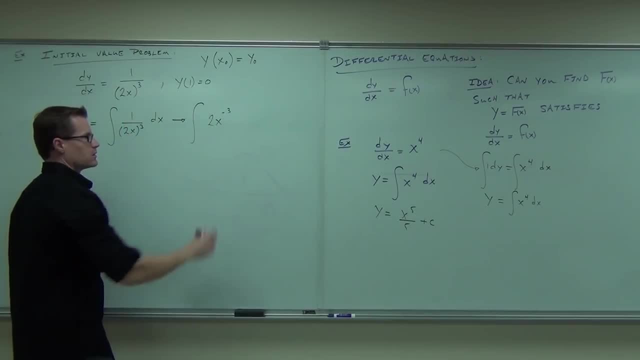 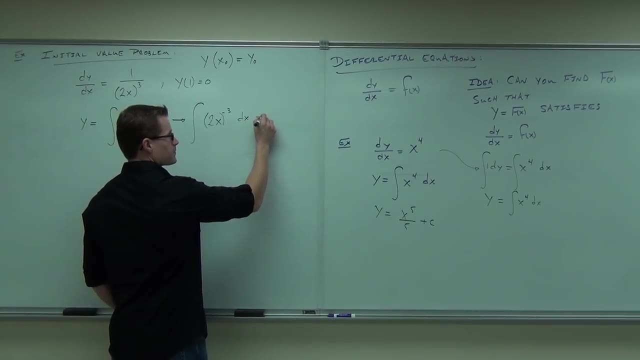 Right, No, Right, Yes, OK, Yes, That's right. If you do this, you can't take the integral. yet You cannot do it. What you would have to do is split that off, but you're going to get not 2 to the third. 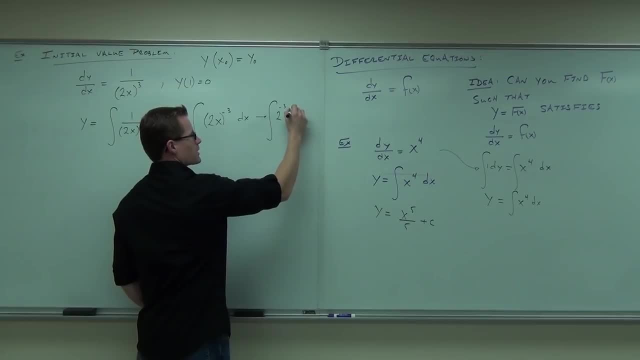 You're going to get 2 to the negative. You're going to get 2 to the negative. third over x to the negative. I'm sorry, times x to the negative. third dx. Do you see that? Oh, it doesn't go to 8.. 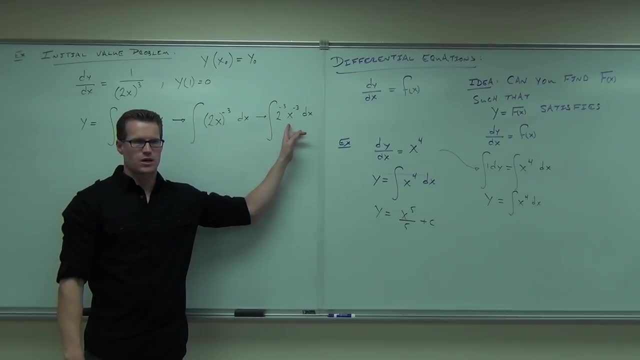 That's actually 1 eighth. Do you see what I'm talking about? It's not 8.. It's 1 eighth, So be careful on that. You get 1 eighth x to the negative 3.. That one you have to leave, because that does fit your table. 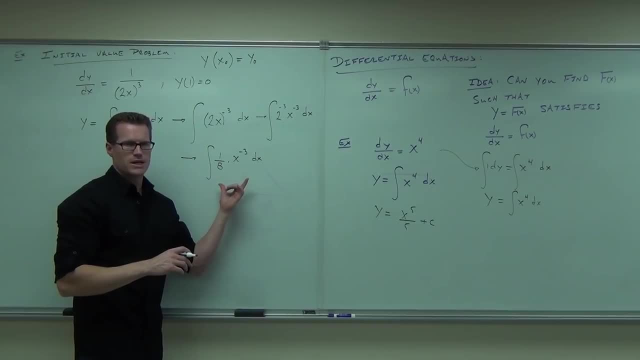 What can you do with the 1 eighth? Probably a good idea to do right. We don't want to mess around with fractions too much, Because if we create more fractions it's easier. if I write this as 1 eighth, x to the. 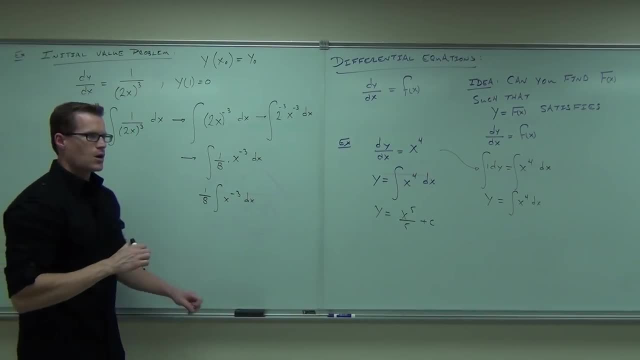 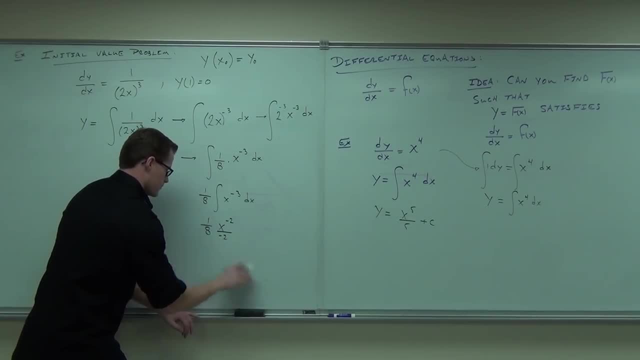 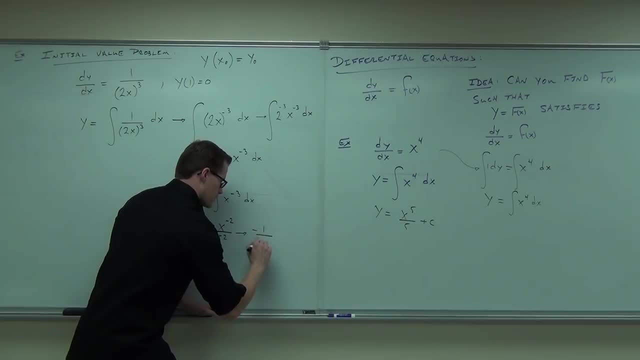 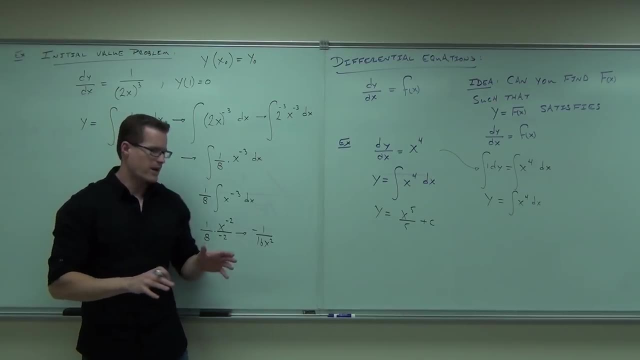 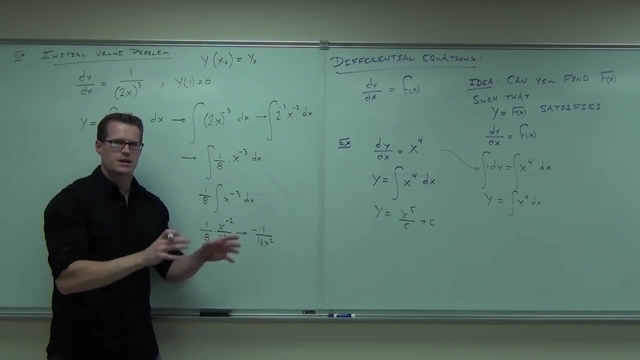 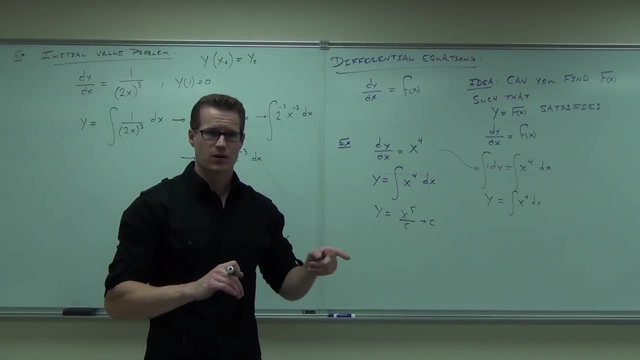 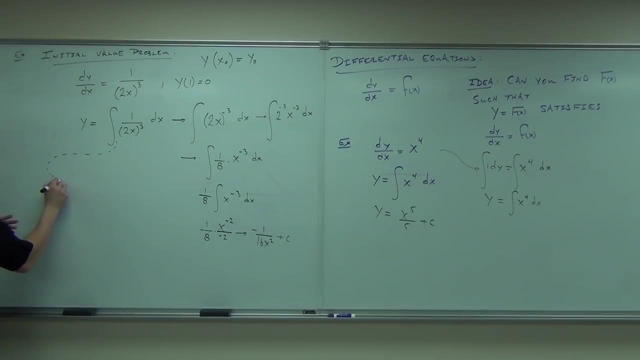 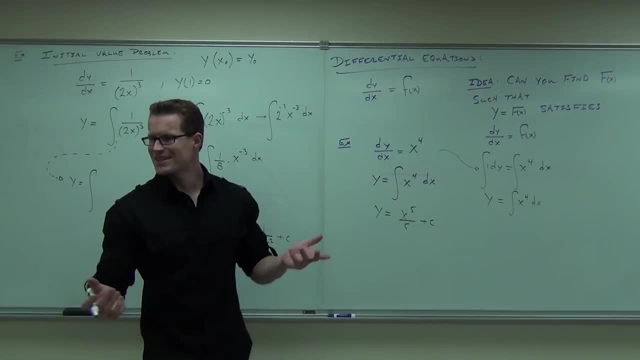 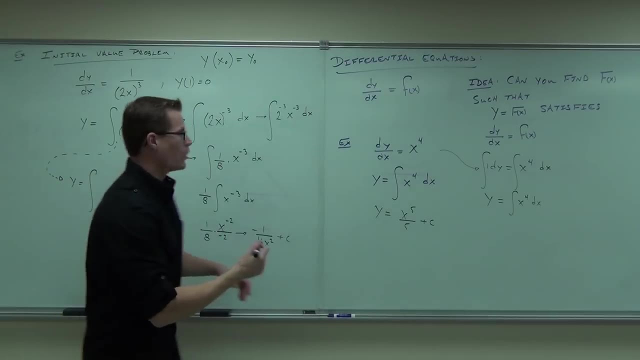 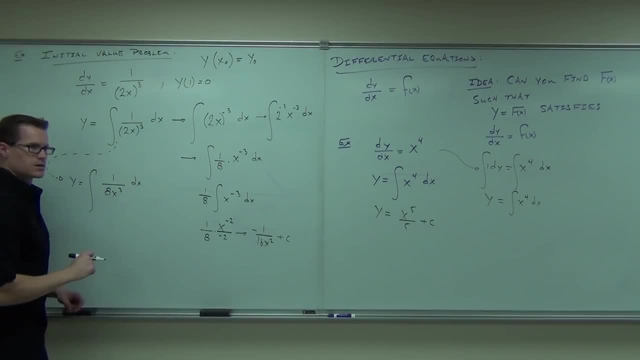 I'm lying. I'm lying. Is that it? Yes, Do you follow? Then does the 8 move to the top? No, It's just the x to the third. That's the integral of one-eighth times x to the negative 3.. 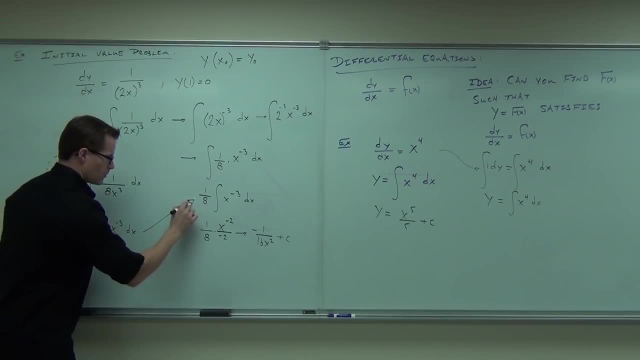 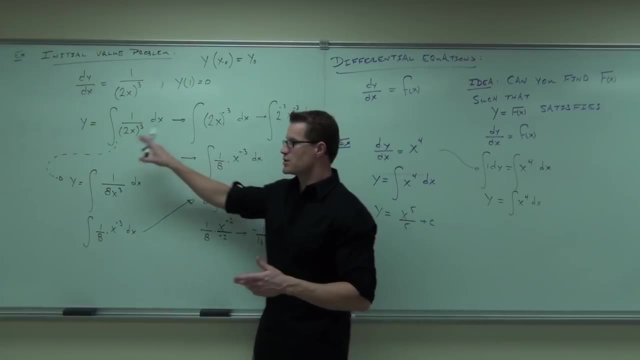 And that gets you right to that step. Can you follow that one as well? So, either way you want to do that, I really don't care, But sometimes it's easier to deal with those parentheses first off, before you start moving all these pieces around. 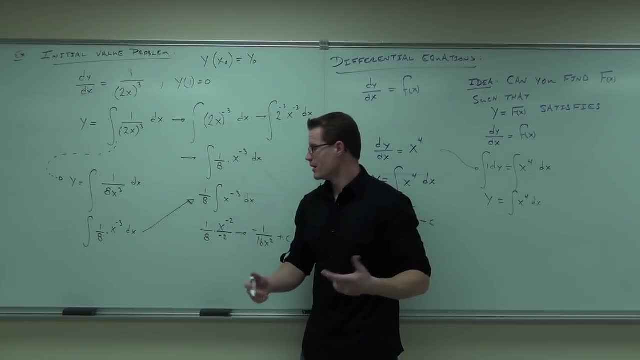 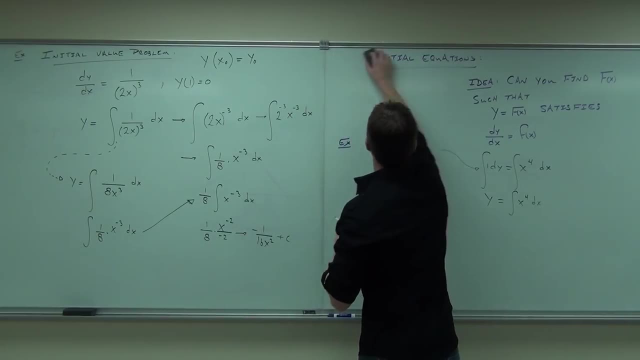 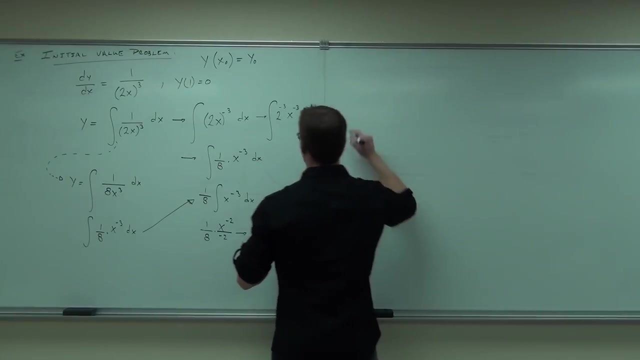 because you have to end up moving it back down to the denominator in the first. give down to the denominator anyway. In either case, though, we're going to get negative 1 over 16x squared plus c. Tell me what I found. 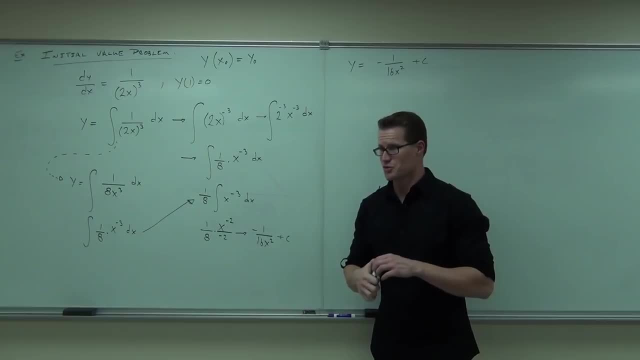 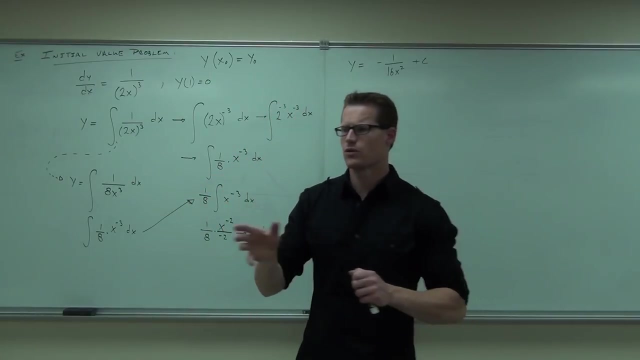 What is it? It is an integral, yes, It is an integral. A family of what Functions, Functions works, Family of functions that does what for us? What does this family of functions do? Solve your initial, What do you mean solve for? 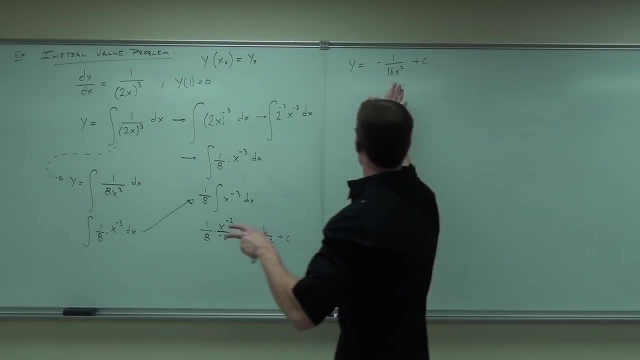 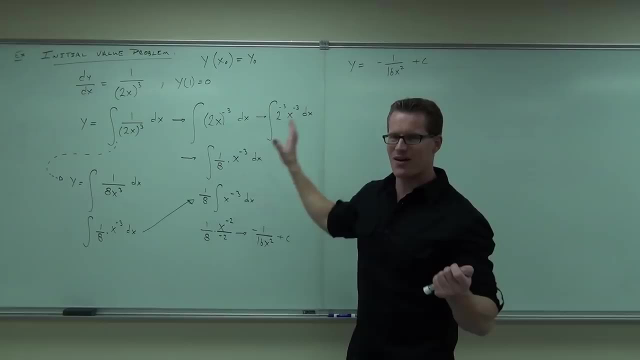 Someone over here tell me, what does this family of functions- I said it wrong functions- represent for us? Come on, help me out. We've had two ways to represent this Way. number one was: what's an integral or an anti-derivative represent? 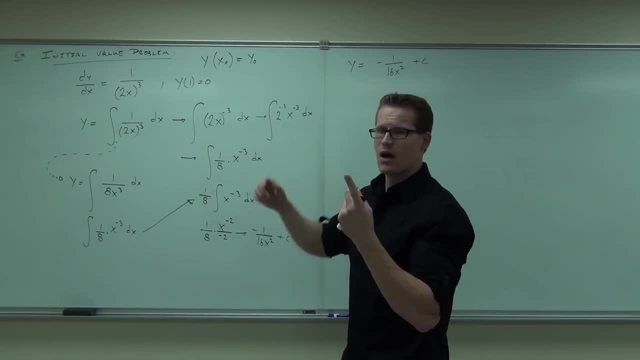 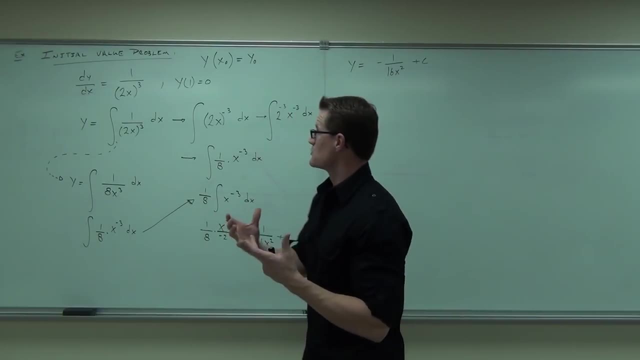 Represents areas. We can consider that as an area, because that's an integral. yes, In this context, this one, this is a family of curves such that when I take a derivative of it, it gives me that exact thing. Do you follow? 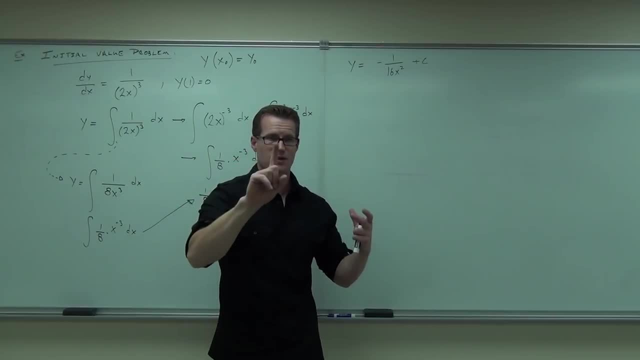 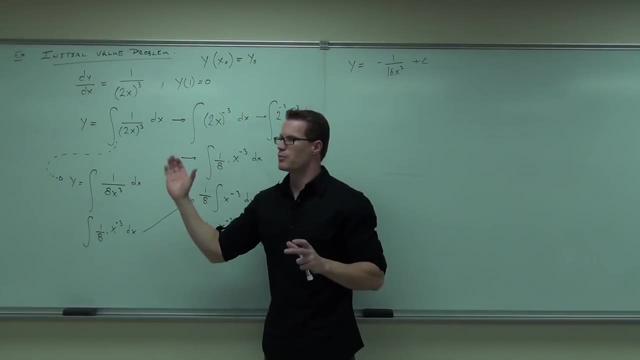 That's what we're representing: a family of curves. How we find one specific curve or one specific function is we use the initial value. Now, this is basically the same idea as me giving you a point before, Only I'm not giving you a point. 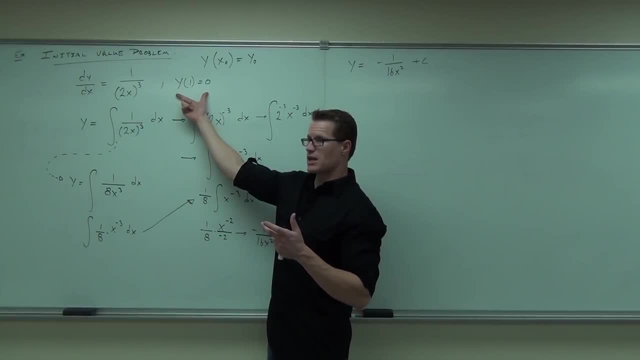 I'm not giving you a point explicitly, I'm giving you a point right here, like this: I'm saying: I'm not saying what x is, but you should know what x is. What is x here? One And y is zero. 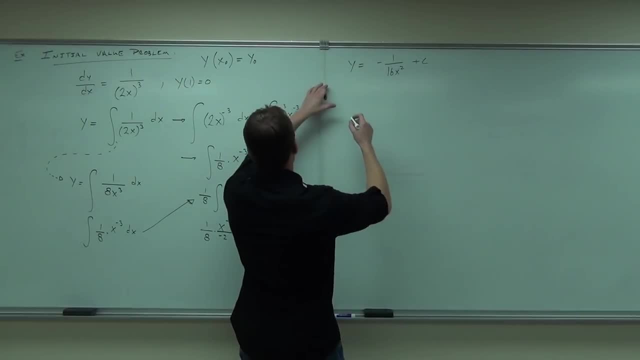 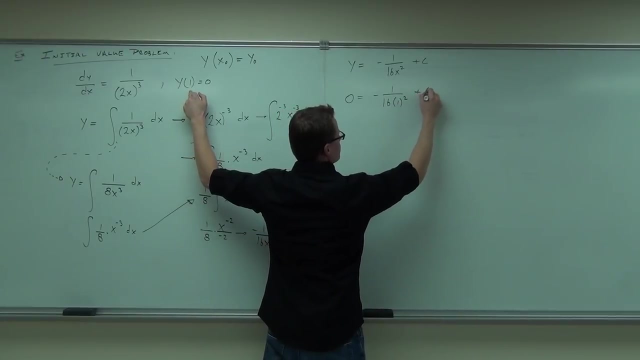 It says y of one is zero. So what am I going to plug in? Well, let's see. It says the initial value for y. the initial value for y is zero. The initial value for x is one plus c. That lets you solve for c. 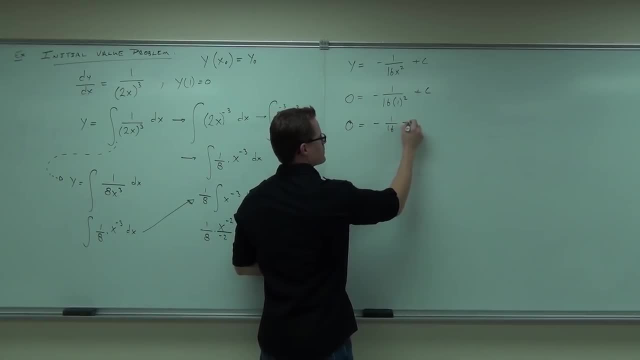 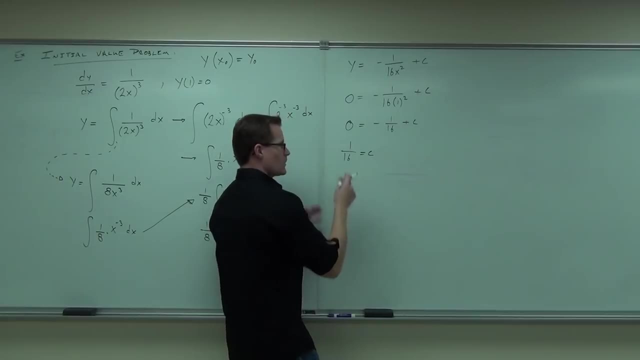 In our case we'll have zero equals negative one-sixteenth. This is kind of nice and easy In this particular case. you add one-sixteenth and you get one-sixteenth equals c. Substitute that back in And the exact equation that we're looking for to satisfy not only the differential equation. 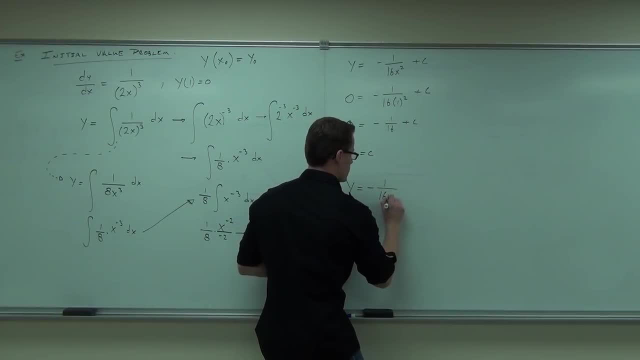 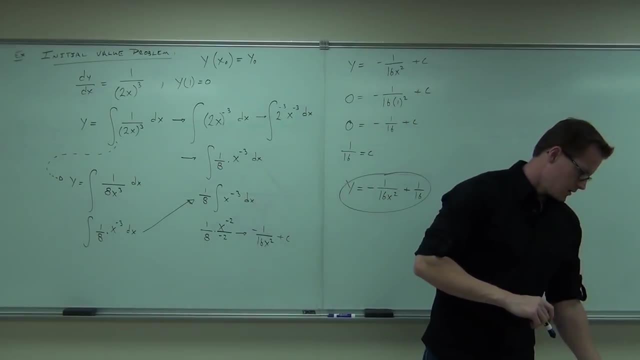 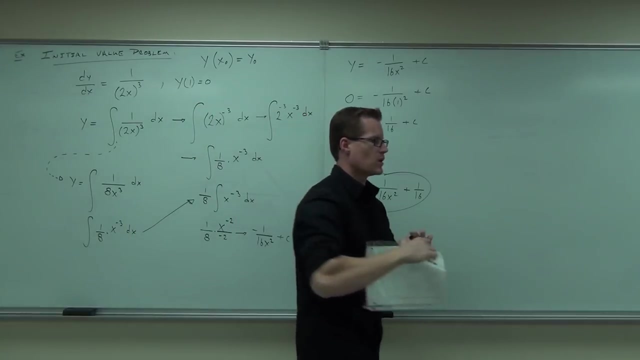 but the initial value is this: Let's try one more. just to make sure you really grasp this. I'll show you an example of how you can do it in actually real life, how this stuff works for you, and then we'll be done for the day. 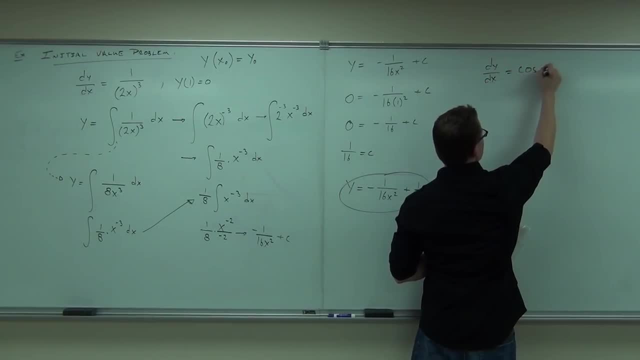 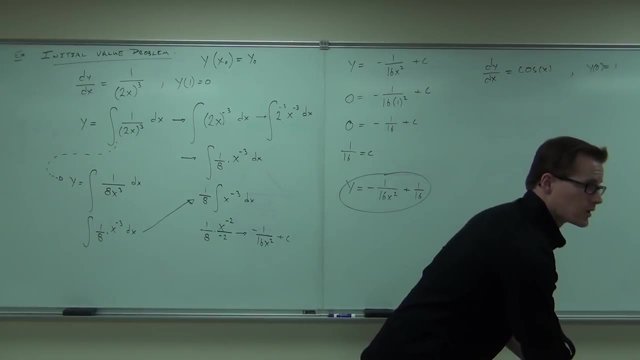 So last one. Let's say dy dx is cosine x. Initial value is y of zero equals one. This one's going to be nice and quick for us. We're going to go quickly through it. If dy dx equals cosine x, y has to be equal to c. 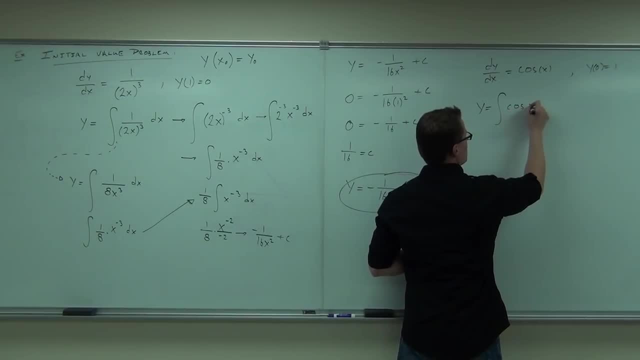 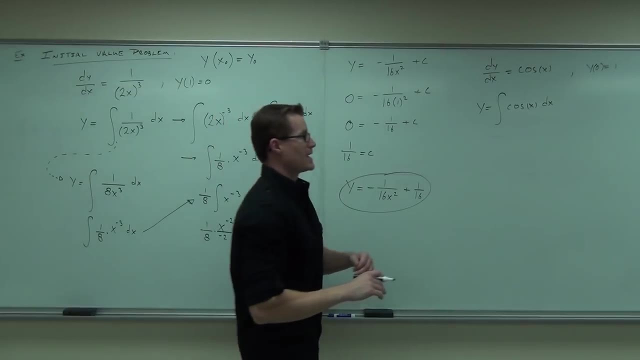 So we're going to do that. It has to equal the integral of cosine x dx. We know that. We know that that is going to undo that derivative. So, hey, can you tell me what's the integral of cosine? Think about it before you answer. 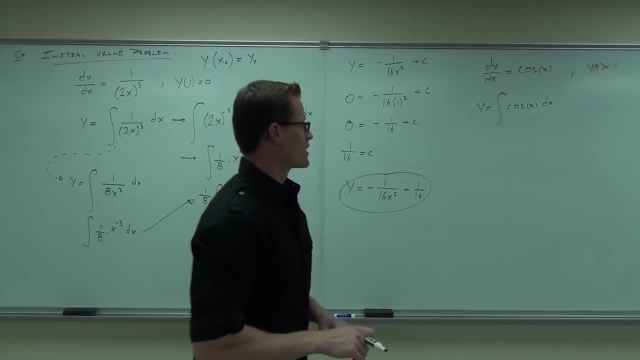 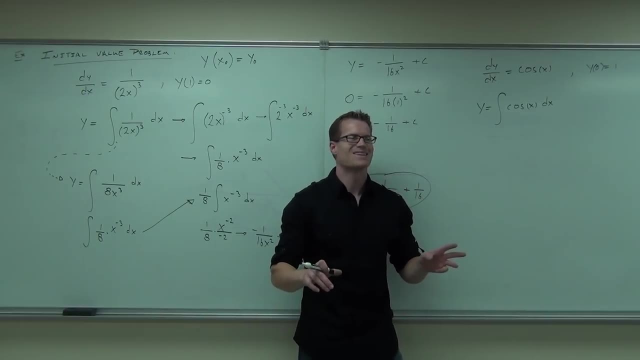 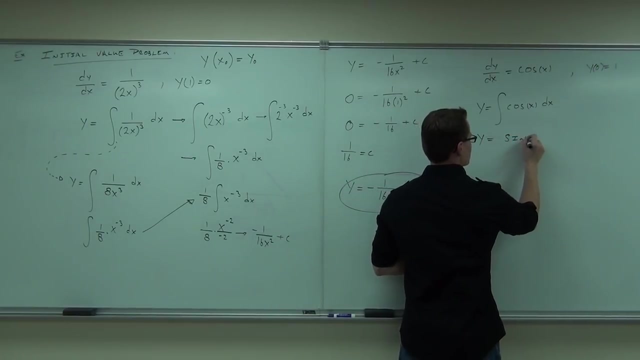 I don't want anybody answering in the first two seconds what you think. Think of the integral of cosine x. Double-take it. What is it? Sine or negative? Sine or negative Positive? Positive sine, Positive sine. What's the derivative of sine? 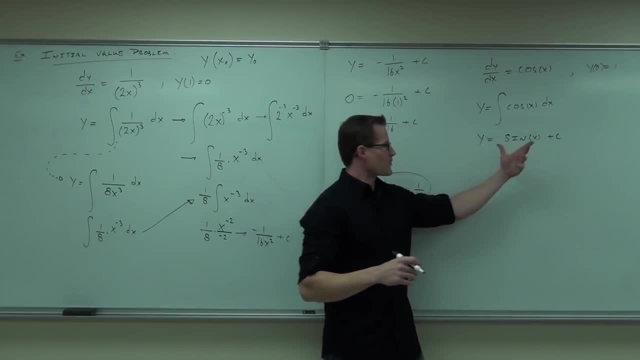 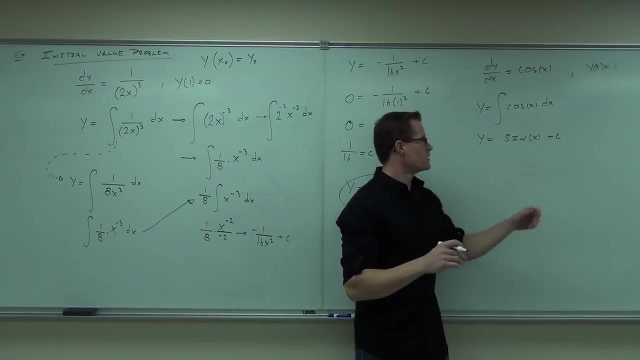 Plus c. The plus c is important, right? Hey, if you forget the plus c, that initial value is meaningless, isn't it? You got to have that plus c to solve for something, So you had to have that. Do you see why? it's sine, by the way. 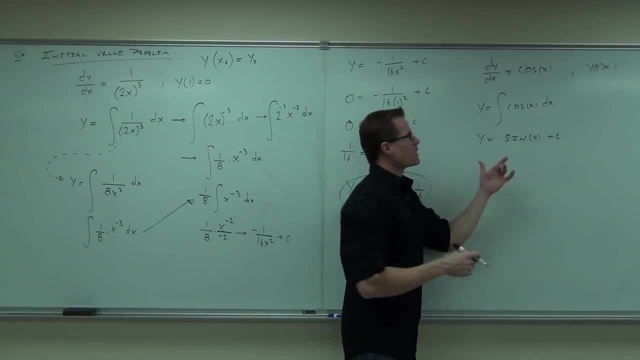 Take a derivative of sine. you're going to get cosine. Now we plug some numbers in. What do we plug in for the y in this case? That's my initial value. Is y zero or is y one? Which one One? 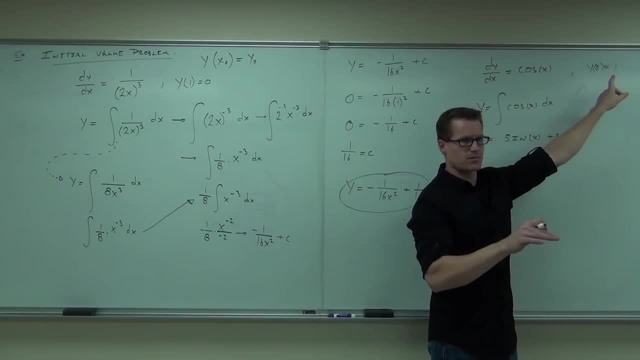 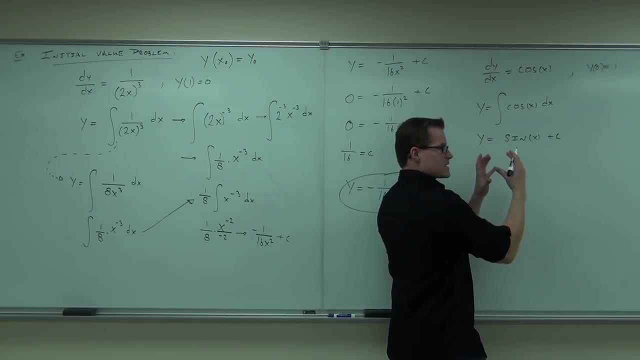 Y of zero gives you one The of zero, that's your x. This would be like y of x, That's y of one One. So I had it right here. Y of x equals y sub zero. So our x is zero, our y is one. 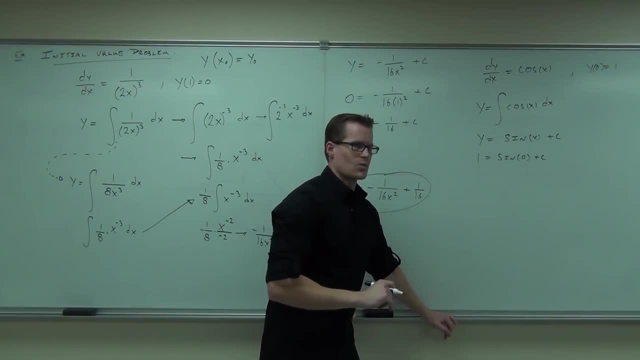 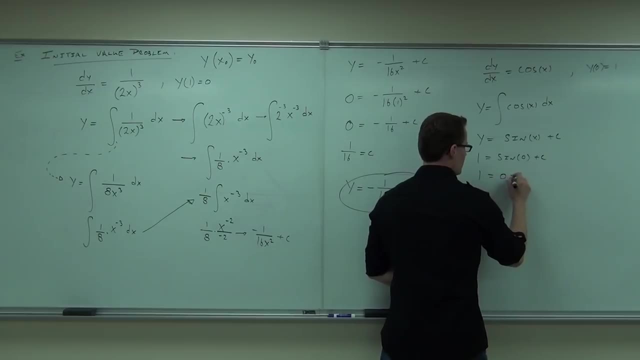 How much is sine of zero, Zero, Zero. Oh boy, some of you are killing me today. How much is sine of zero? Zero, It's zero, It's definitely zero. yeah, One equals c. No, you guys are right. 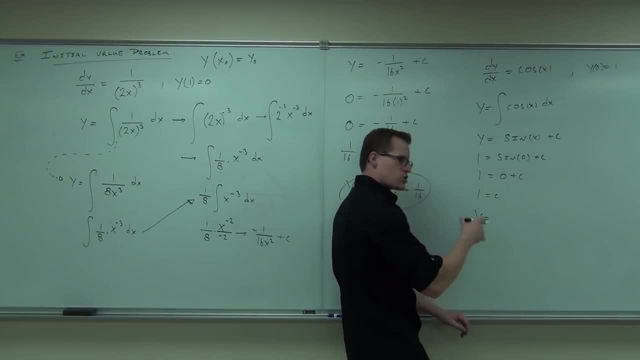 One equals c. So our function that we were looking for is sine of x plus one. Is it true that the derivative of this is going to still give you cosine x? Yes, Yes, Is it true that it goes with that initial value? 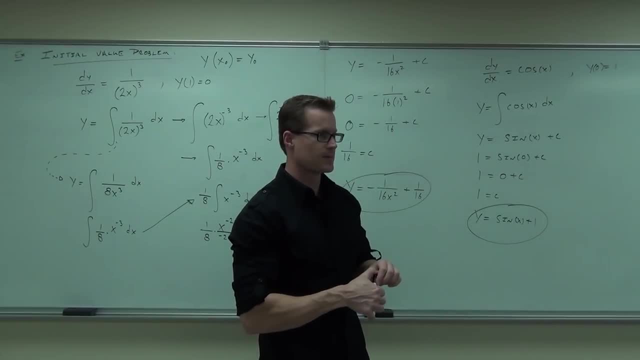 Absolutely. Being that x is zero, that means that y, it would be the y intercept. So whenever you have the y intercept, would c always come out to be the same? Yeah, It should. yes, Yeah, absolutely. Because you're plugging in zero for x, it's got to be on that y axis. 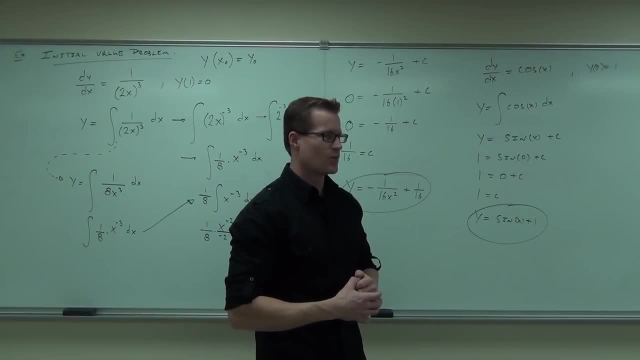 Special case. I suppose It's kind of nice When you think about it. when you do an integral right, you're always going to have something in terms of x or whatever your variable is, plus some c which does not have your variable. 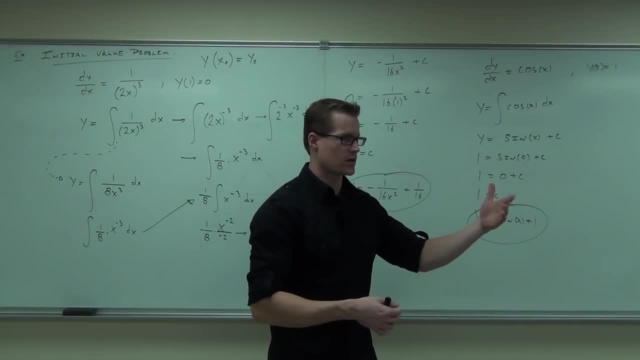 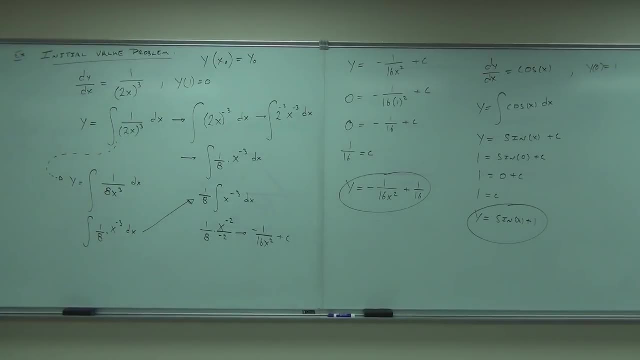 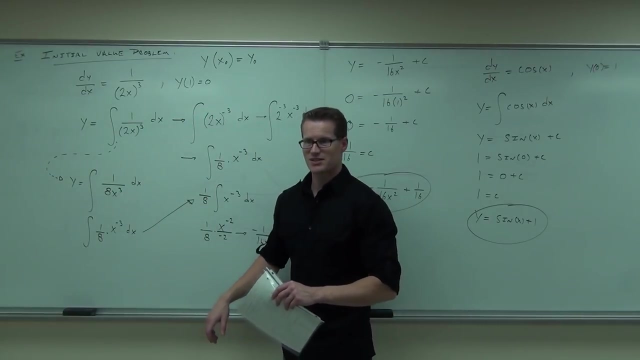 So that, naturally, if you're plugging in zero, everything else will go away. except for that. Would you like to see a real-life example? I'm afraid it's. Are any of you in physics? Not yet. Are any of you going to take physics? 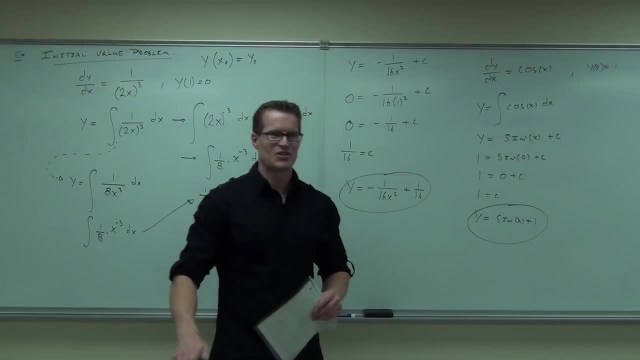 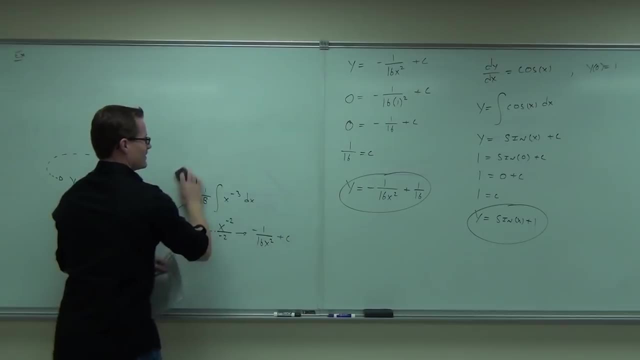 Oh good, Do you know that you can build catapults? Yes, We're going to do a catapult example. That's the main reason to take physics to build a catapult. That's what I would take it. I hated physics. 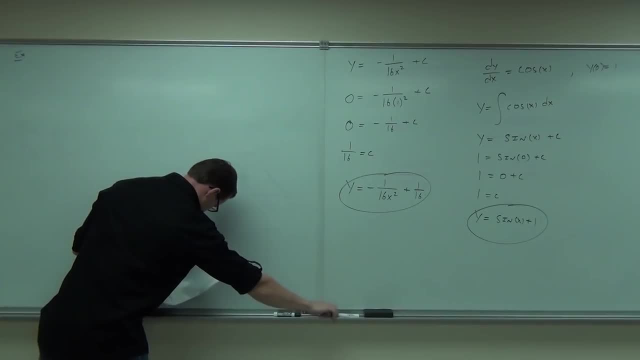 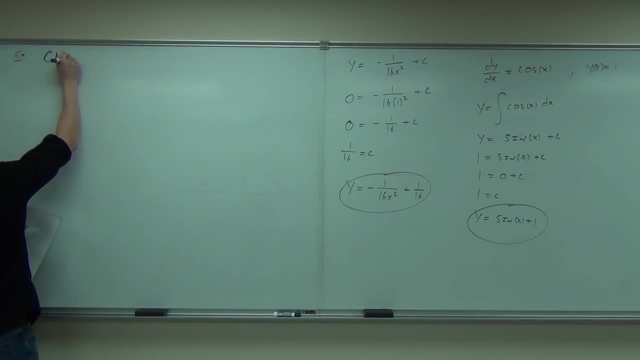 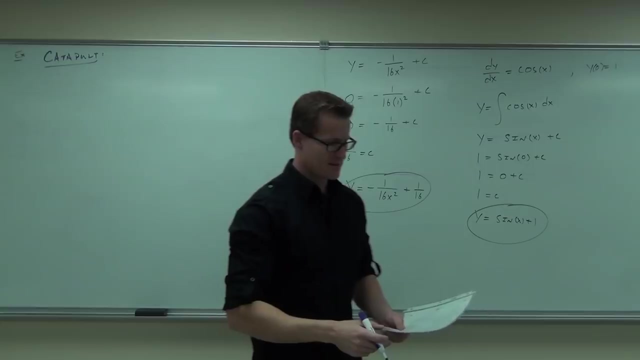 I mean, I loved it. I loved it. My teacher was not very good, Not like the teachers we have here. They're good. here I'm going to give you a catapult. Is that what you call a catapult? You know they're originally intended to shoot cats. 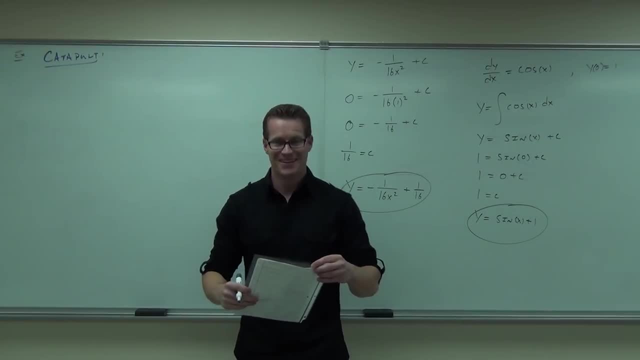 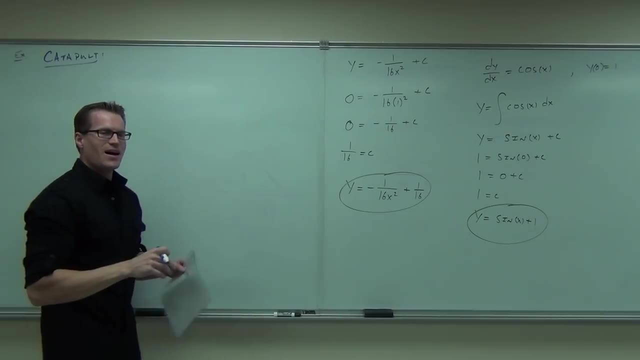 That's why it's called a catapult- Just kidding, but that would be pretty fun. I don't like cats, Especially when you don't like them. There's no cat I like. Now let's say you really suck at building a catapult. 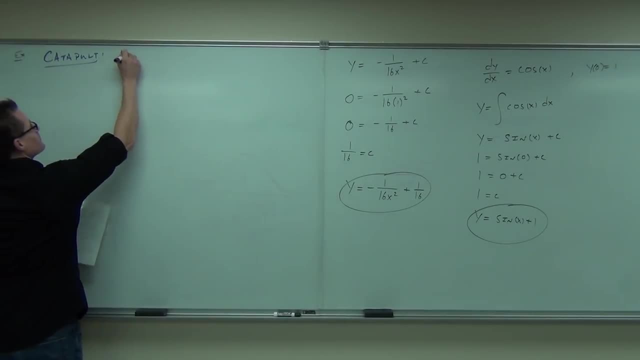 One of you guys is going to be really bad at it. I don't know if you've ever done that. It's not good. I'm going to give you a catapult. It's really bad. I'm going to give you a catapult. 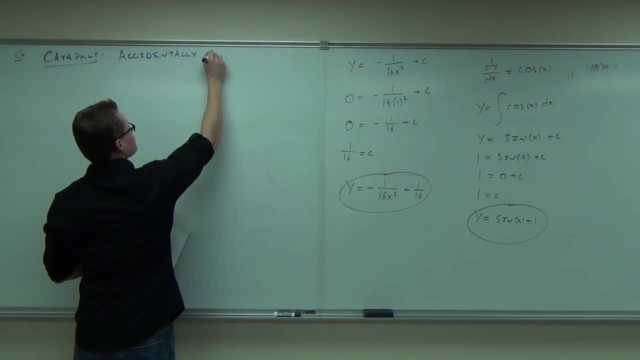 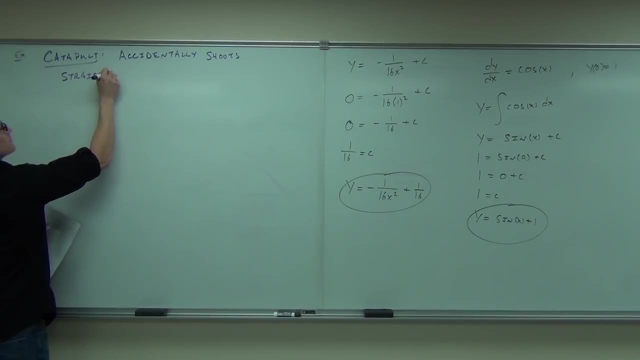 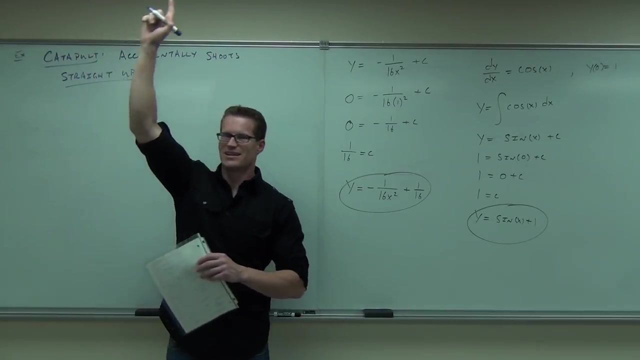 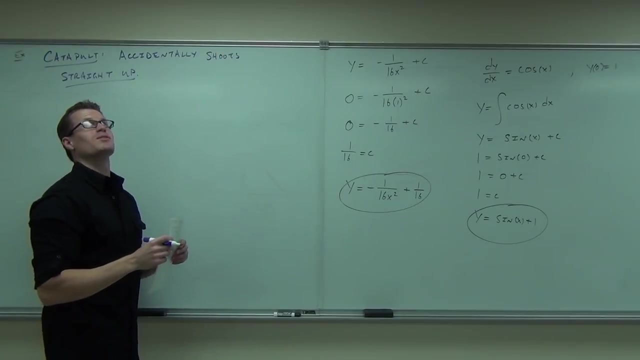 It's really bad And you shoot it accidentally straight up in the air right above your head. Is that a good thing? No, Not with a catapult. It's possible. It's possible. I've seen it happen with a really badly built catapult. 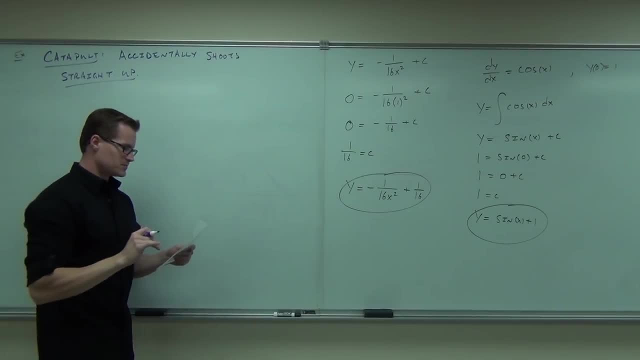 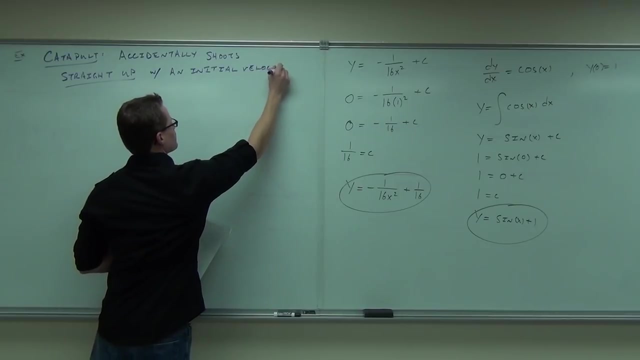 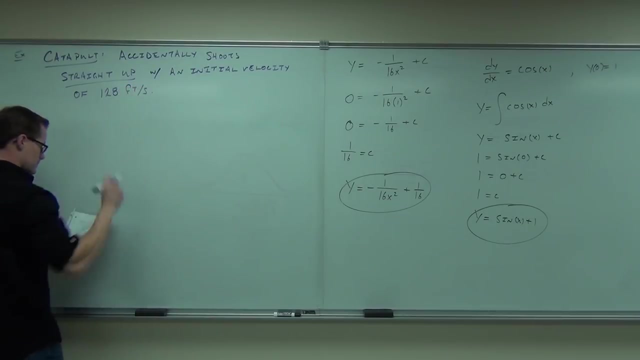 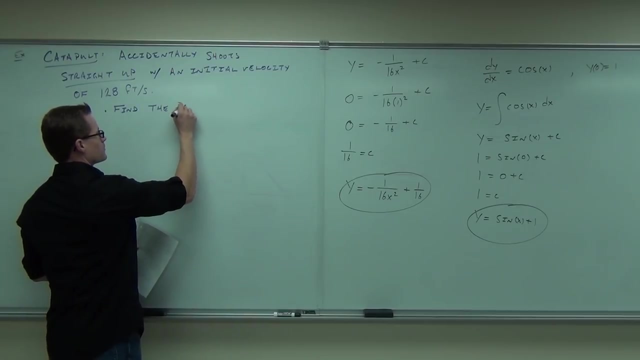 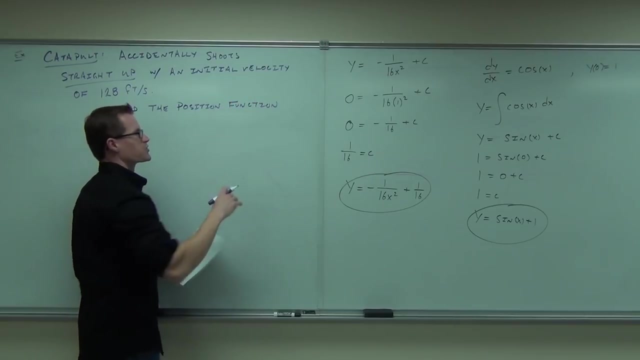 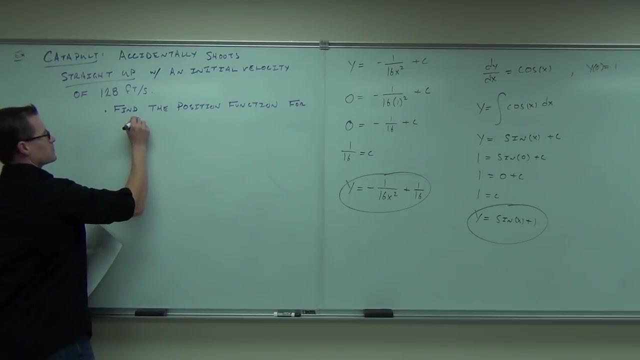 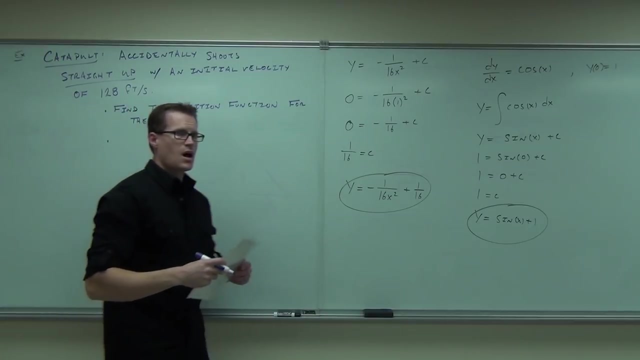 Straight up in the air. It actually shoots straight up in the air with an initial velocity of 128 feet per second. I want to do a few things. I want to find the position function of this for the projectile, basically for the height. 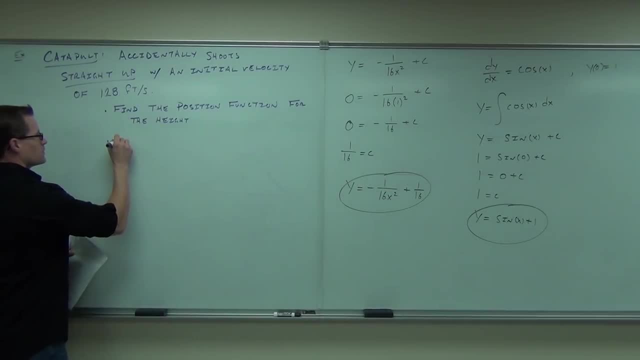 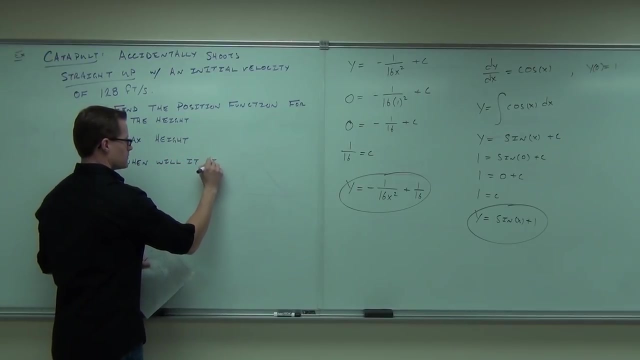 I want to know what the maximum height is And I want to know when it's going to hit you in the head. Actually, when it hits the ground. So hit your foot. When will it land on your foot? When's he going to hit the ground? 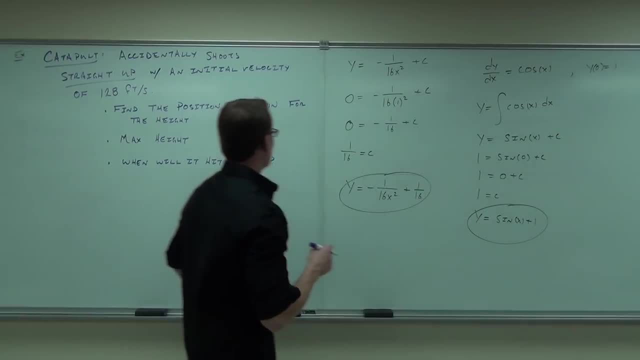 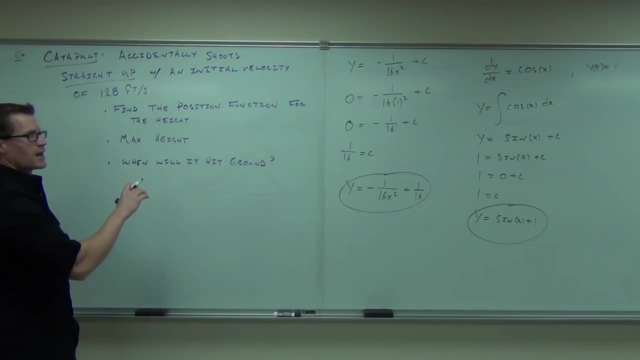 Well, let's say one more thing about this. Let's say that it actually shoots straight up with an initial velocity of 128 feet per second, and you're launching it off of a 16 foot platform. So you're up 16 feet and then you launch it. 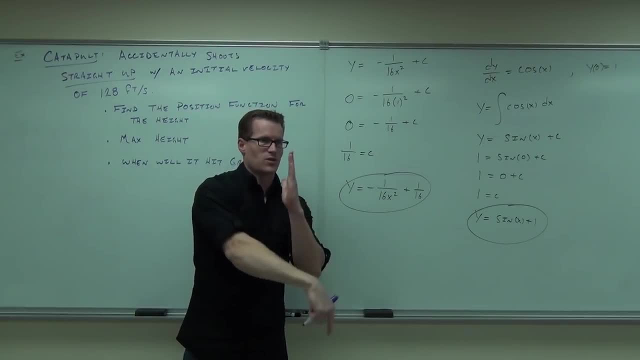 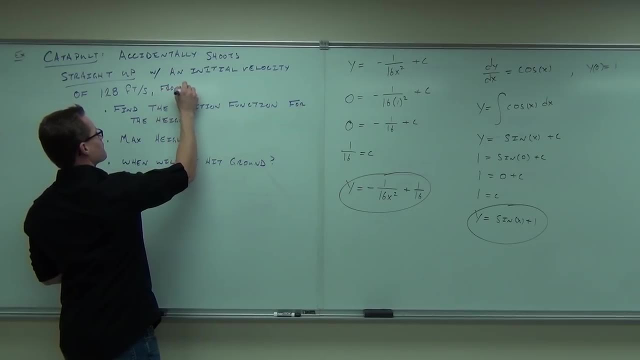 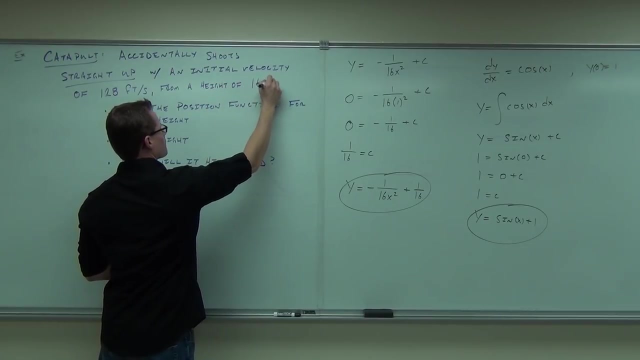 So maybe not straight up, but just slightly over, so it's going to land on the ground. Okay, Does that make sense to you? Or you move the platform real quick, Or maybe your catapult is 16 feet high, So when it starts throwing it it's at 16 feet. 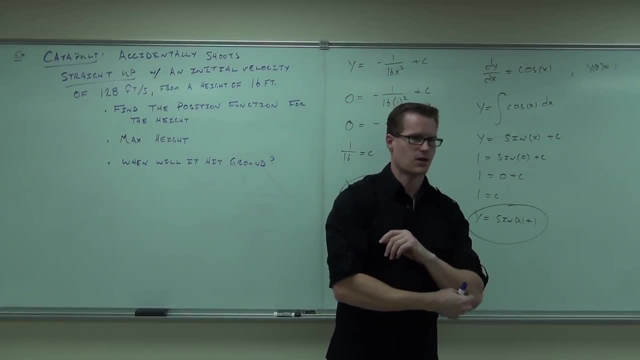 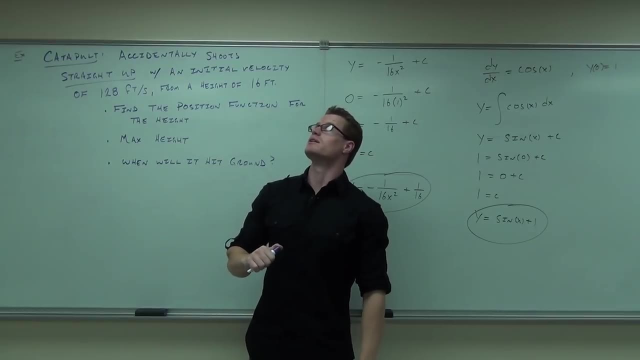 So maybe the top of it launches it straight up, Something breaks. I don't know you messed up, but it launches straight up from your huge catapult and it's going up there and you're like, oh crap, it's going to hit me. 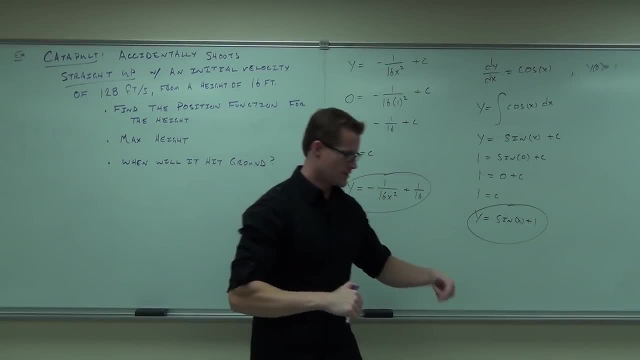 And so you just watch it and you count. Let's see when it's going to hit me. It's going to hit you. That's the idea here, Because we would all do that. naturally, Let's talk about a few things that we should know. 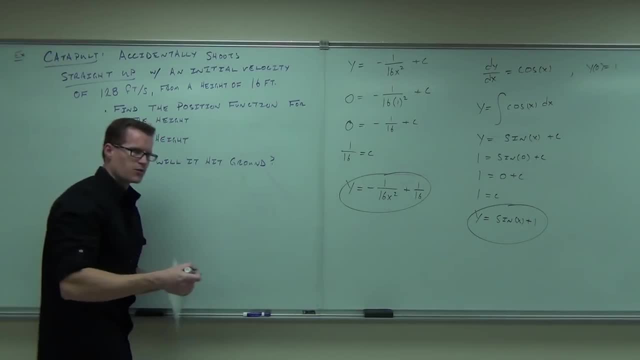 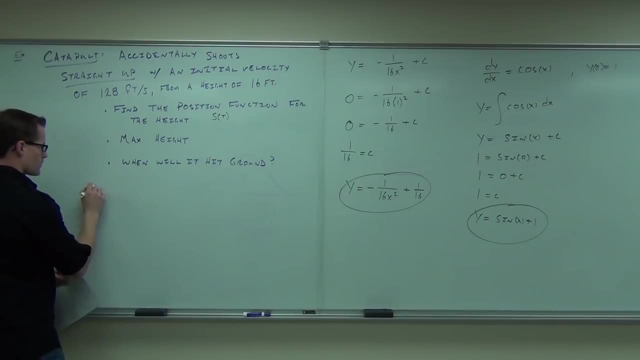 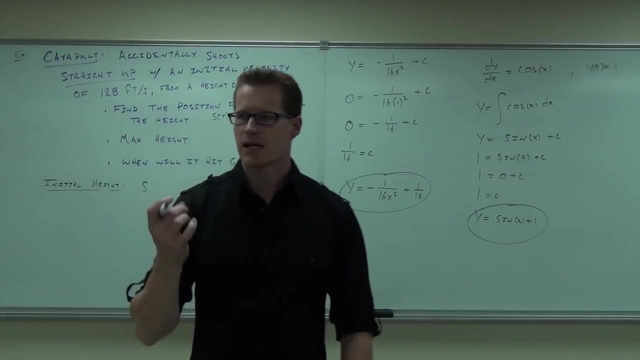 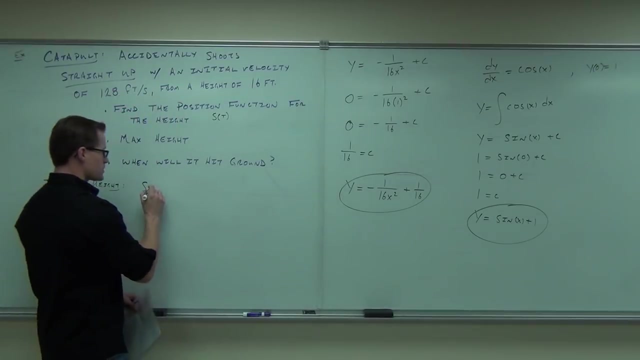 Firstly, let's call our position function S. That's typical for a position function, So S of T. according to time, The initial height, What is the height of this thing at T, equals zero Right when you launch, So S of zero is 16.. 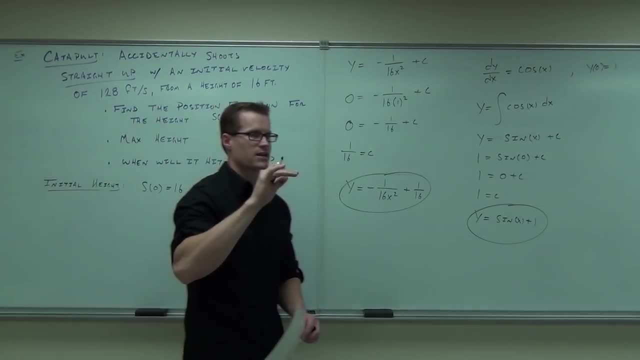 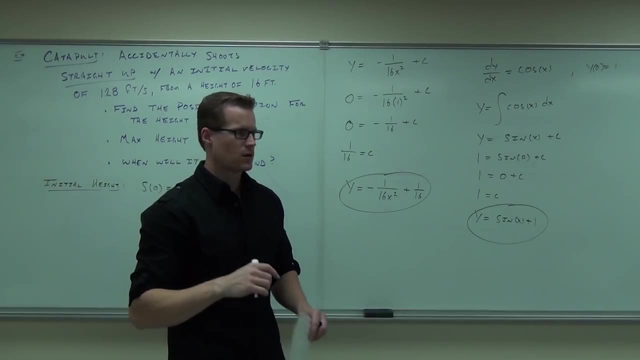 Do you follow me on that? 16 feet, So right, when it's launching it's 16 feet high, because that's when it's letting go. What's the velocity? 120 feet per second. Aha, Yeah, that's exactly right. 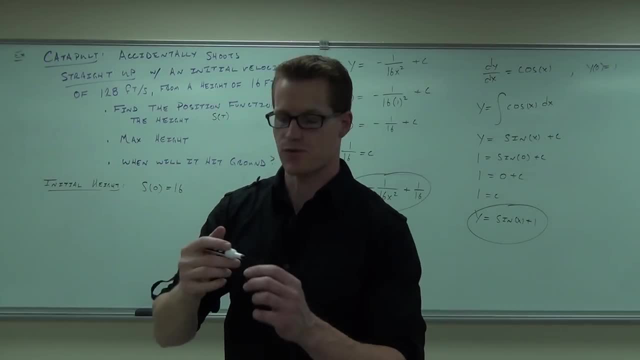 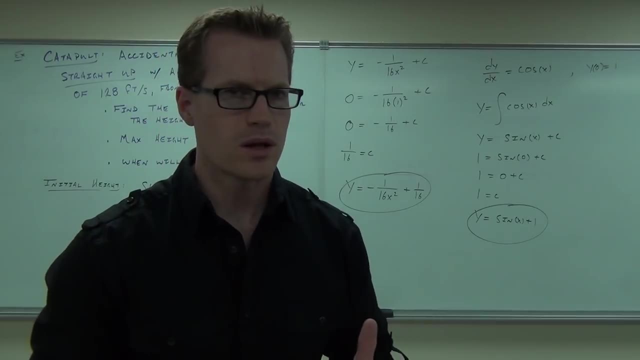 You're going positive 120 feet per second. Now here's a good question for you. What is velocity in relation to a position function? Velocity. Velocity, It's the what, The what. Second, Velocity: It is the first. Do you remember? that's the first derivative. 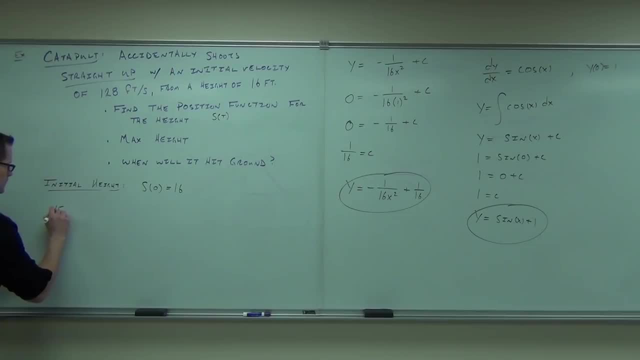 So velocity is the first derivative of a position function And it's an initial velocity. So the initial velocity, The initial velocity, is going to be this, The first derivative at time zero. Because what's going to happen to your projectile? Is it going to stay at 128 feet per second forever? No, Probably not, because it's going into outer space. It's going to slow down immediately after you launch it out of the catapult Right. Gravity is going to affect it. We're not going to do wind resistance, but gravity is going to affect it. 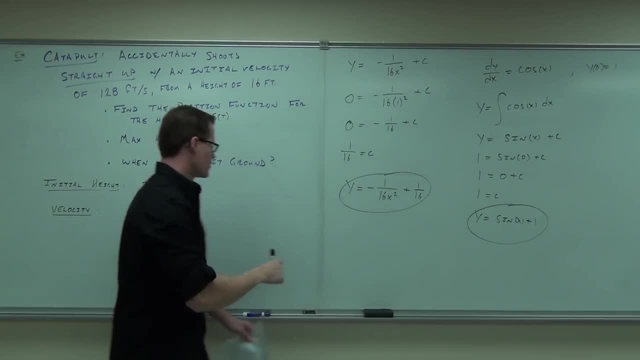 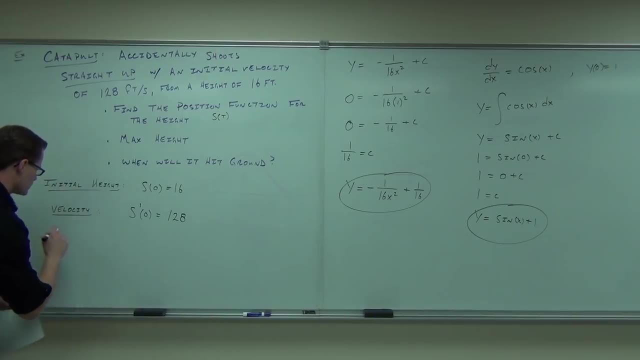 It's going to come up and then it's going to come down. True, So the initial velocity at time zero is 128 feet per second. Okay, So the initial velocity. I don't know if I spelled that right. I probably spelled it wrong. 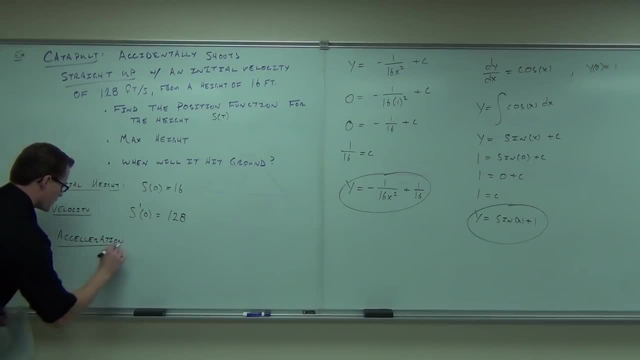 I'm not good at spelling. I think I have too many L's, Do I? Yeah, Acceleration, There we go. If you have acceleration like that, What's acceleration? I didn't say anything about acceleration, But think outside the box here. 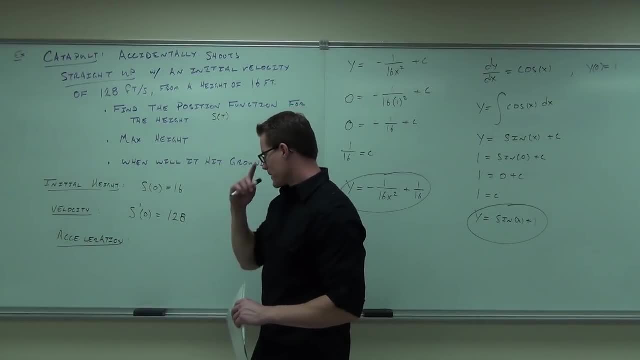 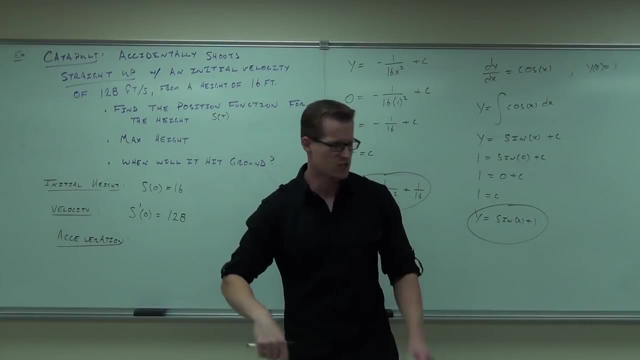 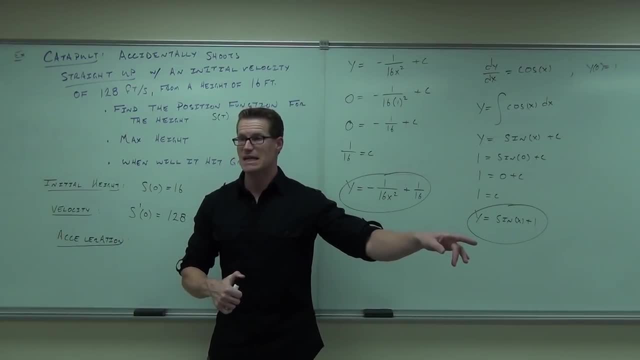 No, Now look, Now we're very good. Did you hear what he said? He said it's going to be decelerating. Decelerating It's still a form of acceleration, It's just in the reversed direction. So you're going to be accelerating negatively because he's pulling it toward the ground. 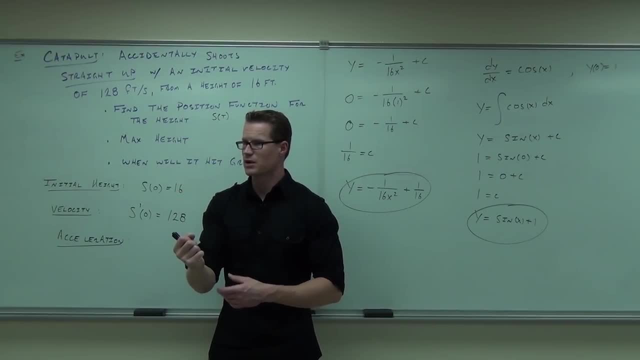 and he said 9.8 meters per second squared, which is true, but I'm talking about feet. Oh Okay, So not 9.8.. Do you know 32.? Yes, Accelerate Now. Oh wait. 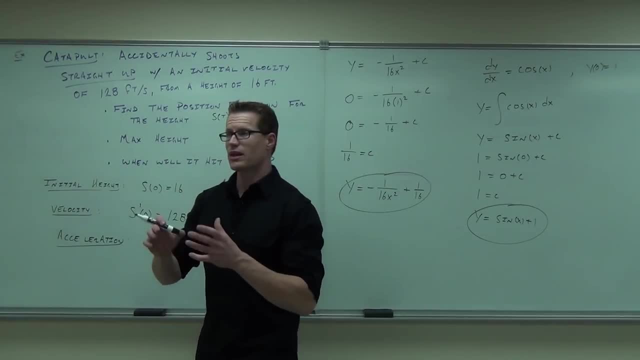 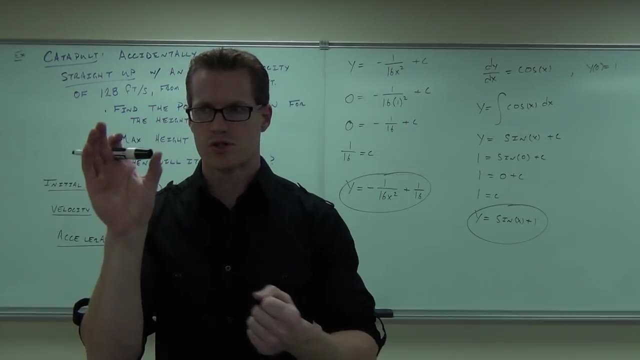 Another interesting question: Acceleration, as it relates to a position curve. Do you remember all this? Rates of change? position function was a position. The first derivative gave you velocity, The second derivative gave you acceleration. So here's what we know. 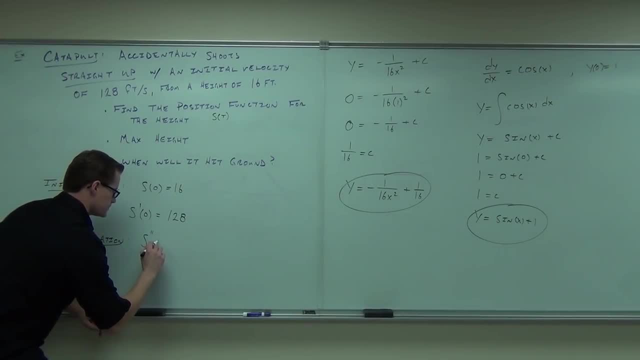 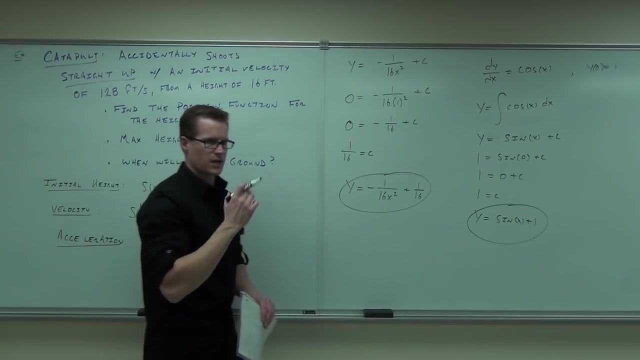 We know the second derivative. Actually, that's gonna be a constant, isn't it? The second derivative is negative: 32 feet per second squared. Why is it a constant? Well, gravity doesn't change for us, So it's gonna be pulling down a constant acceleration. 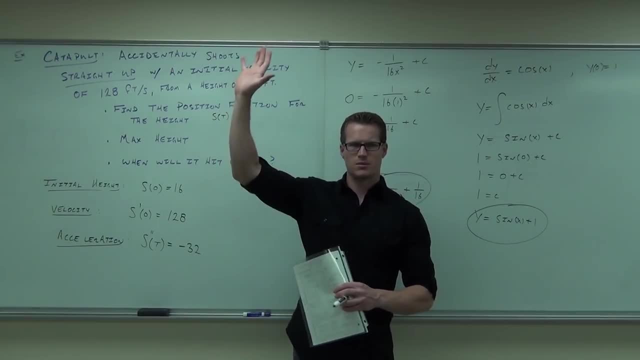 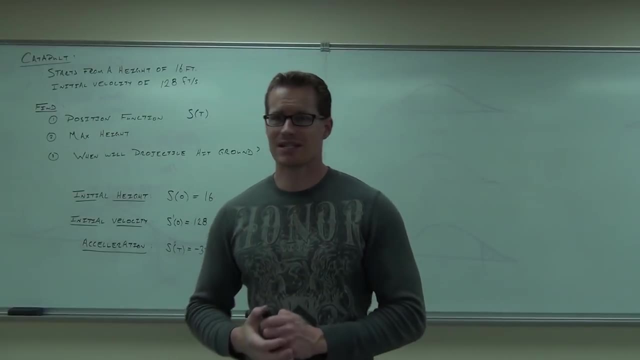 of negative 32 feet per second squared. How many people feel okay with our setup here? I'm gonna show you what to do with this next time. We'll start here. We're gonna continue talking about our catapult problem and here's what we knew so far. 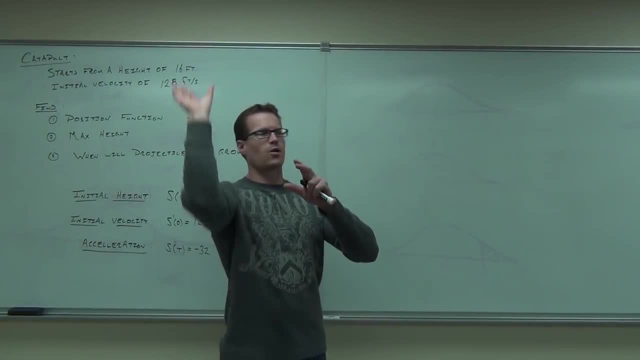 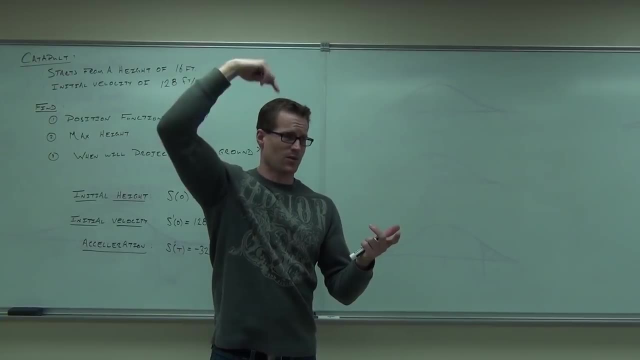 We're launching from a catapult and as the projectile leaves, the arm reaches up and reaches the maximum height of 16 feet. and then let's go and this thing shoots straight up in the air. because you built it wrong. It's gonna have fallen on the ground right in front of you. 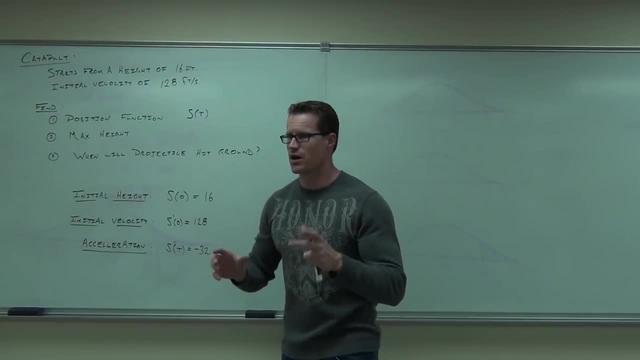 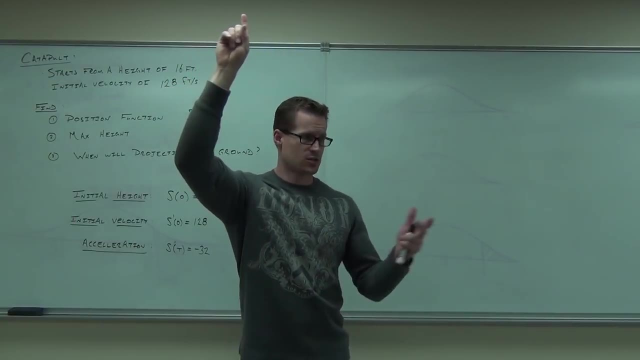 Got it. It leaves the catapult with an initial velocity of 128 feet per second. Now, what's gonna happen as soon as it leaves the catapult? What happens to that projectile Deacceleration? It starts slowing down. that's right. 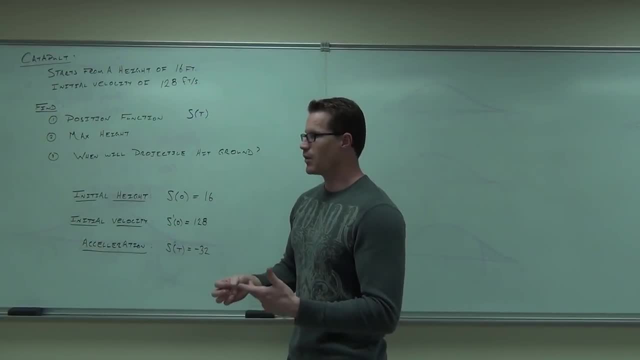 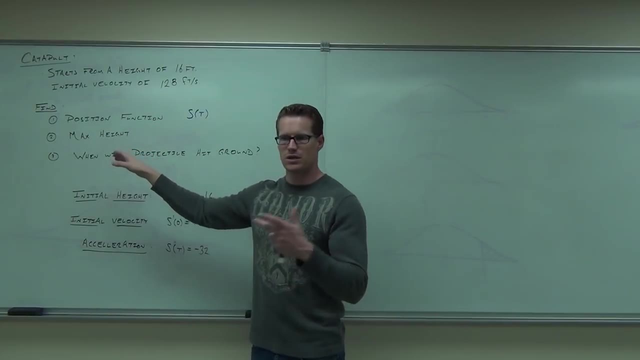 The velocity starts slowing down because gravity is affecting it. Now what our goals here are to do is find the position function that's positioned according to time, find the maximum height. we can do that. We already know how to find maximum and minimum. 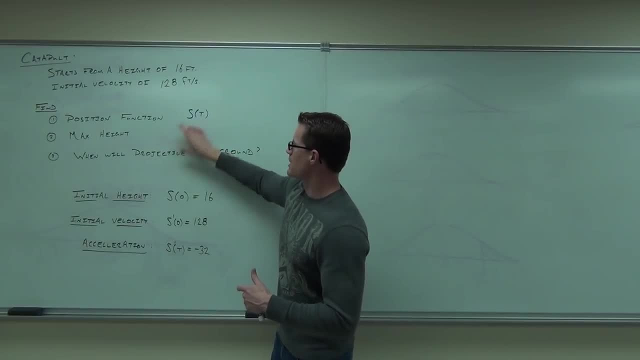 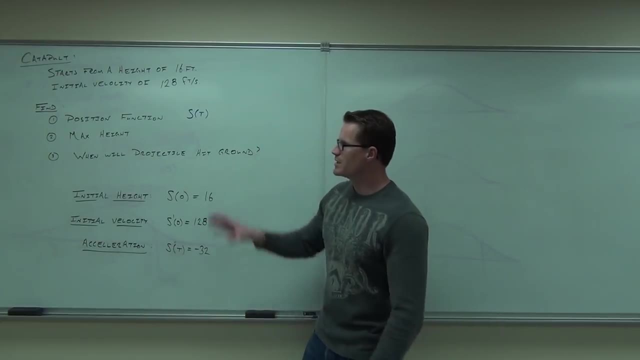 and we're gonna find out when the projectile will hit the ground. This is gonna be based off our position function, The maximum height. we're probably gonna have our first derivative for that. You with me on this. So what do we know initially with our problem? 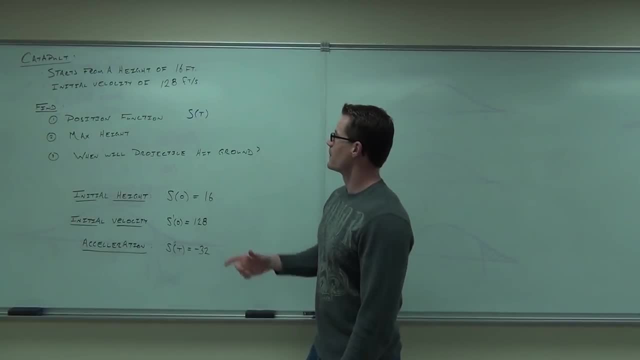 Well, we know that it's starting out at 16 feet. So I said it starts from a height of 16 feet. That's because our catapult arm reaches a height of 16 feet, and then let's go. So the position at time equals: zero isn't zero. 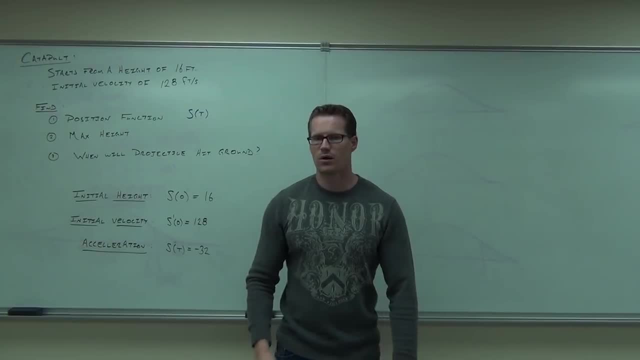 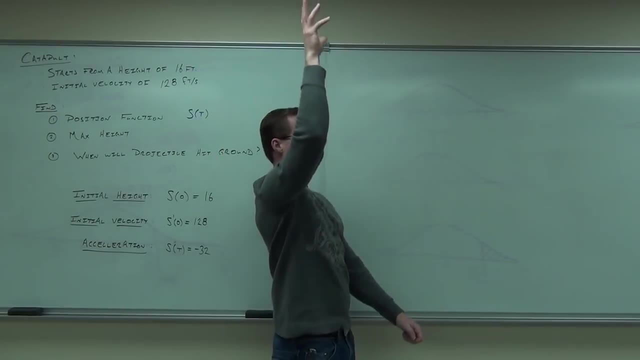 It's 16.. It'd be like a pitcher throwing a ball. If the pitcher throws a ball, the ball doesn't start from zero, right? He's not gonna go. uh, that'd be the worst pitcher ever. He's gonna throw it from up here, right? 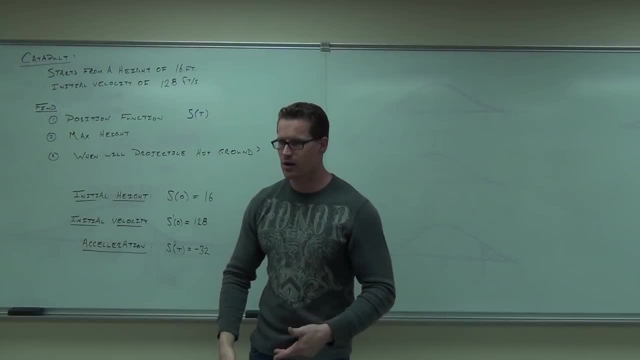 It starts from like eight feet and then goes up. It's not gonna start from the ground. Same thing with our catapult. So the position at zero is 16 feet. The first derivative gives us velocity, So our initial velocity is 128 feet per second. 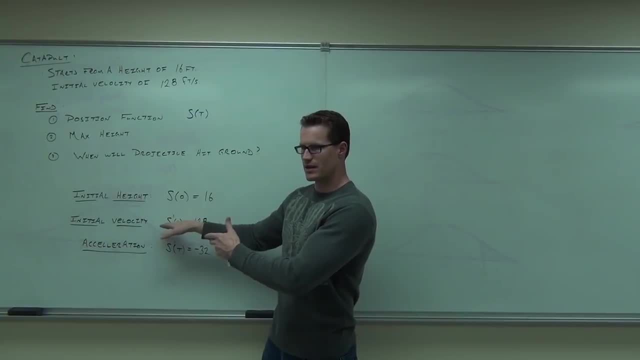 That means that our initial velocity at zero- that's where we start right here- the velocity at zero has to be 128 feet per second. Right when it's leaving, it's traveling at 128 feet per second straight up. Are you guys okay with that? 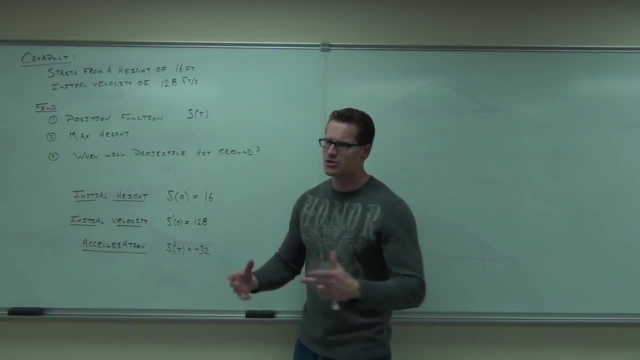 All right, now acceleration. How we came up with acceleration isn't magic, It's just something to do with the Earth's gravity. It says that acceleration's negative 32 feet per second squared, It means that gravity's pulling everything with that acceleration. 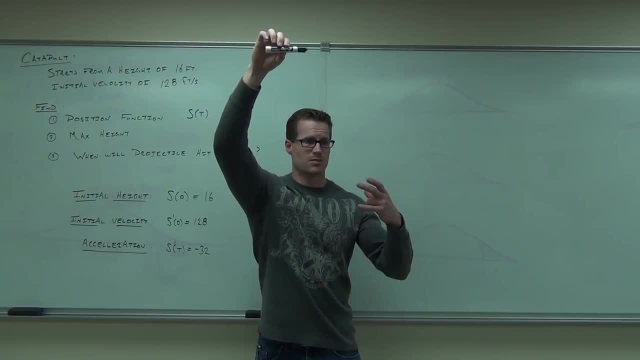 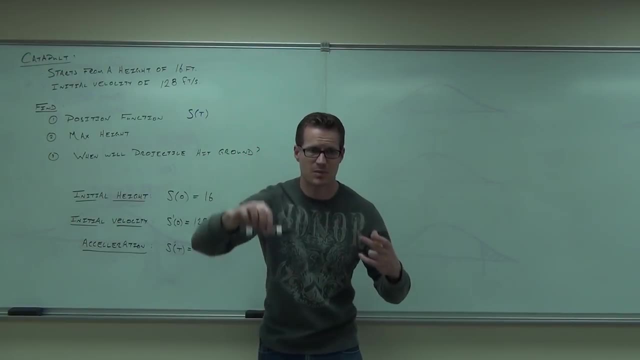 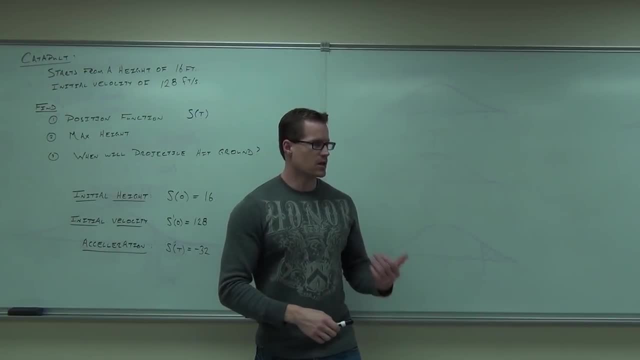 You follow me, And that acceleration that's acting on it is a constant negative 32 feet per second. squared, That means that the velocity changes at 32 feet per second every second. So it drops. after one second it'll be at negative 32 feet per second. 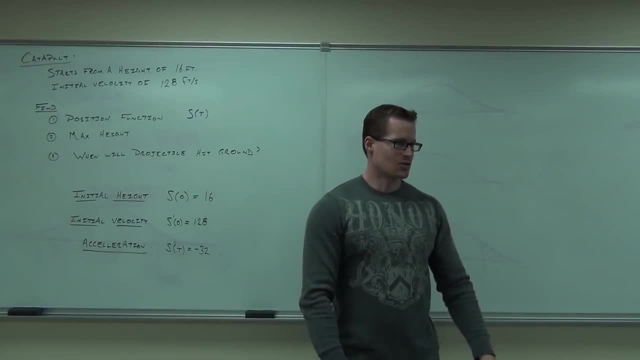 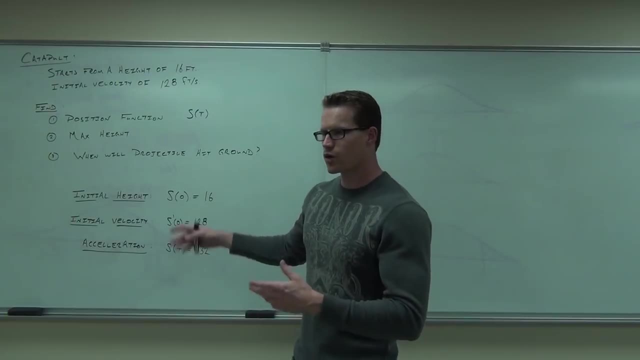 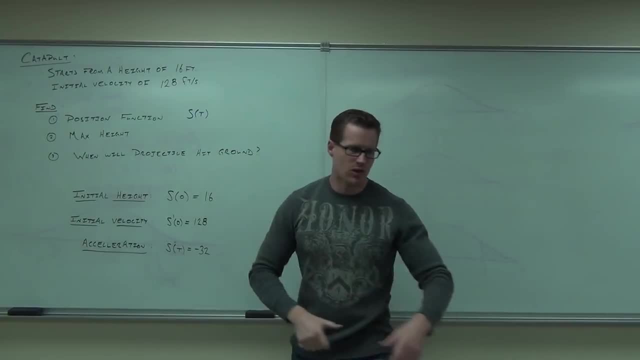 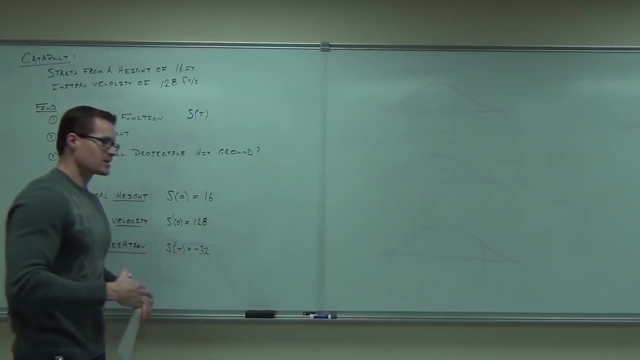 So let's try to work on that. First thing right now, what we know is basically we only know the second derivative. Notice how this is S, prime of zero and S of zero. We don't have a position function, We just know something about the position at zero. 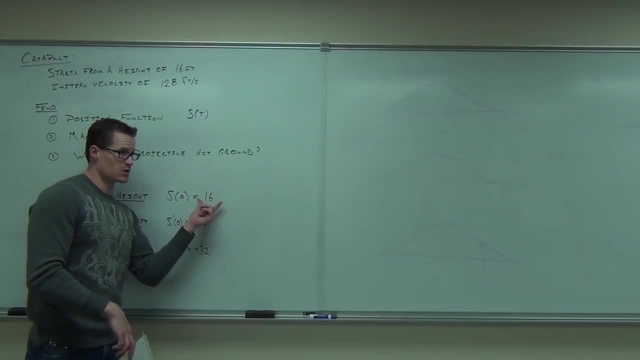 We don't have a velocity function. We just know something about the velocity at zero. at time equals zero. Are you with me on this? What we do know is that the velocity at zero is the same as the velocity at zero. It's the acceleration function. 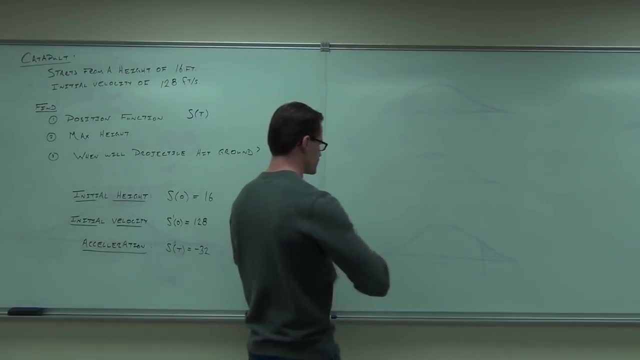 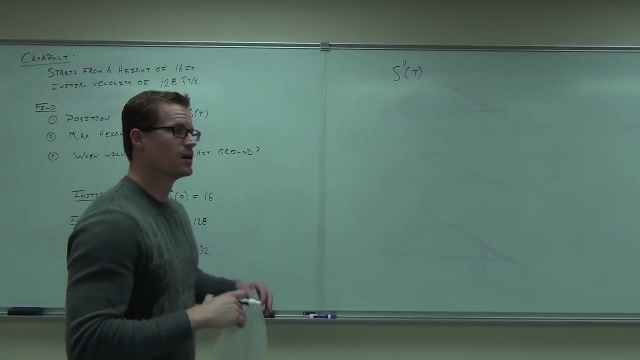 That's all we know as a matter of fact. So if we know that we've got the second derivative, the acceleration function in terms of T, Can you explain to me how I could get maybe somewhere else besides that? 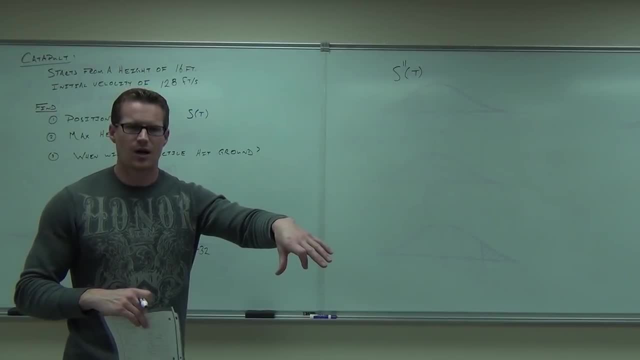 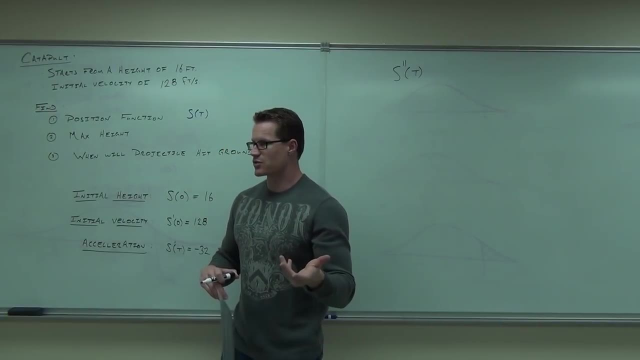 Not taking a derivative because that would give me a third derivative. I don't want that, But is there a way I can get from here to maybe one derivative higher? Better, If we integrate the second derivative, it must give us the first derivative. 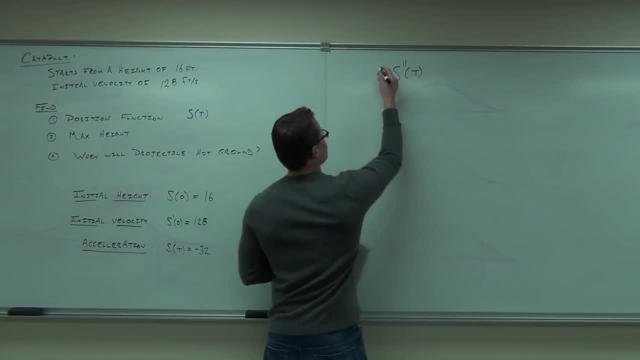 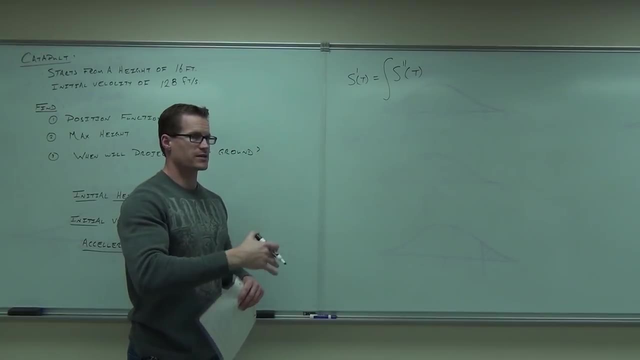 Does that make sense? Well, it's kind of an interesting concept and that's going to work for us. So here's what we know: S prime of T is going to be the integral of S double prime of T. The first derivative is the integral. 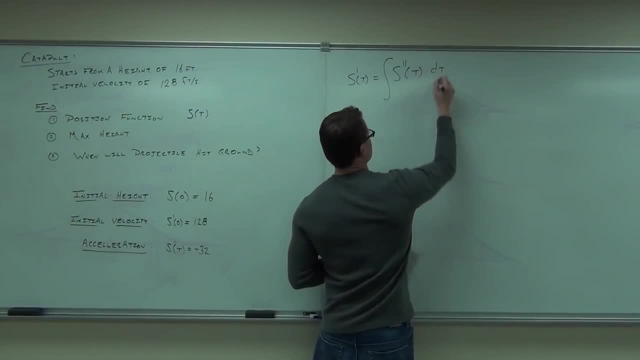 of the second derivative. And, of course, you need a DT. Are you okay with that one? All right, Now, why are we doing this again? Well, we don't have the velocity function, We just have the velocity at zero. 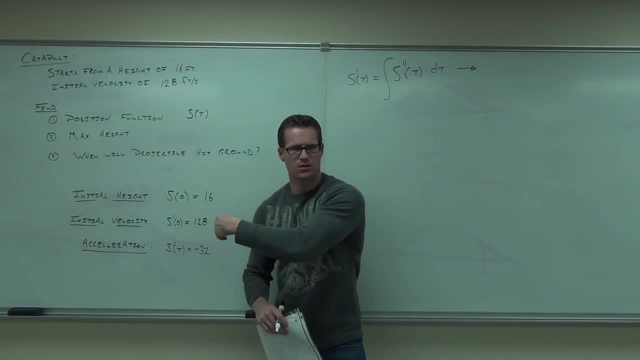 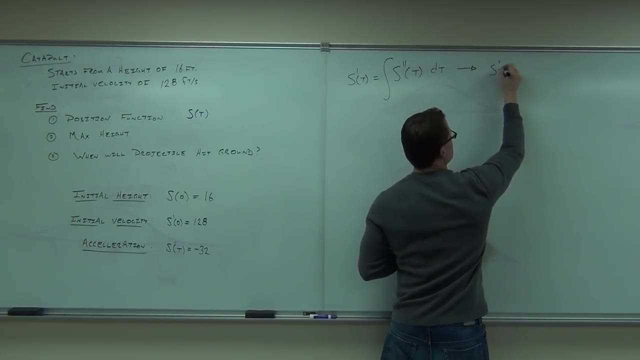 So this is actually going to help us Remember the initial value problems that we did earlier. This is basically what that is, So this says: all right, my first derivative is going to be the integral of whatever my second derivative was. 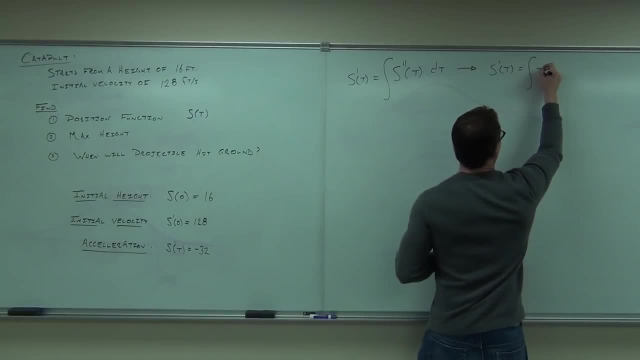 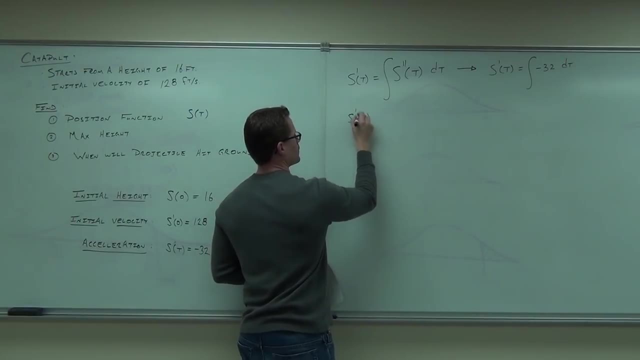 In this case it's just negative 32.. Well, that's a pretty easy one. What's the integral of negative 32 DT? Can you tell me that? Negative 32 T plus C T. why not X? Because our first derivative is T. 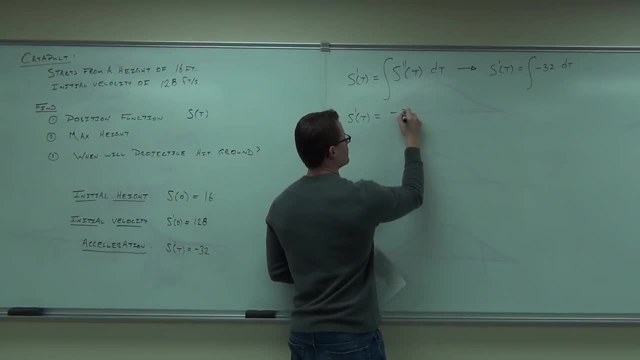 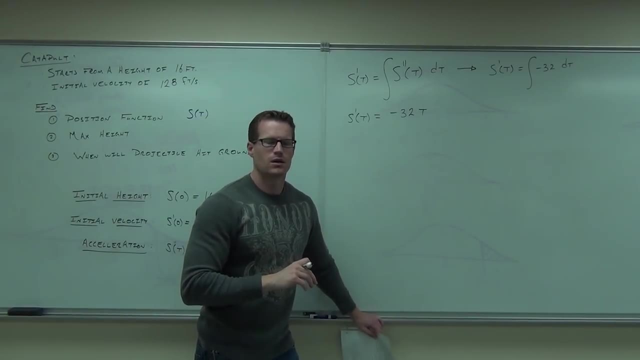 Yeah, it says T. Might as well, use T Negative 32 T. oh wait, and you said: what F plus, C Plus? is a C important? Yes, Okay, A student asked me today: why is the C? 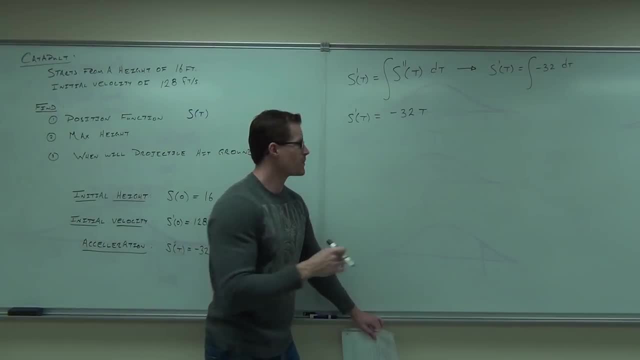 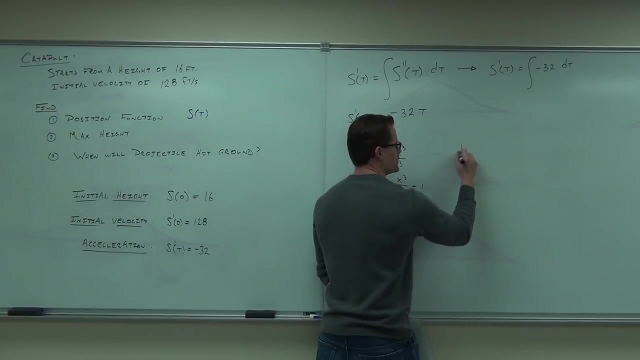 Why do you even need the C? And the answer is: well, if you take a derivative, let's say this and this and this. you don't have to write this down, just kind of watch right here. If you took a derivative of all these things, 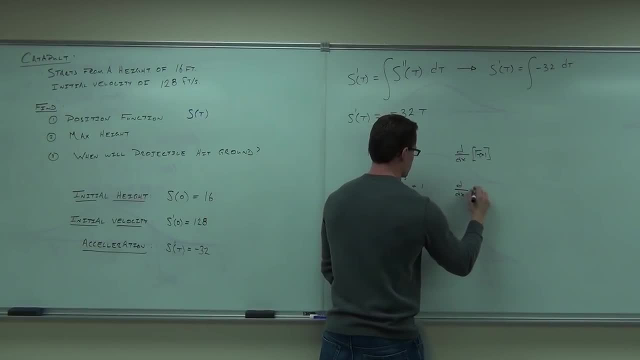 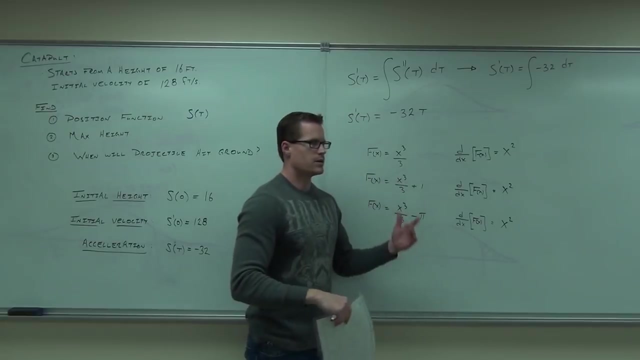 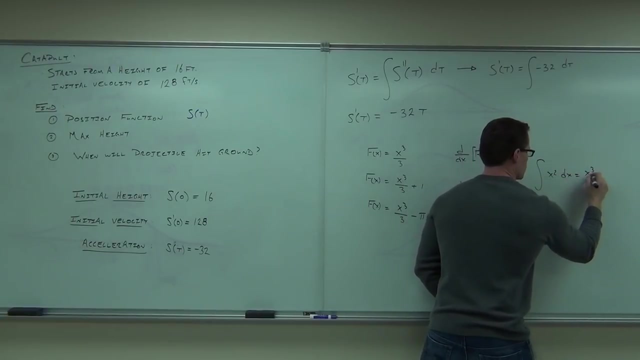 what's the derivative here? What's the derivative here? Square? If you take the integral of all these things, you're going to get this Right. Is it necessarily this one? No, I know that all three of these came from three different sources. 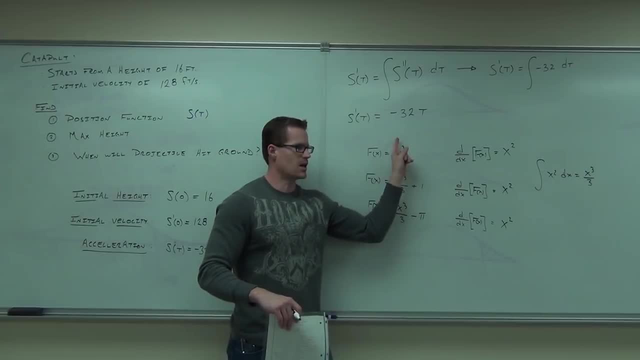 So I can't take the integral of this and get one thing back again. It has to represent all of them. How we represent all of them is there could be a constant over there. That's where the plus C is coming from. That's why we have that. 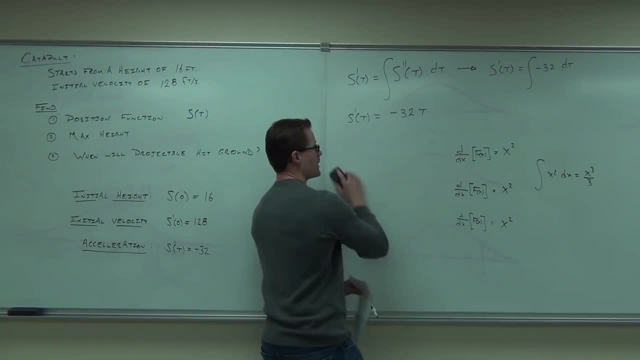 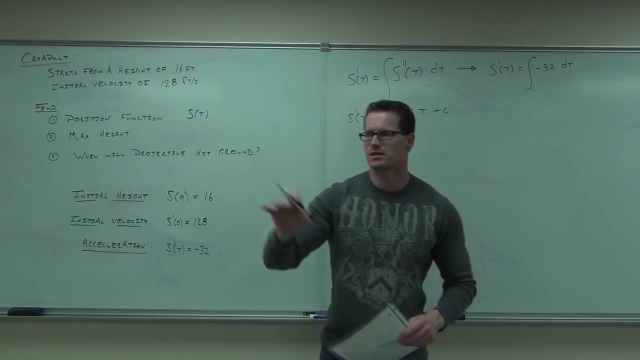 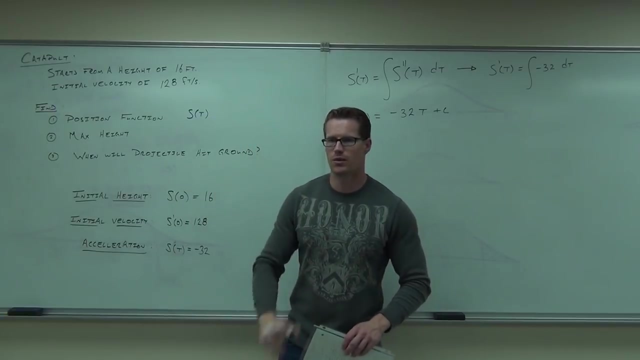 So, anyway, we certainly do need the plus C here. So good, catch on that. Now tell me something I can do. Someone on the right-hand side of the room, Since we have S prime of T equals negative 32T plus C. tell me what I can do now. 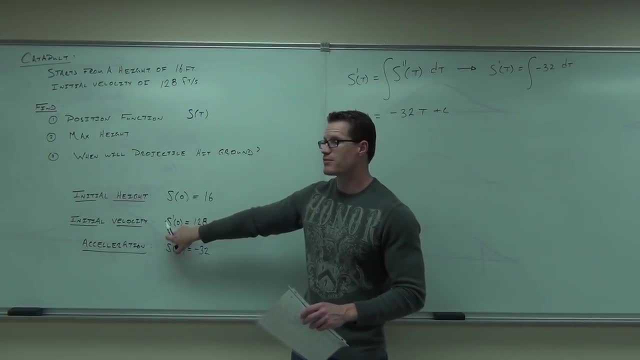 Initial velocity. Okay, So initial velocity. Hey, I have that. It says: S prime of 0 equals 128.. Where does the 0.. Where does the 0 go? Where does the 0 go? That stands for T, right. 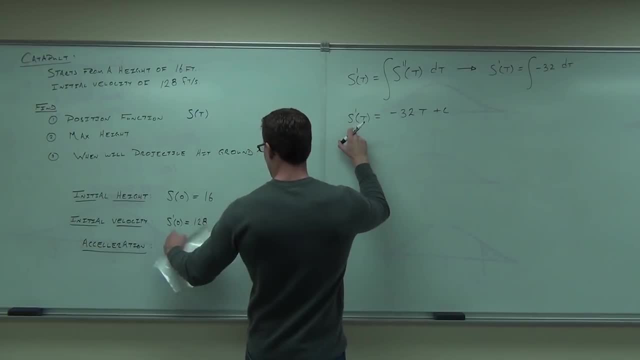 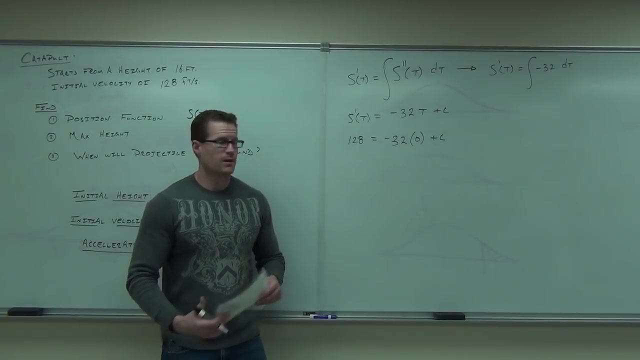 So S prime of T or S prime of 0 says I know the first derivative equals 128 when the T equals 0.. Does that make sense to you? Are you sure S prime of 0 equals 128, right? So S prime of 0. 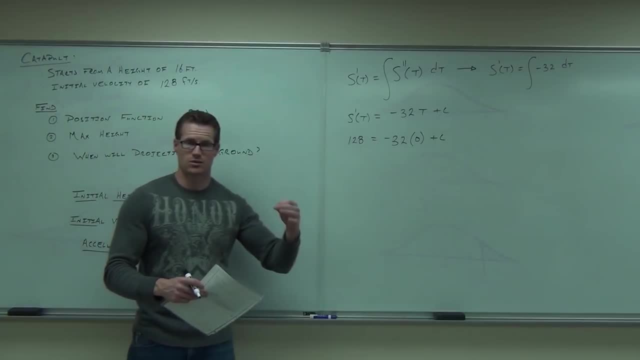 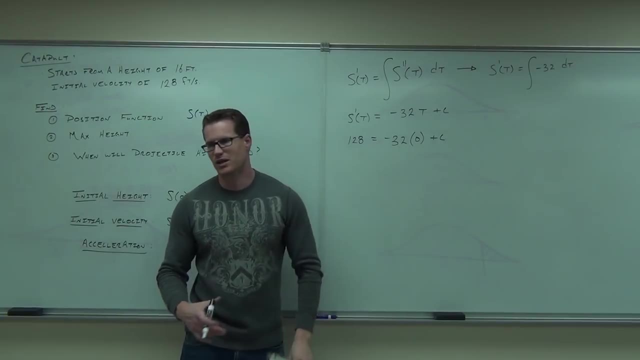 The 0 meant the T, The 128 meant the T, The 128 was the velocity at 0. This means the velocity at 0.. That's 128.. Can you solve for C? That sounds really nice. How much is C? 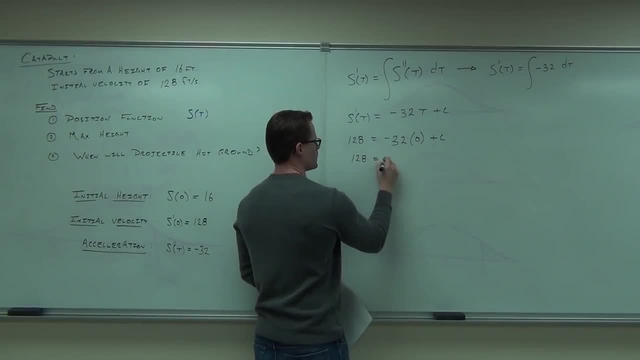 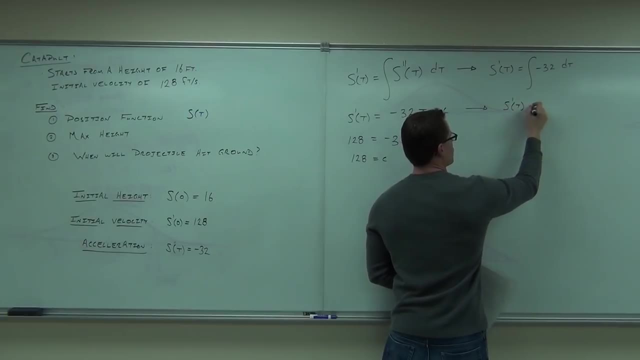 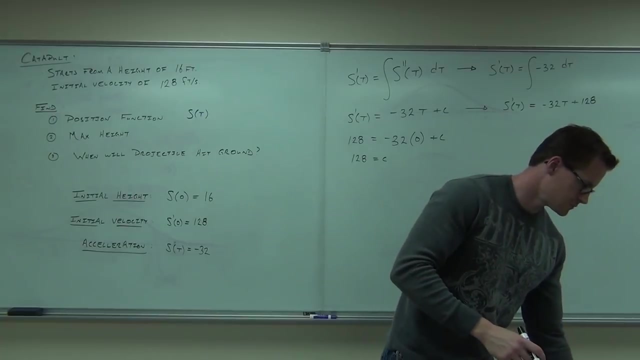 128.. So with a little substitution we have that S prime of T is negative, 32T plus 128.. Okay, So, all right. So that's the answer to question. Oh, is there anything else? You're like neither of you get the fact. 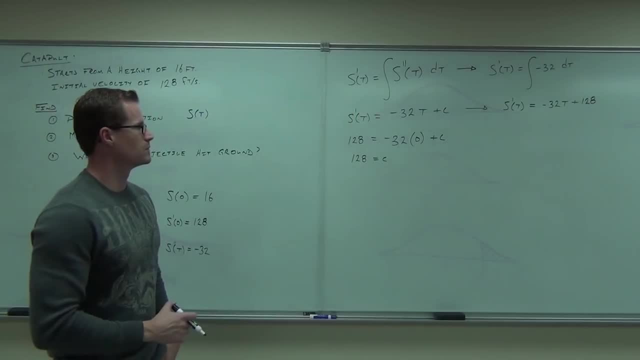 There is another. Oh, we don't get that right. I know that it looks really miserable. Maybe I went all into the math right now. You know my programmed憨 one. Okay, This is the fact. Actually, It says: 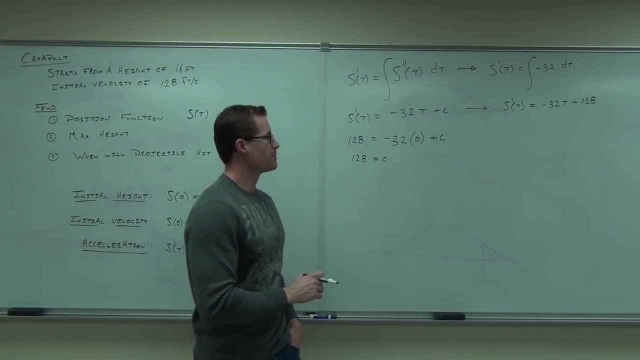 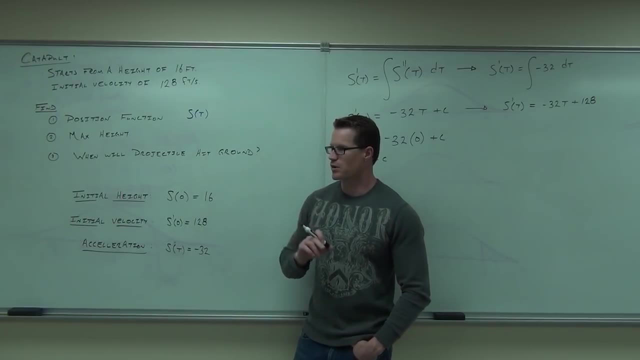 So you're trying to ln, You have the velocity function. It says velocity at anytime, t. Now here's something interesting. Which question can we answer right now? The first one, the second one and the third one? Can we answer the position function yet? 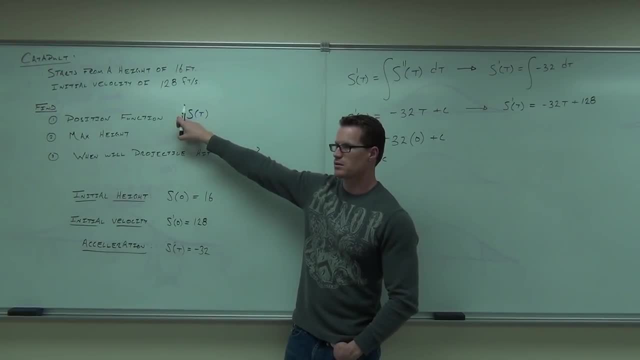 We don't have them on the board. Can we answer the maximum height? yet The things I don't know are kind of messed up. I just want to make height, yet kind of almost almost we can get close to this one we'll talk about. 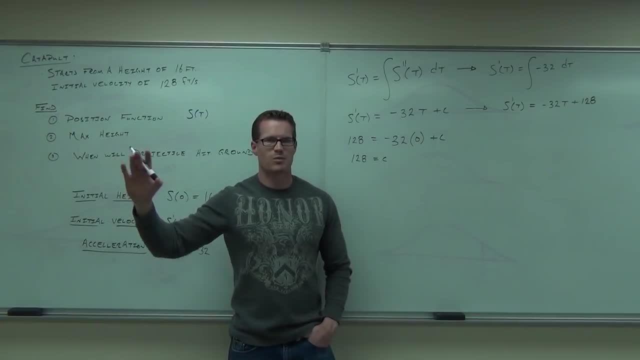 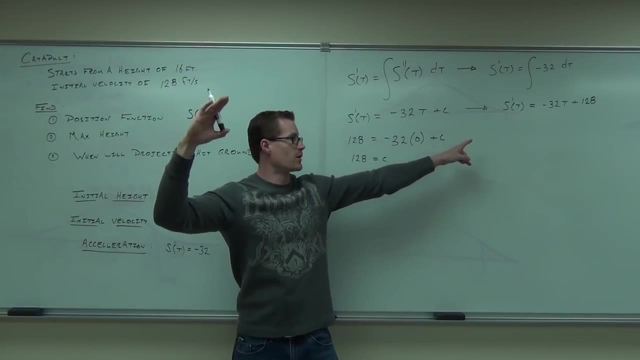 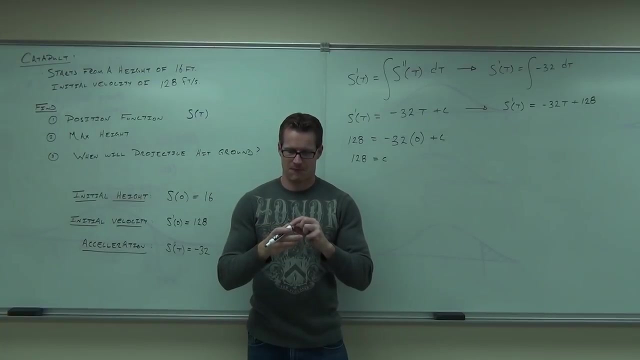 that in a minute, but we're very close to this. why? where would a maximum occur when the slope is zero? do we have a formula for the slope? yeah, we do, it's right there. that's the slope right. so when the book, think about that. when the catapult goes up and it stops, that would be where the velocity would. 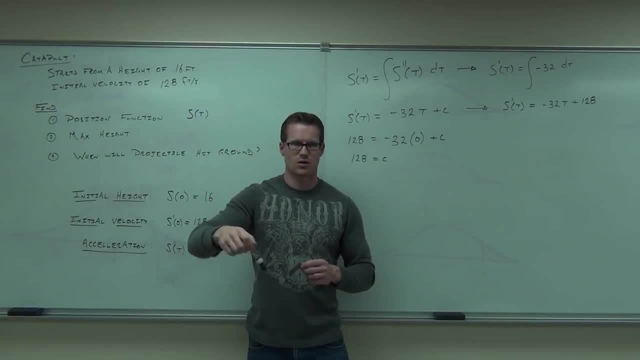 equal zero. right, this is start moving negatively. so, right where the velocity equals zero is where we should have maximum, or in other words, where the slope of the tangent line then it is zero, it's gonna reach its peak and come back down. so that's gonna be what we're gonna be using in just a bit. 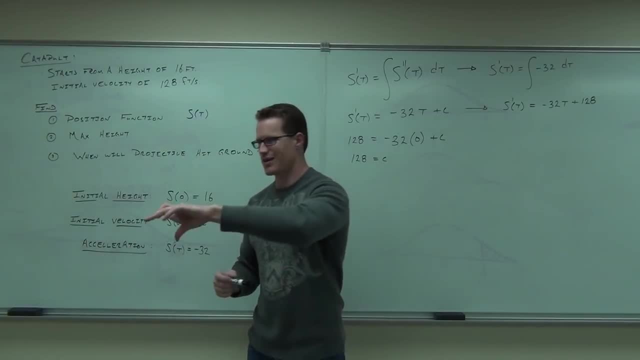 now. before we can actually find the maximum height though, because we're gonna have to plug that number in, we need to figure out the position function, right that? so let's go ahead and do that next part. if we know s prime of T, is there a way you? 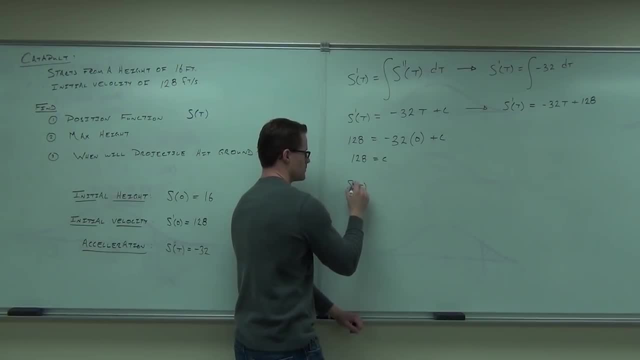 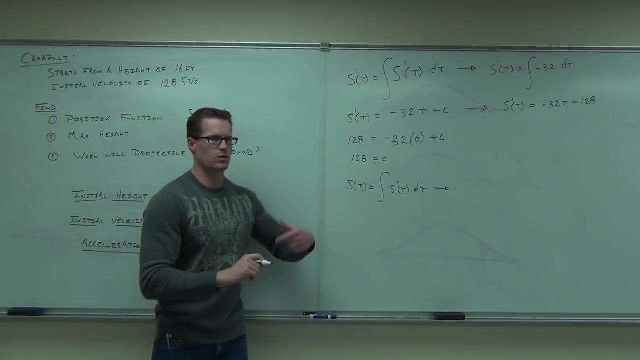 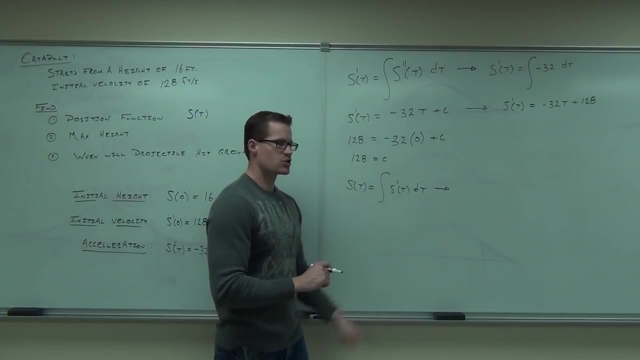 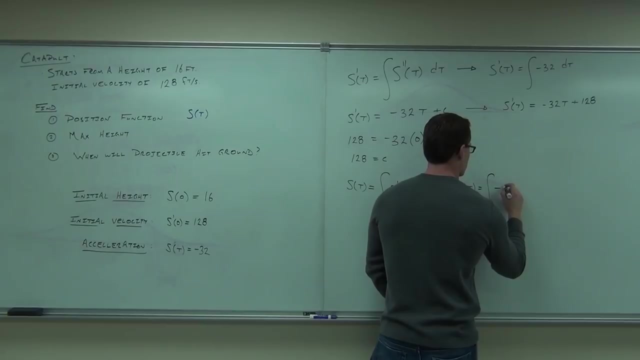 can figure out s of T, our same, our same basic idea, as if t equals the, the integral, that's what of T, and integral will undo that derivative. so, in order to go from our first derivative back to a position function, let's just take any. so that's how we write it. this is said, take the integral of the first derivative. 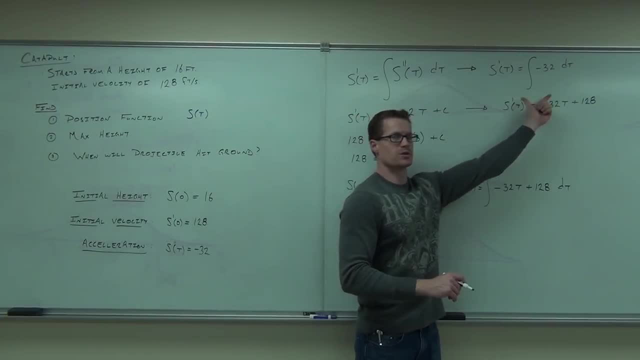 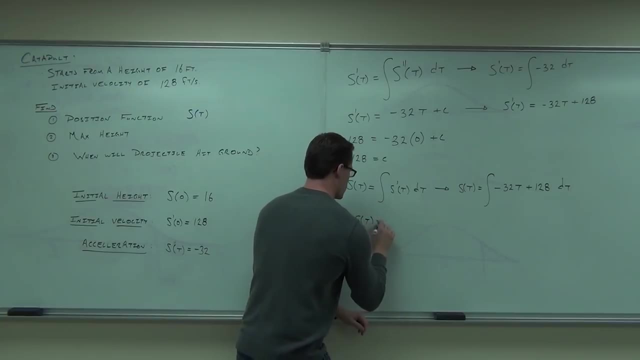 of your position function. this is: This is the first derivative of your position function. I substitute that back in. I'm gonna take an integral of this. Can y'all help me? What's the integral of negative 32t? What would you do? 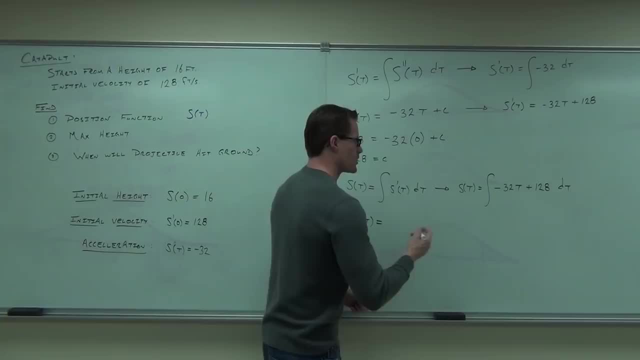 Negative 16t squared plus 128t. Okay, I'm gonna do this a little bit longer, but yeah, you guys are right, I'm gonna do negative 32t squared over two, just so people can see where that's coming from. 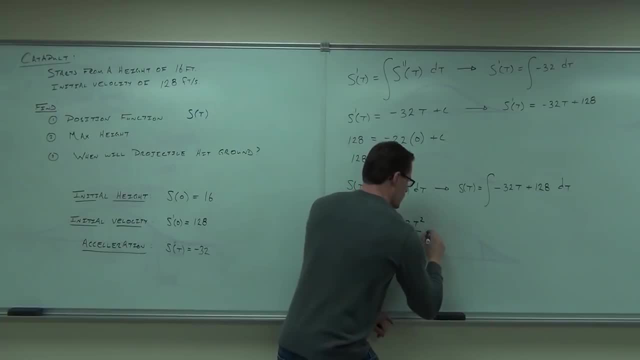 I'm gonna take an integral. I'm adding one to the exponent. divide it by the new exponent Plus. don't forget about the 128.. It doesn't go to zero. this is not a derivative, it's an integral. So 128t. 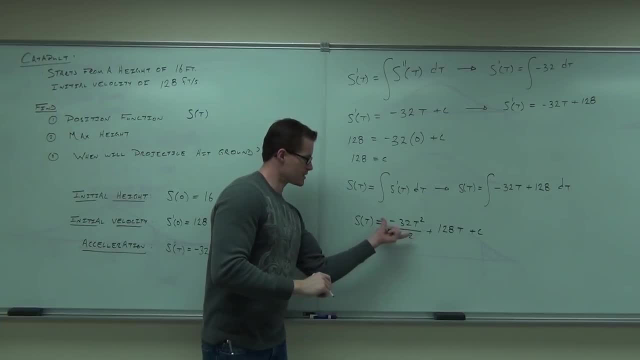 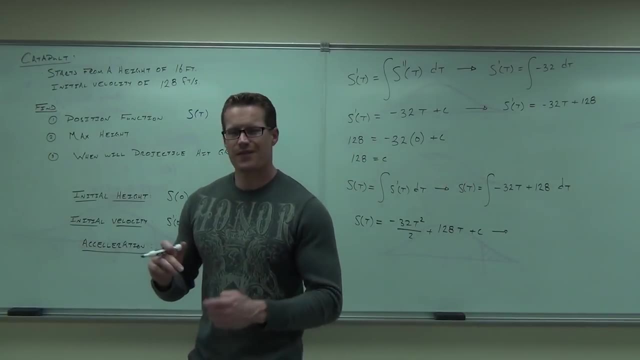 Plus c. Good, plus c. Now, of course, you guys are right. This is gonna be negative 16t squared. In fact, if you've ever seen position functions for projectiles, they always have that negative 16t squared in front of it. 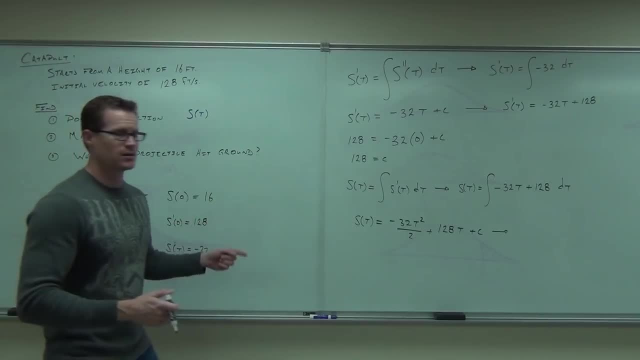 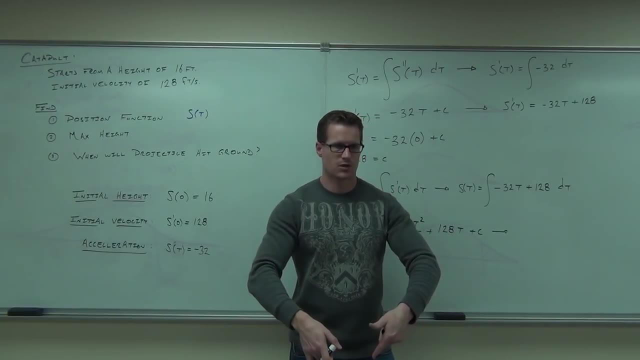 Why? Why, Gravity, Gravity. That's why It's not magic. It's not magic. Someone actually did the work and said: oh yeah, if we're accelerating downward, negative 32t squared. I student about 32 feet per second squared. 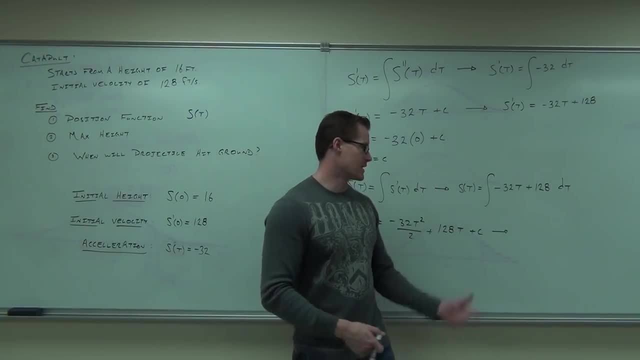 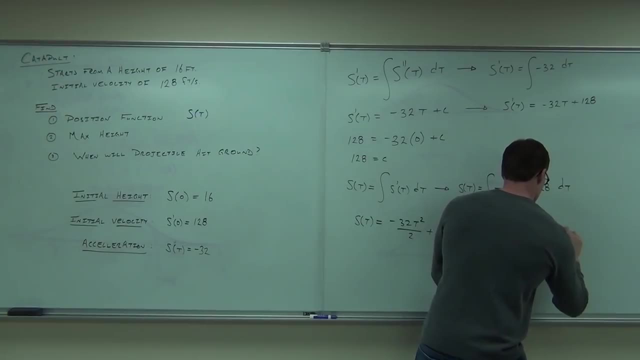 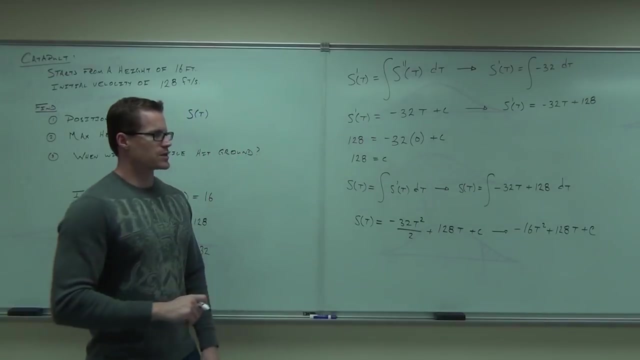 if I integrate that twice, I get a position function. that's gonna be in my problem. Okay, Now tell me people on the left hand side of the room what would be the next step that I would do here. Solve for c. 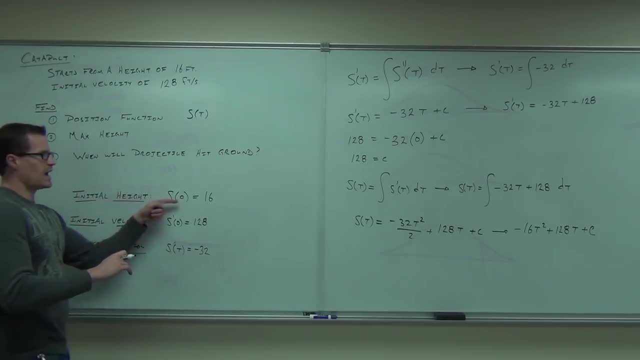 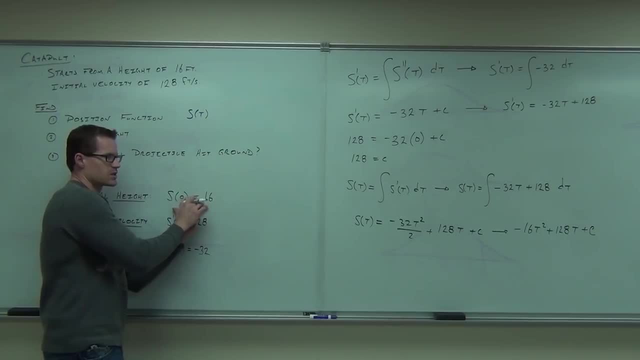 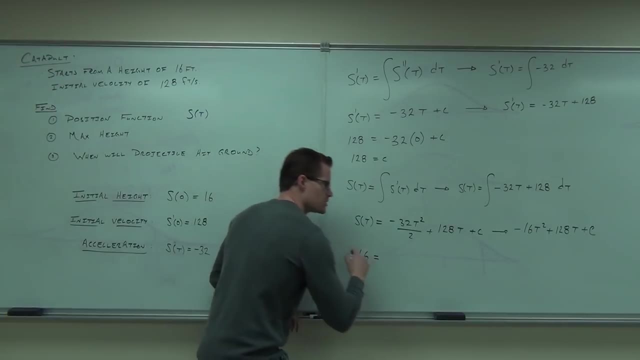 My position at zero. my position at zero is 16.. My position at zero says: plug in zero to your t. This is my position at zero and I knew that had to be equal to 16.. It says: if you plug in zero, look at this what it says. 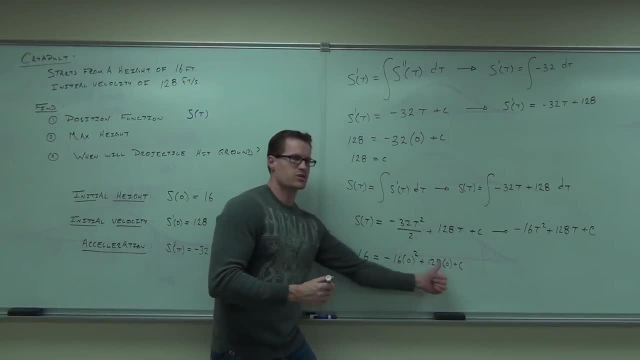 If you plug in zero, it's gotta be equal to 16.. It says: I plugged in zero, it must be equal to 16.. You okay with that? How much is c 16.? Clearly, everything else goes to zero. 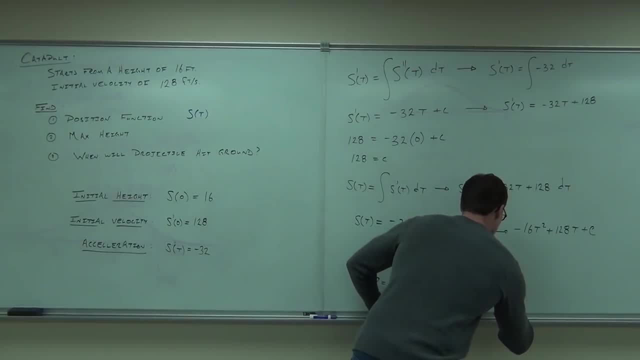 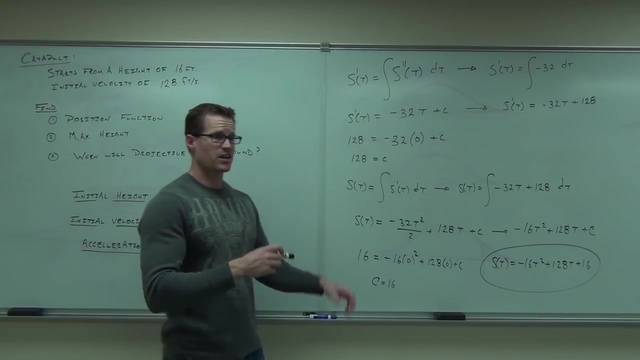 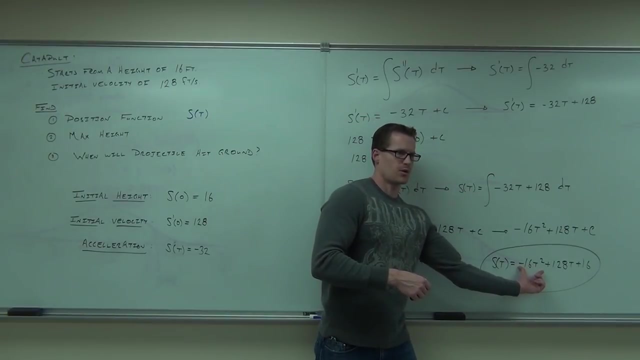 So that means our position function is. that Should make sense. Think about this, diagnose this. What's this from That part? What's that from Second group? Well, what is it from, though? Where does it stem from? 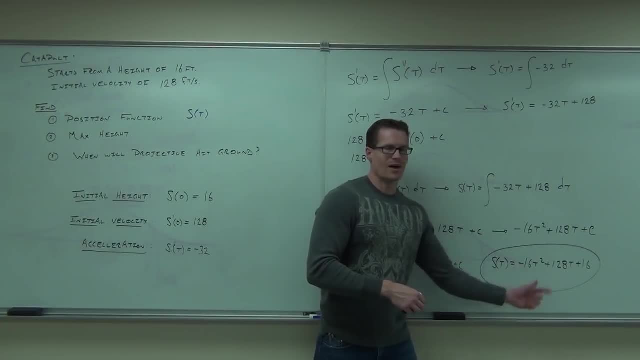 Integral? Well, I know it's integral, but is it from the height, Is it from the velocity or is it from the gravity? Gravity, Oh dear goodness, Gravity. Where did the negative 16 come from? It's from integrating this twice, right? 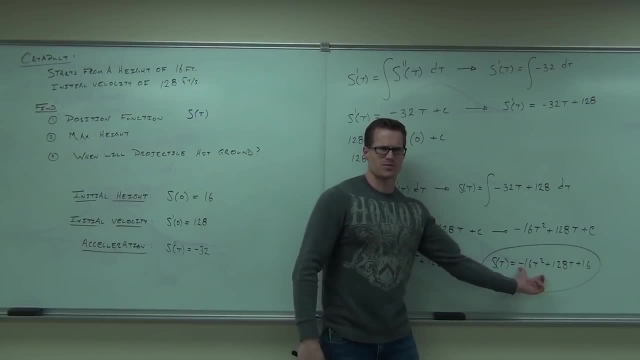 I sure hope so. This part is from gravity. We just talked about that. Come on, people, Some of you are zoning out right now. Stop zoning out. Are you with me? That's from gravity. You integrate negative 32, you get negative 32t. 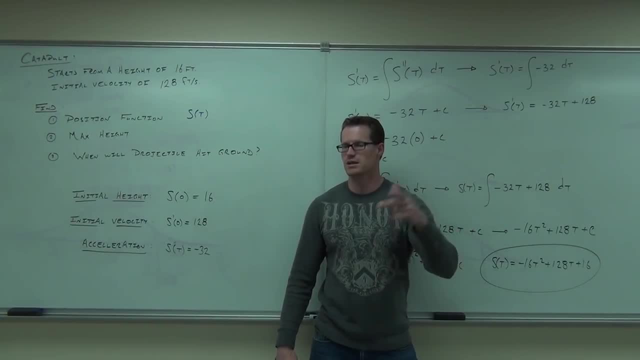 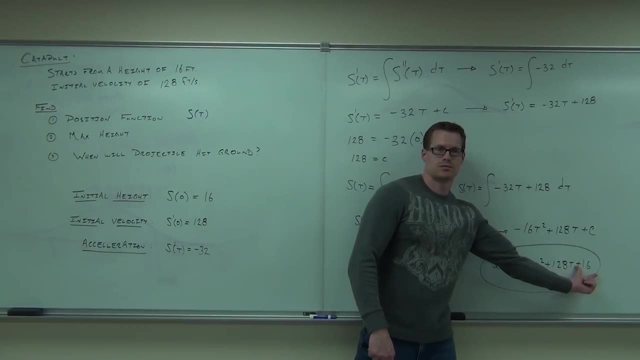 Integrate it again. you get negative 32t squared over two. That's negative 16t squared. That's gravity. What's this? What's that come from? That's the initial height. In fact, if you plugged, in time equals zero. 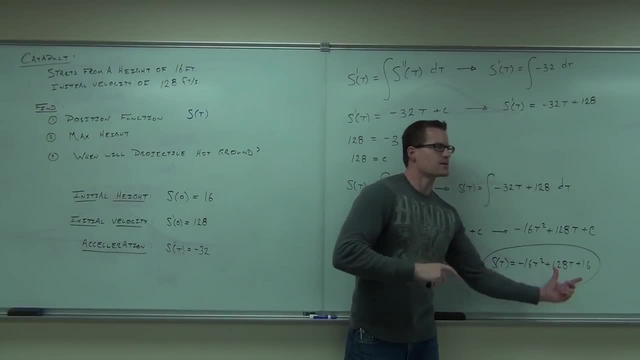 you get 16, right. So you start from 16 feet. What's this from? That has to do with your initial velocity When you start out. what are you at? So, basically, I'm shooting something off and then I'm like: 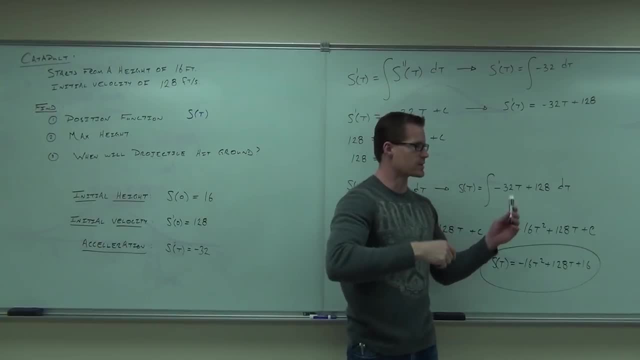 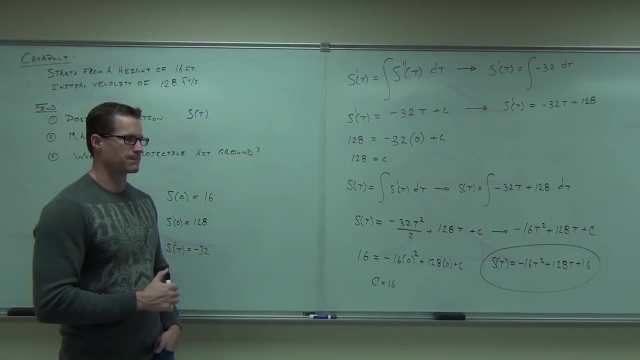 let gravity take its effect on that, and that's what that says. Feel where this stuff is coming from, at least Now. with any type of projectile problem like this, couldn't you just derive the answers? Your initial value is the same. 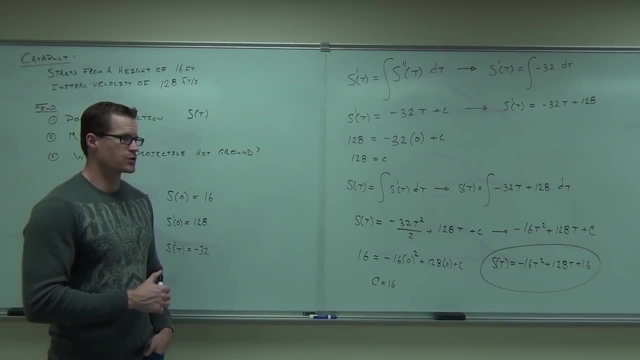 There's a definite pattern between the value and your initial value. Oh yeah, absolutely. All you need to know is your initial velocity, gravity and your initial height, and you can do basically the same thing with projectile functions. Now, of course, this doesn't take into account certain things. 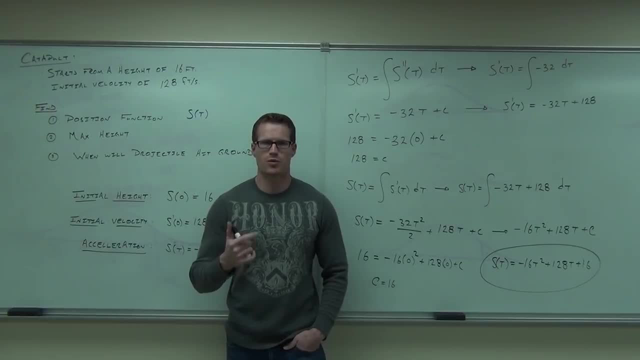 Everything. It doesn't take into account wind resistance It doesn't take into account, like a propellant. So you know how South Korea launched a rocket. or North Korea, sorry, launched a rocket yesterday and it went up and came down. Well, we couldn't model that exactly right, because 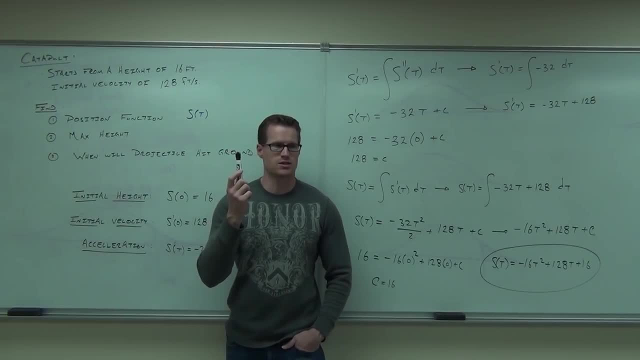 of wind resistance, because it probably didn't go straight up unless they were really just not very bright, Because from what I know you don't launch rockets straight up. That would be stupid. But even if they did right, we wouldn't be able to model it great. 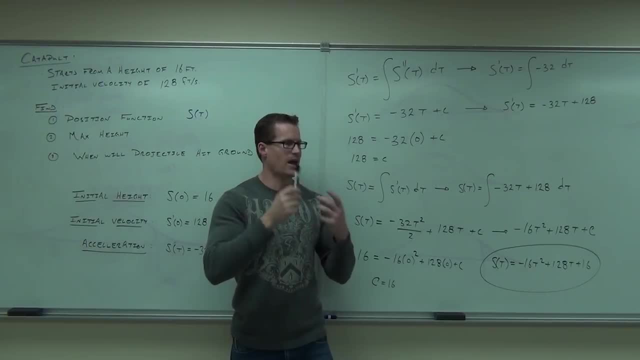 because if they have some sort of propellant that's launching it. you have to take that into account- How the propellant's burning off things of that nature. This just basically says I'm launching it and letting it go. Or maybe the rocket took off and then the moment it took off, 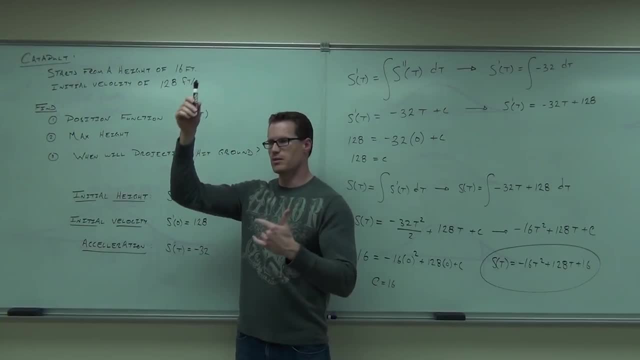 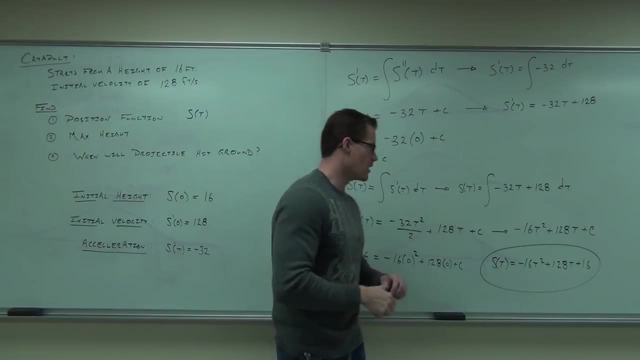 it just blasted real quick and but then it's not firing anymore. That would be a different story. This just has an initial velocity and then we let gravity take its course. There's a difference there. Now we're almost done. We have the first part. 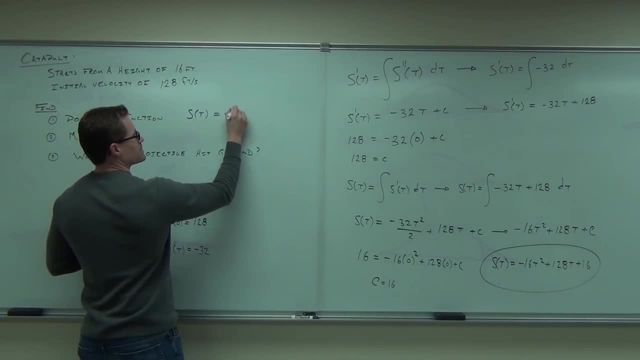 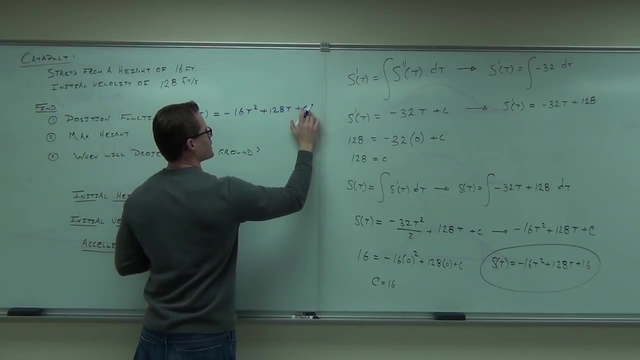 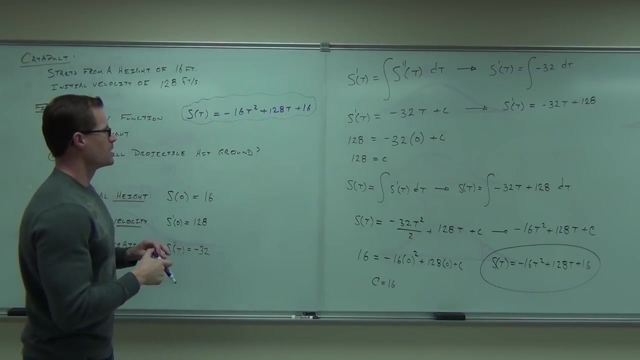 We've got this. We know that this is equal to negative 16t squared plus 128t plus C. All right, All right, We've got C. In our case, C was 16.. OK, Part one done. We can do part two and three at the same. well, not the same time. 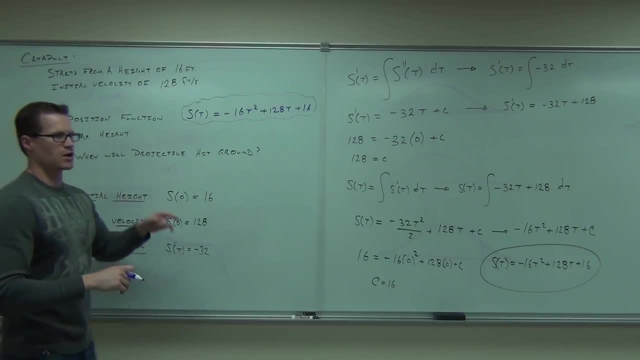 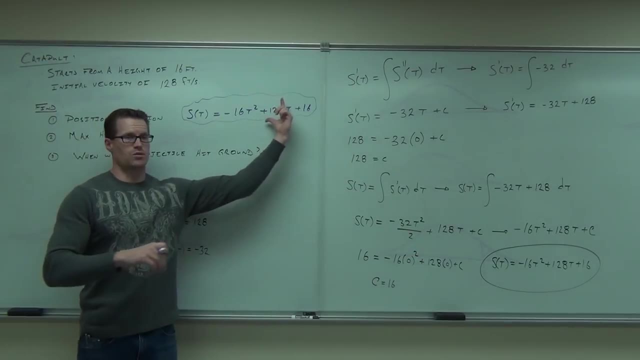 but any time that we want. How would you do part two? Let's talk about that. When would part two happen? Why don't you set it to zero? Set what to zero? The prime of t, Not the position right. 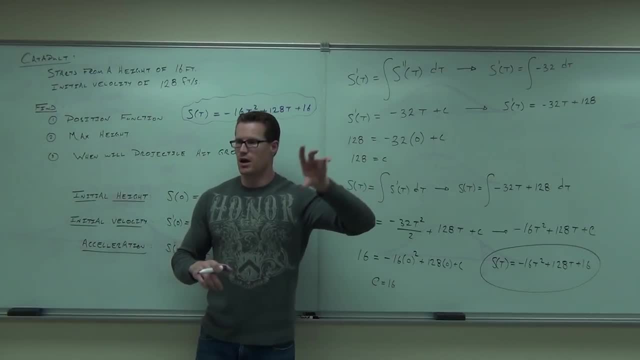 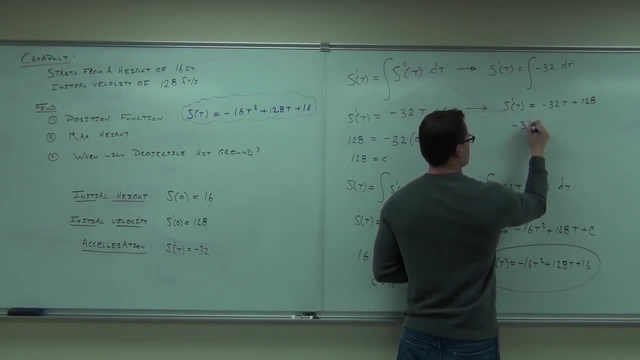 No, That would be a height. The first derivative, though, gives us the velocity. That says, when it's zero it's going to be at its peak. So if we set this equal to zero, 32t equals 128 plus t equal. 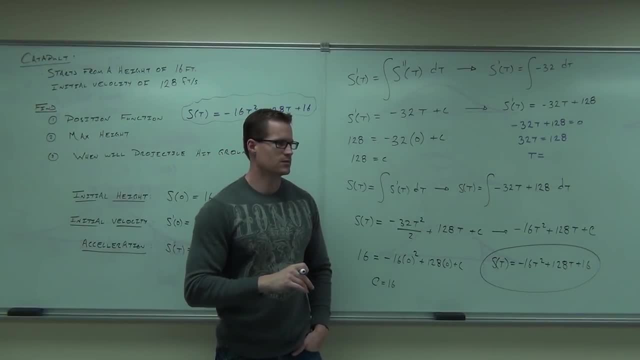 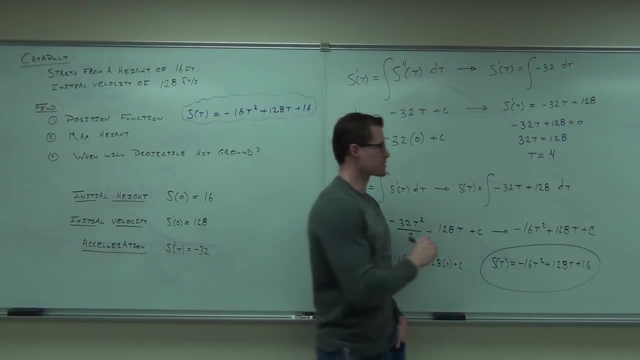 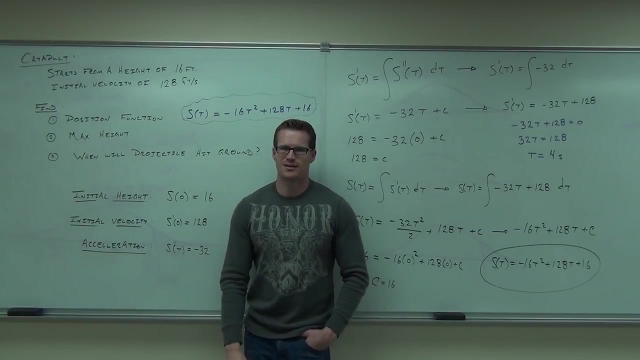 if you divide 128 by 32, executive form: Mm-hmm, I love it. For what? Second? Second Second, Because t is a time second point. So what's your maximum height? Is it four? 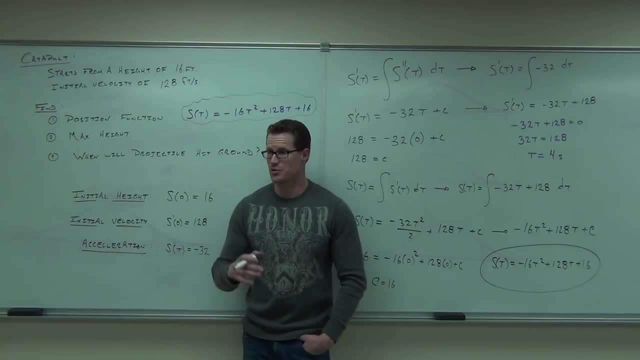 No, No, That's four seconds. How would you figure out your maximum height? Here's what you know: Your maximum height occurs after four seconds. So after four seconds you're at the maximum point of your height And then you start dropping. 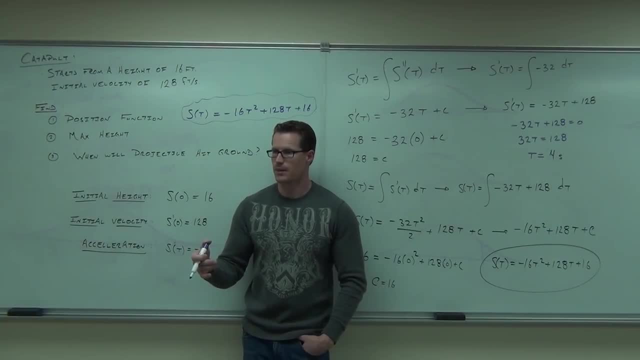 How would you figure out the maximum height? Plug it in. Plug it in where In your position, The position function? Yes, That's why we had to figure out the position function first, so that we could actually find the maximum height. We could have found out when it is the maximum height very easily. 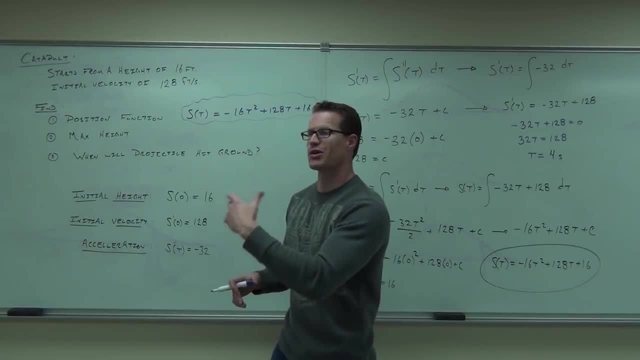 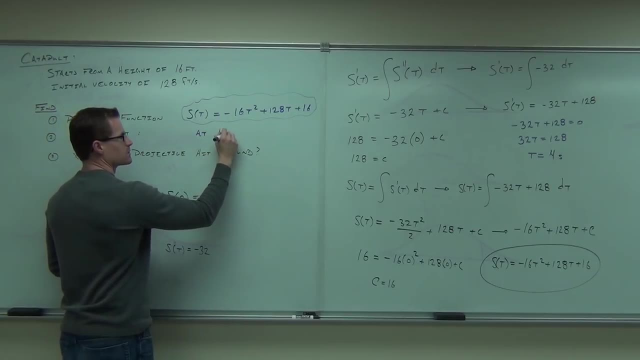 As soon as we had that we could have done it. But to figure out the actual maximum height you've got to have something to plug it into. So maximum height occurs at four seconds. Can someone please plug that in for me into my position function. 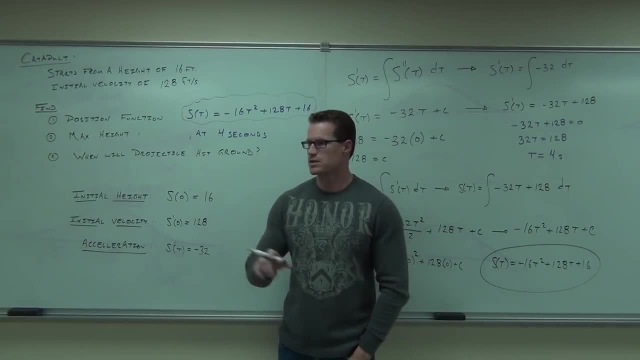 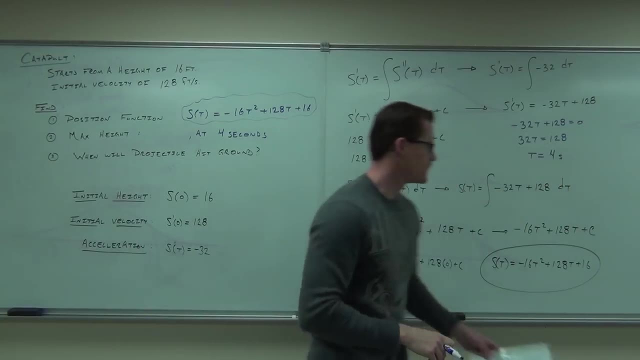 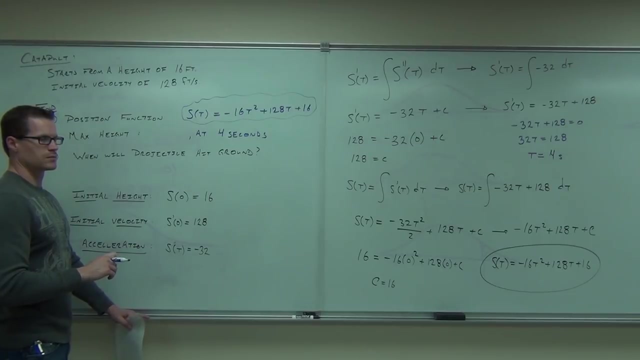 And find out exactly how high we get 784.. 784 feet. Someone else double check that for me. 784 feet, please. It's probably going to be a whole number. So what this says is that your catapult you built is going to launch something from a height of 16 feet. 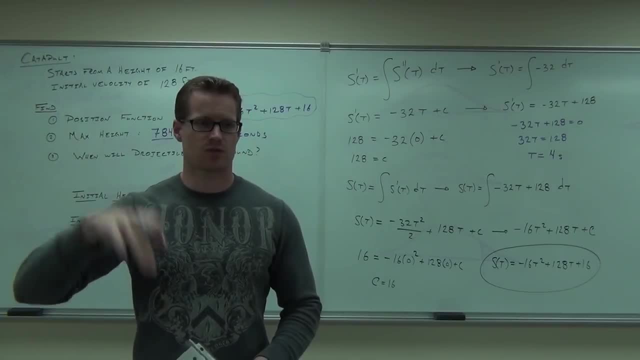 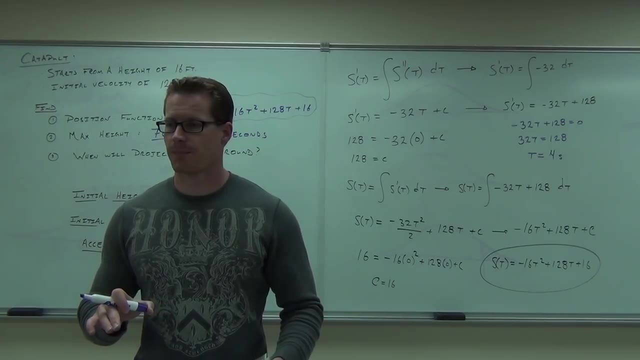 It's going to go to 784 feet- That's after four seconds- and it's going to start dropping like a rock. When is it going to hit the ground When the acceleration is zero? Acceleration is never zero, It's a constant. 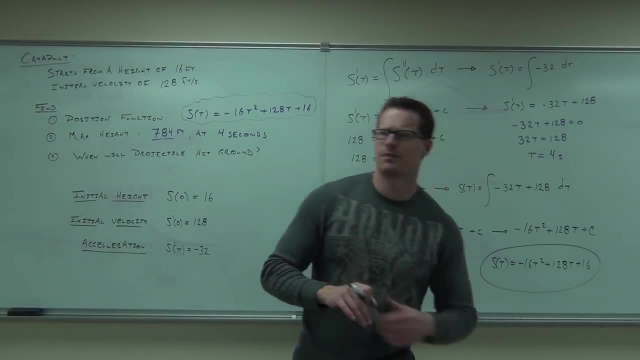 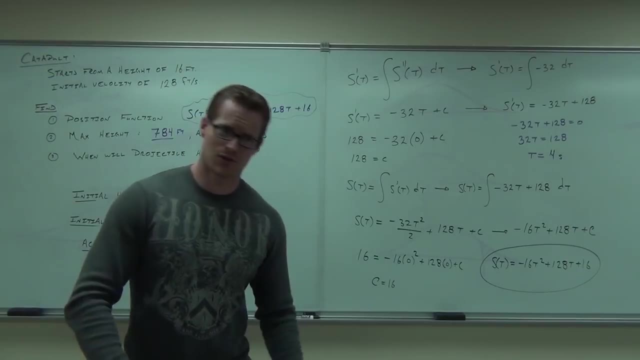 Or what is Zero, Zero? Hey, let me ask you this question: What is the height when you hit the ground? You understand the height. If you fell on your face, your face would be at zero when you hit the ground, right? 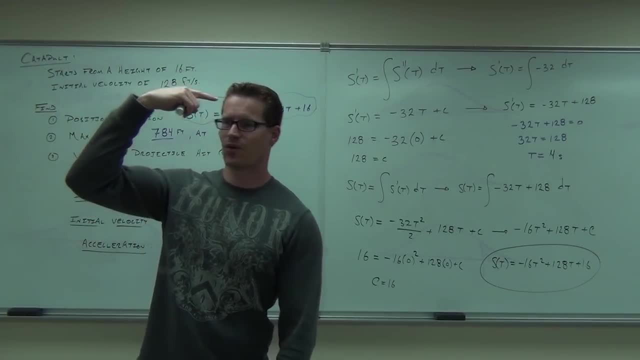 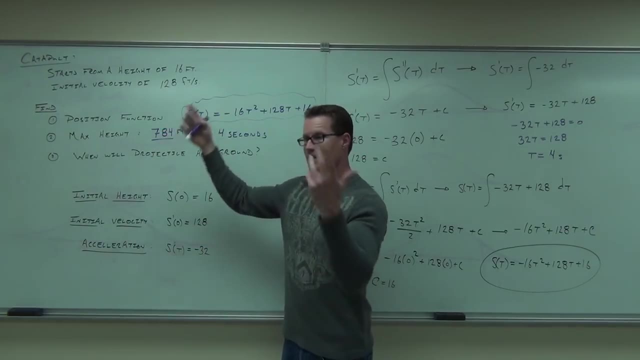 Right now, my face is at six, six feet, And then it's going to go And I'm going to get zero feet off the ground. Does that make sense? Now? which one of these represents your height? Is it the position, the first derivative? 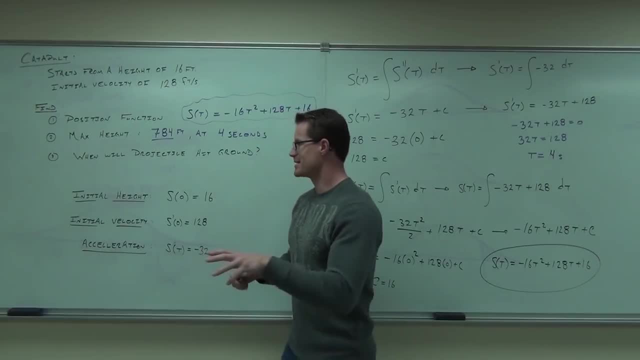 or the second derivative, Your position. So what this says is: What? When does this equal what number Zero. When does it equal zero? This is actually a intermediate algebra question. We just did this today. I just taught this in another class today. 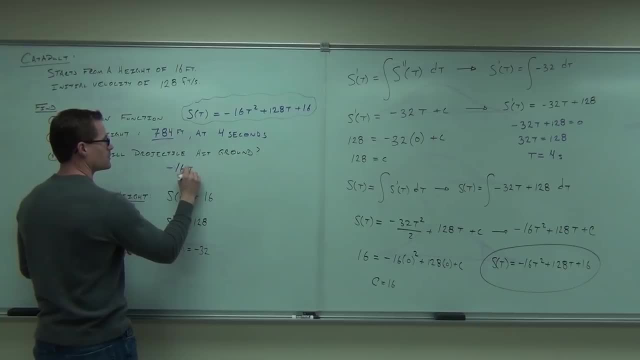 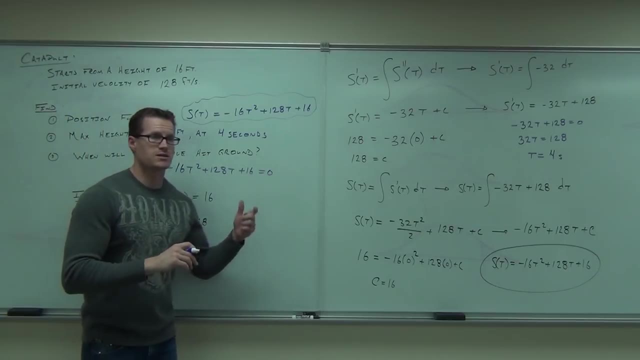 It says: take this, set it equal to zero, solve for t. That's going to give you a time. In fact, it's a quadratic right. It's going to give you two times. Do you see the two times that I'm talking about? 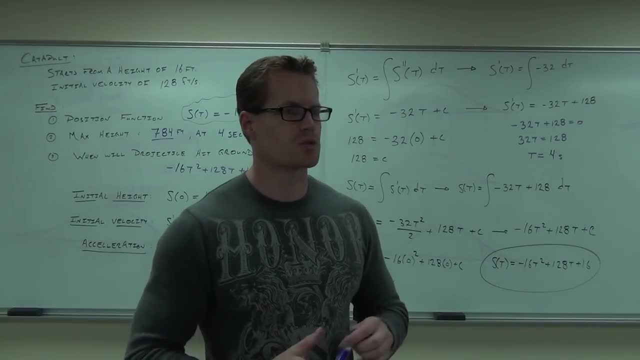 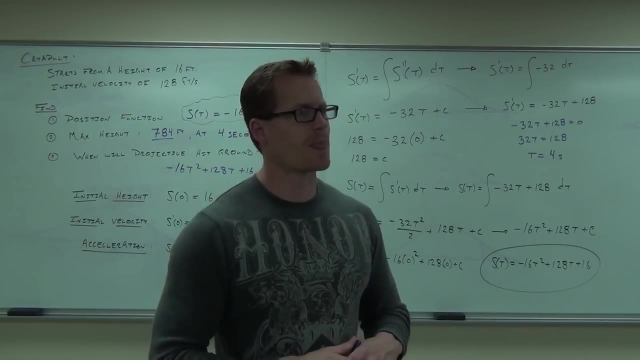 One will be positive, one will be negative. You're going to take those two times. Which one is going to make sense for this problem, The positive t or the negative t? Positive t: Well, some of you guys are not with me today. What makes sense. if you're going to hit the ground after some amount of time, A negative time, Can you launch a catapult and it hits backwards in time. There you go. That'd be pretty sweet. I'm sure North Korea would have loved that. 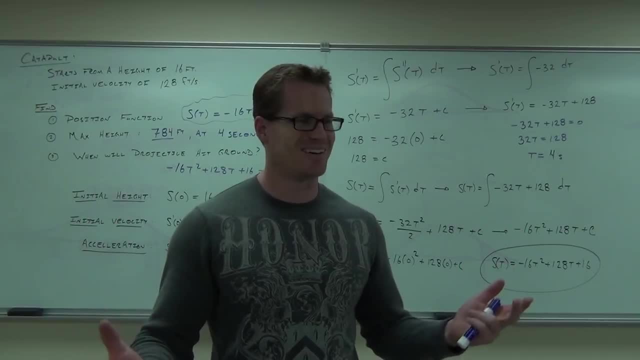 I launched it and it hit them in the past. Ha ha, ha, ha ha ha. They would have won the Korean War. They would have won Yeah. so that doesn't work. So what we're talking about is in your quadratic. 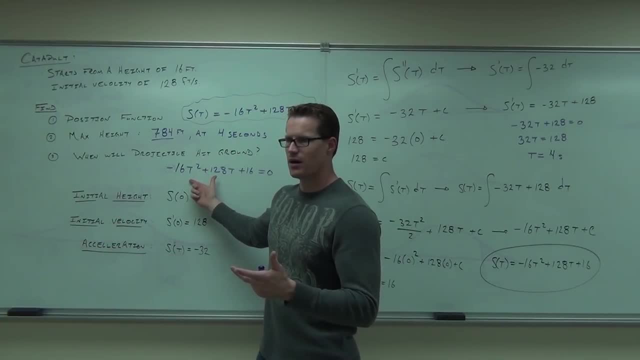 when you use quadratic formula or whatever, you're going to get zero. Whatever you want out of that thing, you're going to set this equal to zero. That's not right. That's not right. That's not right, It's two. 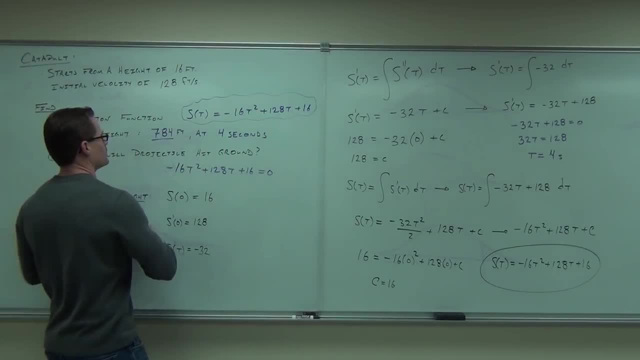 Why'd you both give me that? then I forgot Two people get it's negative. it's 270.. You didn't do negative 16.. Oh yeah, 272.. I can't believe it's been driving me crazy. 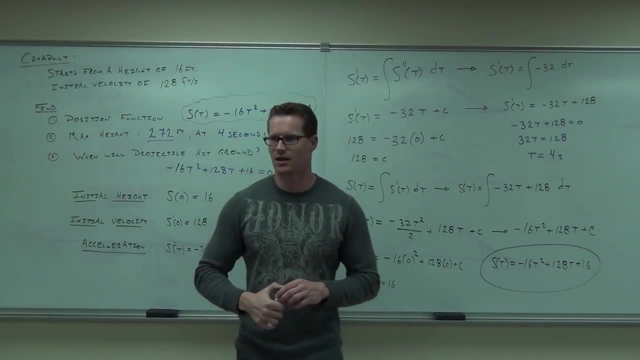 272.. How do you calculate if people make simple mistakes like that? I'll never get it. I don't understand. We have good intentions. later You know what you match. Yeah, Enough with good intentions and bad. follow through A bunch of crap.